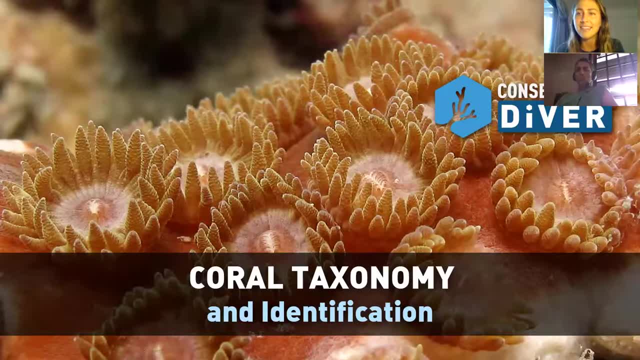 that coral. I know that that's the one that looks like an earlobe or you know something like that, And it is this sort of interesting way to remember things. And for me, the other thing that I personally do to remember new Latin taxonomic names is often I'll just write them down over. 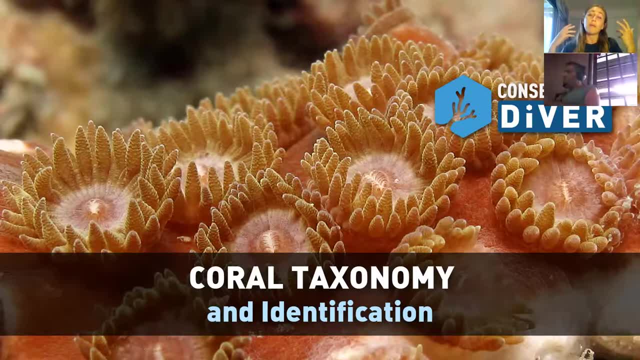 and over again, which I know seems a little bit boring, But if you are one of the people but really do need to or want to get around this sort of topic and it's important to you in your career- it could be anything- biology, really, or anything that involves you know a new language. 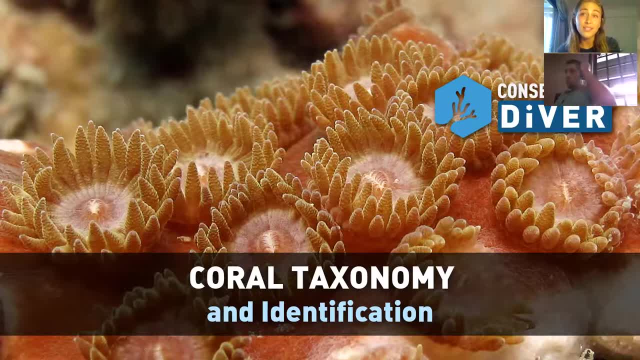 that is, I guess, sort of layman's, then I would recommend trying it. So for me. when I am learning new names, I like write them down over and over again. Here's some of the pages of some taxonomic names I was just trying to learn myself for some gastropod species that I was totally unfamiliar. 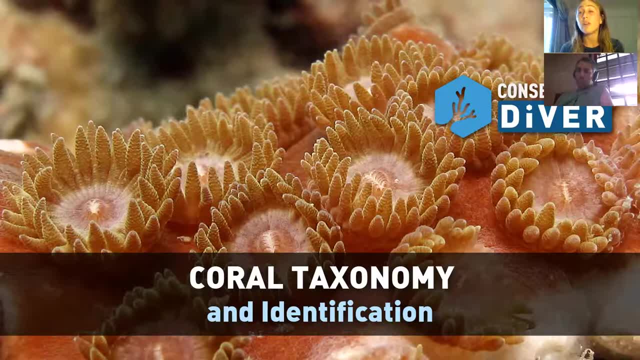 with And you kind of do seem like a little bit crazy writing them down over and over again, But for me it really really works And I've gotten some of my students to try and they sort of say it's annoying and it's time consuming, but you do get them stuck in your head once you've had to go. 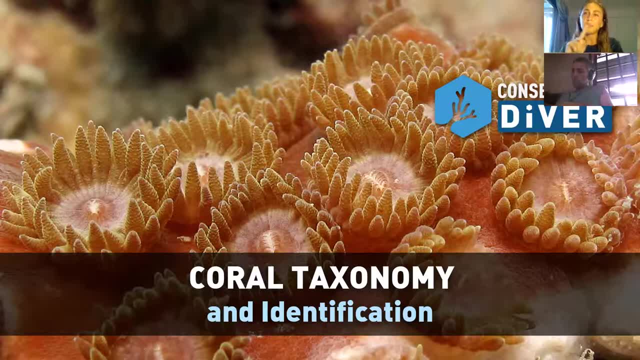 through that motion of just copying them over and over again, And the other PDF I showed you guys was just some extra resources that I would very highly recommend. Worms is a world register of marine species And, as some of you guys may be diving into taxonomics, you might want to take a. 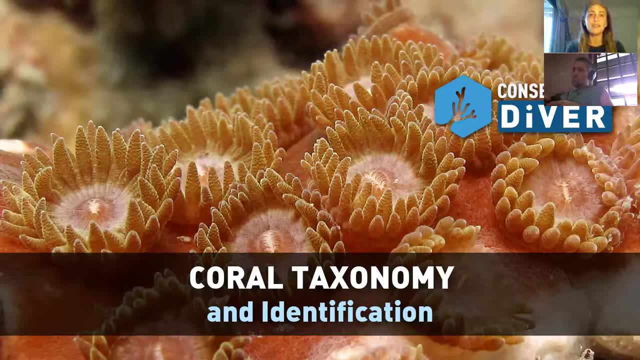 look at that as well. So if you go into taxonomy more and more as your careers or studies progress, you'll notice that a lot of names within you know taxonomy, especially within the marine world, sort of getting juggled around- And I don't mean juggled around, pretty much We've recorded things. 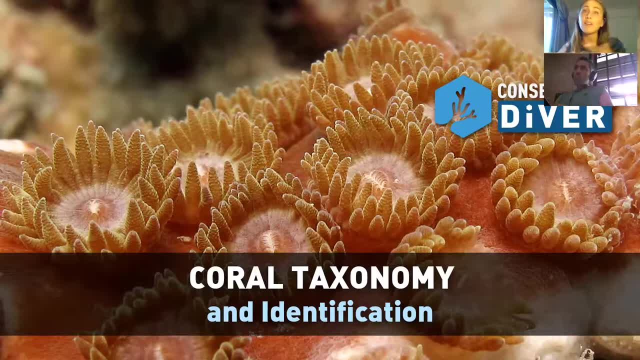 as one species, perhaps in the past, and use morphological features to do so. And as technology is advanced and we might be gaining more access to, you know, to genetic testing, we're realizing that we've made maybe a few mistakes in the past and we can more accurately place them in a 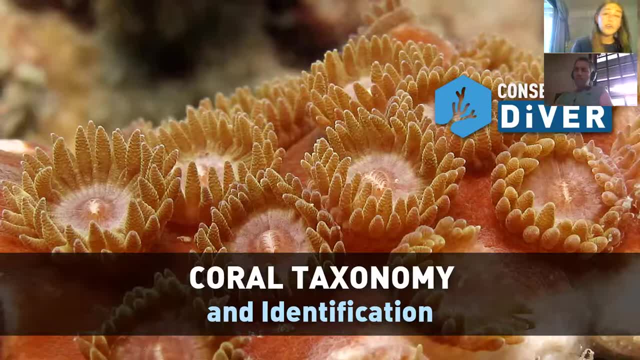 phylogenetic tree, which is really awesome. So World Register of Marine Species is amazing. If you ever want to double check a name, check that you've got the spelling. see its relatedness, you know. see its classifications all the way up to phylum. So very useful. Another one that 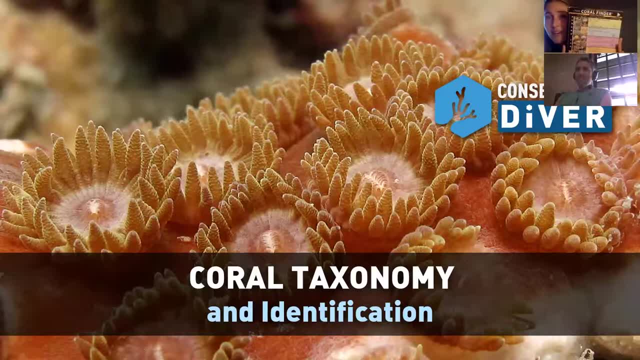 I highly recommend is The Coral Finder. I've got one myself and it's my favorite book ever. Okay, This is just. it's the shit. It's so good And it's incredibly easy to use. it's color coded, So if you are in the Indo-Pacific, I would recommend getting your. 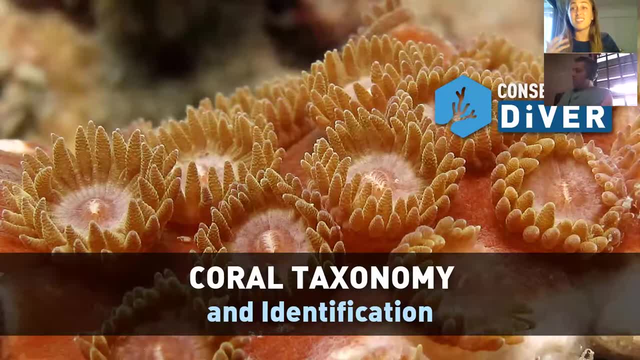 hands on one of these. They're a bit expensive, which is annoying, but I actually would say it's worthwhile. But a lot of centers that do sort of a lot of you know, conservation work and education, will often have a copy or a few copies of this book, And so they should. 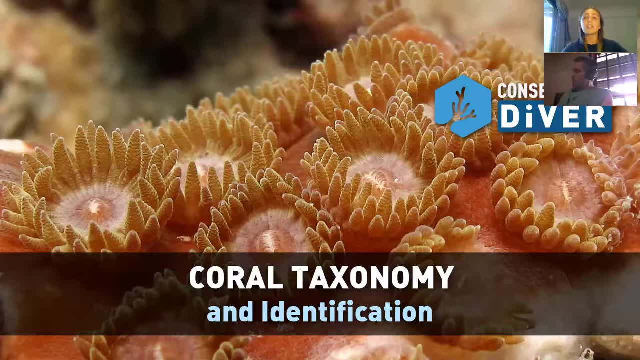 So yeah, also after this lecture, if you guys have any questions related to coral taxonomy, if you took a photo on your GoPro and you want to help ID it, send it through. I love this stuff. My email is at the bottom of that PDF sheet, but also my email is just lconservationdivercom. 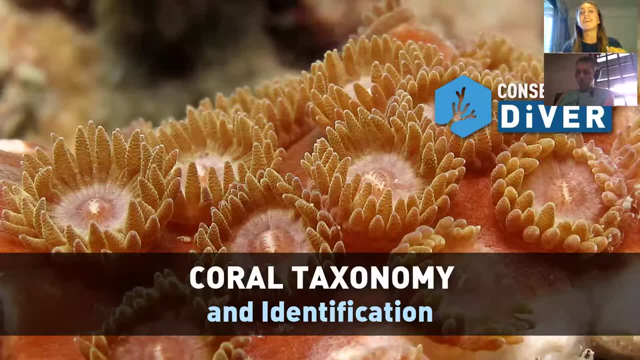 So it's pretty easy to remember. Anyway, so that was our introduction, I suppose Now let's get down to it. Can everyone still hear me? Give me a thumbs up or like one of those you know reactions: Awesome, Cool, Getting them from a couple of you guys, That's fantastic. So welcome. Coral taxonomy. 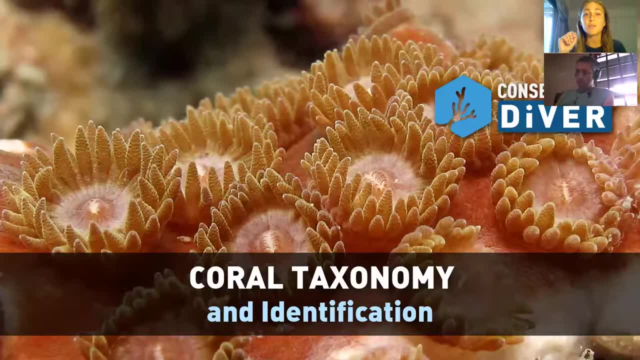 and identification. So first I just want to express why this is actually an important and essential part of conservation. It's more obviously an essential part of monitoring. When you monitor things, you know being able to record them to the most amount of detail. that 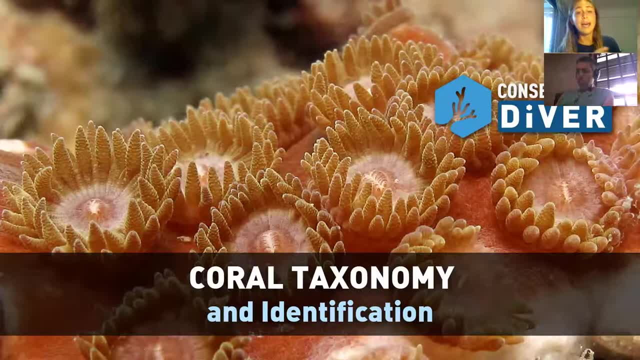 you can is obviously more ideal than having less detail. How do we apply that to conservation? That's obviously something that we at Conservation Diver are doing. We're applying active restoration to our work. So I've just got a question. I haven't changed slides yet. I'm so sorry. Who was that? Oh, it just says Zoom user. I am just 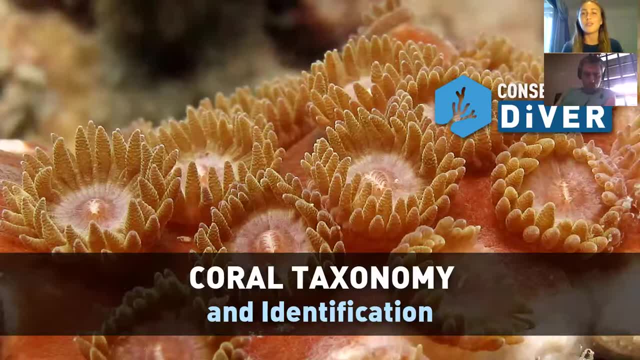 still on the first slide. Sorry, I took a while to introduce everything, So your screen's not frozen, I assure you. But yeah, so essentially, when it comes to applying taxonomy of corals into conservation, it's really important to know what corals you're. 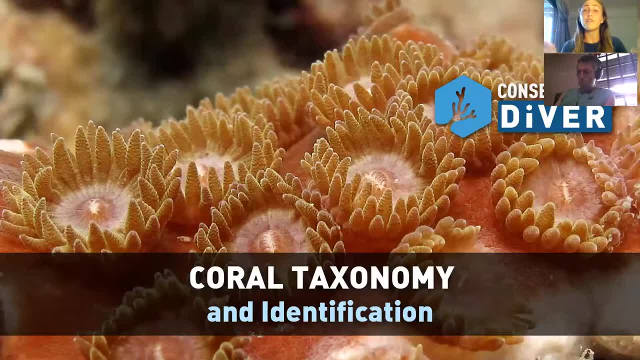 dealing with, as opposed to saying, hey, we've got this reef and this high coral cover, It's good, We don't really need to do anything. What having an understanding of coral taxonomy can help you with is understanding the level of diversity which exists within you know your restoration area. 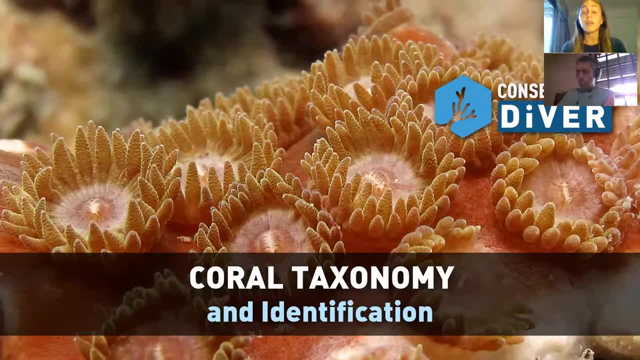 whether that be one bay or one island and so forth. Well, I used to work. I was on an island called Koh Tao in Thailand, which I know that some of you guys have been before We. our base was in an area called Sherlock Bay and it had really really high coral coverage. 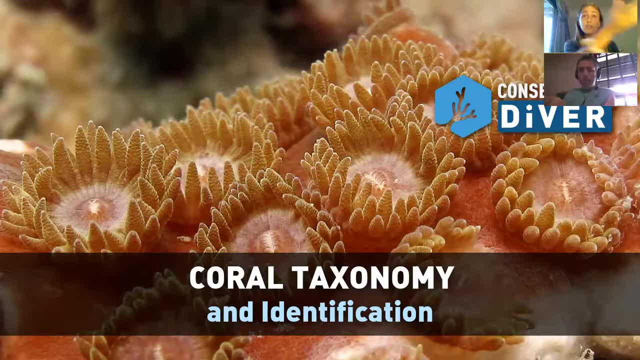 And a lot of people thought: you know what's the need for restoration? here There's all this coral. You know what's the problem? But the fact is it was pretty much monospecific stands of acropora and a few other specs of different genera floating around the place, But it didn't have a lot of 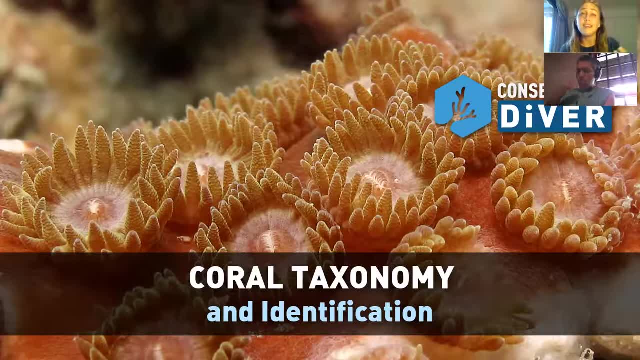 diversity, So it's actually very susceptible to coral. So it's been really fun to work with, to take a look at, and because coral is very resistant to diseases and also storm action and other events like that, And often we did find outbreaks of. 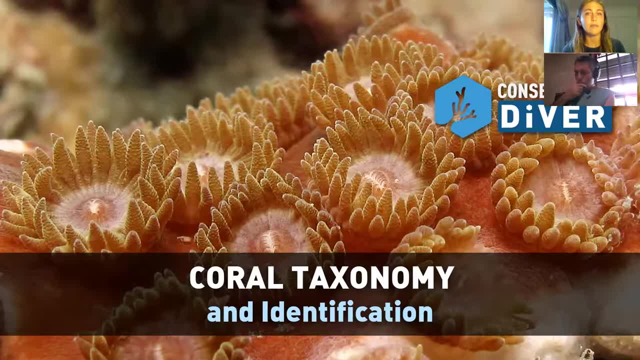 diseases and coral predators within this bay. But yes, that's just one very simple example That being able to understand that you know coral coverage is one thing. you know 100% coral coverage is good, But if it's 100% coral coverage of a single species, then you might not have a 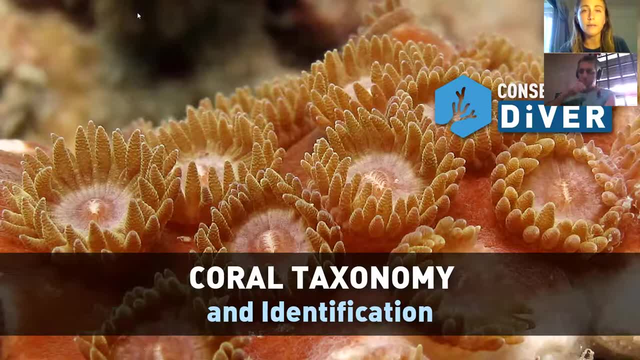 very resilient reef. So also today. oh, I'm just going to admit someone, Brad's back Here you- He must have dropped out there for a moment, Awesome. So oh yeah, that's right. So during this lecture, we are gonna mostly focus on identifying corals. 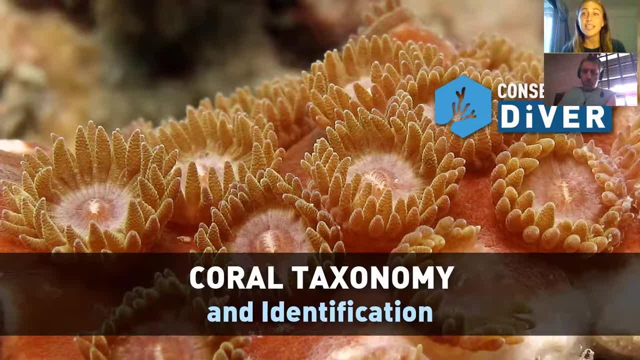 to a genus level, And that's because genus level is quite reasonable. Hey, Aiden, you all right, I'm good, I'm good, how are you? Yeah, good thanks. Oh, someone's not on mute, Okay so. 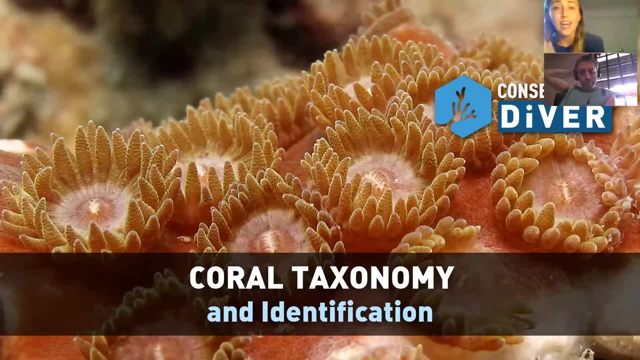 oh yeah. so when we're making in the field identifications, often it's quite realistic to be able to ID them to a genus level, whereas to a species level can be a little bit tricky. You sometimes might need genetic samples, or you might need a skeletal sample and a microscope. 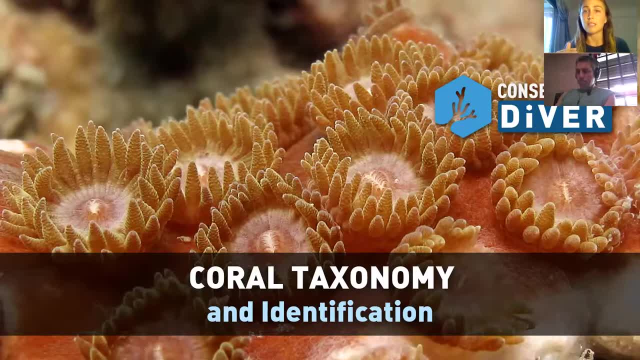 So we do focus on IDing things to a genus level cause it's just more realistic. And, of course, getting to the most specific level of diversity of taxonomic classification is better than just saying hard coral or the branching coral or the bouldering coral. 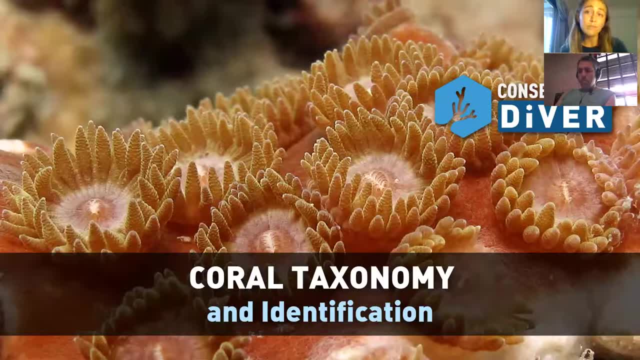 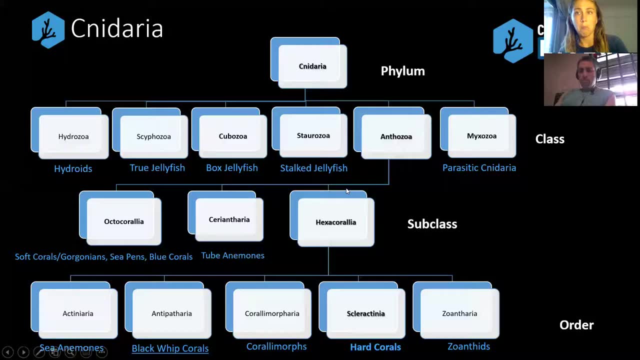 So, yeah, any questions so far. If not, we'll actually properly start getting into the lecture. There we go. Cool, yeah, there we go. So what are we focusing on today? We are focusing on hard corals. So if we look at this sort of graph here, 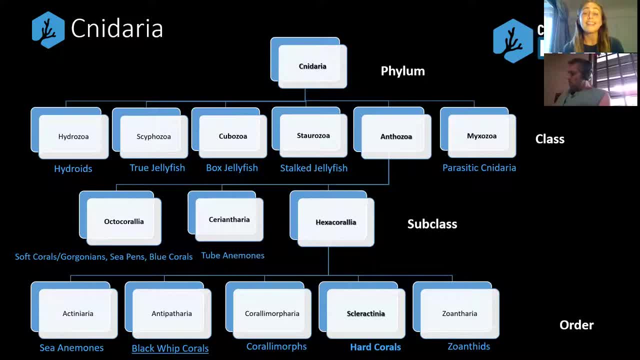 we can see at the top of the phylum which hard corals fall under, is the Cnidaria, the Cnidarian phylum, And this includes other animals such as your hydroids to your. oh, that's right, I've got my pointer. 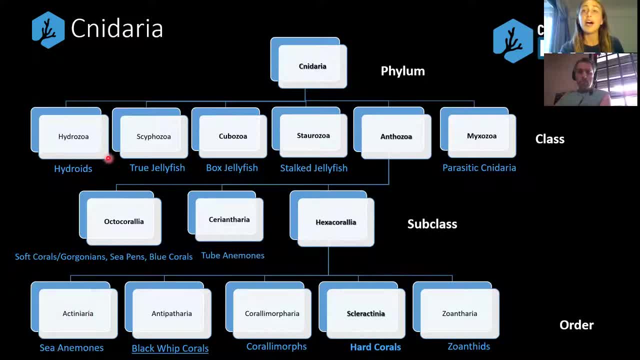 I don't have my pointer, laser pointer. We've got our hydroids, as you can see to the far left. So some these are very small animals, generally speaking. Often they'll grow on things like mooring lines Sometimes, if you ever you know. 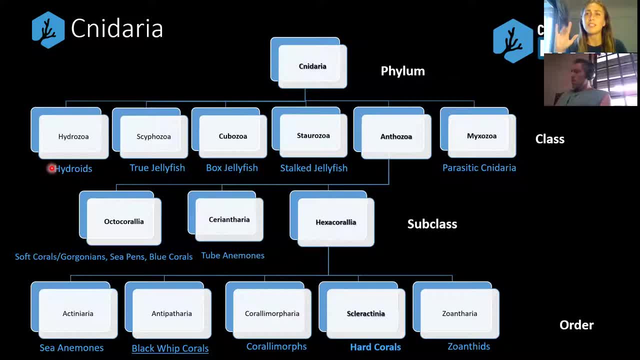 maybe held them to a mooring line on your safety stop and then going to the surface and your fingers were a bit stingy, then that's because you were probably actually touching some hydroids by accident. You can call the Cnidarian phylum the Cnidarian phylum. 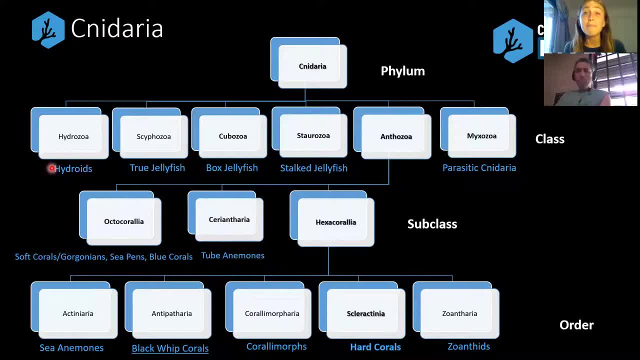 the stingy phylum, if you really want to, because you know, nematocysts, or stinging cells, are one of the things that all of these animals that we're talking about have in common. okay, We've also got different varieties of jellyfish. 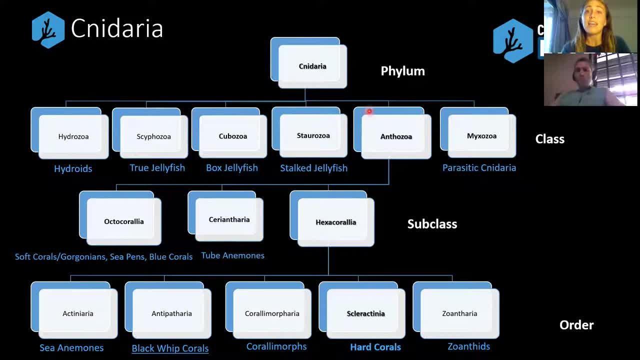 These also fall within the Cnidarian phylum. okay. If we go to the next step, we are looking at the anthozoa. okay, Which have our hexachoralia, which includes our hard corals or sclerotinia. 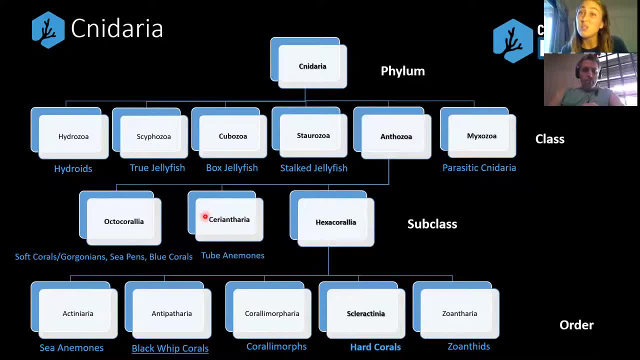 Anthozoans also include ceriantheria, which has tube anemones. Sometimes you find them in silty muck ecosystems. They kind of do look like tube worms. often they're called- And then also your octochoralia. 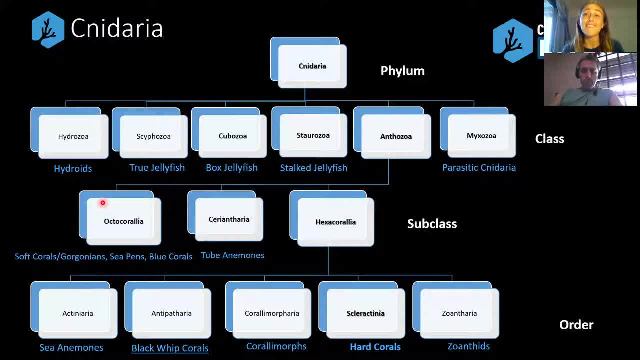 which is your soft corals, which are identifiable as having eight tentacles per polyp. Okay, This also can include your gorgonians and sea pens and blue corals as well- Blue corals not being blue, but having blue skeletons. 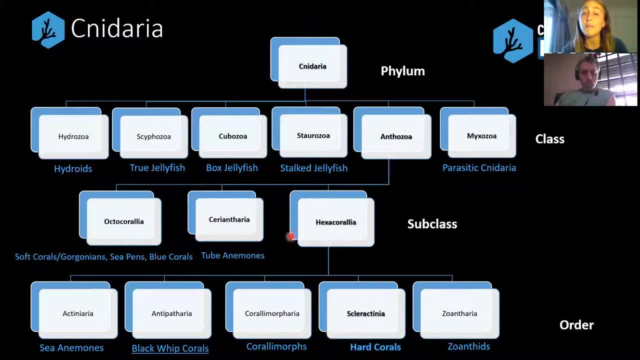 All right. So next step: we do have the sclerotinia and within the hexachoralia subclass with the sclerotinia, we have zooantheria, which is like your zooanthids, which we're going to look at in a moment. 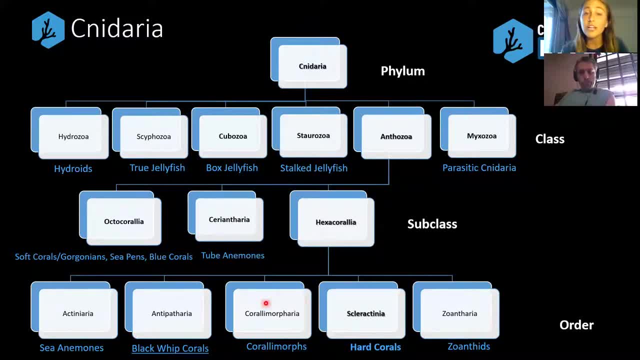 because they can be easy to mix up with hard corals. We've got our corallimorphs also a little bit similar looking, So we'll look at some photos of them in a moment. Our antipotheria, our black whip corals. 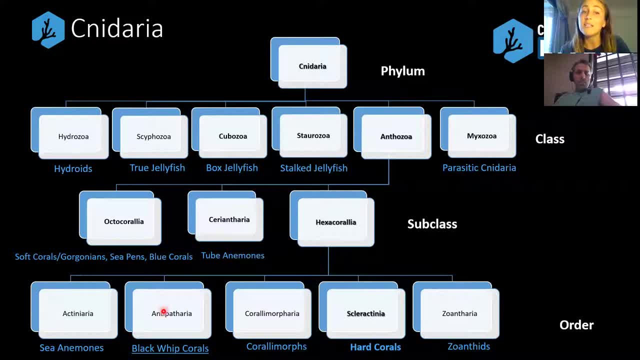 this is underlined because it's currently being revised, So antipotheria hasn't sort of been confirmed by you know the best in the field of taxonomists or that particular group. We've popped it in there because thus far it has been quite official. 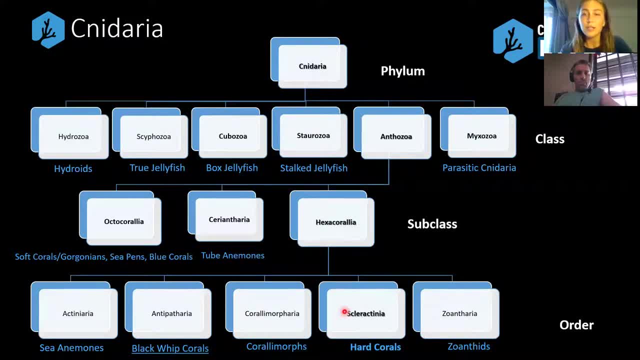 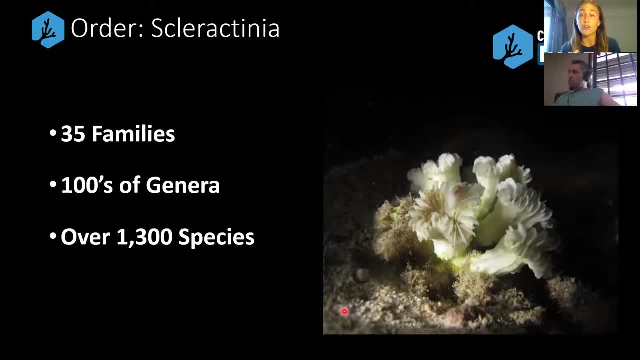 And the actinaria, which is our sea anemones. Okay, So let's go a bit further. So, within the order sclerotinia, we've got 35 families of corals. Within that there are hundreds of genera. 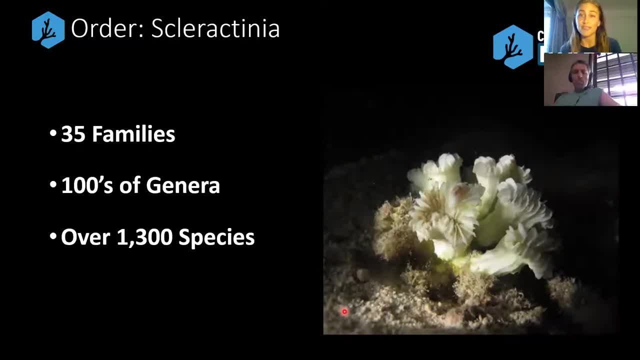 and within them there are over 1300 species. So again, just for the sake of practicality, I deem things to a genus level. as opposed to, you know, as opposed to a species level is also a bit more realistic. 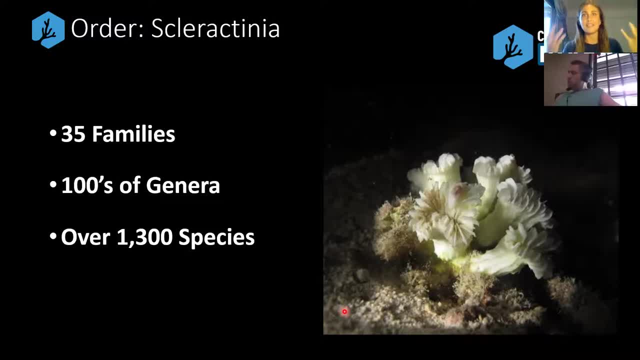 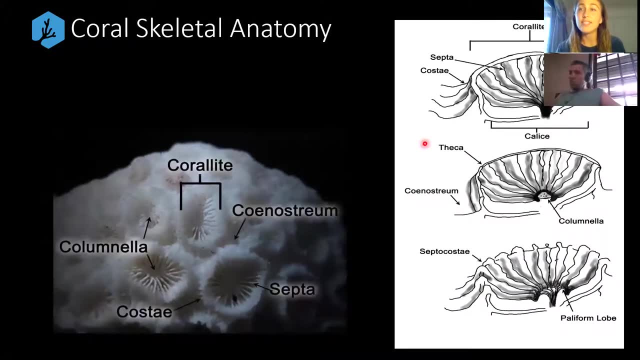 in terms of just you know the size of your brain and how many Latin taxonomic names you might actually be able to fit in there. Okay, So let's just quickly recover or go over coral skeletal anatomy, which I'm sure a lot of you guys. 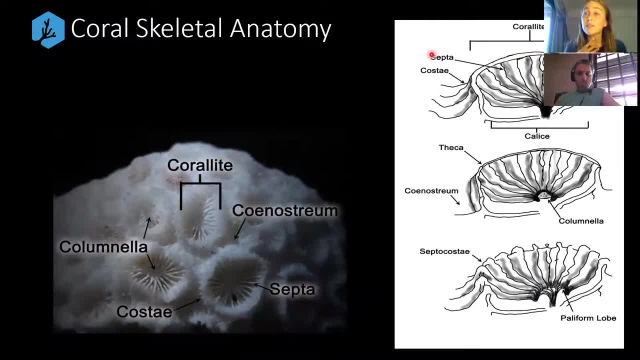 will have a basic understanding of, at least if you've done maybe any of our courses or if you just have a general interest in corals or coral reefs at all. So we have the corallites which you can see- I'm pointing to the real photo here- but also this and this and this are all different variations of a corallite. 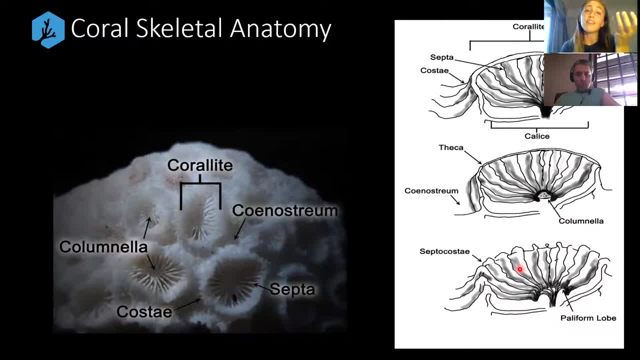 You can think of it as the cup-like structure in the coral skeleton that the polyp- that being the living animal- sits on top of, And they're layering down calcium carbonate and pretty much thickening this up as they go. But the corallite is where all the action is. 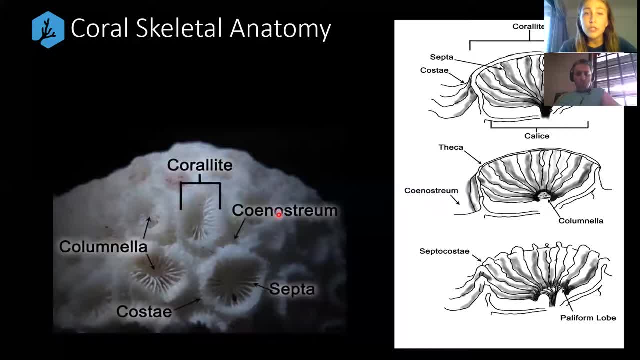 It's where all the important stuff is. We've got the columnella, which you can kind of see- I nearly pointed it with my fingers in instead of my pointer- which is the central part, essentially where the mouth is going to be sitting, of each of our corallites. 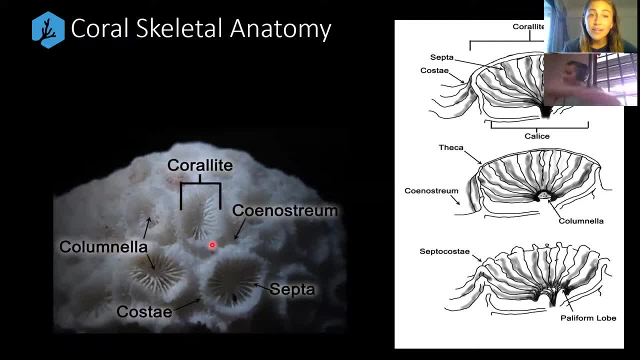 Then we've got the synastrum, So not all corals will have one. What this is a fancy word for is for space in between the corallites, So the synastrum sits in between the corallites, If there are indeed separate walls. 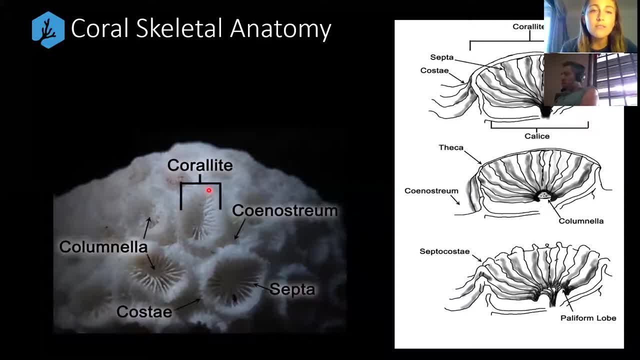 And while walls aren't technically labelled, here you can sort of tell and guess where the wall is going to be on this. This is the edge, This is the wall, And each of these are also walls. here You can think of the scepter as sort of like the ridge-like structures that run from the columnella all the way up to the wall of each corallite. 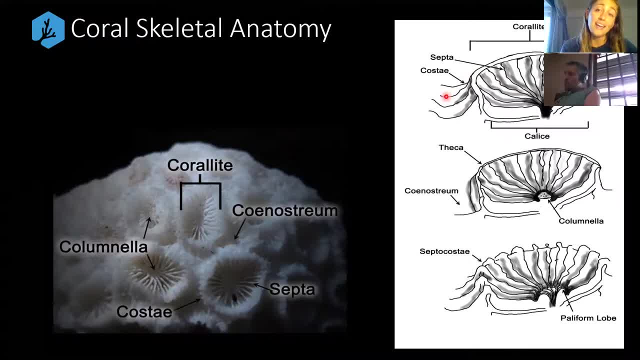 And then the costae are the ridges that run down on the other side. Okay, Occasionally we're going to have corals where the walls are joined, which means we're only going to have scepter and there is no other side. you'd just be dropping down into another polyp. 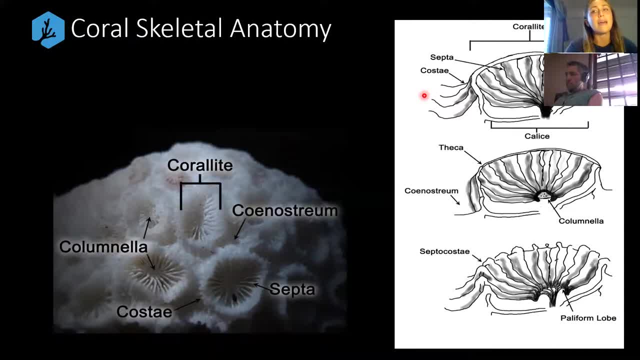 Don't worry if that sounds a little bit confusing, because we're going to be seeing plenty of examples of each of these throughout this lecture. So don't worry too much. At the top, if we have a nice flat rim, it's called the theca. 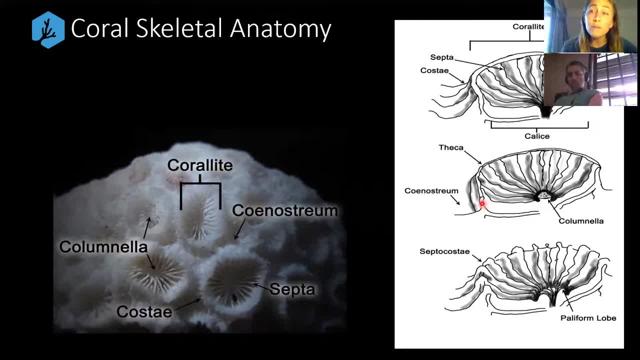 That's kind of, you know, quite a distinct nice wall. Sometimes we don't have that sort of distinct theca, though, And it might just simply be that the scepter run continuously until they die. And it might just simply be that the scepter run continuously until they turn into the costae, in which case they've called it the scepter costae, which is probably like the one time in science where they kept it simple and they just called it what it should obviously be called, which is the joining of the scepter costae. 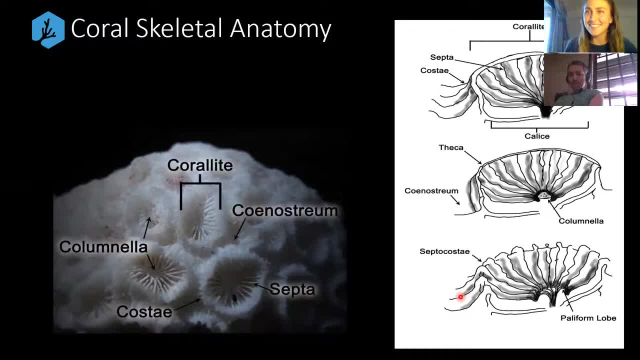 Yeah, so yay, science. That one was an easy naming, I suppose, So then we've also. what have we missed here? Oh yep, Sorry, I forgot to point to the real life photo here. So this is the scepter on the inner part. 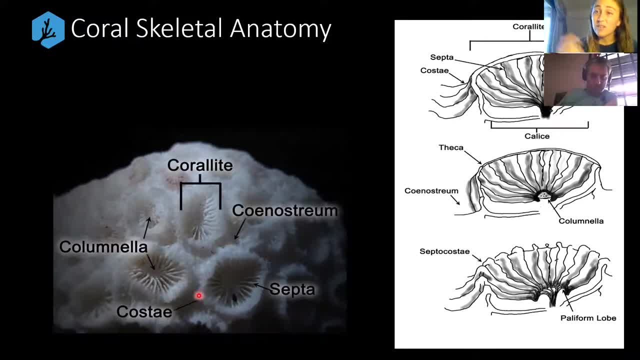 On the outside you can see the scepter. Okay, So this is the scepter. on the inner part You can see the jagged nature here, the outside structure of those walls, Pretty straightforward, relatively speaking. You guys might see down here. there's sort of like in this photo, down the bottom or this diagram I should say sort of looks like a secondary wall or a little sort of like crown that sits just over the edge of the mouth or over the top of the mouth. 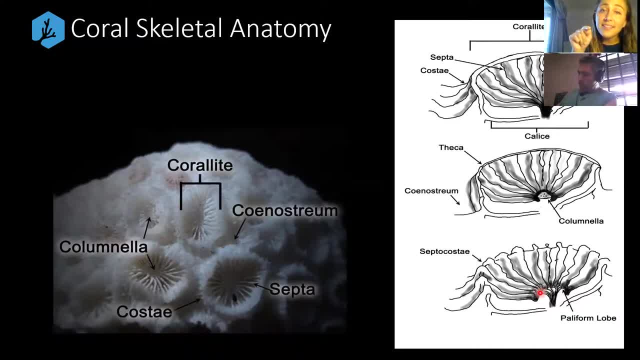 And that's called the paliform lobe. Not all corals have this, but when they do, it's usually pretty important because they look like other corals, And you guys will know what I'm talking about when we get down to some of our Maryland. it's Maryland today. 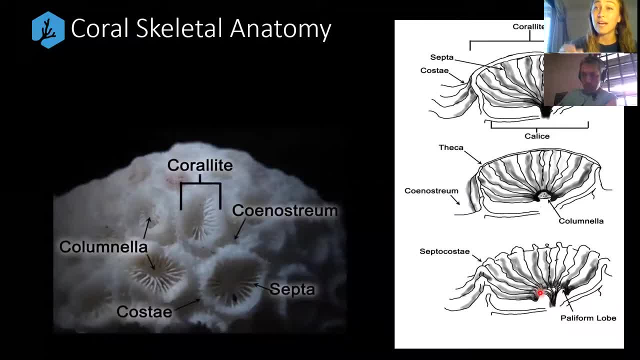 Sometimes the difference might between two corals might be the fact that one has a paliform lobe and one doesn't. But again, all of these terms- don't worry, you don't have to remember all of them, you know right at this moment because I am going to be pointing back to them and referring to them when we're actually looking at corals. 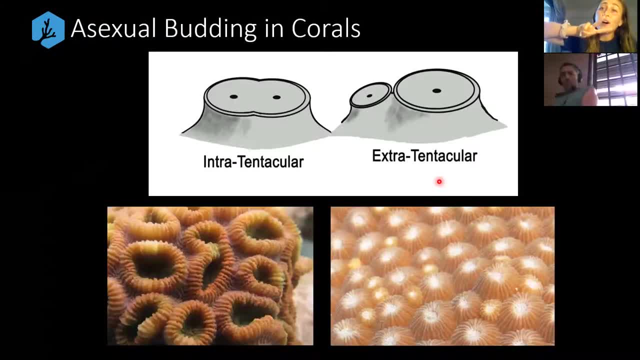 So pretty easy. We have two types of budding in corals. When corals aren't getting their sexy time on during the special spawning times each year, they will be breeding asexually. So every coral colony does start as a single polyp that is produced sexually during spawning seasons, when eggs and sperm are released into their water column. 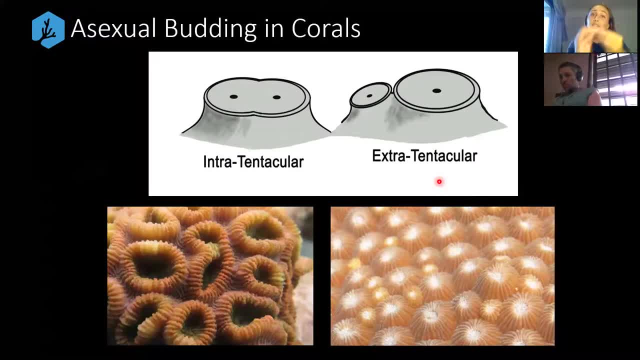 They mix together on the surface because they are buoyant, and eventually they settle down, turn into a single polyp And that's the end of sexual reproduction for probably the next seven to 10 years or so at least. From that point forward they'll sexually- they will asexually- reproduce, but a single polyp will turn into more. 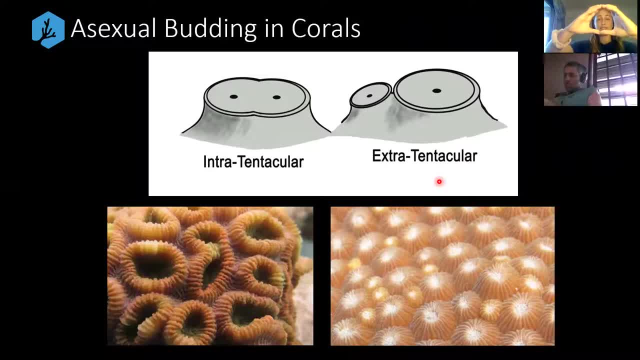 So intratentacular budding is when you pretty much have a single polyp, like you can see on my hands here, and they bud off like this sort of turning into a figure eight and they pop off from one another. Okay, think of intratentacular as internal. internally, you know it's happening from what was already sort of existing there, if that makes sense. 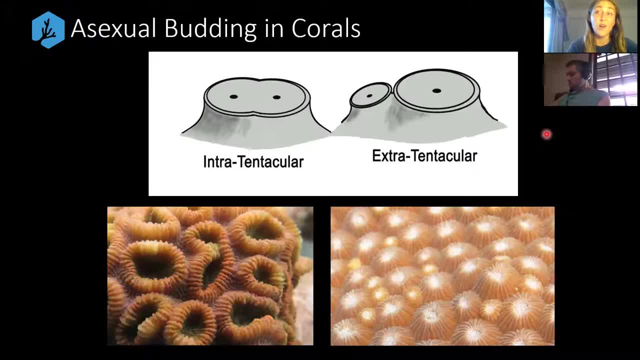 And then we've also got corals, So we've got extratentacular. think of that as external budding off of the polyps that were already there. So they're just sitting their own thing, these baby polyps- You can see them here, these smaller polyps, but just simply sort of pushing themselves up in between these larger ones. 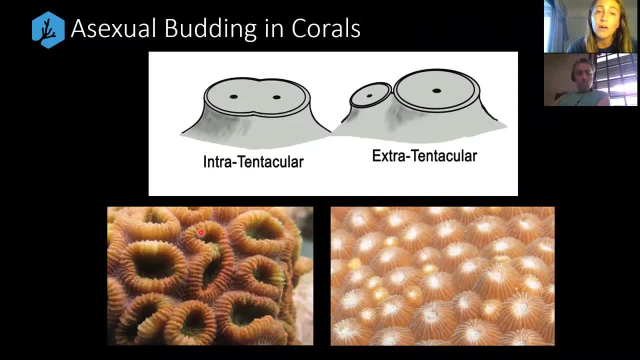 All right, And here you can really see that figure eight shape going on. Again, remembering that, while these are two very different genera- this is a diploastria heliopora and this is a dipsastria- You can sort of still see those structures. 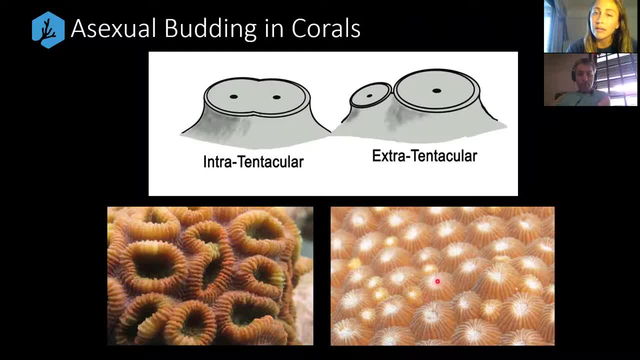 We were talking about before. Here's the whole corallite, the wall, and again here are the corallites. okay, But again intratentacular and extratentacular budding. Sometimes this is very useful to remember because certain corals, of course, have intratentacular budding and some will have extratentacular. 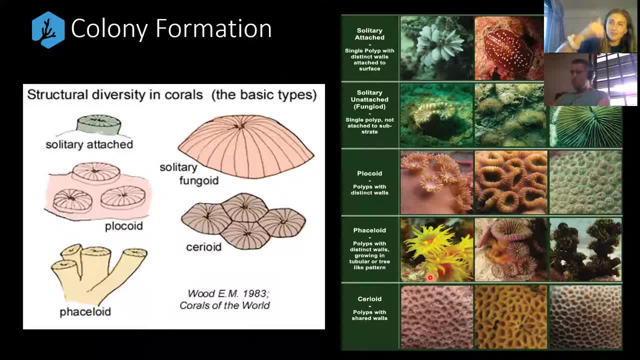 Any questions. so far, Remember that you can do those hand things or like whatever if you guys need to. So just do it if you need to, but otherwise I'm going to keep going. We are going to get, of course, into the taxonomy. 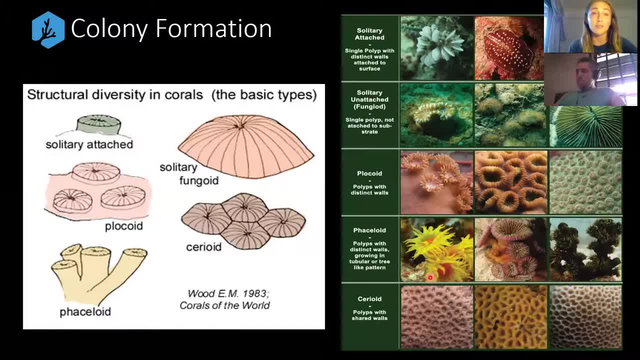 But this is just Some of those essential, like key knowledge points that it's good for you guys to know before we get into it. We'll fly past this bit because we're going to sort of be repeating it during. You can see the real life photos, obviously up to the side here. 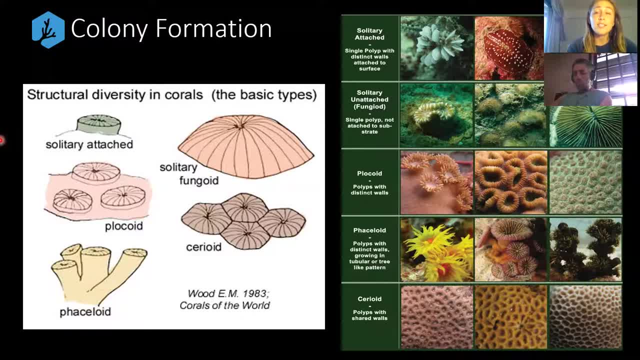 I'll sort of focus on this side here. In terms of colony formation, corals do grow in many different forms, So we do have solitary attached and we have a single polyp, a single individual corallite, and they remain attached and they don't actually bud off. 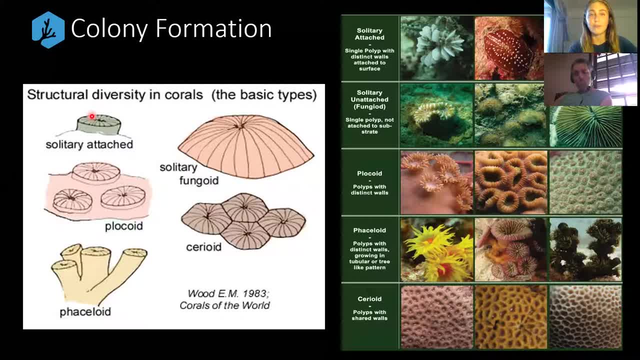 Some corals are not colonial and we'll get a few examples of that throughout this lecture. We have the solitary fungoid, which is again a singular polyp, but they are not attached. So often people refer to these as your mushroom corals, which you guys can see along the side here. 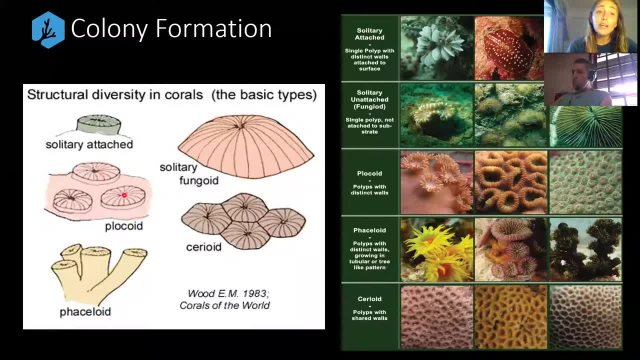 And there's some of my favorites. They're awesome. Then we've got the plocoid. We've got very distinct walls and separate polyps. We've got the gneiss- in this situation, We've got the gneissinastrum. 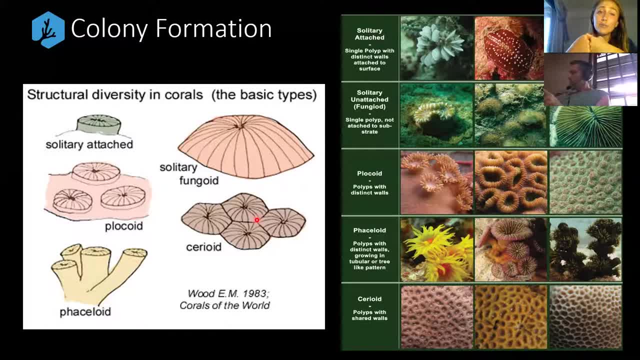 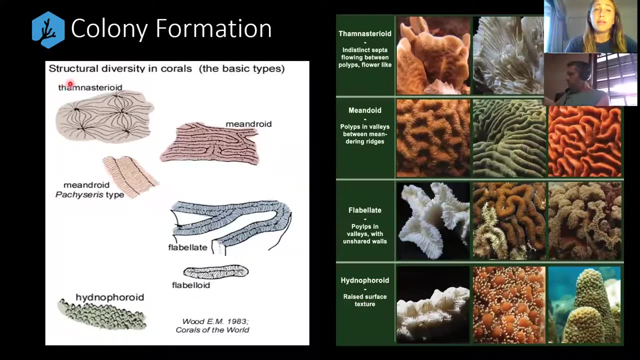 We've got seroid, where they are budding head to head here as well, And then we've got basaloid, where they are quite tubular in nature. You can describe it as two And our equivalents over here. So then we've also got themnasteroid, which is an interesting one. 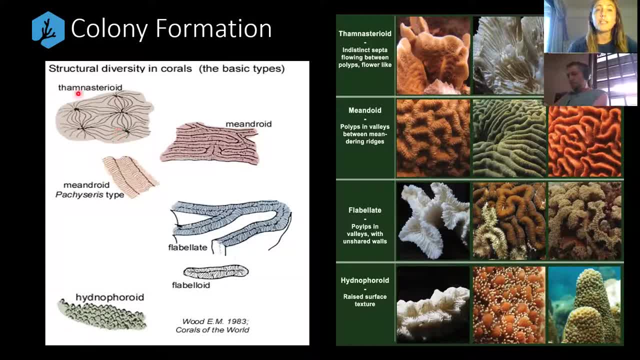 It's ones that have no distinct walls. So this is pretty cool. We're going to be having one of our corals that we're covering today, or a couple of them, such as pavona, which is a viviparous. It's a very, very common coral of the Indo-Pacific which takes this growth form. 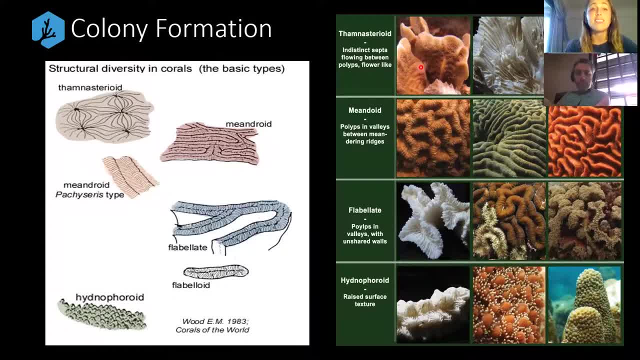 There's actually a photo of it just there. So it is indistinct sceptre flowing between polyps. They're kind of flower-like. There are no costae because there's no wall. that's being met and the costae coming down from the other side there. 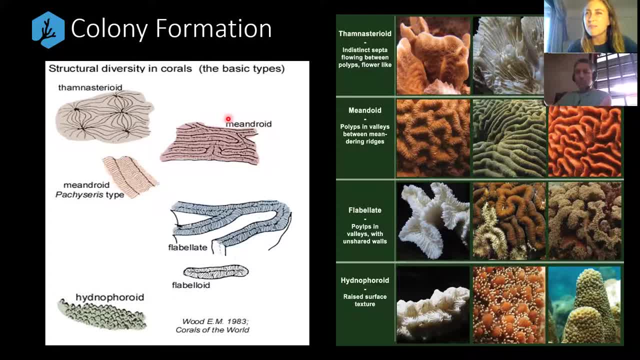 All right. So then we've got meandroid, which is a pretty easy one to remember. Meandroid is meandering, that type of coral. We've got meandroid pachycerius type, which is sort of a very common coral. 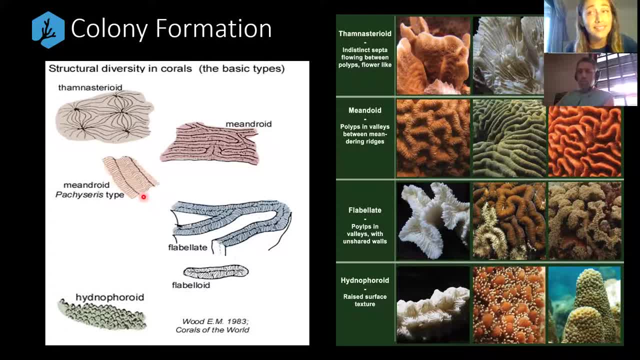 So we've got a lot of meandroid. There is a variation of meandroid. There is a genus called pachycerius. funnily enough, That's just doesn't quite have a colony formation. So this is sort of to describe that genus. 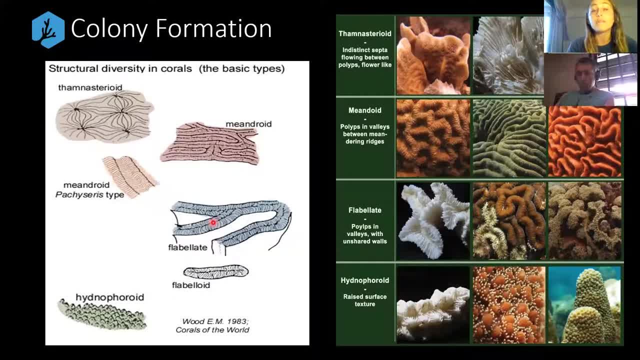 We've also got flabilate, which is practically well. it's meandering in nature. However, we have these sort of gaps in between, And if you ever saw a coral like this, you know sometimes it looks like they're a little bit bit broken. 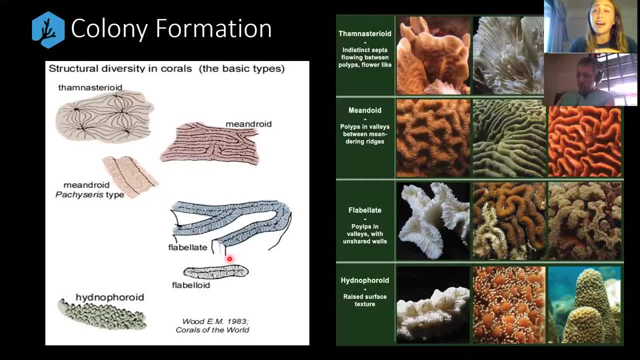 But it's just that they've got these sort of sometimes jigsaw like pieces that kind of half sort of fit together. So it's a very common coral, But you will have sort of gaps in the middle, A flabiloid as well. 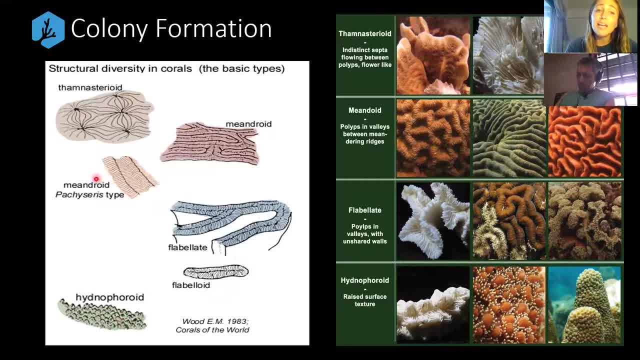 And then we've got hydnophoroid which, similarly to meandroid pachycerius type, describes a single genus of coral called hydnophora, which has these bumps along the skeleton called hydnophores. So there's not a lot of variation in what they call this coral, its bumps and its colony formation in this example there. 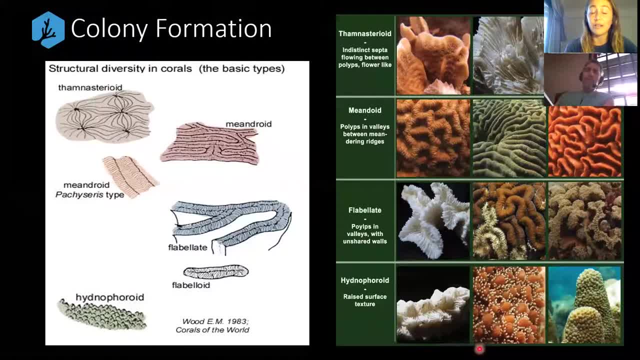 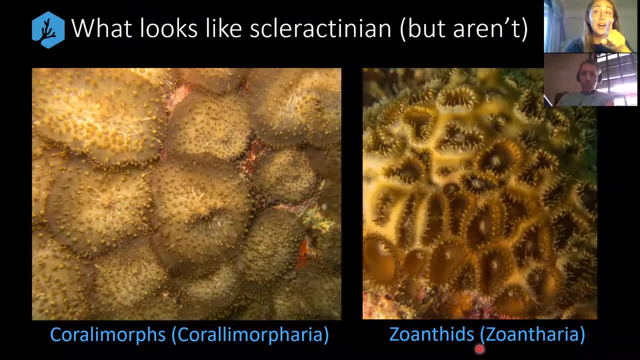 But this is an actual Flabilophidae of the hydnophora. It is a very, very beautiful colony, that's for sure. So what looks like hard coral but isn't hard coral? So when I'm teaching my students, you know, and things are new to them and they might not know what everything is- I always say, you know, try not to be invasive, of course, 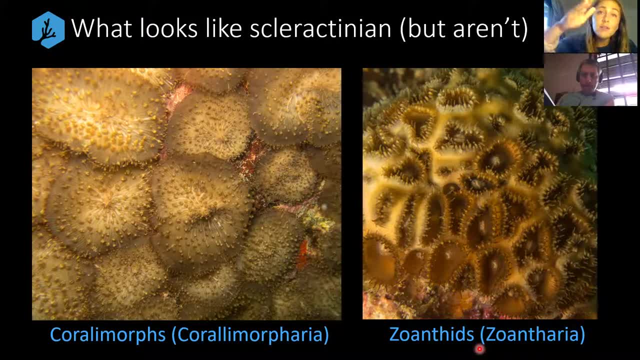 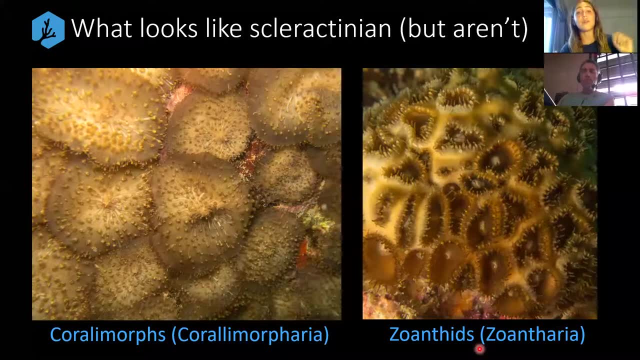 But if you're really unsure about what something is, giving it a little bit of a wave can actually help. so much in helping you come to the conclusion of what that thing is. So when it comes to corallimorphs, they've got these little tentacles here. corals again are cnidarians. they're related to jellyfish. they've got stinging cells called gnatysis and they've got little tentacle-like structures. 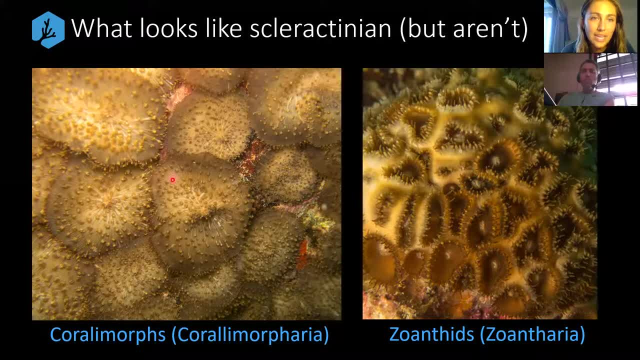 These guys sort of do too. They're a little bit like more short here, but you can see them speckled all around the edges and they've got a central sort of mouth area, So someone who might be a bit newer to this might very well go. ah, is this a hard coral? But if you were to give a little bit of a wave, they only have a single core, So they're not as hard as corals are, So they might be a little bit newer to this might very well go. ah, is this a hard coral? 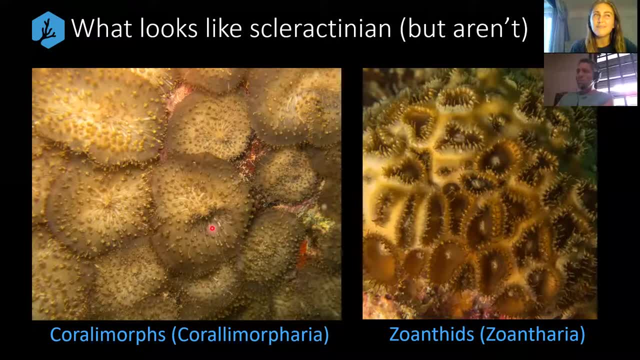 But if you were to give a little bit of a wave, they only have a single core centralized attachment point and the edges of them are quite floppy is probably the easiest way to uh, to describe that there, and then very, very easily you can probably say, oh okay, well, it's. 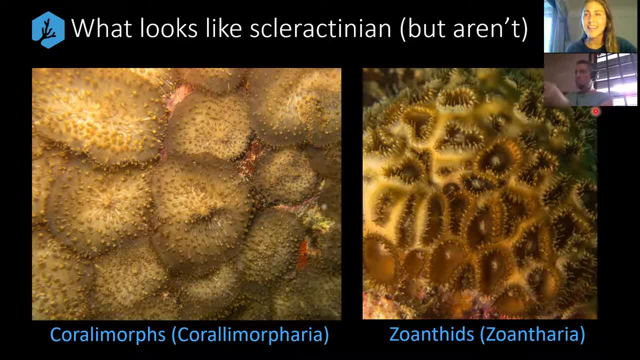 not good a hard skeleton. something about hard corals is that they have a skeleton. they're hard so they can at least let help you work out what it's, what it's not, you know. in this case, you can say: even if i don't know at this stage what a corallomorph is, i can tell that it's not a hard. 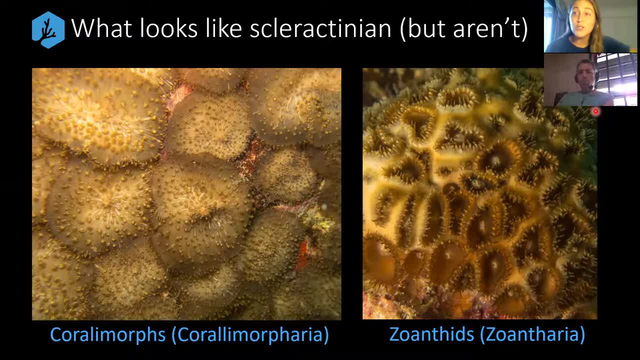 coral, okay, um, and then we've also got zoanthids. these guys in particular look like a few different genera of hard coral, um, they're encrusting, they are often colonial, um, and they look like some of the genera, such as dipsastria and montastria, some of the corals we're going to cover today. 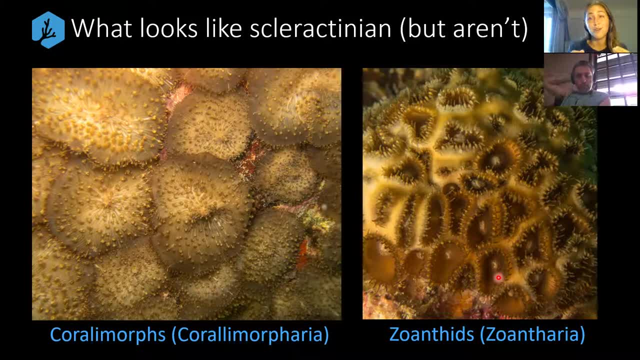 that again the name of the game. if you're unsure, give things a little bit of a wave and see how they respond. and in the case of of zoanthids, firstly, morphologically they're different because they have a double layer of tentacles compared to one, which is what hard corals have, if you want to get up real close and 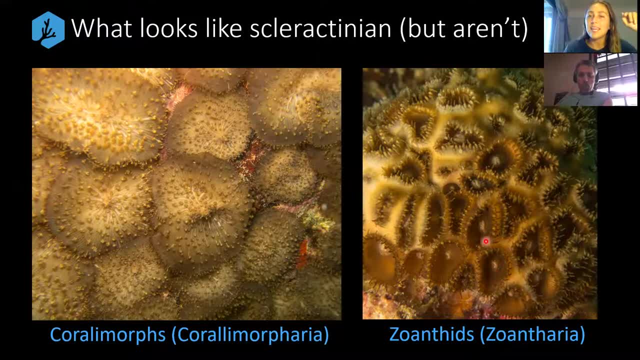 check it out, you can see that. but secondly, what happens to like these entire, like polypy shapes here is that they think: oh, you know, is that food coming? you know what is that water action? so they'll, they'll close up, whether it be that they're trying to catch food or they're trying. 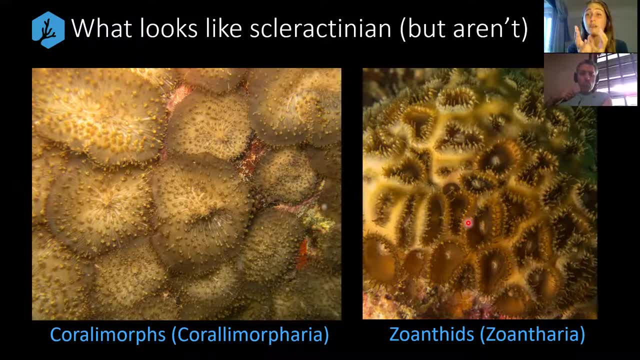 to protect themselves. but you can pretty much see the softness of them when they do that, and they do often close up entirely into, like you know, all these neat little pockets. um, so, even if, again, you don't know what a zoanthid is, you can go. hmm, you know, i don't think that's a hard coral, at least. 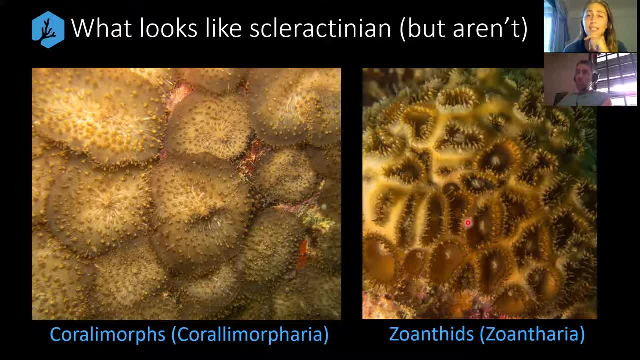 also guys i would just like to mention- so i didn't mention this at the start. why are we focusing on the taxonomy of hard corals versus soft corals or versus corallimorphs or zoanthids? none of these other organisms are not important, but one of the things that they have or that they don't have- that. 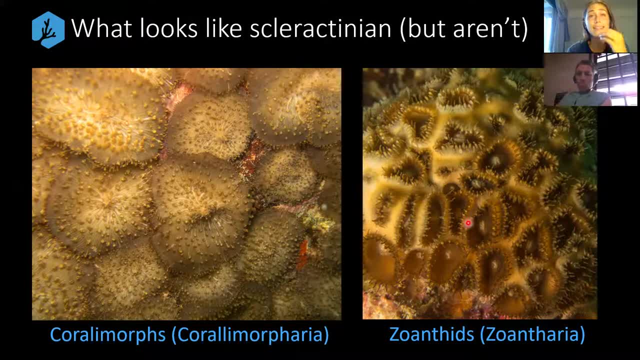 hard corals have is a calcium carbonate skeleton. and when we're talking about, you know, tropical reef ecosystems in particular, what these ecosystems are really reliant on is having hard substrate, because marine animals- you know they don't shoot roots and secure themselves into the sand like with land plants and things like this. they are encrusting animals generally. 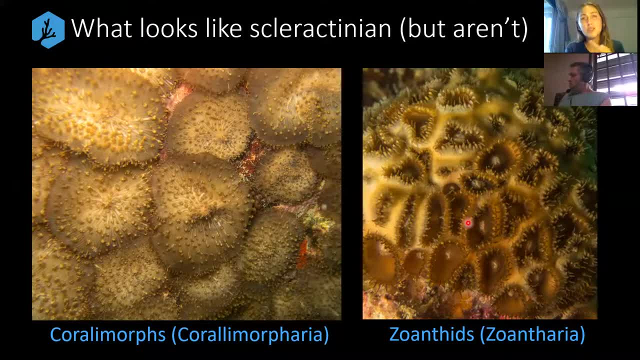 at least when we are talking about our cell animals here. you know, like your soft corals, anemones and things like this, they need to have something hard to sit on. so if we have a sandy area and you know coral spawning is, just a cold occurred and all the gametes are looking for a 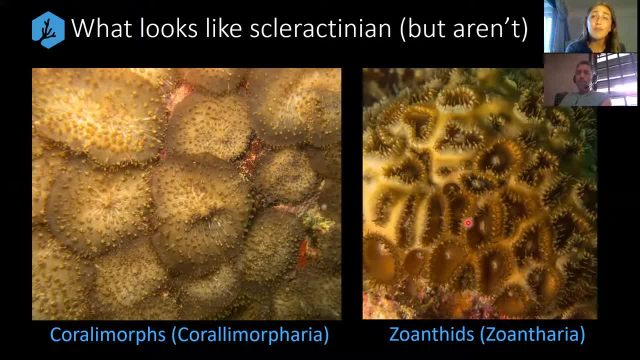 place, or all the fertilized gametes are looking for a place to settle. they won't probably be able to settle on the sand because it's nothing, it's not secure. they're not going to be able to set up a centralized polyp and then um asexually reproduce there, because it's just too mobile. 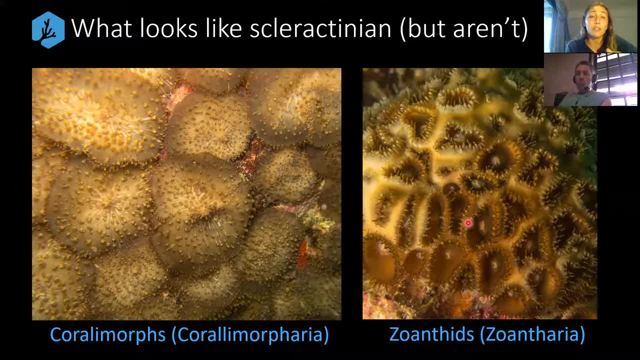 they need something really solid and while hard- you know we've got a lot of people who are- you know, hard corals produce, a hard thing being that it is their skeleton. so hard corals play all these roles in terms of providing habitat and food source and so on, when they're alive, but when 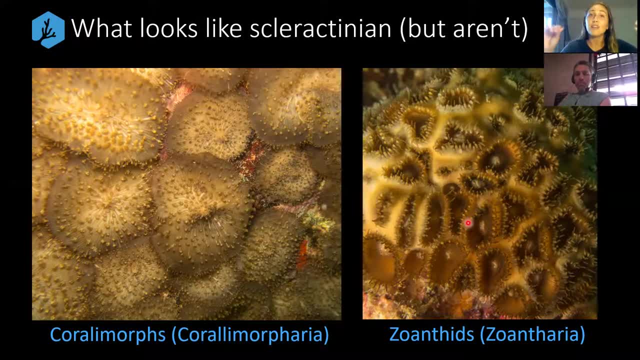 they're dead. they're also really important because, even though that you know, the living tissue on the outside, all the living polyps will die, the hard stuff being the skeleton, remains behind. so maybe that means another coral will settle there and grow into a brand new colony, or zoanthid will. 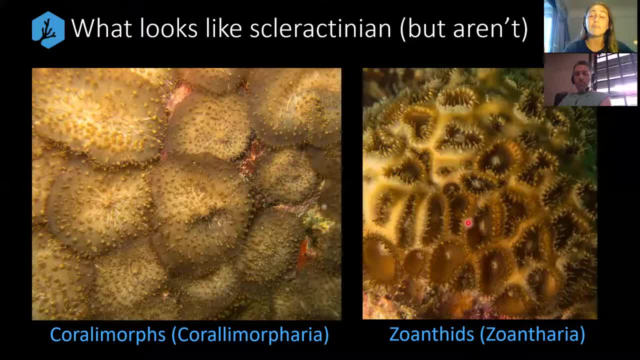 settle there, or a soft coral will settle there and all these things play these really essential ecosystem roles and that's why we do focus on getting extra information in a hard coral. so us at conservation diver, when we do our ecological monitoring program surveys, we collect at least 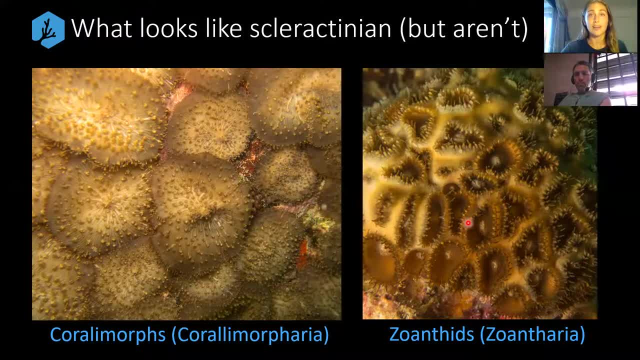 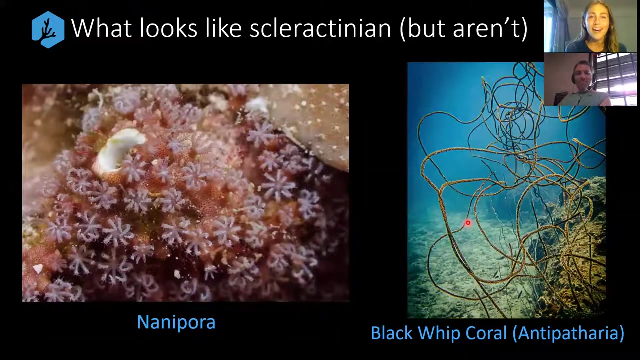 genus level on every coral along our transect lines, so that we can see diversity and if there are diversity shifts throughout time. so i hope that compromised a little bit more clarification, uh, for why we're doing this, because i should have done that on the first slide, but you know, you know it's been a while for me. next nanny pora. so i just said that. 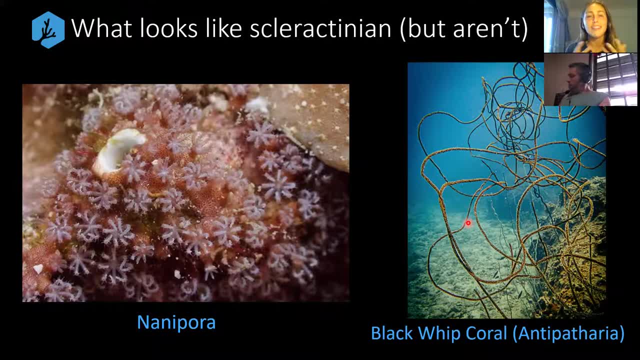 only hard corals produce skeletons. well, i didn't say only, but i said hard corals produce skeletons. there are some very specific examples of soft octocorelia which do it too. so nanny pora is a really cool one, and we at conservation diver we do a lot of research on how soft octocorelia 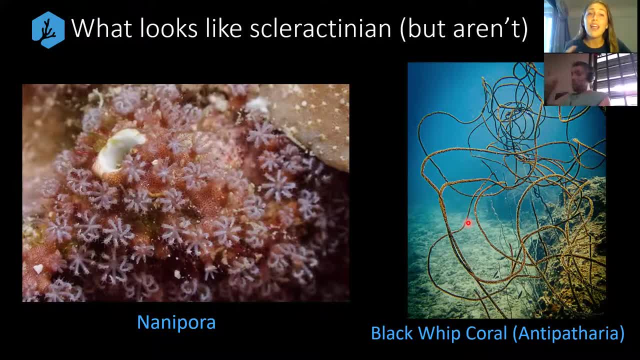 works in the vaults. we do some research on how soft octocorelia works in the vaults and we do some research from the conservation diver- who's the guy in the photo? and i do a lot of research on that. but- and i was a 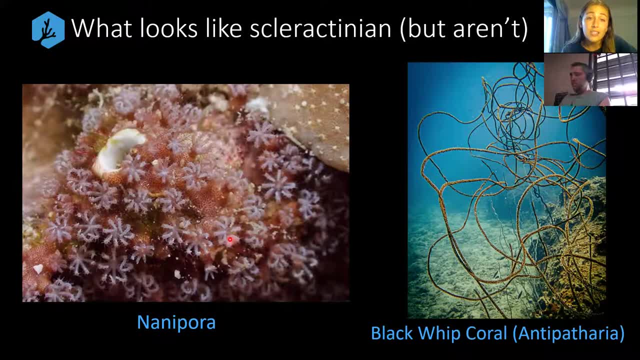 thin skeleton, but we can tell that it's an octochoral here because it's got one, two, three, four, five, six, seven, eight tentacles, hard corals guys, scleric tinea, whether we're looking at big polyp of tentacles or something very small that you've got to get up close to check out. 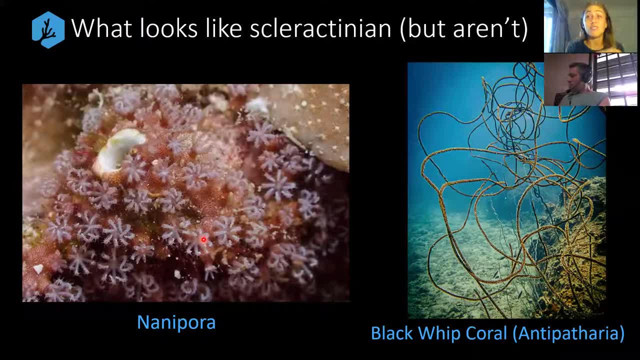 they always have tentacles in multiples of six. so whether it's six tentacles, 12 tentacles or 24, it's always going to be in multiples of six, like unless a predator has come along and taken a bite out of one of them or something like that. but the standard is that it'll be multiples of six. 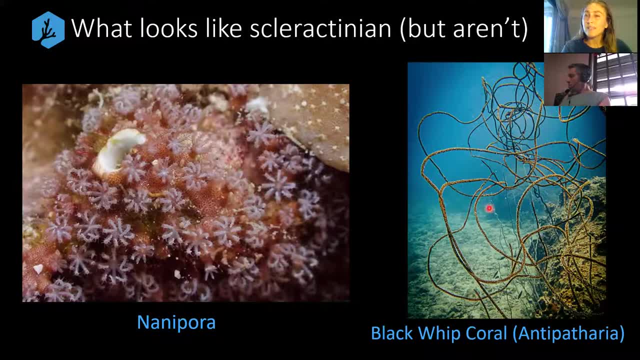 all right. so then we've got our black whip corals. i think these are not too, you know, they're not too easily mixed up with as hard corals, so we can kind of skip past that one. but if you guys hadn't seen photos of these whip corals, this is what they look like, and they generally live in slightly deeper. 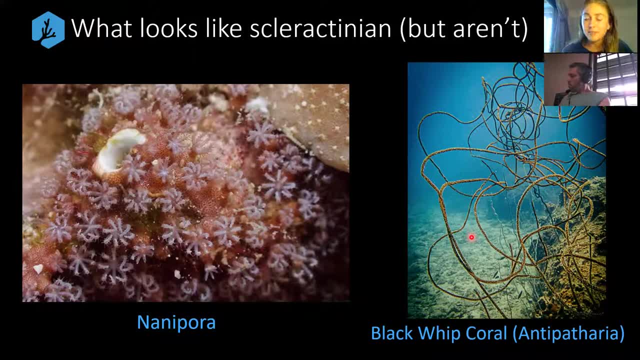 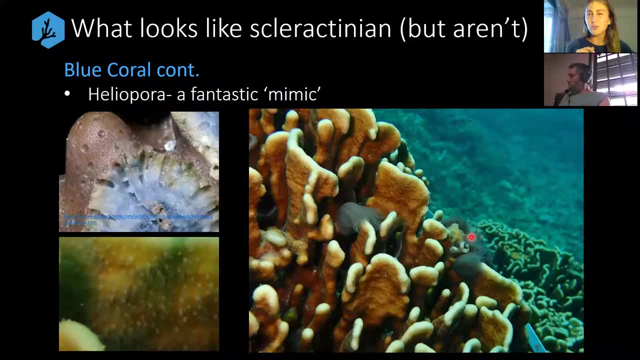 areas, maybe ranging. you know you're 10, 15 minutes plus anyway. now let's look at the one soft coral that actually is very, very cool. sorry, they're all cool, but the one that's really cool and being the exception, um, you know, in terms of producing a calcium carbonate skeleton. so heliopora is a genus of soft coral that make huge. 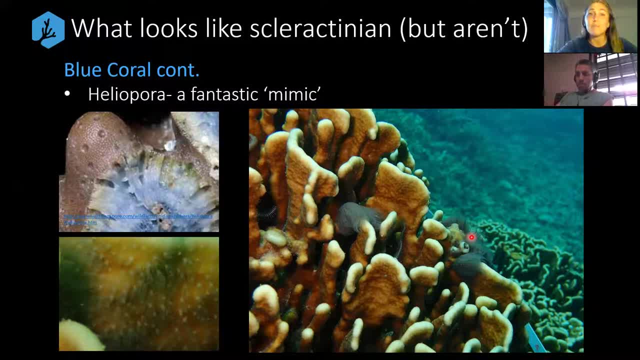 columnar sort of structures. okay, um, it's been really an interesting genus. heliopora was monospecific. until you know, a very cool lady by the name of zoe richards, who's based in australia, described a couple more species to the genus um, which is very exciting for coral lovers in general. 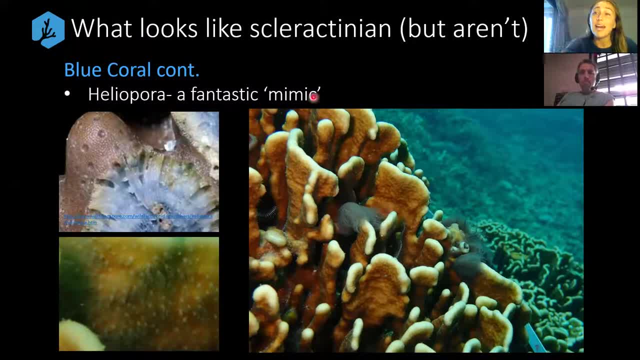 but for any of you guys that may have been to our site in indonesia, maybe you visited leon, which opened up in 2019. leon saw zoe richards paper and thought, huh, you know, i always thought there was something wrong with all the heliopora we have around ghillie air here in indonesia. 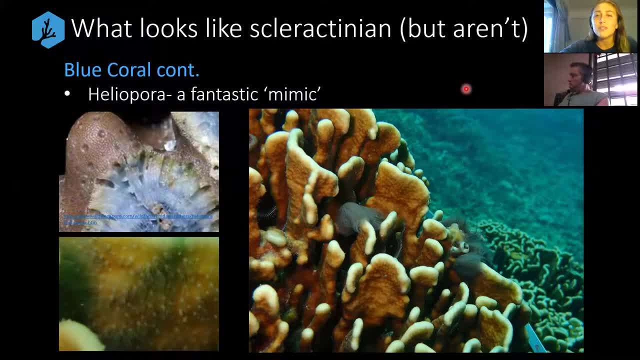 and he took some photos and sent them to zoe. and then he took some samples and sent them to her and he found out that the dominant reef builder around the island he was living on was a species that hadn't been described to science at all up until like the year before- i think it was 2018. 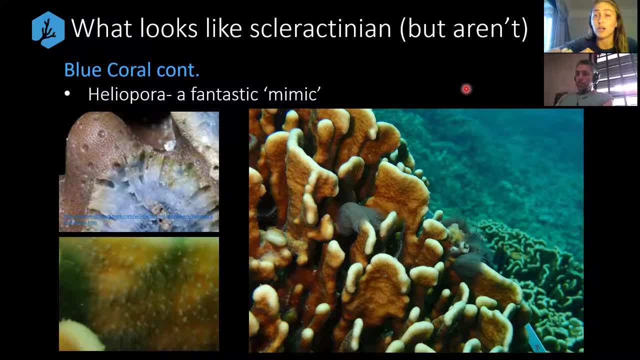 that these new species of heliopora were described. so he and zoe have actually published that now. he also found it in the moldies on previous work that he'd been doing there. but it's pretty exciting, so we are going to go over the rules now. it's pretty relaxing. i think it's a pretty exciting. 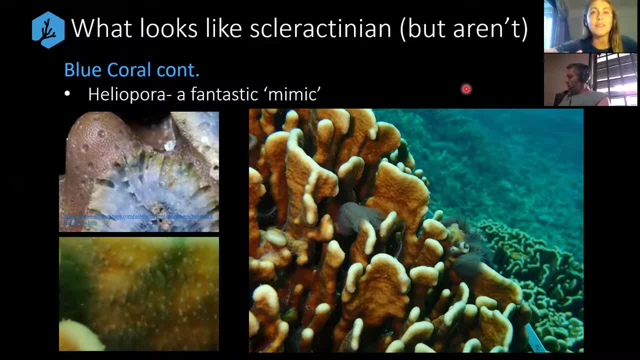 story. we're going to go over what's been going on in the past year or so, but obviously it is a very big exception to the rule. you know, hard corals are hard, soft corals are soft, except for sometimes because science and nature don't like to play by the rules. they make their own rules and while it's 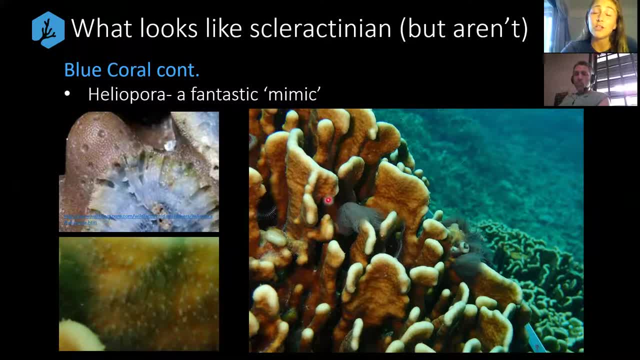 really annoying to us. it's better to just try and appreciate it rather than get frustrated by it. i I've never seen any other coral with such a sort of fuzzy nature to it. okay, So you can see, especially in this box, here the tentacles are out. 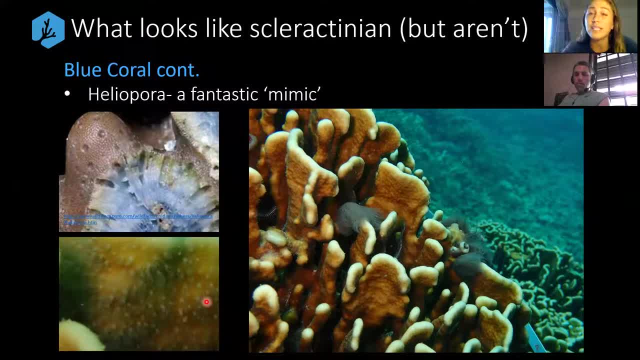 and they're so sort of thin and fine and fuzzy that I probably wouldn't be able to tell in the field if it's eight tentacles or a multiple of six. but it does have this very, very fuzzy nature to it, and small polyps too. 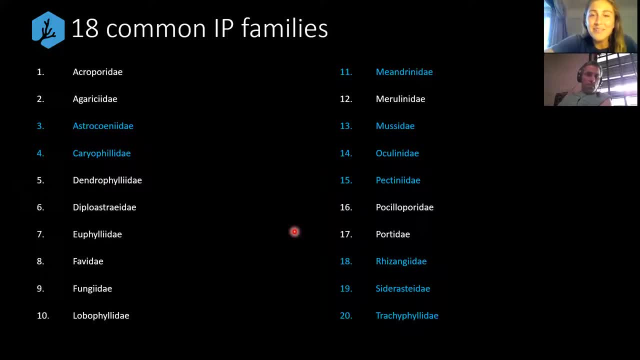 Excellent, So hard corals. Sorry, I've already been yapping onto you guys for a while, but now I finally get into some of the more common Indo-Pacific families. We're going to be covering the families that are white, okay. 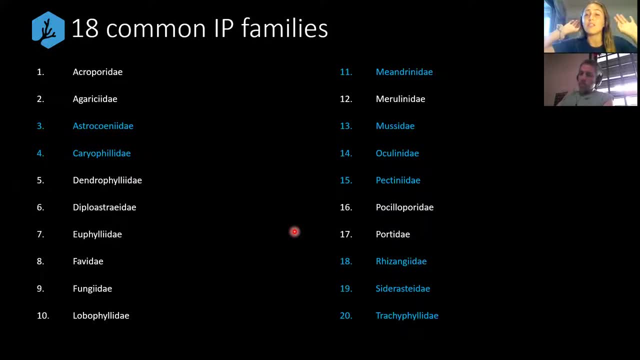 There are more, of course. If you guys want more information of any of these others, you can feel free to message. But pretty much in this lecture we could go on forever- well, not forever, but we could go on for over 300 species worth of corals. 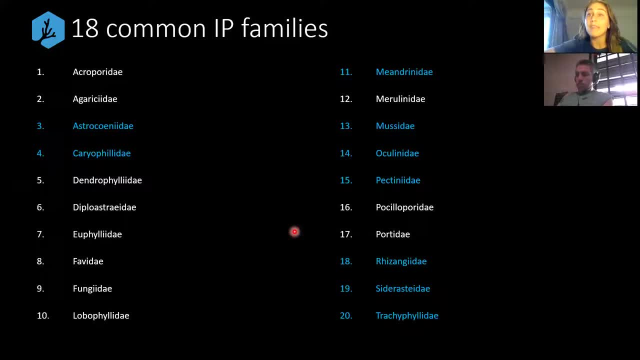 because that's how many in the Indo-Pacific, Within the Caribbean sort of Atlantic regions- closer to 70. So most of the diversity exists within the Indo-Pacific, But I can't keep you guys here all day, slash all night, So we're going to focus on what our team has pretty much noticed. 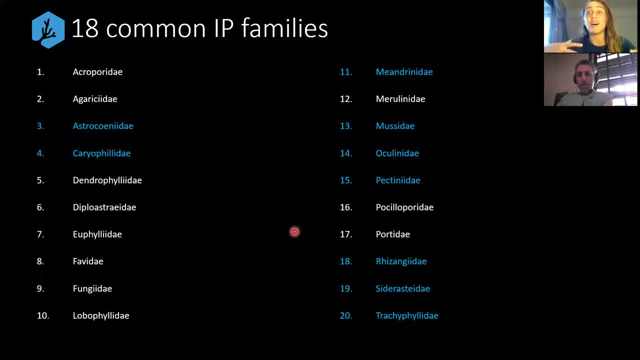 over the years as sort of the more dominant, really kind of useful ones to know, especially if you are wanting to monitor and implement conservation practices in your local area or if you plan to be doing this kind of work in future. So let's start with Acroboraidae. 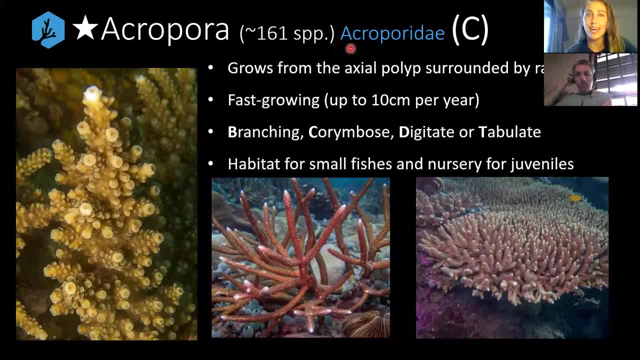 So all of our families are going to be blue. okay, If I have plastered a star next to it. what that means is that I think this should be high priority on your list to learn. okay, This: you know the genera that we're going to be covering today. 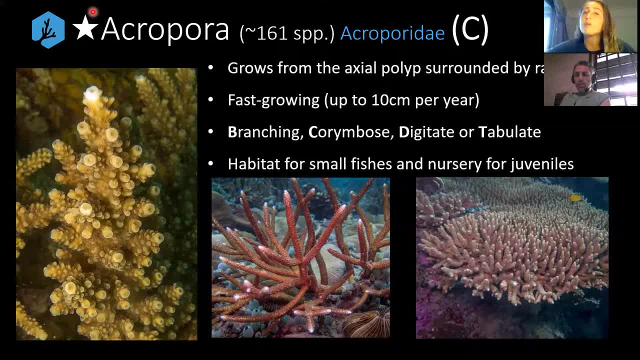 that have a star next to the name I've noticed are frequenting the literature so much. So if you really do want to get into the sciences of coral taxonomy and so on, I'd say this is you know. these ones are particularly useful. 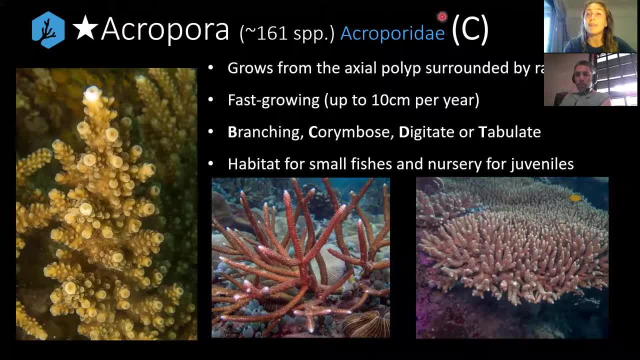 to have a good understanding on What it means if I've got a star next to it and I've got a plastered a sea next to it, is that this genus also occurs in the Caribbean, Just for you guys, because obviously we do have people. 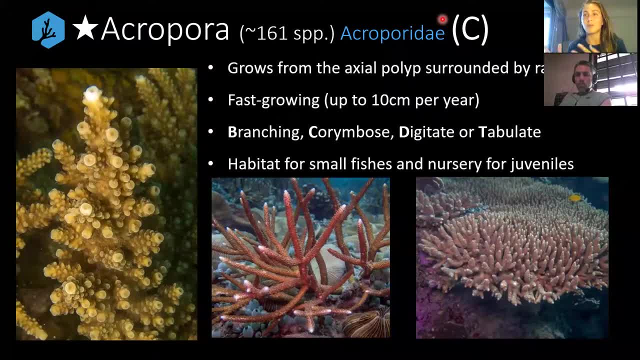 from all around the world. Sure, the Indo-Pacific has more diversity. It doesn't mean that we're all going to live and work in the Indo-Pacific, okay, So that's just what those codes mean. just so we're all aware. 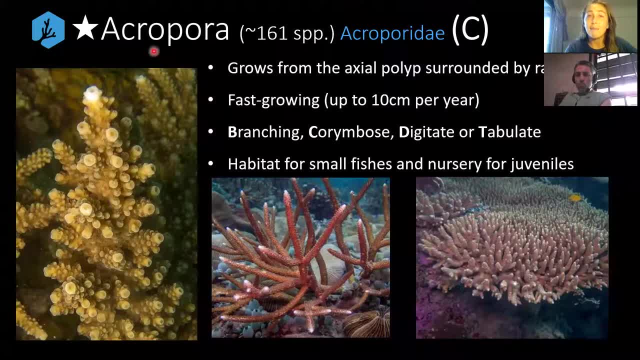 Acroboraidae is the family name, Acrobora is our genus name and it's got a lot of species. okay, We're going to cover the species names in the Caribbean in a moment, because there's only three In the Indo-Pacific. 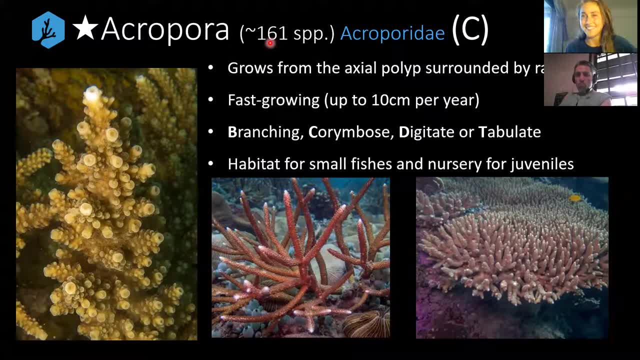 knowing that there's a lot is good, for now at least, okay. So how do we identify Acropora? Main identifying characteristic is that it has what we call axial polyps at the tip of each branch, and they are surrounded by smaller radial polyps. 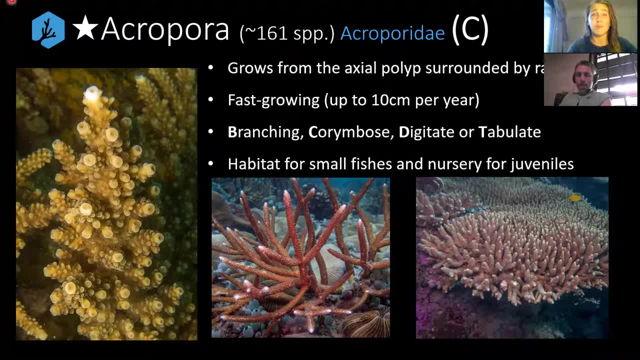 Radial meaning surrounding. So, quite literally, radial polyps are the ones that kind of surround the tips of each branches you know, such as here. So just so you guys can see, this is an axial polyp here, So is each of these. 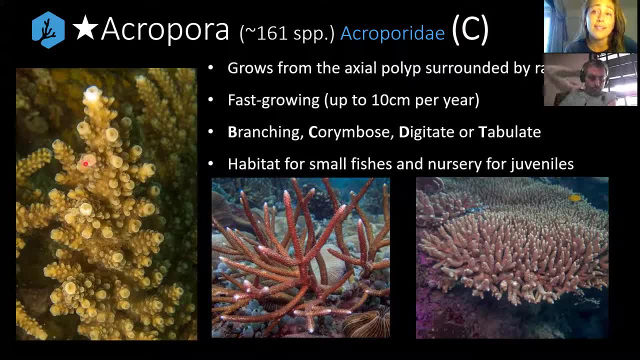 as we can go down the branch. This is a Corumbo's Acroporaidae, okay, So that means that it's quite a dense branching coral. This is what we'd call just a standard branching coral, And you can still see that quite obviously. 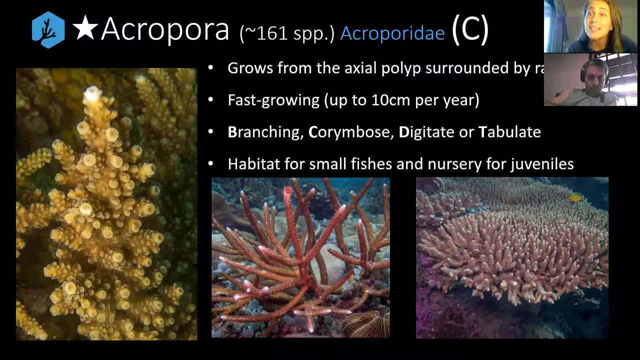 you've got the tip of each one, which has got this rather distinct and large axial polyp surrounded by all these smaller bump, nubbin-looking. and then you've got the tip of each one and they're their radial polyps. okay, 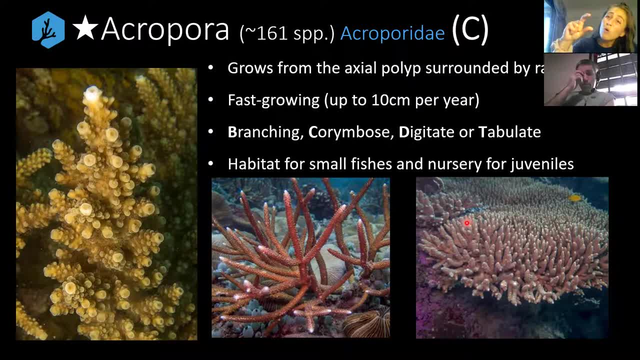 We also have them growing as digitate, where you get these small vertical upward-facing branches over and over again, and your large table corals. I think everyone knows what we mean when I say table coral And those are sort of the main growth forms. 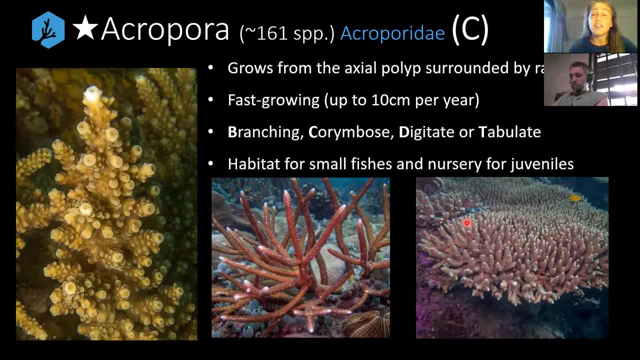 which Acropora grow into okay. They are ecologically very important. They provide a lot of habitat for small fishes and nurseries for juvenile, and they're also very important for recovering quite quickly after events of stress such as a storm or a cyclone. 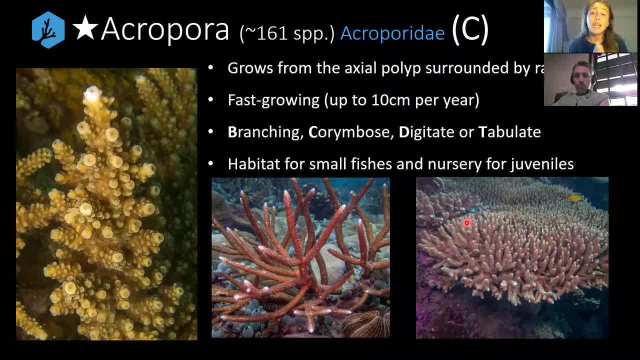 or a bleaching event or something like this. However, even though they're fast-growing- and they can grow up to 10 centimetres per year, they are also more susceptible to threats, unfortunately, And this is because, well, they're investing a lot of time into growing quite quickly. 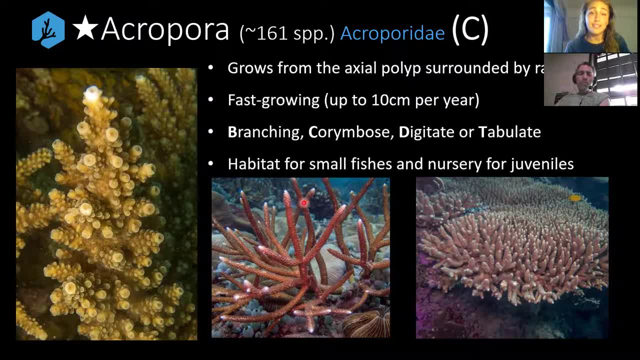 They also, as you can see, don't have the densest of skeletons. okay, So some of our larger, more bouldering corals. they are a lot slower to grow but they are taking a lot more time spending energy. 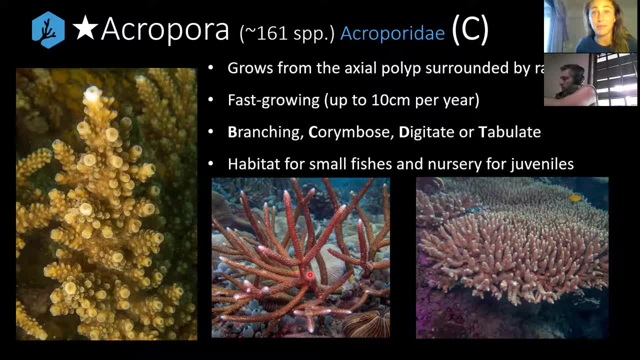 putting the energy into creating calcium carbonate and extracting the components they need out of the water column in order to do that. So they're playing these very different roles, But these guys are really important for providing structurally complex habitat, because nursery grounds are very, very important. 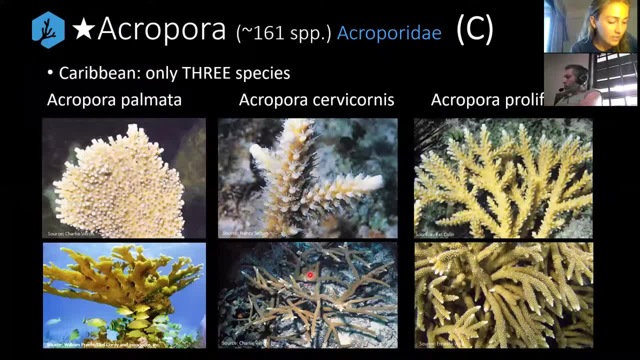 in the marine world. I'm just going to see if this was someone. okay, beautiful Imogen. I'm going to send you the taxonomy exam after this. Got your message, So let's very quickly cover the acroporas that exist in Caribbean waters. 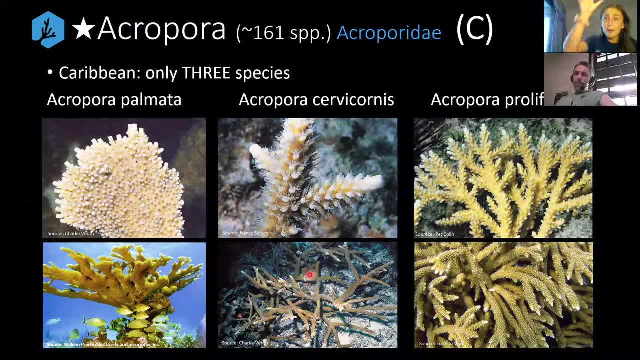 Now, I don't know, give me a thumbs up or a hands up or something. if you've heard of just the state of corals in the Caribbean, Can anyone has anyone, does anyone know? Sort of a little bit, maybe, maybe. 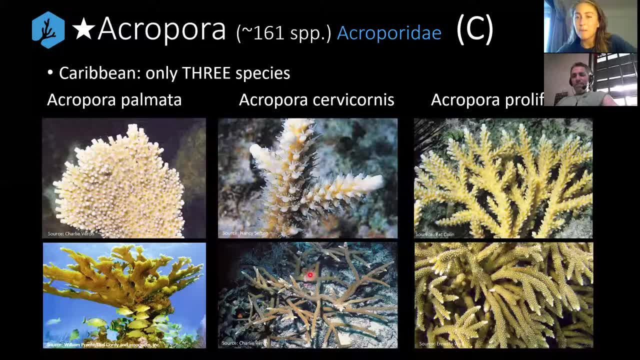 Hmm, Brad. yes, Okay, There's a couple of us. So the Caribbean is very famous because unfortunately, it has a lot of coral diseases. This region has been hammered by coral diseases and other stresses to their corals for the last couple of decades. 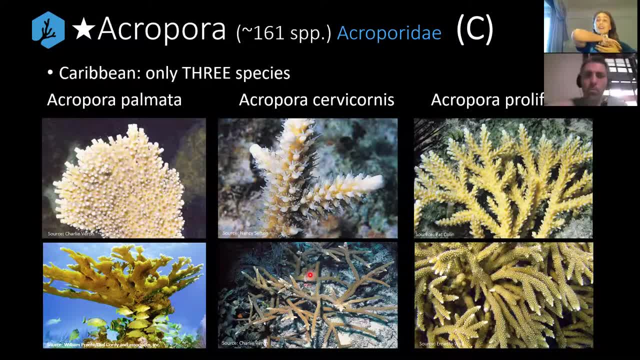 It used to be incredibly famous for its vast like seascapes of acroporid corals And then, unfortunately, it was hit by a coral disease called white-tailed corals, And that's a very common disease. So it was a very common disease. 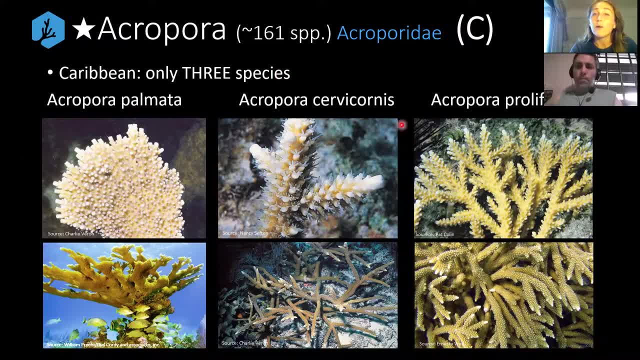 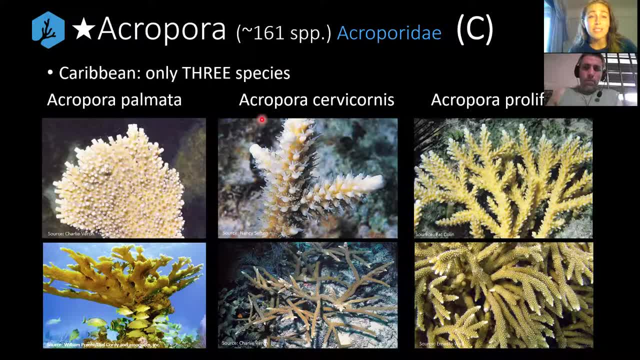 And they pretty much wiped through the populations And in some places brought down the coral coverage by 99%, So they essentially nearly lost everything. So there's a lot of restoration projects and research et cetera being done. 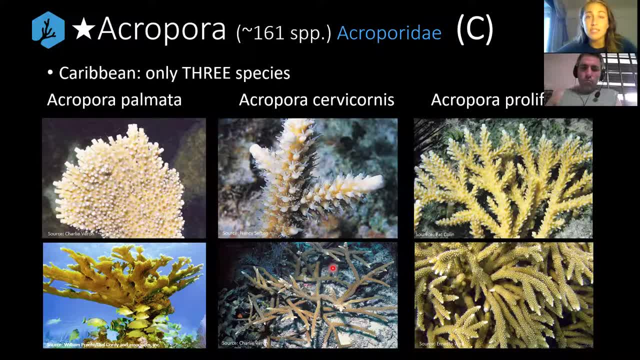 especially on these corals right here, And if you guys are interested in the literature and look it up in your own time, you'll see Acropora cervicornis, Acropora palmata, in particular, being mentioned a lot. So these are kind of very important species. 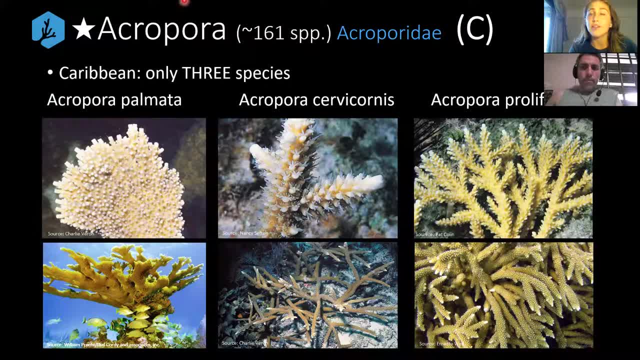 So, yeah, there are only three species out of the over 160 Acroporas that exist globally, Again mostly in the Indo-Pacific. This is the one that a lot of people refer to as the staghorn, So when people say staghorn coral, 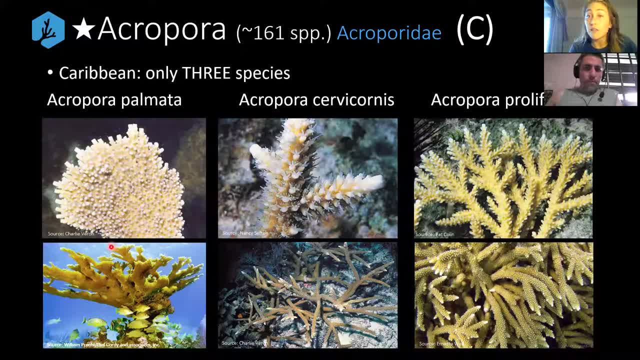 this is the growth form that they're sort of referring to. I don't think I've never seen, I don't think we have this sort of growth form quite in that degree in the Indo-Pacific. okay Again, guys. so you guys probably noticed. 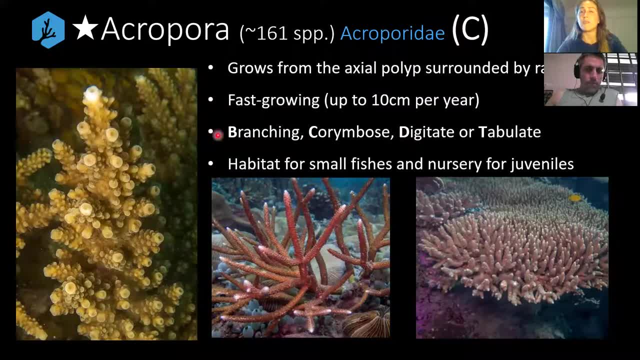 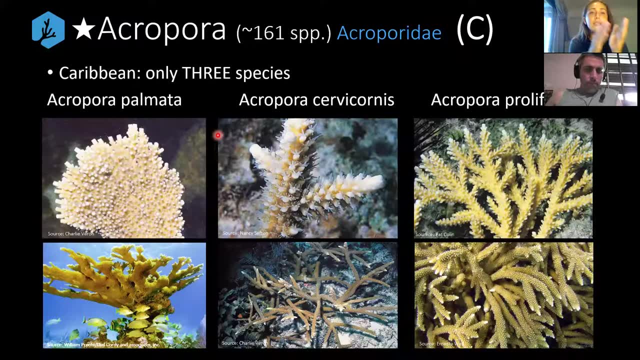 that I just mentioned the fact that these are different growth forms. This is what they grow, as, When it comes to coral genera, it's quite variable. Each coral species grows a particular way, So a coral species will be branching, or it'll be plating, or it'll be bouldering- okay. 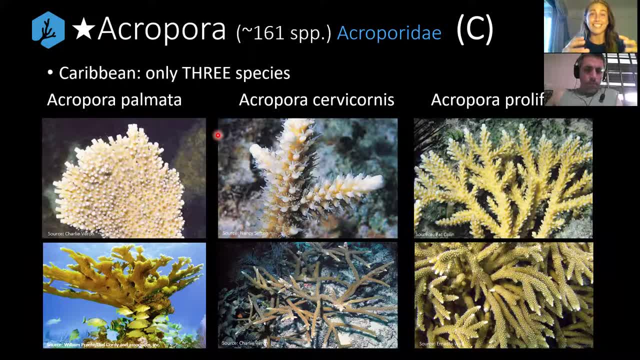 For the genus level, because we're obviously looking at particular genera and they might they have a variety of species. I'm just giving you the ones that they generally grow as quite frequently, But do just keep that in mind, that a particular species 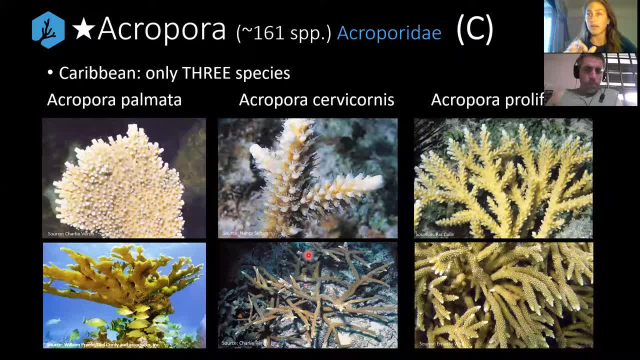 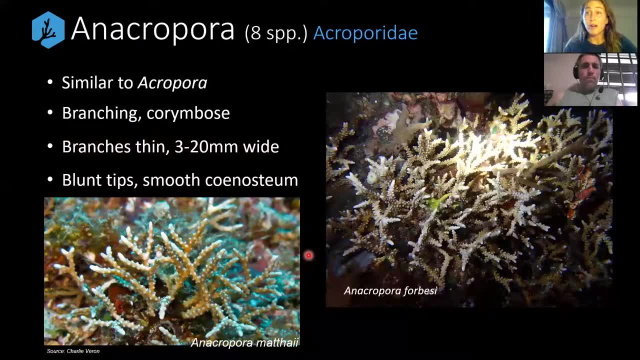 you know, Acropora cervicornis grows branching, And that's the way it grows and that's that Just sort of a good thing to keep in mind. Okay, then we've got an Acropora, which for me, I never had a mnemonic device. 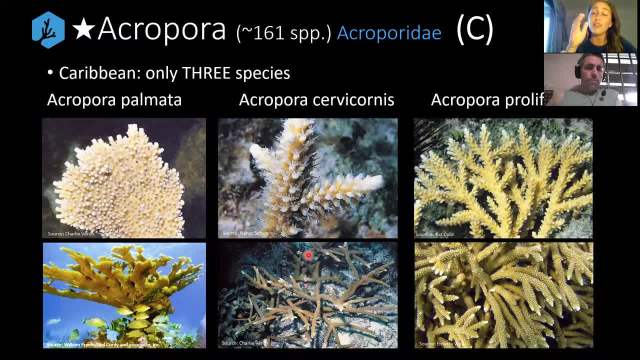 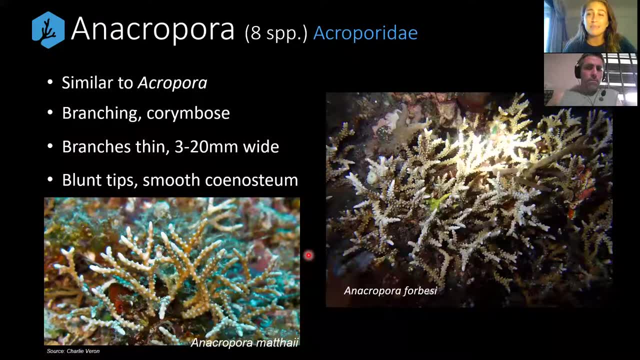 or a way to remember Acropora. It was just mentioned so frequently and drilled into our heads and was all over the scientifically literature that I just ended up remembering it. The way I remembered an Acropora was that like it's like the very skinny. you know bristle version of Acropora. They are in the same family. They do have these sort of nearly like rounded down axial polyps. They're not technically quite axial polyps And I just remember it as like anorexic Acropora. 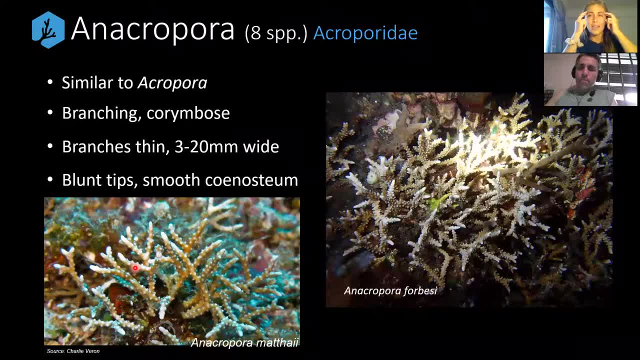 which, again, don't take these names seriously, but just by like word association. it's a pretty easy way to remember this coral genus. Okay, So these ones grow as branching or current bows. They are very, very brittle, offering similar roles. 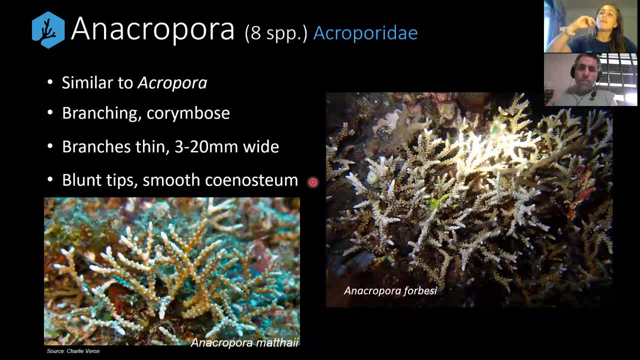 They do make nice little nursery grounds for things to hide in, but again particularly susceptible to say storm surge, waves, cyclones and so on forth. The branches are very thin, three to 20 millimetres wide, So three millimetres sometimes. 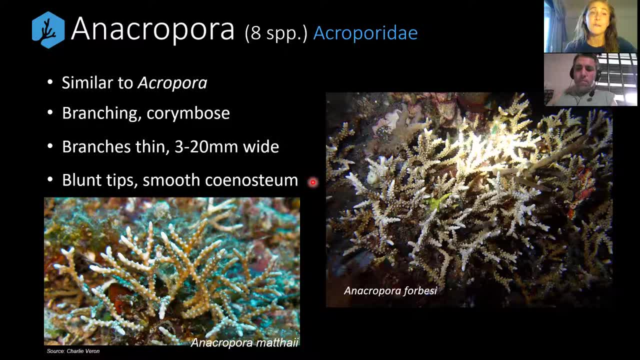 is the entire thickness of the branch, So very small colonies. They've got blunt tips and very smooth synostrum, So remember that just signifies the space in between the polyps, And especially on this photo here you can tell that it's very smooth in the middle there. 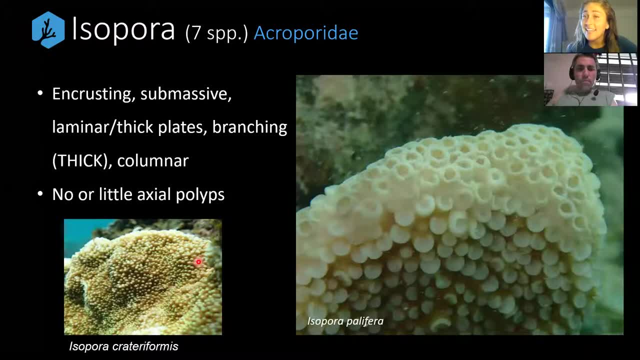 Cool. So then we've got Isopora, Again, an Acroporaidae. The way I remember this is that it does have, technically, some axial polyps, but they're, like, barely visible or, in some species, are just not there. 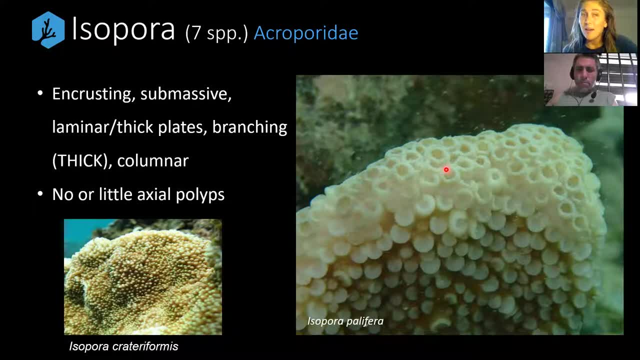 So if you can think of Isopora being an Acropora- but it's axial polyps- had to go into isolation and go away, So it doesn't have those obvious tip ones you know, at the top of each more hill here. 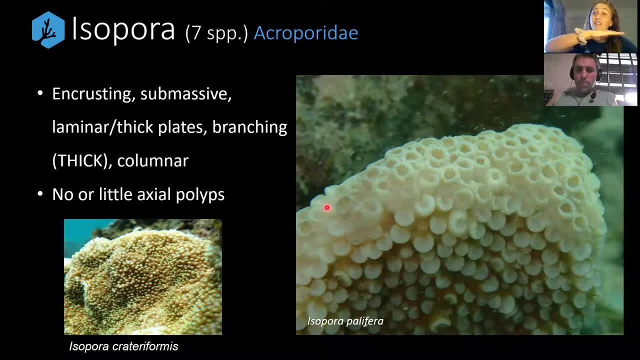 These guys generally grow as in crusting, which is literally just when they're covering a surface. They grow in the submassive, which is quite a lumpy sort of growth form that can get quite large: Our lamina, which is sort of like our plating coral. 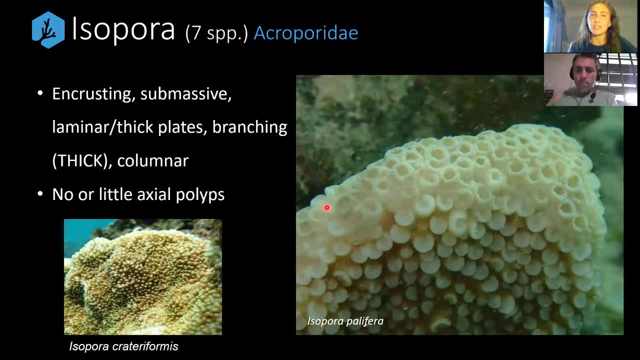 rather thick plates too, or very thick branches, All right. Well, someone's getting back into the room. There we go Right again. Awesome. So again, very little or no axial polyps. Okay, But the polyps are very similar to other Acroporaidae. 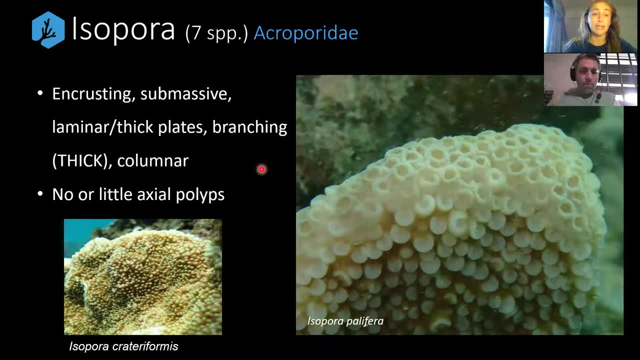 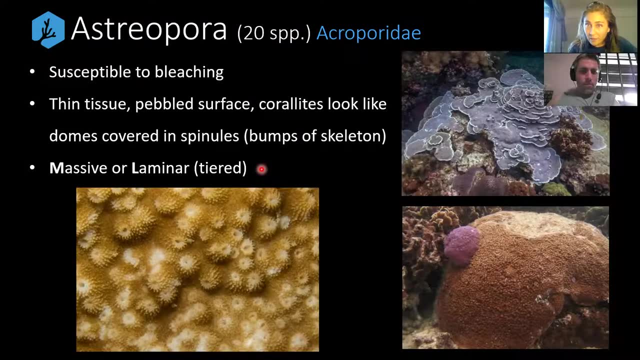 And by that I do mean our Acroporaidae, So just keep that one in mind there. Then we've got Astropora. Okay, Still Acroporaidae. Astropora is such a weird coral because it grows. 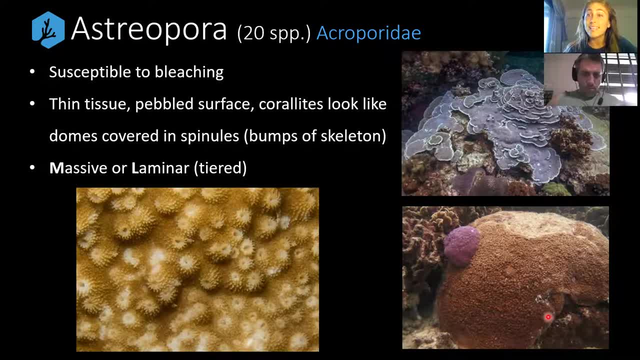 in very large, massive growth forms, as we can see on the bottom right there, And usually what we with. the general rule is: when you get these sort of large, massive growth forms, they're usually pretty resilient to things such as bleaching. 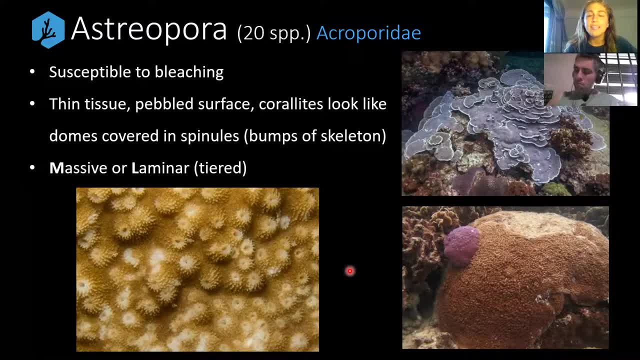 for example, Whereas for some reason Astropora- it seems to be the first one to get stressed out in bleaching. I know from my days in the field when we saw a little bit of bleaching on Astropora we thought oh, hadn't noticed it yet. 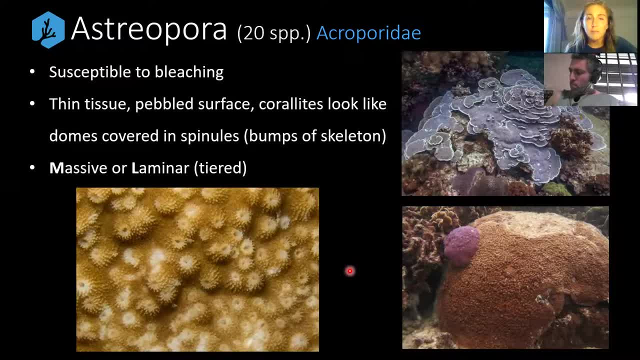 but the temperature seems to be rising And, you know, maybe a few weeks or a month later some of the other corals might be bleaching too. Again, if we're having a heat year And somehow it'd usually be the last to recover as well, 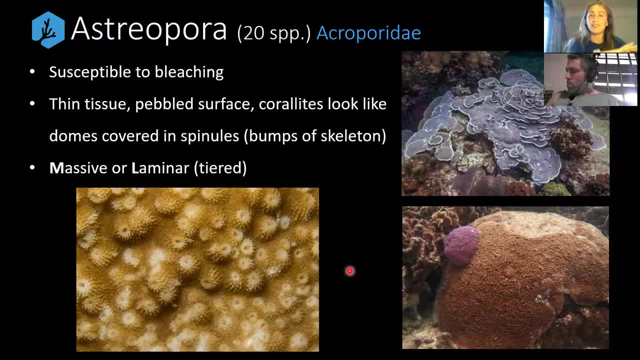 But clearly this coral has, you know, got better susceptibility to like sustaining itself in times of stress, Cause you know they often did recover, but they would just take longer and sort of be the first to express those first signs as well. So a very interesting genus. 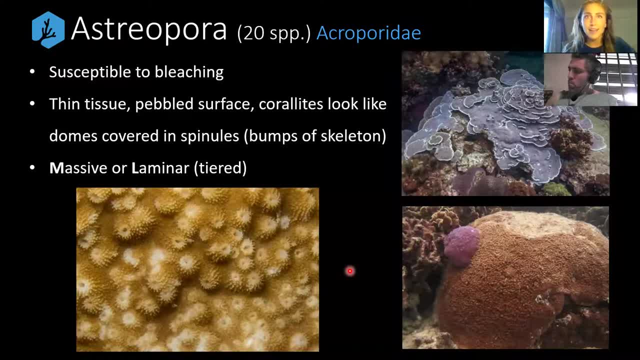 It's sort of not usually the general rule, but again, Astropora is a very interesting genus And science. nature does its own things And there are exceptions to every rule. The top very thin tissue And it's a very pebbled surface. 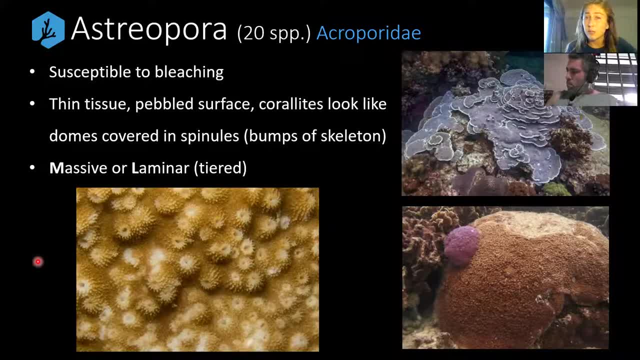 Coralites look like the little domes covered in spinules. Spinules is a fancy name for saying bumps of skeleton, And we're going to see throughout this lecture that there are a few scientific ways to say bumps in skeletons, But spinules is the one we use to describe Astropora. 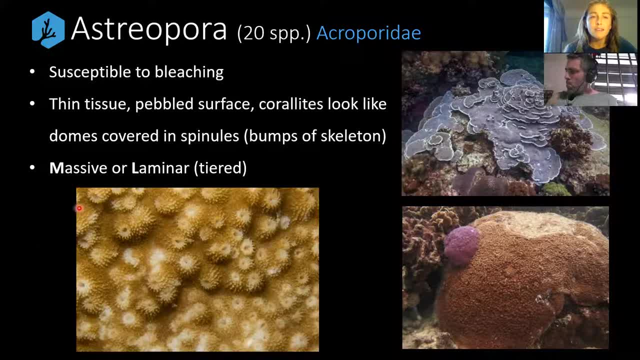 But it's bumpy. I think that this coral looks like- and I hope you guys see what I mean here. It looks like someone took a bucket of googly eyes, stuck their hands in it and sprinkled it over the floor And they've just landed all over the place. 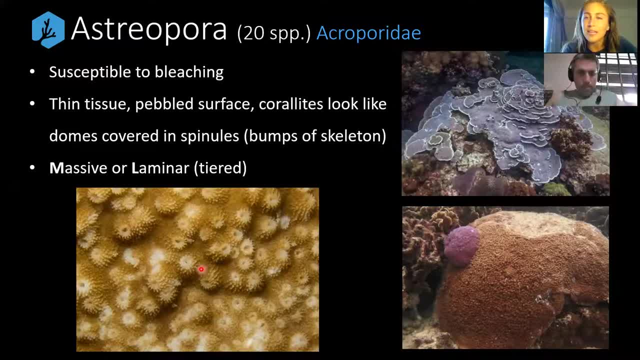 They're kind of facing all different ways And all the little googly eye bits are facing different ways too. Okay, I think the easiest way to remember this and again, these demonic devices are sometimes a bit of a stretch, but just you know humor me. 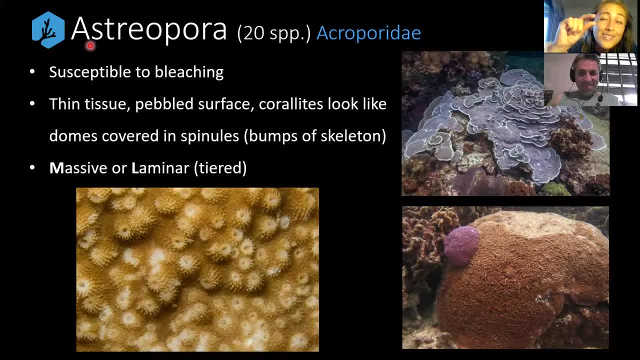 Astropora, I feel like looks like little asteroids, Astroids- hit this coral colony and cause these crevices, these big bumps in the central parts of the coralites, Because, look at this, they're so dug out in the middle. 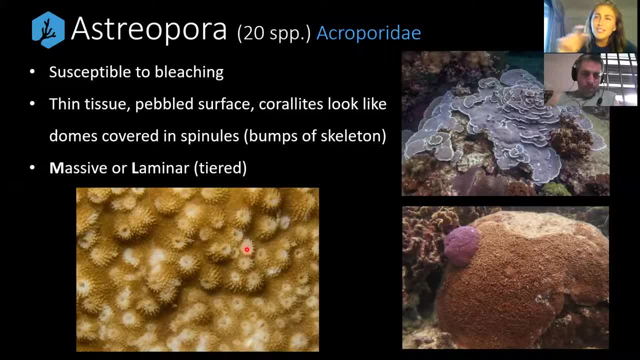 And that's very typical of Astropora. Astropora, asteroids hit it. You guys are probably thinking: thank you, Elle. Now I remember this coral so easily. Wonderful, You're welcome, guys, Anyway. So this one goes all right. 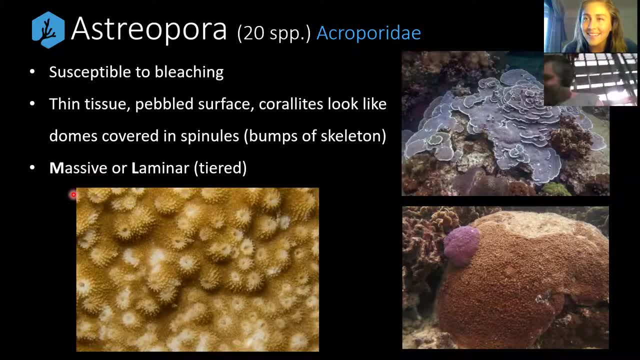 I'm getting thumbs up from Trevor, Thank you, Thank you. The rest of you? I can't see So in my head you're smiling and going. ah, yes, That was wonderful, Thank you. Thank you, No worries. 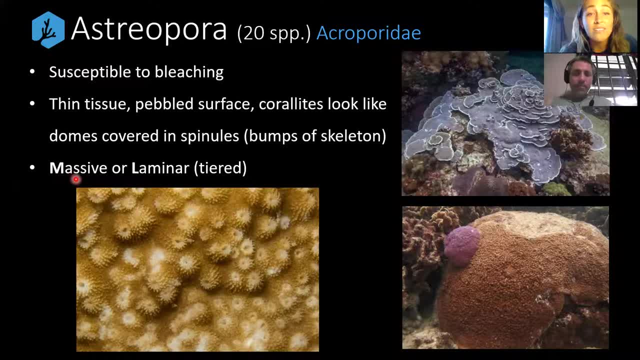 Anyways. So these guys grow as massive or lamina and tiered. So that's sort of what we're talking about here, These sorts of like different levels of little shelving. nearly is what it looks like here. All right, Wonderful. 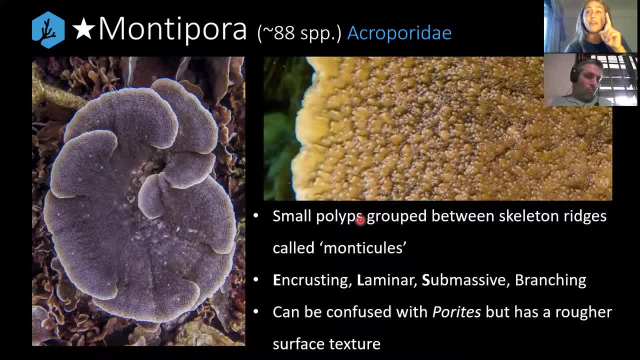 So then we've also got Montipora- Not everyone that. we've got the little star next to it right here, OK, So what that means is that I think this is of particular importance And I think you should put at the top of your priority list. 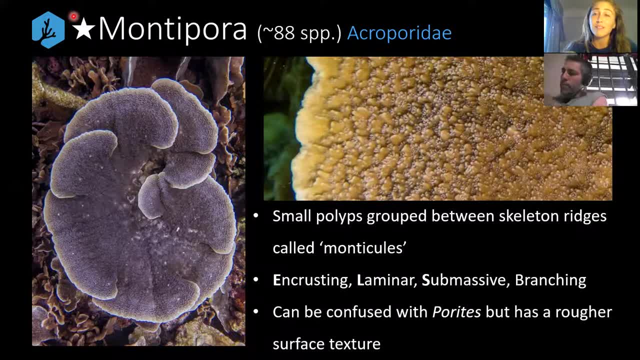 for remembering this coral genera out of you know. I mean remember all of them if you can, by all means, But this was one that's quite relevant to the Indo-Pacific and also mentioned in a lot of scientific literature, So it's a good one to remember. 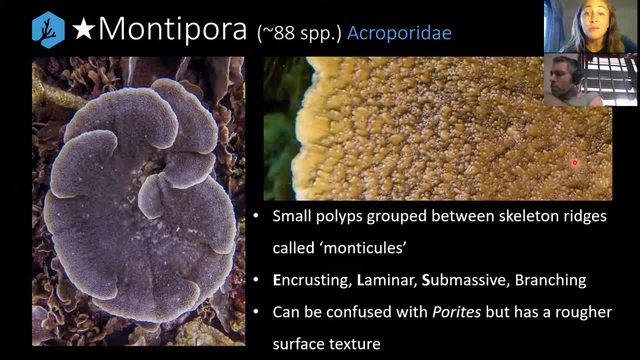 They have very small polyps. They grip together between skeletal bumps. They're called monticules. So here is a bump, name number two being, yeah, monticules, Montipora, monticules. These guys grow as encrusting lamina submassive. 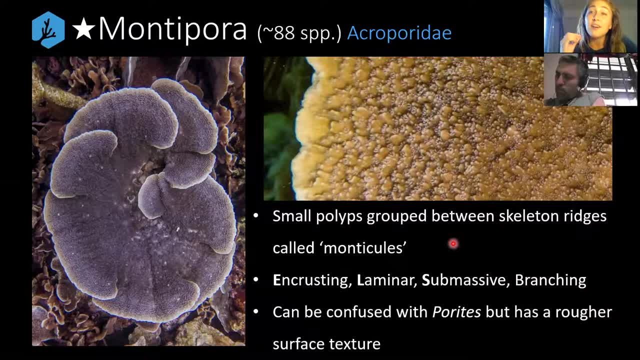 branching sometimes depending on the species. The coral, the polyps, are small, just like a genus called Parites which we're going to look at in a moment, And some people say, oh, that makes them quite similar. But actually I don't really agree with that. 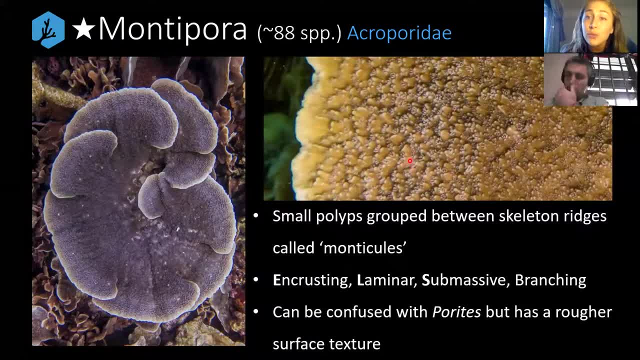 Montipora has this very textured surface from all the monticules, And this is what I'm talking about here. All these little sort of spiky bits in the middle, or fluffy bits, those are the actual tentacles of each polyp. And again, they're nested in between all of these bumps called monticules. So montipora has monticules, you might say has lots of little mountains across the landscape of this coral And all the little polyps are just dangling. 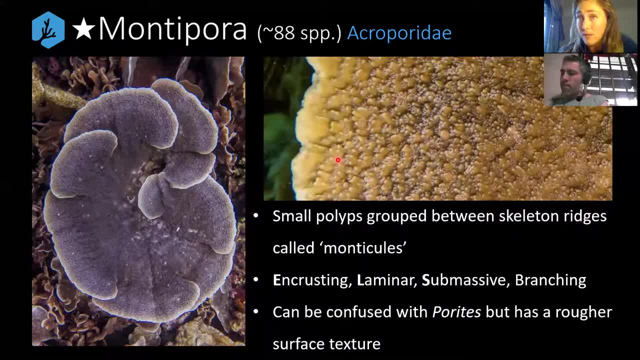 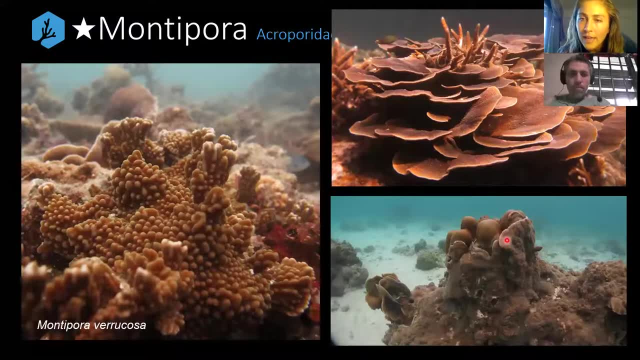 walking along between there Must look like a bit of a mountainous landscape to them or a monticulous landscape to them. All right, Here's another few examples, just showing you guys, how they can grow. So this is actually a different genus called Parites. 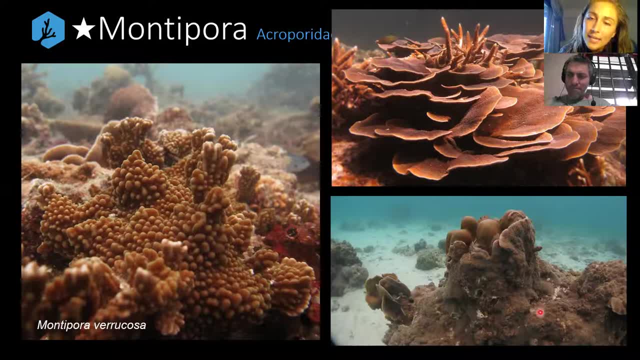 the one I just mentioned, very small polyps, These guys here. this is all montipora, And here again we can see it's sort of taking a laminar growth form. Looks like very nice, delicate little shelves. This is a cool one called Montipora varicosa. 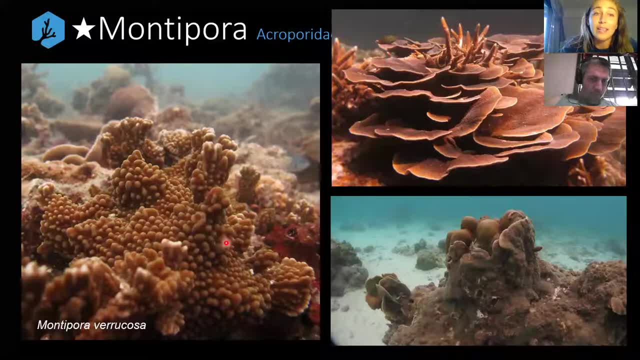 where the bumps are like on steroids. Those monticules are very, quite large, And often, even though they're very large, even though it may not be obvious to us unless you speak a language that has more Latin origin, like, maybe like Italians or something like that, 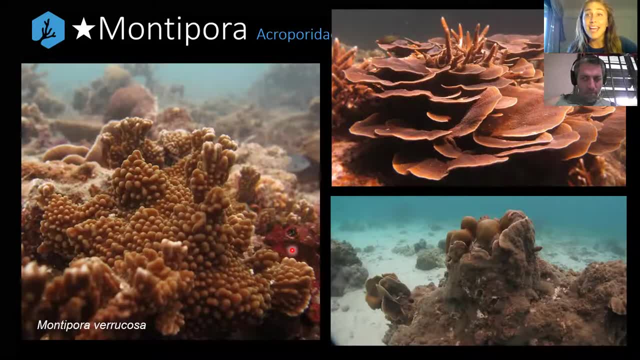 often the Latin taxonomy names of animals quite literally just describe them. So in this case Montipora is the genus name and varicosa is the species name. And varicosa, directly translated, pretty much just means warty like bumpy, like a bumpy wart that you get. 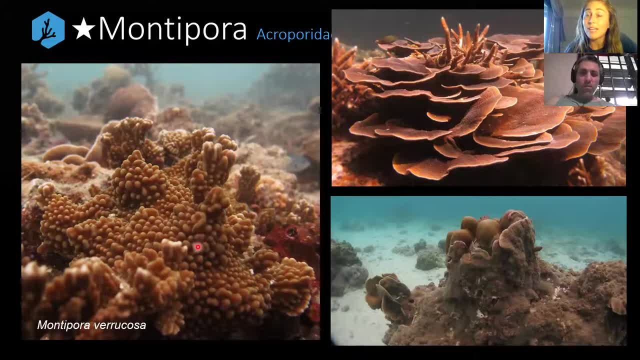 on your skin And that's sort of just simply what it's describing right here: these very large, wart-like mounds over the colony's surface. And there are many other animals that do this too, Like in the slug world, in sea slugs. 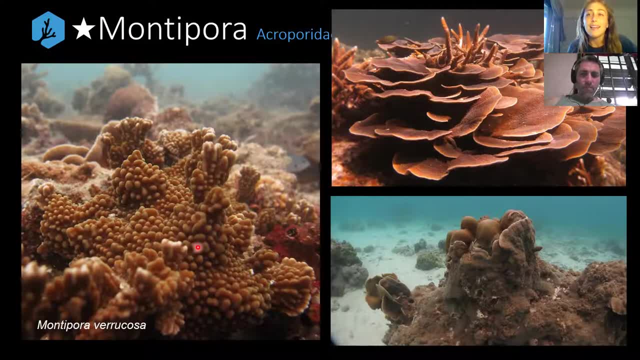 a lot of the species names might be lineata, like Hypsilodorus lineata, And it's a Hypsilodorus sea slug. that's a genus that has lines running down its back, Lineata meaning lines or stripes, things like that. 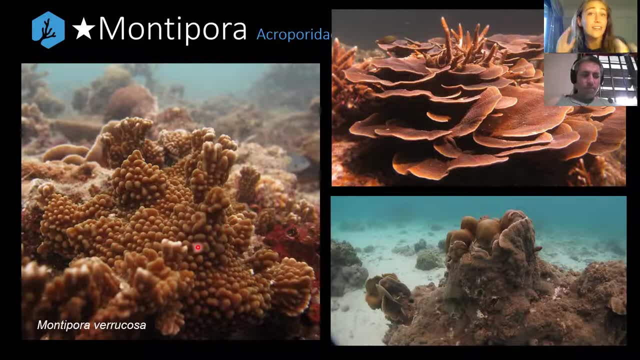 So even though it's unfortunately not really obvious, At least for us English speakers, it's actually really practical names that most of them have been given. So it's still really cool to think about, even though it's not maybe many of our native languages. 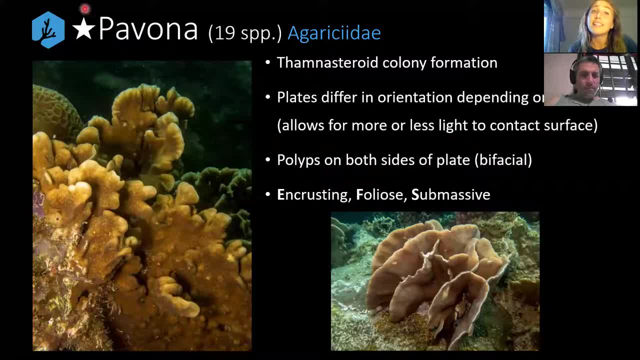 So then we've also got Pavona Note here. we've got another star next to the name, so a high priority to remember. So we've swapped over now from the Acroporidae to the Agaricidae, So this is a really nice family. 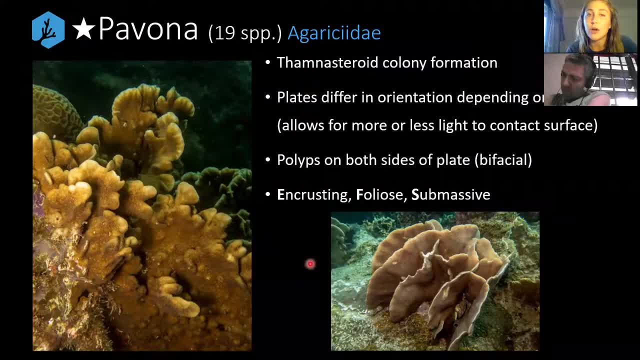 Has that Thamnasteroid colony formation, which we'll show just in a moment on the next slide. a little bit more up close, The plants differ in orientation depending on their depth, which is so cool. So not that we'd ever just move a coral for the sake of it. 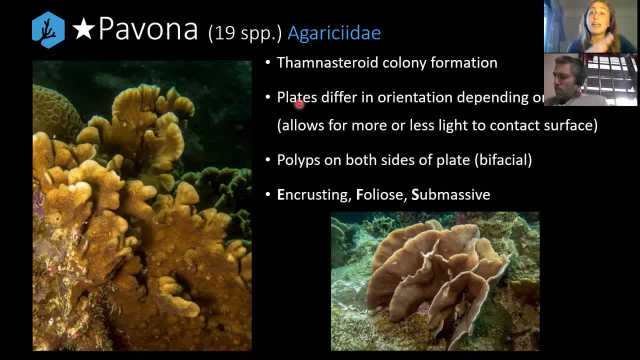 But a single species of Pavona growing in the shallows. that has sort of planting orientation. if it's very shallow it might grow quite vertically, like the one pictured in the bottom right here, And that is because it's in the shallows. 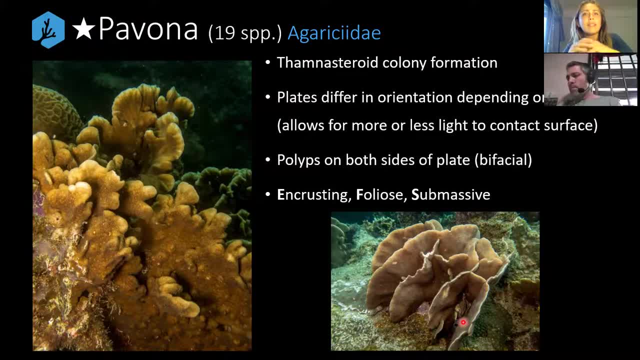 There's plenty of sunlight, You know, Water isn't getting in the way. Maybe the conditions are very clear, But they don't want to get too much sunlight. Maybe they don't want to overheat, which is why they're growing so vertically. 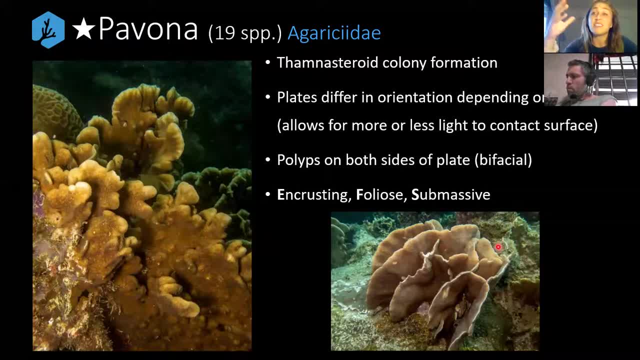 If this colony were to be pushed or were to be somehow transferred to a deeper area- maybe part of the ocean that has got quite turbid, unclear water, or it's just deeper so that less sunlight is penetrating- what will happen is that those plates 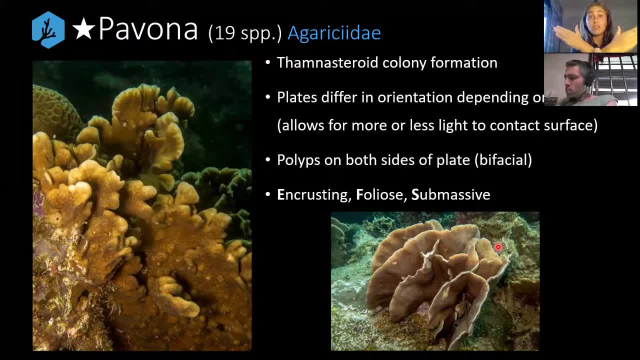 will start to grow more horizontally to pretty much expand the surface In which they can have access to the sun. So pretty much like shifting their solar panels depending on their location so they can best utilize their environment. And if that's not cool, then I don't know what is. 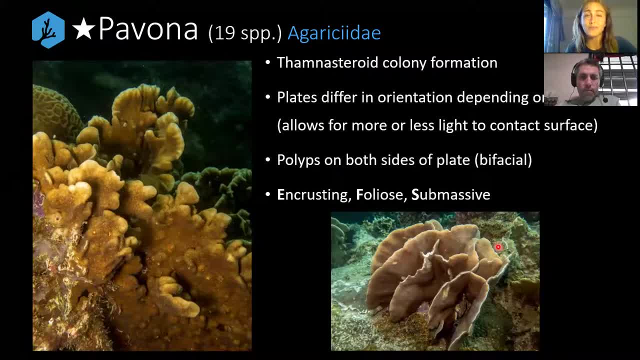 But Pavona very, very cool coral. It can be a little bit of a fast recoverer. It recovers fast after periods of stress. Where I was working we didn't do much transfer of Pavona When we would do coral restoration. 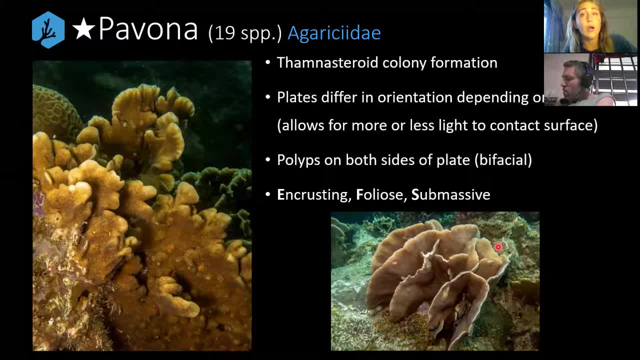 we would work with naturally occurring coral fragments, say, that got broken up during storm surge. We would never frag or break corals because we already had naturally high diversity. Again in the Indo-Pacific this is quite common, But we would do collections of naturally occurring fragments. 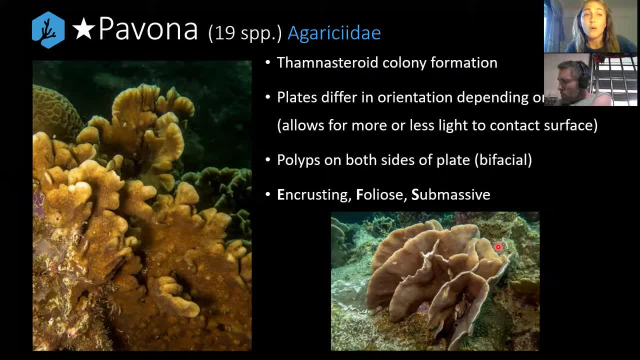 And we would sometimes avoid certain genera because within that area they were in high abundance. We'd prefer to spend our time working on corals if those fragments were available to us that did not have such high abundances, And if we were able to save a fragment of one of them. that 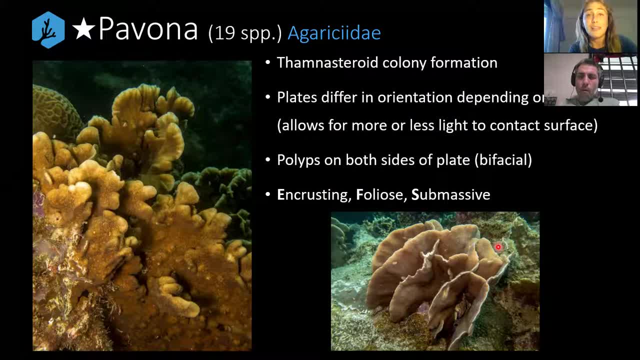 was struggling, it would be more sort of worth our while to use one that did have less representation on that reef than, say, something like Pavona in our situation, But again a very good one to know. They grow as encrusting, growing over rocks, for example. 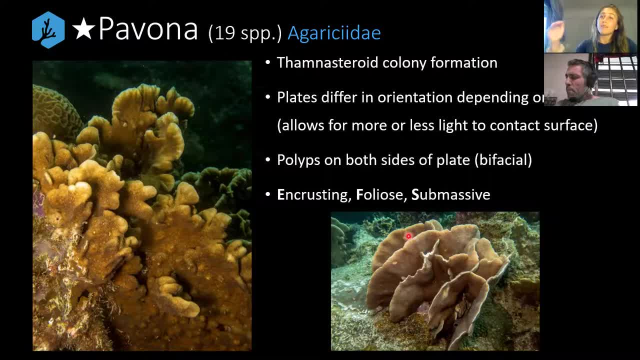 Folios- what we're seeing here- and sometimes even submassive, when they're growing a lot slower there, And good thing to know is that they have polyps on both sides of these plates. Obviously, these are 2D photos, so I can't show you both sides. 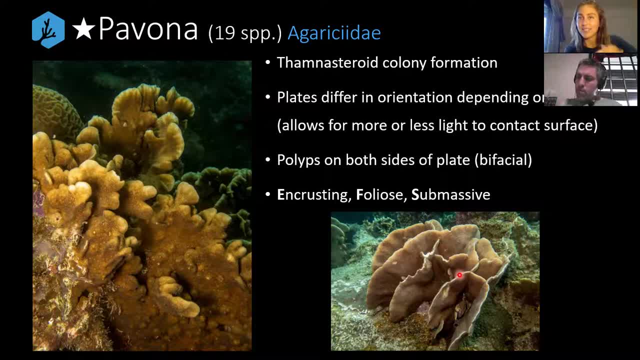 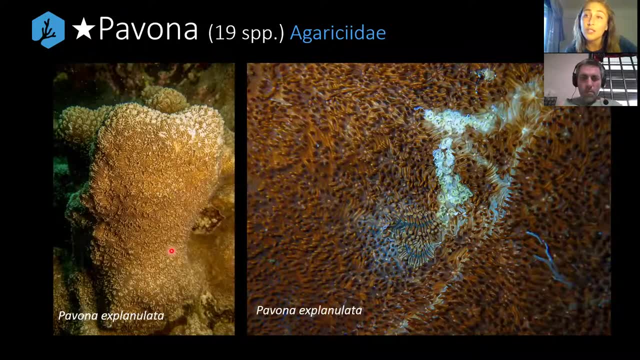 But imagine you're looking at the other side and they look the same on both sides. All right, so here's another photo. These are two photos of the species called Pavona explanulata. That's the submassive one we were just talking about. 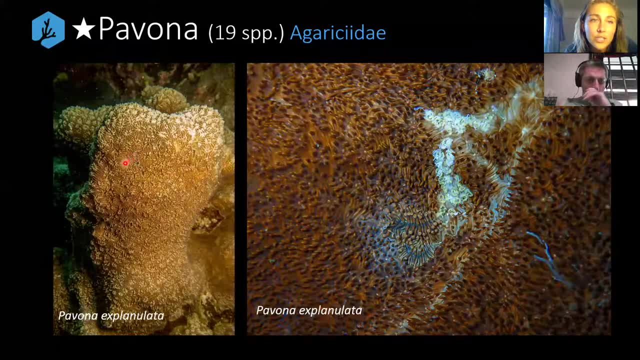 And you can really see here especially the lack of walls, the scepter, And you can see that they're just continuing on from polyp to polyp. OK, Now, if you guys want to unmute yourself, if you want to put up your hand, that's fine. 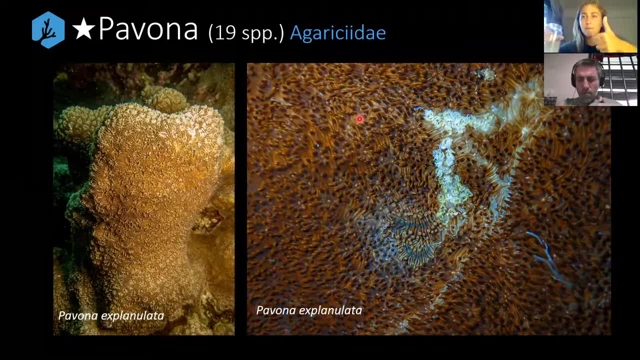 But can anyone see anything weird about this photo on the right Trev? what are you thumbsing up in? Do you see something weird? Disease, Not sure. Trev says disease. Are you looking at this area here? Yeah, That's a really good observation. 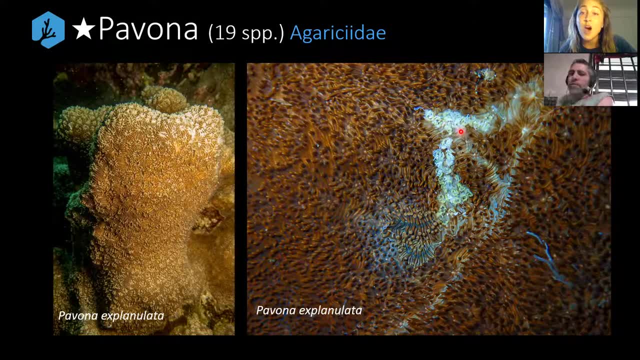 Does anyone? before I tell you guys what the answer is, does anyone want to make any comments or observations about that? If you know what the answer is, maybe keep it to yourself. I know what the answer is because I've done this before. 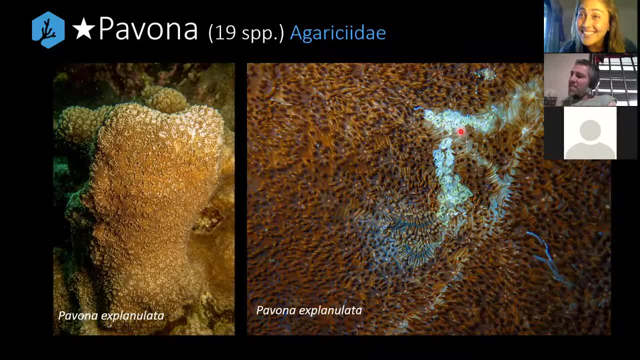 Oh, that's right. So I'm talking to myself. It's a good one, isn't it, Zakia? Yeah, it really is. Yeah, It really is OK. so Trev was totally on the right track. Well, OK, he's noticed that something. 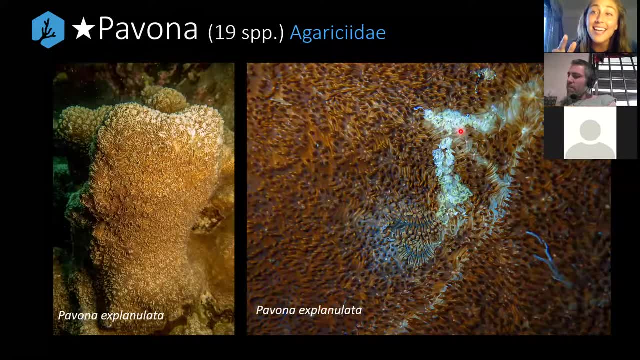 is not quite right with the corallites, the right track. It's not disease, though, This, my friends, It's a sea slug and it's egg trail. So we have got two sea slugs here from the genus Fistula. 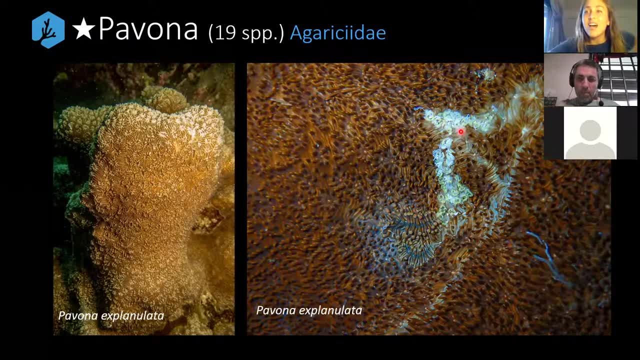 And some of our team members at Conservation Diver describe this genus or this species to science. So this here is a sea slug and this is another sea slug, So there's actually two here, and this sort of white-yellow trail is a series of egg ribbons. 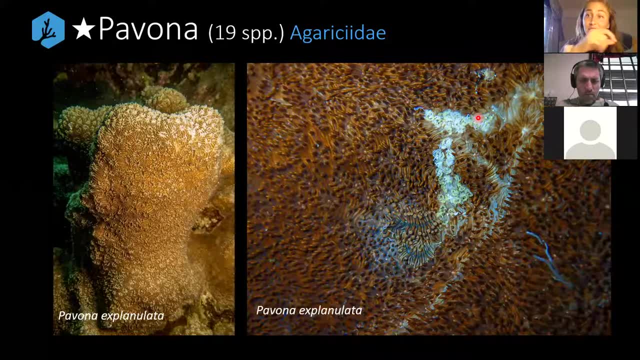 They've just done the dirty and they're laying all their fertilized eggs down so that they can develop and then hatch. So that's awesome. This was referred to as Fistula species three for quite a few years, And then our buddies at Conservation Diver. 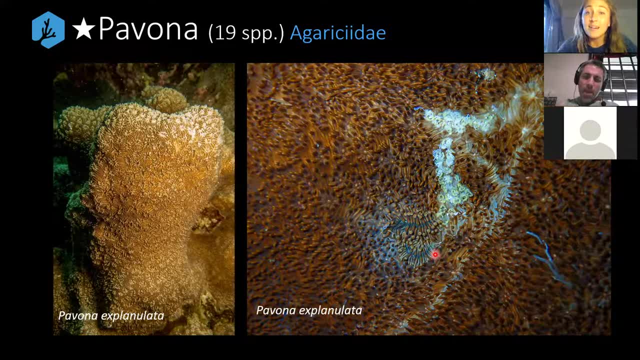 one's called Spencer Arnold, one's called Rahul Mehrotra. they, together with a couple of other people, actually end up describing these guys getting samples, genetically testing, et cetera. And now it's called Fistula v And these guys 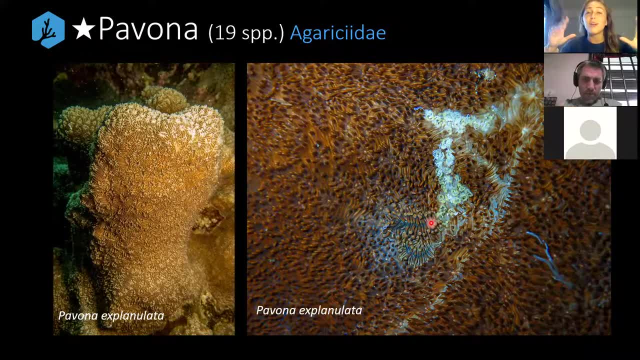 are awesome, So they their whole life motto. sorry, I know this is a coral lecture, but I'm just going to quickly do it anyways. So their whole life thing is that they've got this coral. They look just like it. 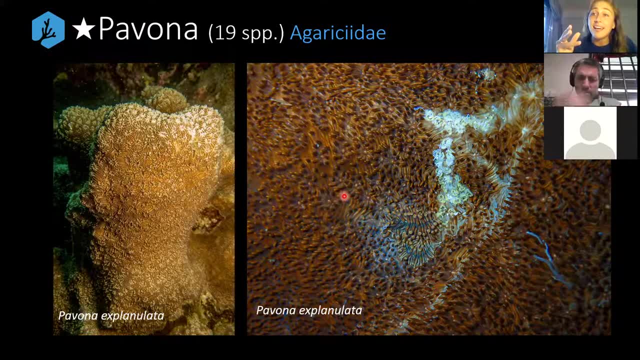 They eat it, They mate on it, They lay their eggs on it and then they die there And they just hope that nothing notices and eats them in the meantime. That's their approach to life, And I think that's just so cool. 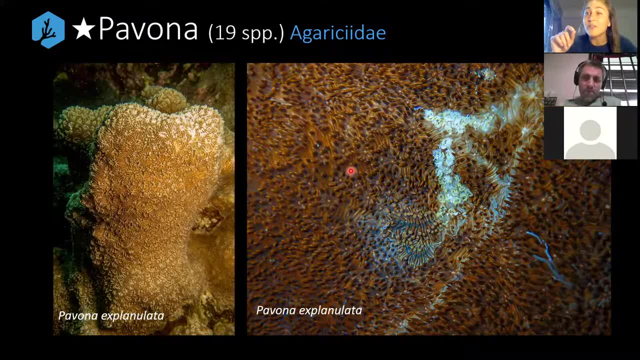 They even, they even will eat the coral and utilize the zoo And they have a zooxanthellae in that coral. So for those of us who it's been a while, for corals are animals. They've got polyps and mounds. 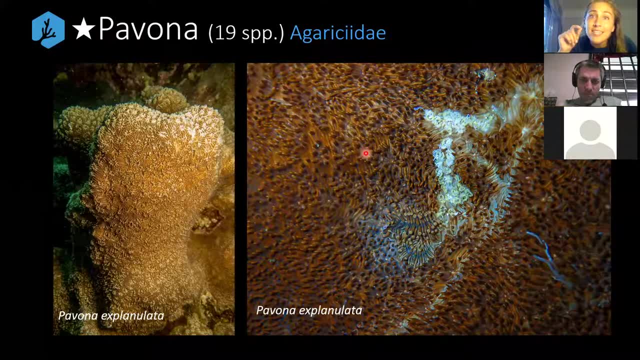 You can see them around here and here and here, And they've got a symbiotic relationship with the symbiotinium called zooxanthellae, which are little plants essentially, And that's what gives the corals their color. So these slugs eat the coral tissue. 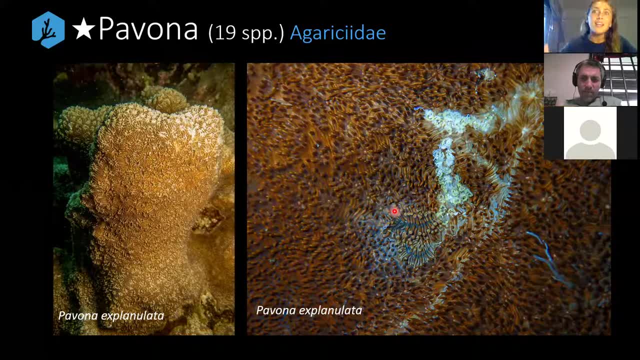 and then keep intact the photosynthesizing mechanism and incorporate it into their mantles. They're gastropods, And then they can even photosynthesize. That's so cool. Anyways, I just quickly want to show you guys two more. 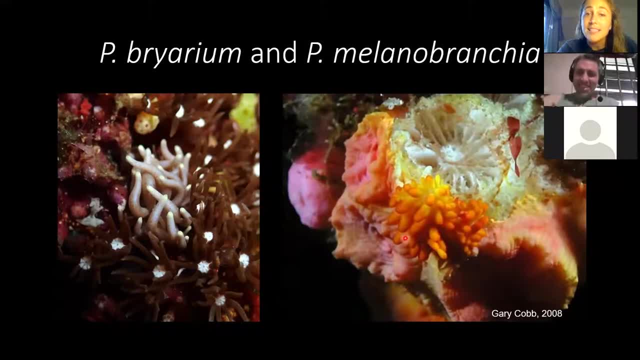 This is my photo. This is a Fistula bryerium And this is a Fistula melanobranchia. Sorry, I forgot the name there. So they look like different corals- This one. it's quite easy to see. 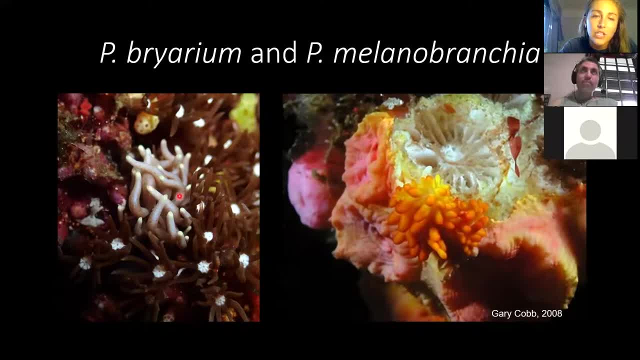 because these tentacles of the slug look just a few shades lighter than the tentacles of the coral here, But again It just blends in. And here's another one. This one's not my photo where they've got the coloration of the coral behind it. 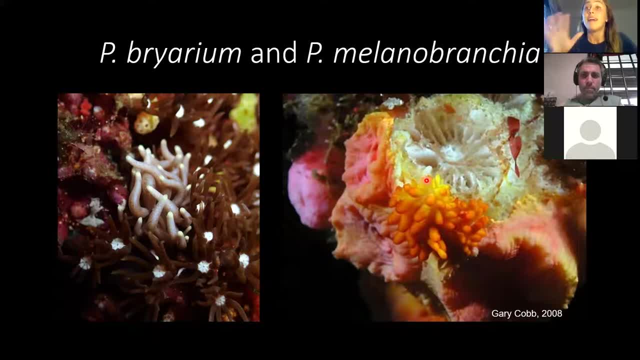 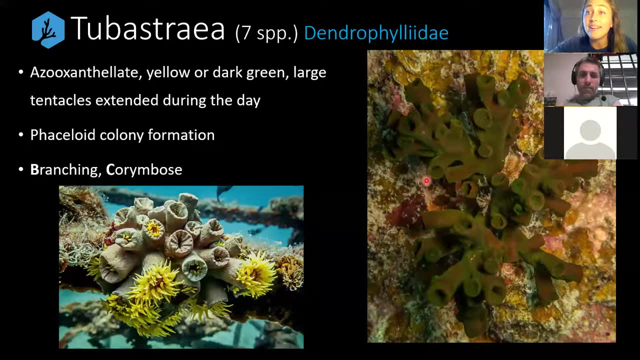 And you can see the mortality that's being caused there. Anyway, back to corals. Just wanted to show you guys some cool other stuff as well. So let's move on to Dendrophilidae as a coral family. Does anyone know any interesting facts about Dendrophilidae? 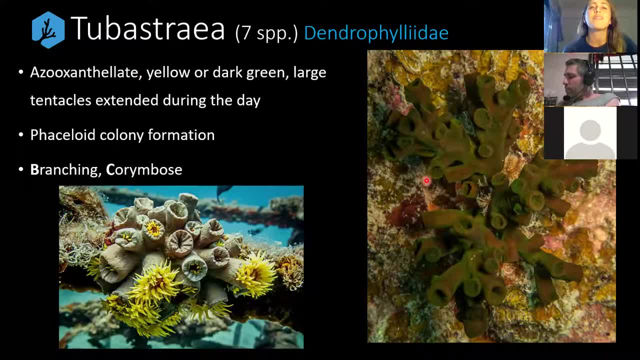 Oh wait, Actually, I just realized it says it on the slide, So I'll just continue. So the Dendrophilidae- not every single one of them, but a lot of them- are A zooxanthellae. 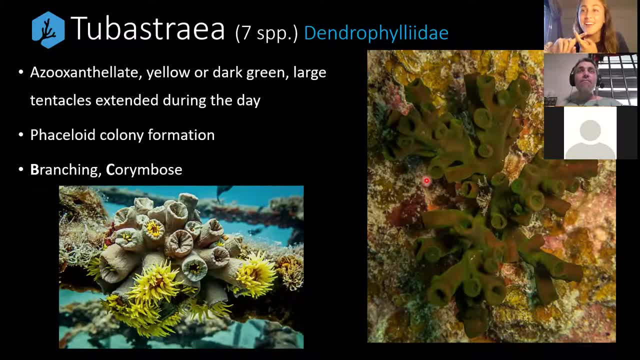 So that symbiotic relationship we're just talking about with the zooxanthellae doesn't exist for all the corals. So they are A zooxanthellae, which means they do not photosynthesize because they haven't got that relationship with the plants. 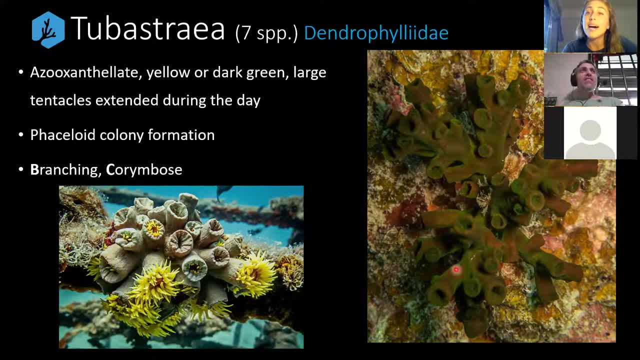 OK, Tubastria are generally yellow or dark green. OK, If their tentacles are contracted, like in these photos here or not, quite down the bottom, that means that they might be feeding or they might not be trying to feed at that point in time. 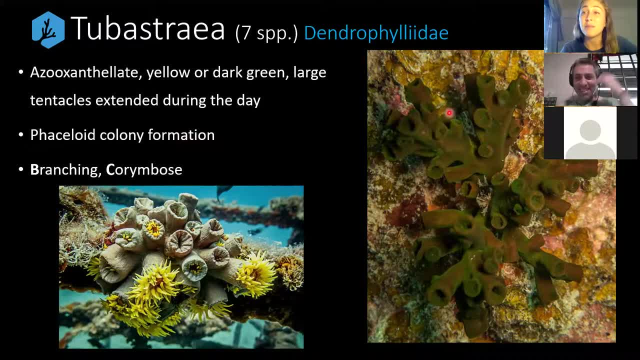 for some reason, And that's just the natural pigmentation of the proteins within their tissues. So they don't bleach due to heat, for example, like corals that are zooxanthellate do OK When the water gets too warm. most zooxanthellate corals 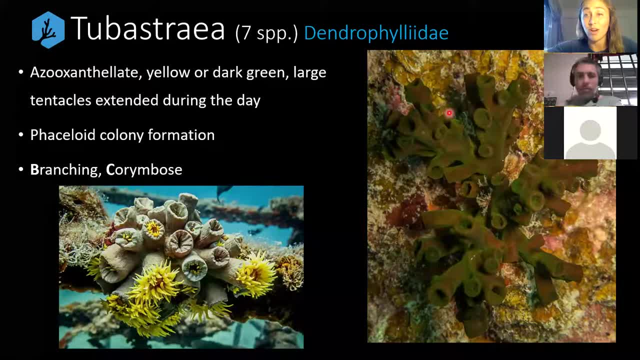 might expel the zooxanthellae Because the conditions are no longer right for them to continue photosynthesizing. But these guys don't have that reliance, which means that they can absolutely take advantage of conditions and locations that other corals cannot. 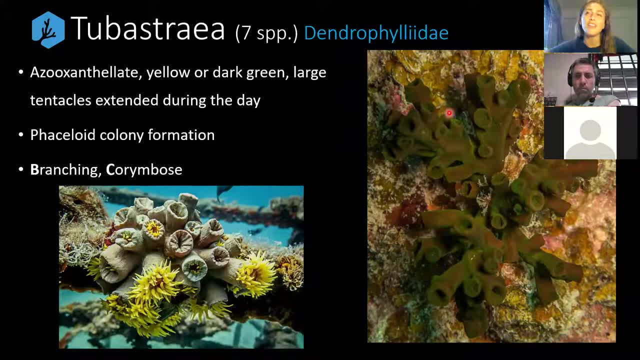 Can anyone tell me where a coral that doesn't rely on sunlight might be found, compared to a coral that does rely on sunlight? Underhangs of the reef- Yeah, Underhangs on the reef, Exactly, But also just deeper in general. 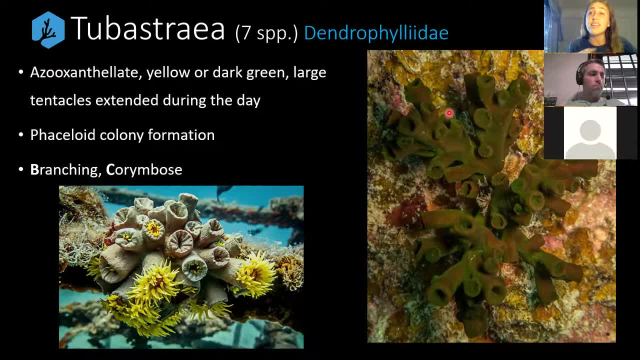 So where I've done a lot of my work- often the sort of standard coral genera that we see all over the place. they start to thin out and are less and less frequent after 15 meters or so, maybe 20 meters, Whereas these guys will start to become more abundant. 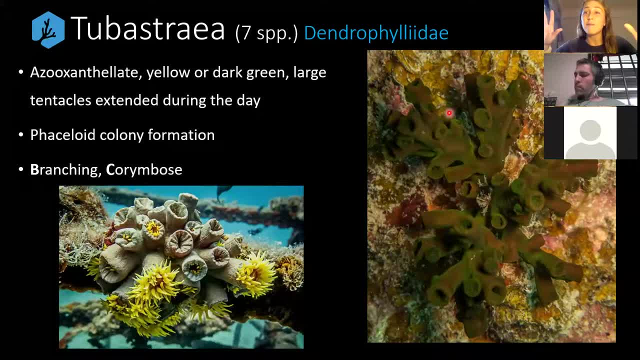 after those areas, Because there's all this available hard substrate that these other corals really struggle to make the use of Because they can't photosynthesize And that's where they get most of the energy. These guys are like we don't need the sun. 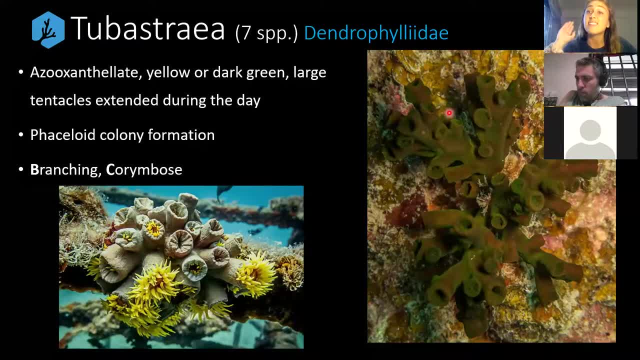 We eat ourselves. We're heterotrophic And they can just live wherever they want to, pretty much. Of course, there are other conditions that need to be appropriate, such as pH and so on, But they can make do without that light, which. 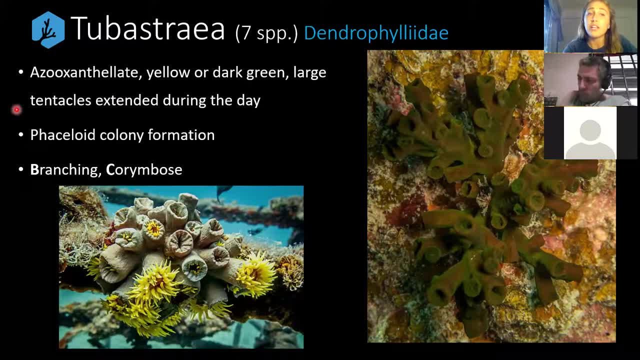 is really, really cool. So they've got a phasaloid colony formation. So again, the polyps are very separated and tubular is the easiest way And you get them quite branching And corumbos as well, And I think Tubastria is a very easy genus. 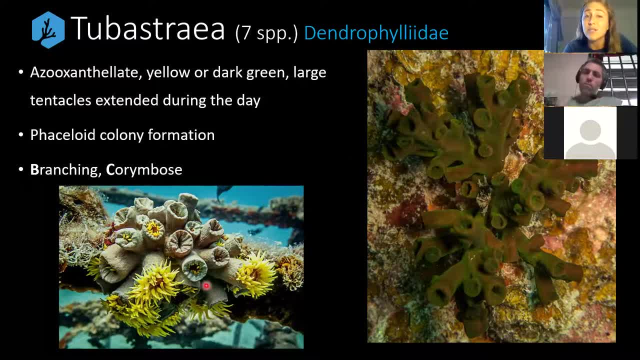 to remember because Tubastria looks like a series of tubes. Easy one, right. It's not as essential as, say, the Acropora in terms of the frequency of its mention, But I hope you guys remember this one because I think it's a pretty easy one to remember. And also really pretty. Sometimes they're called, or often they're nicknamed, the sun corals And you kind of, when you see them with their tentacles extended, You really get it, You really do understand why- Awesome. So then we've got another Dendrophilidae. 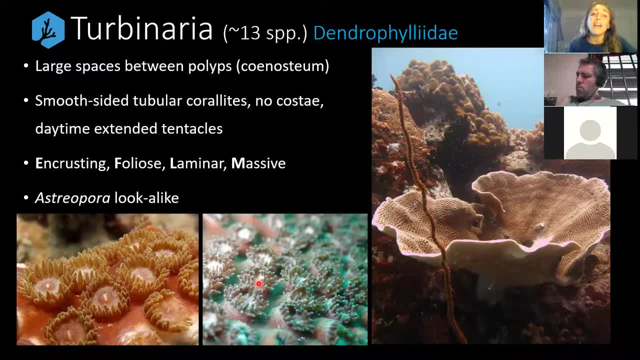 which is called Turbinaria. So these guys have quite large spaces between the polyps. Again, scientific word for this is the synastrum, So this space in between where all the polyps are Pretty easy, So smooth-sided tubular corollates. 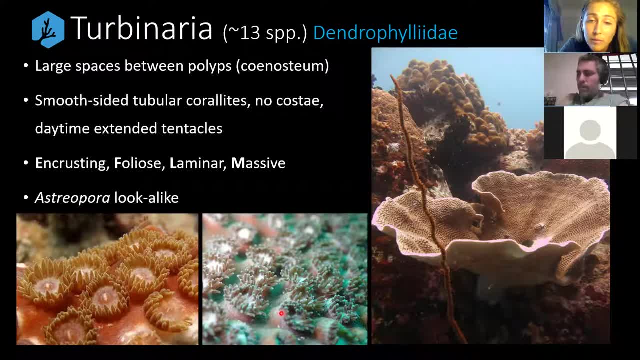 which is talking about literally the sides of the corollate. So if you guys can see where my cursor is, those sides are very smooth up until you get to the tentacles, in which then it's tentacles galore. We don't have any costae. 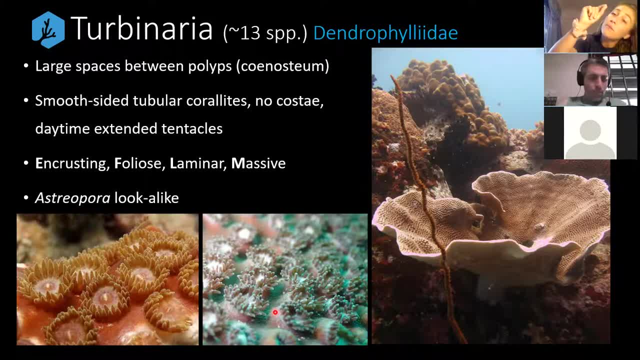 Remember, the septa come up from the mouth to the wall And from the wall down would be where the costae are, But not all corals have them And this is a coral that doesn't OK. Septa would be there underneath the tissue. 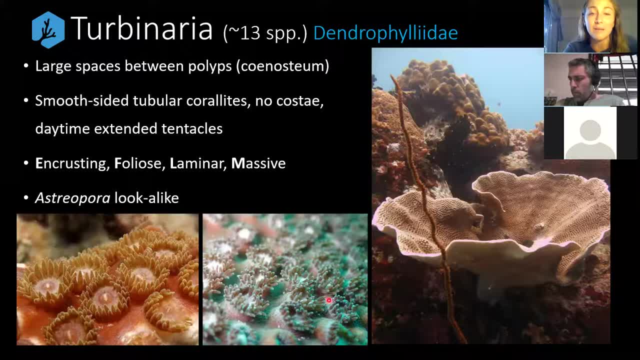 But they're so tentacly that you can't really see them, at least in these photos here. We typically get them in crusting in folios, sort of vertical, thin structure, laminar and massive sort of growth forms as well. 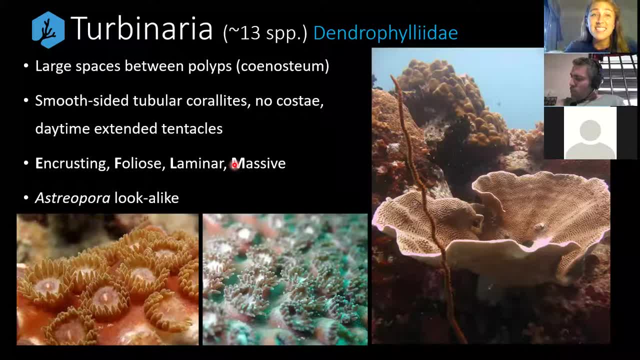 Interestingly enough, I'm in Perth at the moment, And down south of here, even a few hours down south, I've seen massive colonies of turbanaria And it blew my mind. So, so, cool. I didn't think they were just existing in such cold waters. 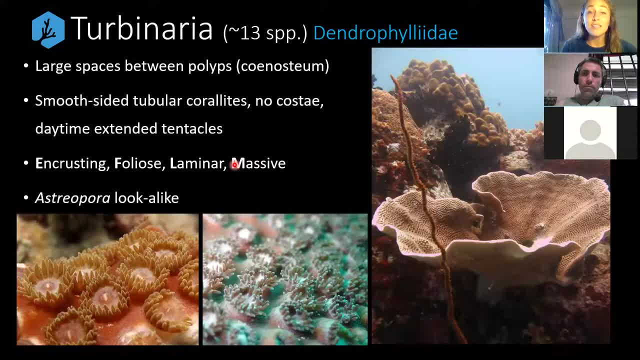 Sorry, just knocked my computer, But yeah, Really really great. Some people say they look like Astraeopora, And when we're looking at a colony like this, for example, from a bit of a distance, remember Astraeopora is the one that looks. 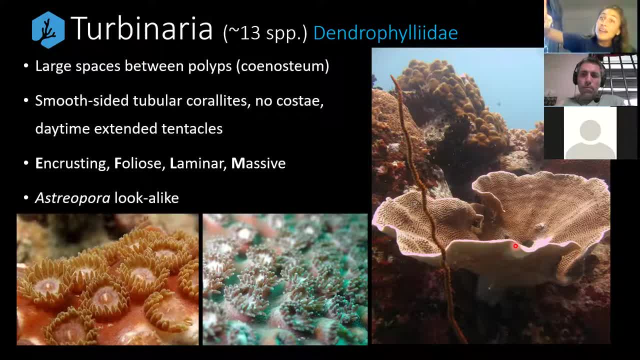 like little asteroids hit it, Very sort of bumpy, googly eyes being spread all over the place. That kind of bumpy nature. from a distance can look a little bit like turbanaria too. But we get up close We can see that turbanaria has got these daytime extended. 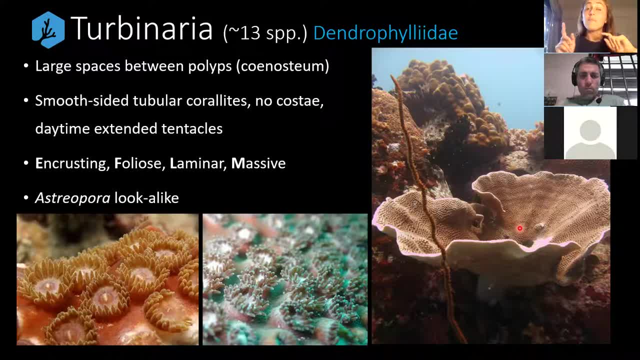 tentacles. They're also azes and phthalate, Our Astraeopora, have got the little pebbled appearance to them, all these spiky little bumps called spicules as well. So those are the main differences there. 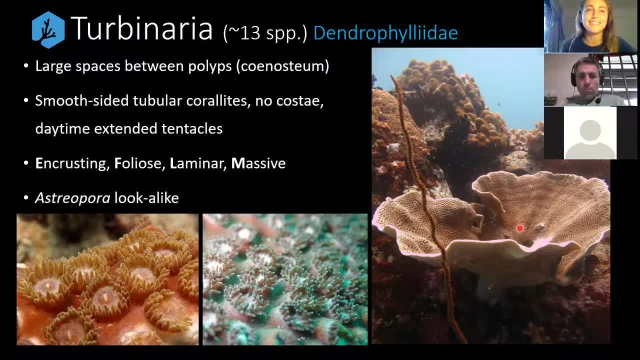 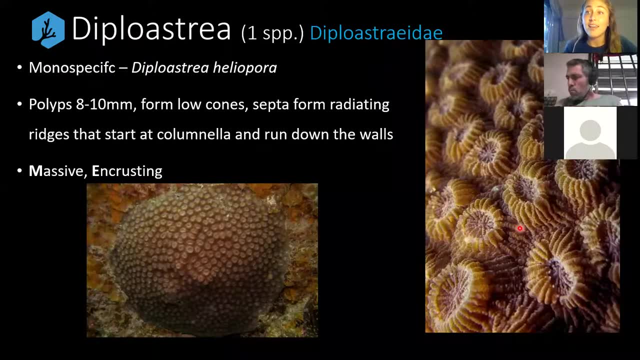 So pretty good one, Good one, Good one to know, Awesome. So then we've got Diploastria, which is our first monospecific coral genus of the talk. I think, Yeah, no, it is, And it's called Diploastria heliopora. 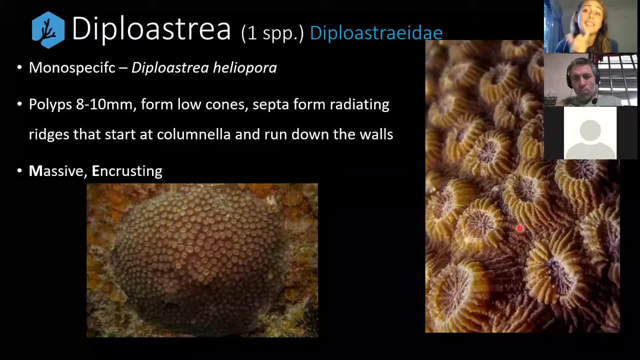 Monospecific means that within the genus it's called Heliopora. Heliopora means that within the genus it's called Heliopora. Heliopora means that there's only one species. So if there's a single species, I implore all of you guys. 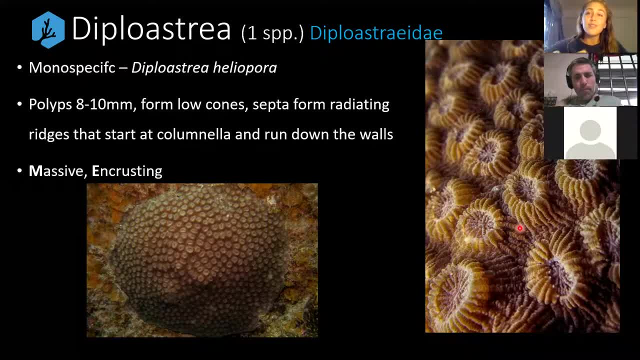 to remember. I would say it's this one. So then you can be like snorkeling with your friends and you see this coral and you go: oh, Diploastria, heliopora, friend, that's what this is. And they'll say: holy moly, you know your coral species. 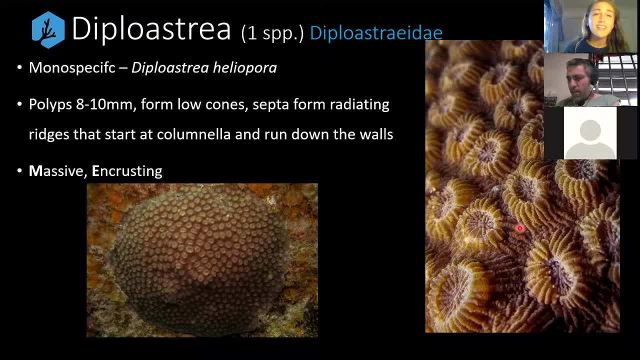 That's so cool And you'll just be like, yeah, I am what I am. I know my coral taxonomy. What can I say? I know all the species, even if you don't, But you can learn this. Learn this one. 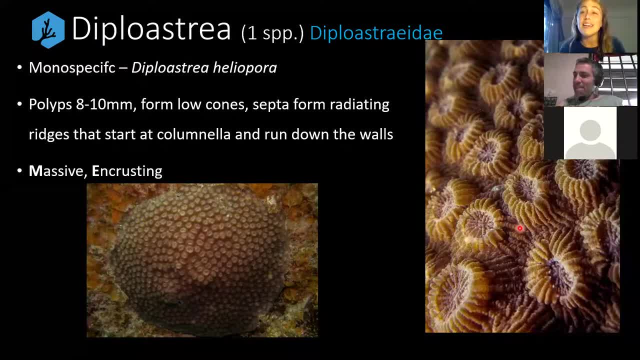 So Diploastria heliopora, single species. It's got large polyps ranging from 8 to 10 millimeters across, so maybe nearly a centimeter across. Usually it's kind of like low cones, like a cone that's sort of been pushed inwards. 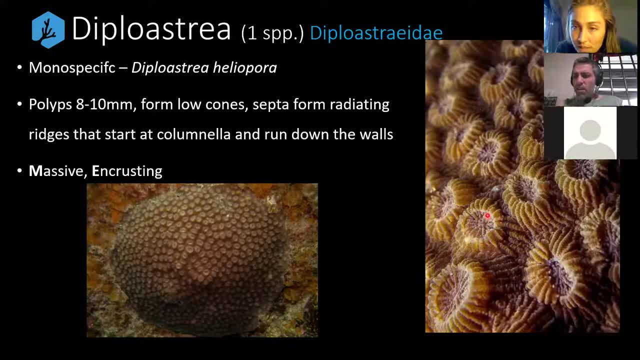 And its septa form is radiating sort of ridges, as we can kind of see coming up around here And they eventually run down the walls into the costae And technically every coral does start as encrusting when it's just a few polyps large. 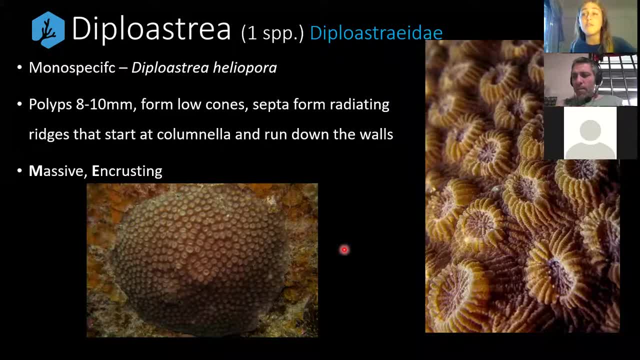 But these are the corals especially- yeah, it's just in the Indo-Pacific. This one doesn't exist in the Caribbean Often forms these sort of huge dome-like structures And they're very impressive. What large Diploastria heliopora can signify on a coral reef? 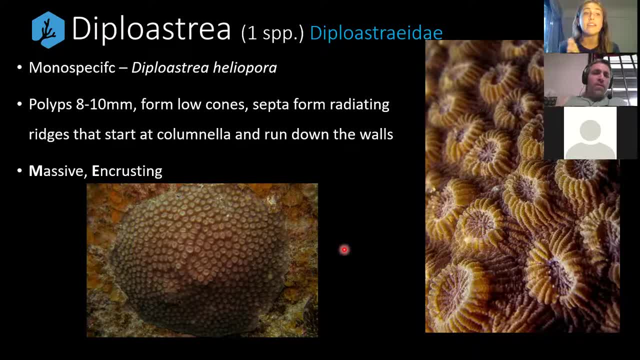 ecosystem. is that actually what they could signify? if, say, you're diving in the area and there's very little in terms of coral coverage, but these, these guys are existing, you can think to yourself, OK, this area clearly does support coral life. 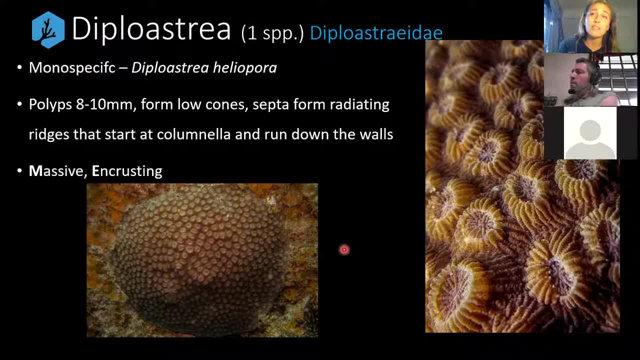 because this coral is living here. It's very slow growing, So this area has supported coral life for a long time. But if there's no coral anywhere else- or maybe you see the rubble leftovers of coral- what you can think or what you can sort of conclude from that? 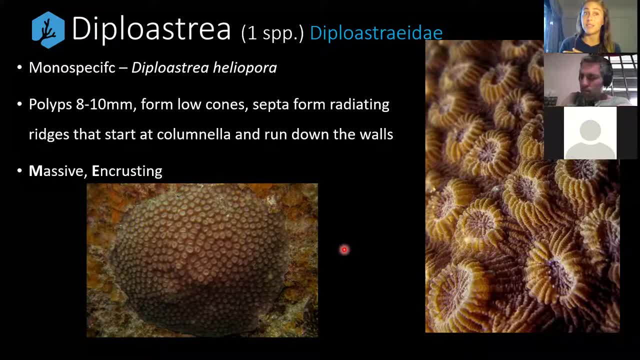 is that there may have been some rather recent disturbances. So Diploastria are very good at recovering. They grow so slow And they put a lot of energy investment into reserves, Whereas our other corals, like maybe our Montiporas and our Acroporas- they were both from the Acroporidae family- 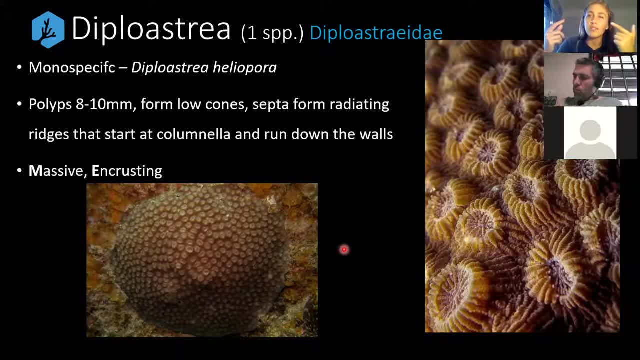 that we were talking about earlier. They were more fast growing, if you guys remember. And even though they were fast growing, and that's all well and good, they're also more susceptible to stress because they weren't putting all of this energy into reserves. 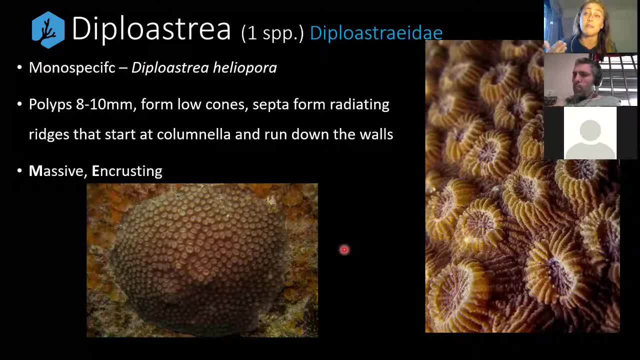 and lipid stores essentially, So they're also more susceptible. They're more susceptible to bleaching, to cyclones, diseases et cetera. So presence of maybe rubble patches and lots of Diploastria says there's been some stress here. 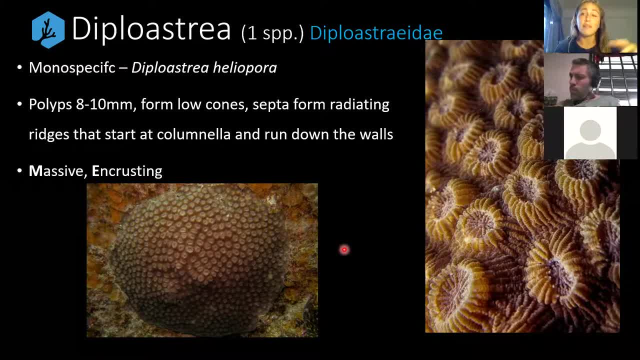 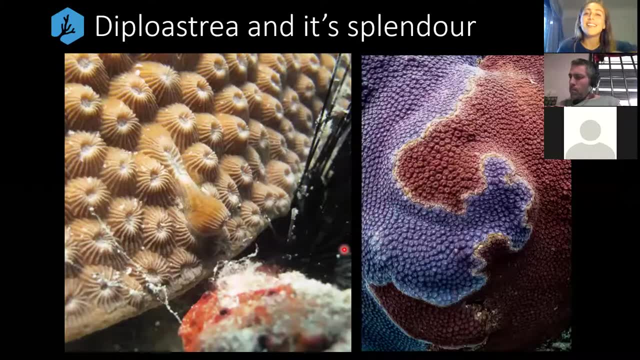 But clearly this is an area that can support coral life And it can give you a bit of an idea about the timeline as well. Let's just look at some cool Diploastria photos. So these are provided by our good friend and founder Chad. 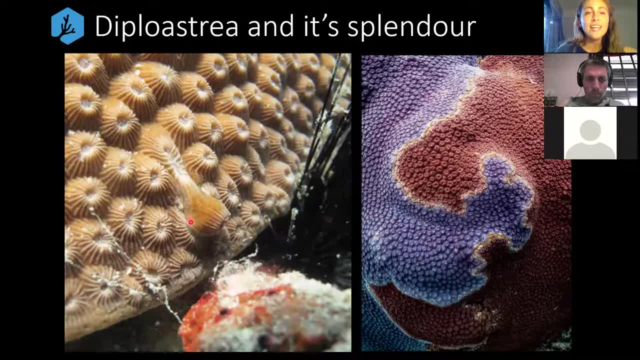 Scott And he sent me this photo once And I was like Chad. it looks like someone took a blowtorch to this Diploastria And a polyp is just like melting off the side And he said it's budding off. 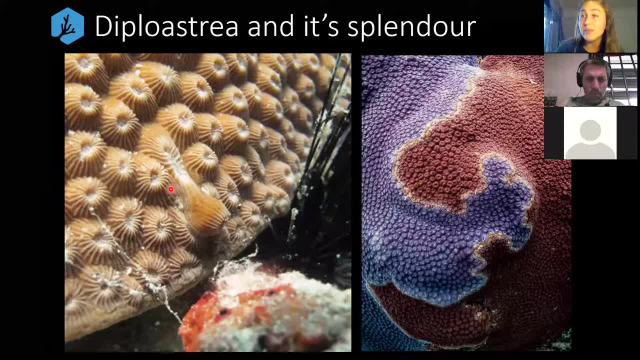 And I thought, wow, I didn't know that was a thing. But here we are. So isn't that just crazy everyone? Second photo: on our right We have got competition within species, but different individuals. OK, If this was the same. 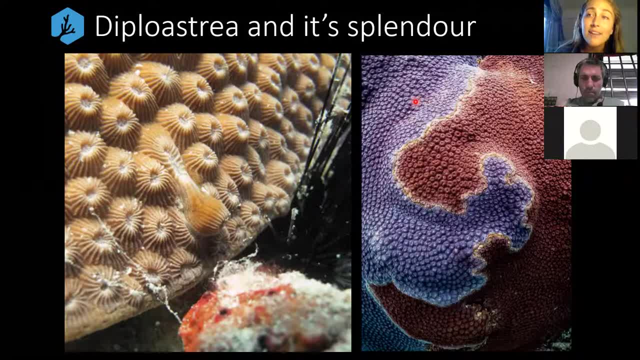 These are two Diploastria helioporans. We can tell that they've got different clades of zooxanthellae species- sorry, species of zooxanthellae- within their tissues. We've got this sort of different color happening here. 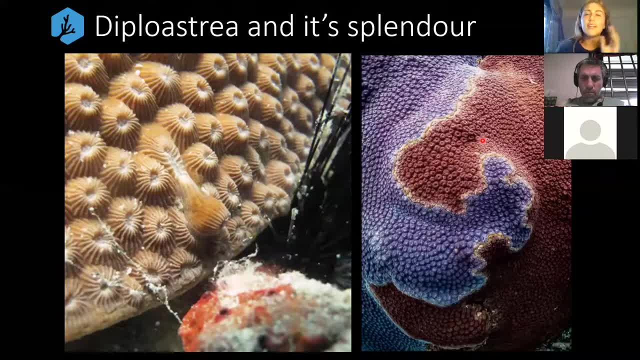 And they're competing for space. Coral reef ecosystems are such a huge competition for space, like all the time, for that hard, valuable substrate, that rock or dead coral that we were talking about a little bit earlier, And when corals are growing and they meet. 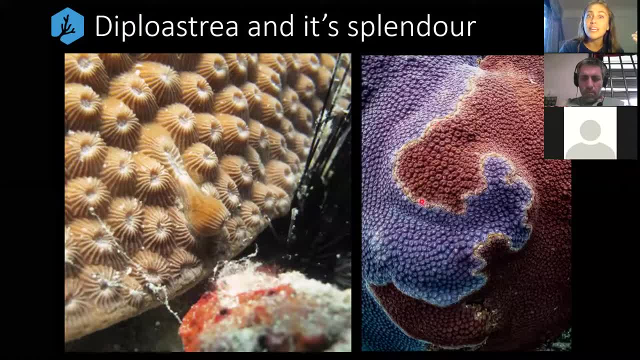 it's like flight to the death And you get these really, really, really, really, really, really really beautiful, interesting patterns forming along the edges. One might be winning a little bit over here, a bit further down, The other one might be winning. 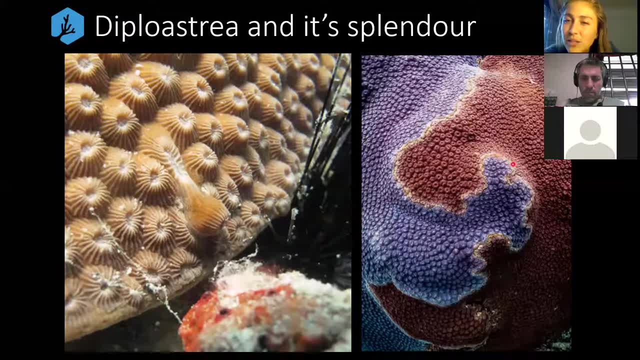 But you can see that there's a little bit of paleness and nearly like a little bit of bleaching. That's just the stress of the colonies actually fighting each other. you can say, But really cool, And of course this is just interesting. 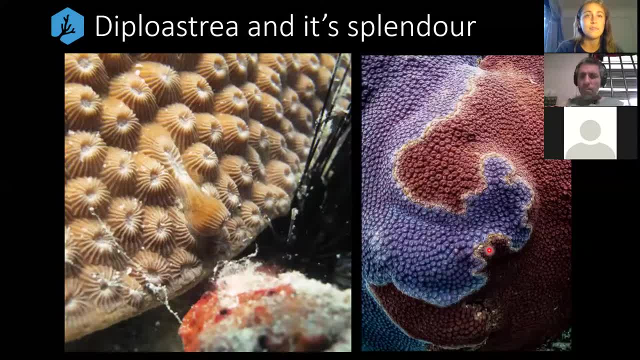 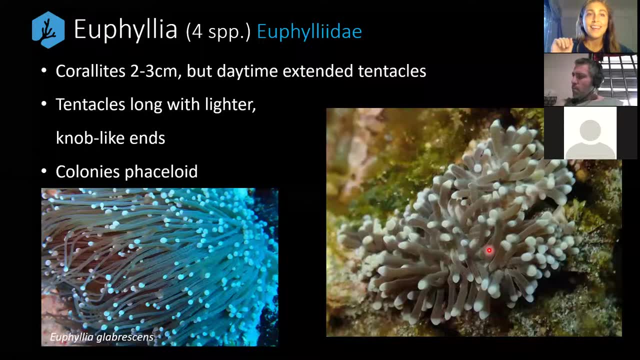 because it's a war between two of the same species, which I guess is what we do too. Anyhow, There you go, Very cool diplasteria and all of its splendor. So moving on to different family, that being the Euphyllidae. 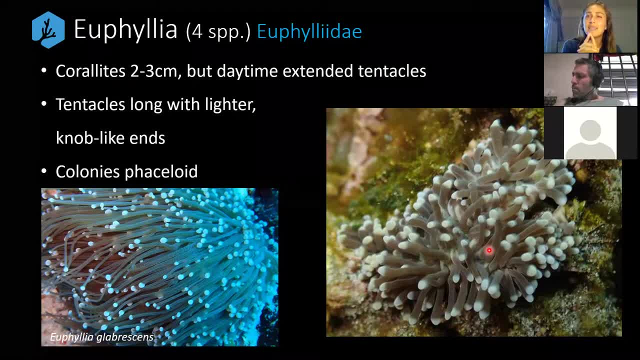 So first let's look at Euphyllia. Now some of you guys might be thinking to yourself: that's not Euphyllia. I remember it being this overlooking coral. Remember how I said earlier that, as like taxonomy, 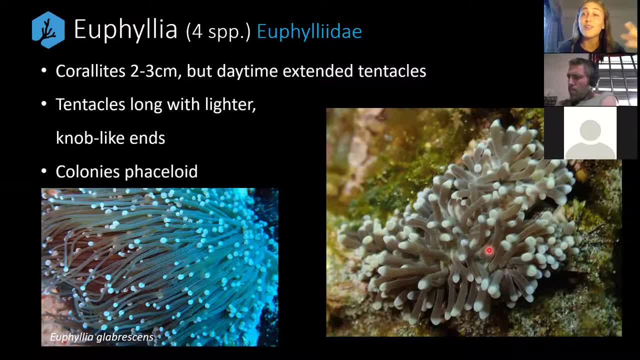 and genomic sequencing and DNA is technologies advancing that we're pretty much getting more correct in terms of our taxonomy than we used to be. So this is one of those families in general where there's been a little bit of shifting And we realize, oops, we did something a bit wrong before. 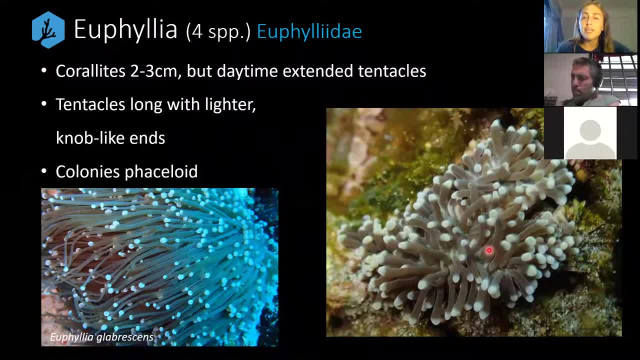 We're going to fix it up. So Euphyllidae is pretty characteristic by having these beautiful long tentacles And the next few slides in general we're looking at are all going to have these sorts of characteristics. But yeah, we'll dive into it. 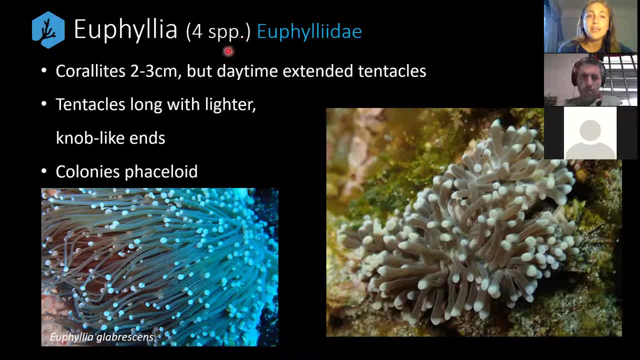 So Euphyllia as a genus here has four species. The correlates are two to three centimeters And you guys might be thinking to yourself: where's the correlates in this photo right here? And I can tell you I don't know. 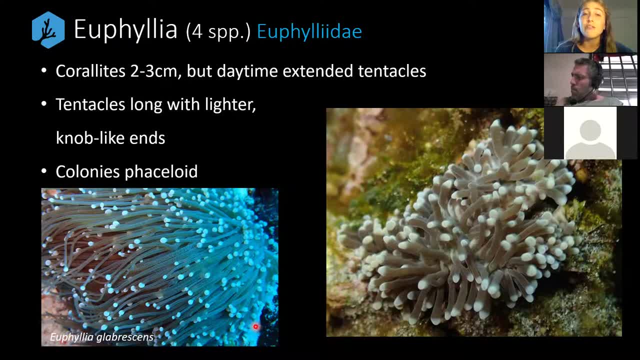 They're under there somewhere But we can't tell because they've got these wonderfully long daytime extended tentacles. The ends of the tentacles have these kind of really cool lighter-colored- not black- ends. That's pretty characteristic of all the tentacles. 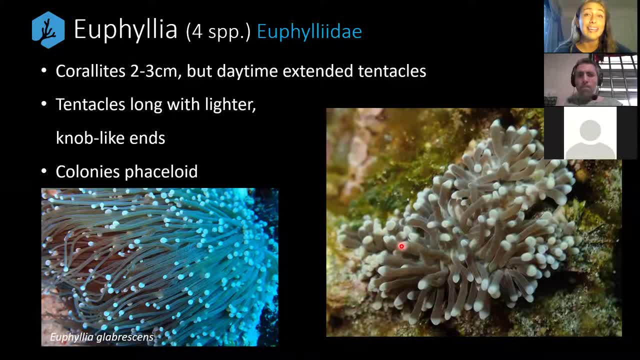 within the Euphyllidae family, at least all the ones that we're going to be looking at in these lectures. And the colony? it's a phasaloid. That was the colony formation that we were talking about before separate correlates. 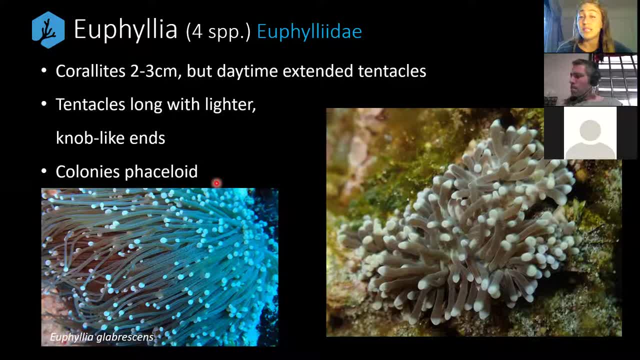 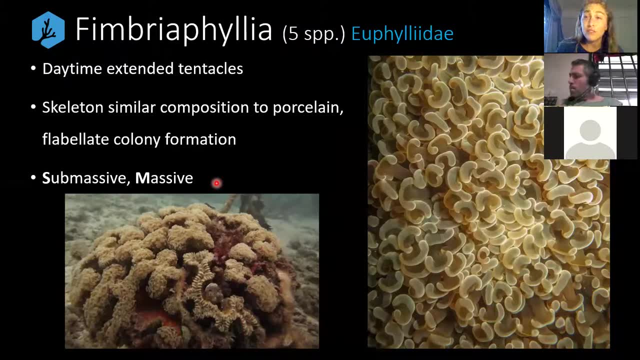 But we actually can't see, unless it was dead and all that was left was the skeleton. all right, So let's look at the next Euphyllidae, which is now called Fimbriophilia. Some of you guys have been to the program New Heaven Reef. 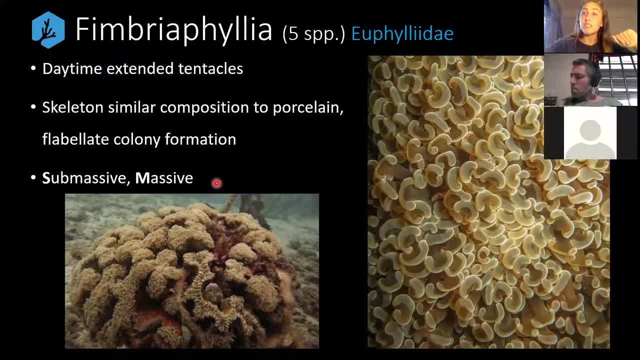 Conservation Program, which is the first conservation diver center that existed, And it used to be that this was called Euphyllia. Sorry, it's been reclassified, So now it's called Fimbriophilia. OK, And it's got the daytime extended tentacles. 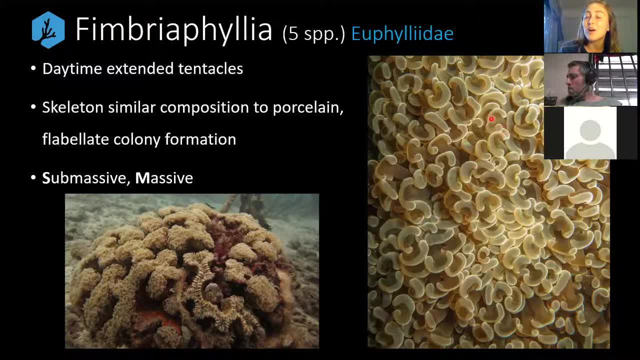 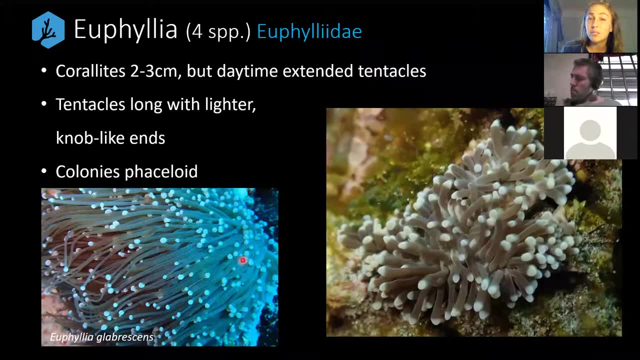 these often kind of jelly bean or hammer-like corals. This is often nicknamed the hammer coral, But it's got that kind of glow and light tip to it, just like the Euphyllia tips do there. The skeleton is kind of similar composition to porcelain. 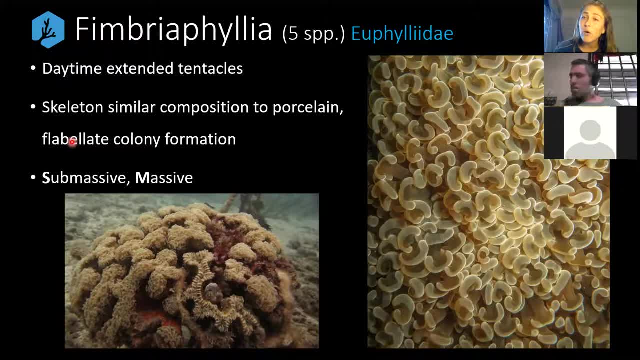 It's got a flabellate colony formation And that's what I was saying before earlier on in the lecture about these. it looks like they're a big, big gaps, like big chunks missing out of the colony And there isn't. 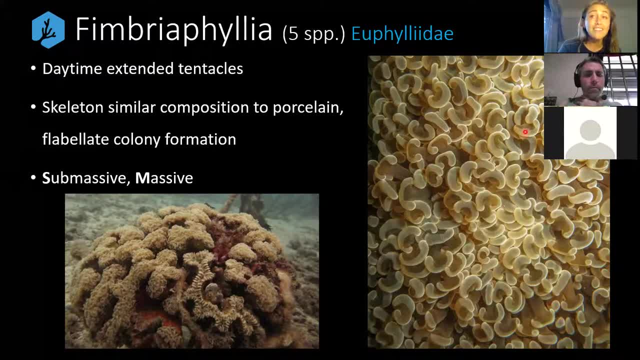 That's just the way it grows. When the tentacles are out again, you can't really tell, Whereas when they are retracted here, if they're feeding, if there's been a disturbance, that's when you can actually see it. OK, 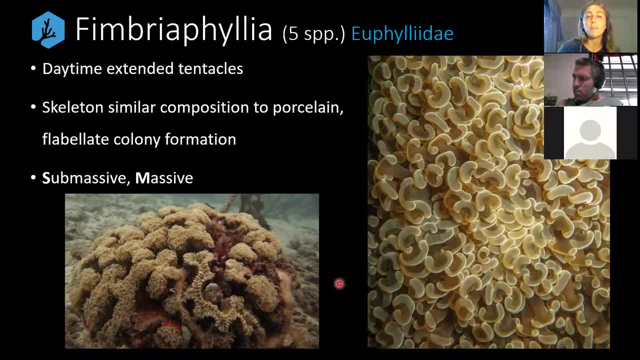 And we get them growing these sort of massive and submassive colonies. And I forgot, guys, Euphyllia, One of my friends, Kate, one of the other instructors at Conservation Divers. she said: always remember Euphyllia because it's just so pretty. 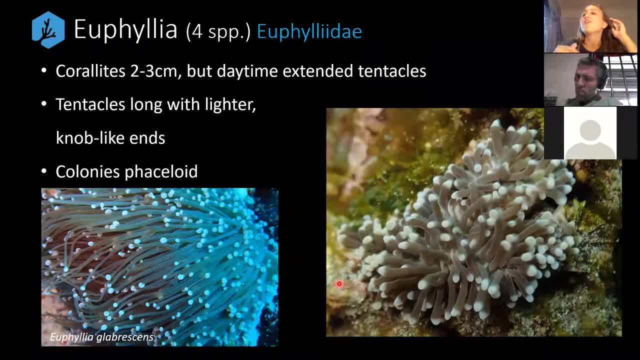 And you know you have these long, long tentacles and I love it And I feel euphoric whenever I look at it And I go, ah, that's a good mnemonic device. So she had that little word association just because it happened to be one of her personal favorites. 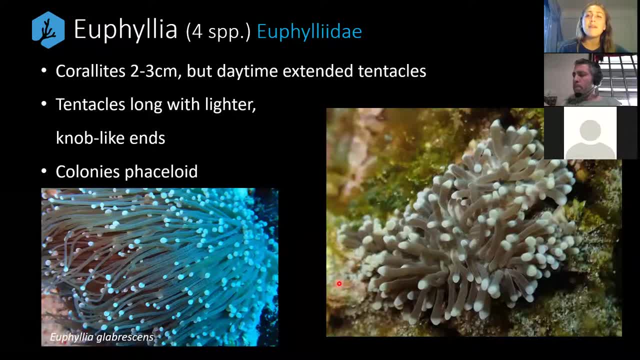 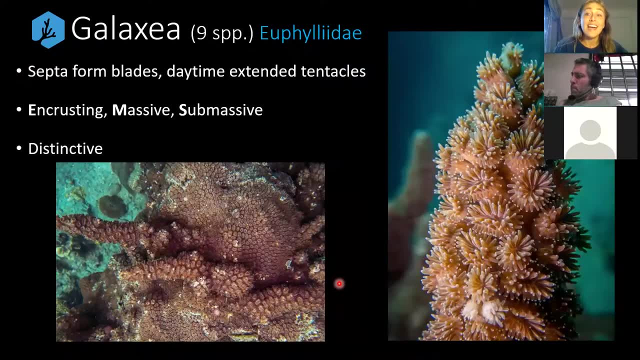 Whether it's yours or not. you can choose if you want to remember Euphyllia with the word association and with the euphoric as well. Up to you Now Galaxia, which is just one of the. this is such a cool coral guys. 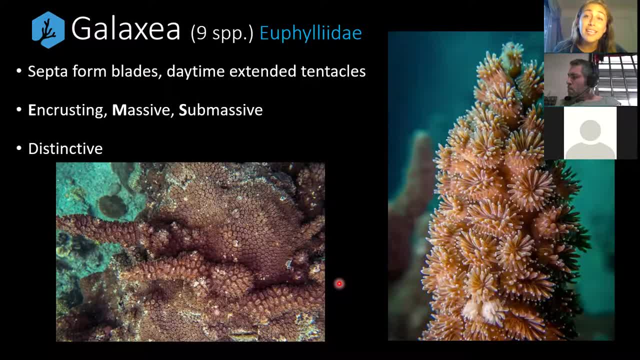 I really love it. We're still part of the Euphyllidae. We've still got daytime extended tentacles, but we've also got these blade-like scepter And it's a little bit hard sometimes to tell the difference between the scepter and the tentacles. 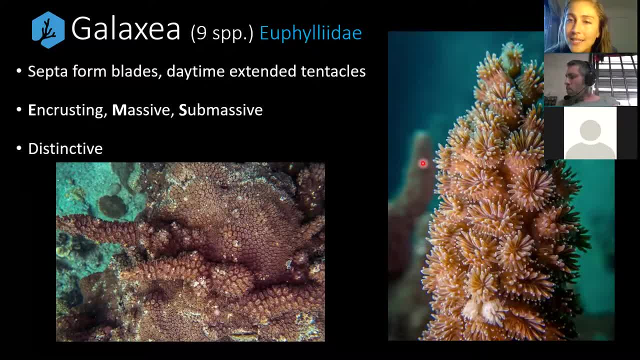 So if you'd like to glance over to the right side of the page, we can see these bits that are kind of sticking up a little bit more vertically. These are the blades, the scepter, which was that structural part of the skeleton, which. 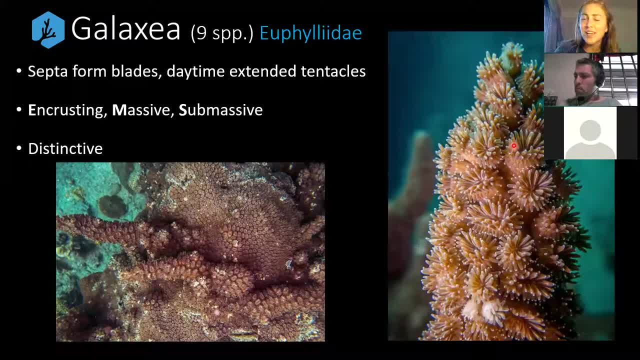 grows from the mouth to the wall. In this case it doesn't do that. It's just like ah scepter attack And it just protrudes out of the colony or out of the corallite completely, And they are very vertical. 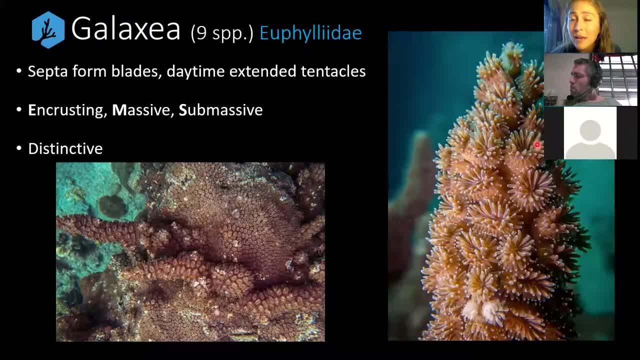 And the fact that they're covered in tissue makes them look very unalarming. But if there's a coral I would not recommend bumping into- not that we'd ever bump into corals, it would be this one, Because I assure you it would leave a mark. 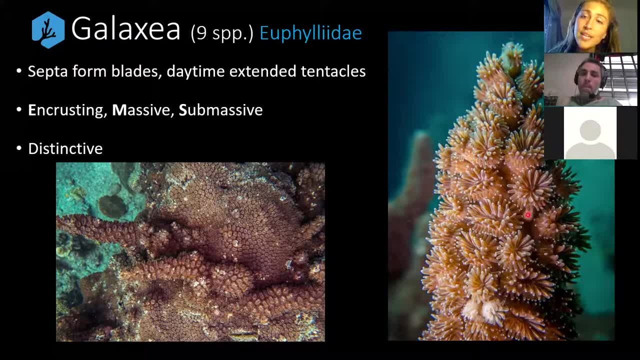 Anyhow, then we've got the beautiful tentacles. These are the corallites. So the corallites are these little, very short, very sharp, very thin. tiny little corallite. They're very, very short, very sharp, very thin. 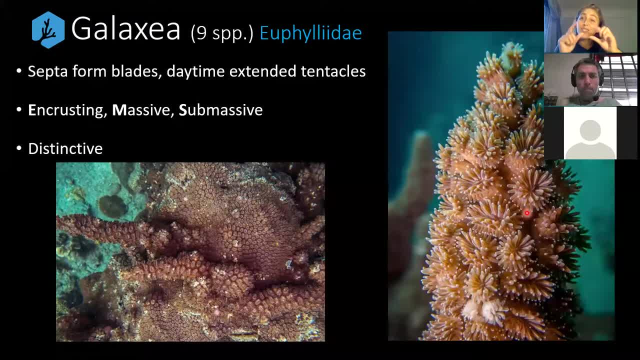 And they're very, very, very difficult to see. So I'll just go ahead and zoom out the sides here And, much like again, the other tentacles of the Uphilidae, at the very tips of each of these tentacles. 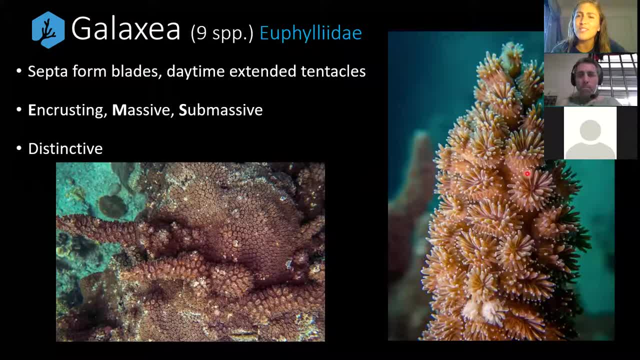 you get that little extra light coloration And especially because it's very short tentacles, they're very the glistening of these, the tips of all of these tentacles. I always thought it looked like a little glistening, you know. 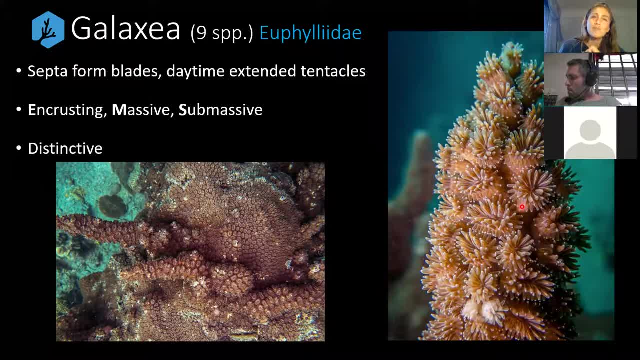 starry night, which leads us into our next new money device of a galaxia. you know being like the galaxy: a night sky, a nighttime sky, you know, glistening back at you with all these rushing around tentacles. 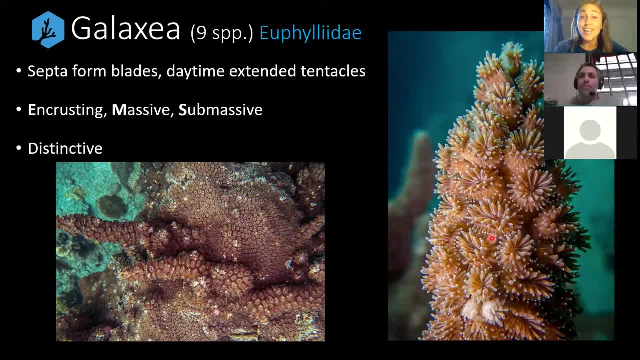 Okay, So hopefully you guys can appreciate this curl as much as I do. So Ethan, which is on this call somewhere. she just has the most wonderful photos of these curls and it makes me smile every time I see it on her Instagram, Coral Wraith Beauty. 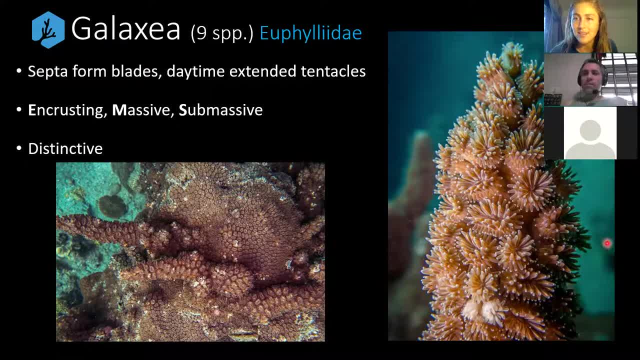 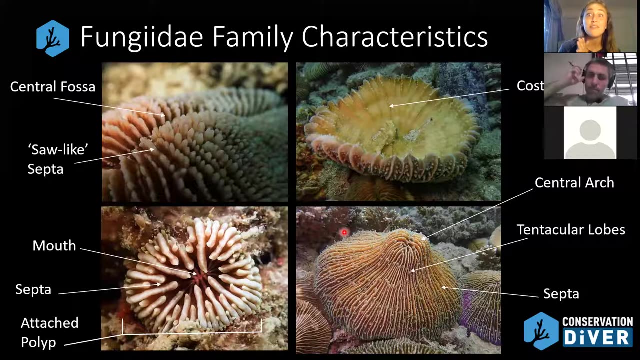 I think she's still around somewhere. I actually can't see everyone on the list to the right. I hope you're still there, Ethan, Maybe Anyhow. So it's a very distinctive coral colony And moving on. So let's talk about some of the fungidae family. 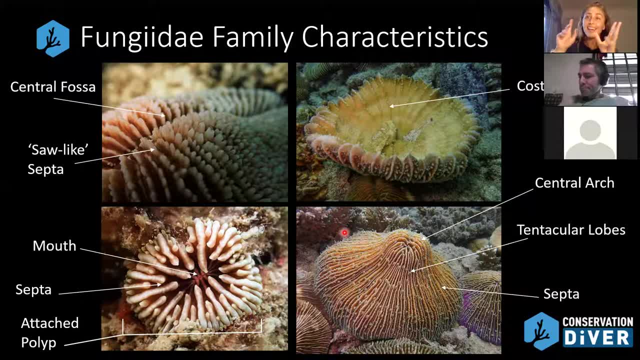 Otherwise known As the mushroom corals. The mushroom corals are very cool because they are, generally speaking, unattached individuals. You know, when we learn about the basics of corals, we usually learn: are you, they're colonial and they're sessile attached to a. 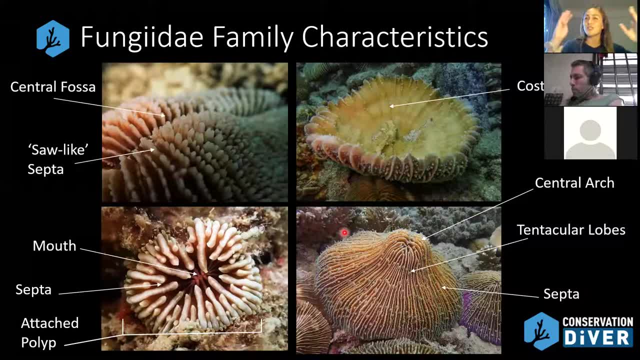 hard substrate on the reef floor And then they grow into these magnificent structures. and the fungidae family of corals just said Nope, we're not going to do any of that And, generally speaking, well, about half the time they're actually solitary. 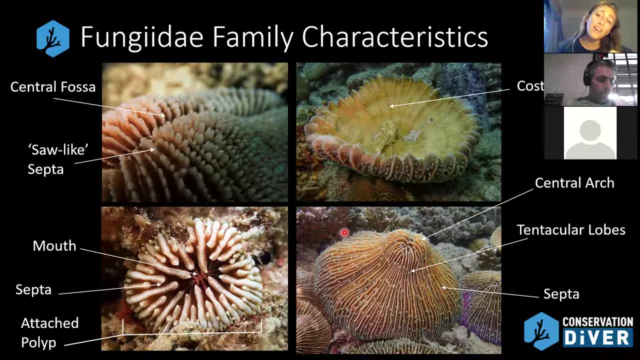 So they are a single polyp, Okay, And a lot of the time they also not attached. So the two large generalizations we often say about corals. these guys just didn't do that. So let's look at the structures here. 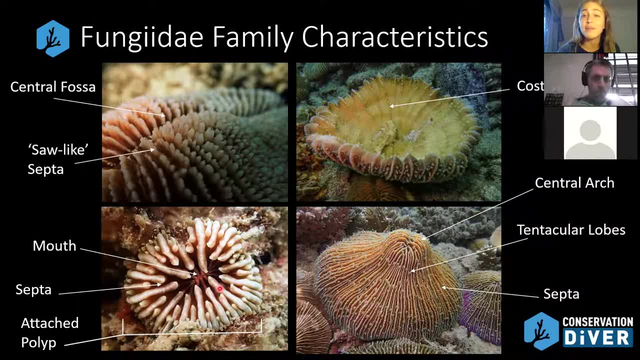 So these are a few different variety of fungids that we're going to be looking at. Here is one here up the top You got so you can see a bit of a slit there. That's its mouth. That's the center of the polyp. 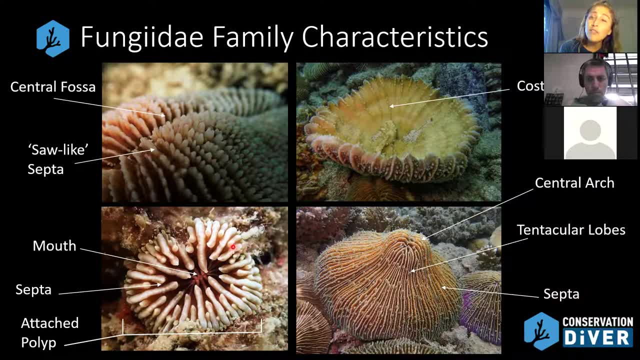 To our right we have a juvenile. All of them are attached when they're juveniles and then they'll detach, kind of looks like they've got a little belly button scar on the bottom sometimes, especially when they're still quite young, but you can see them out quite easily in this little one there and the scepter. 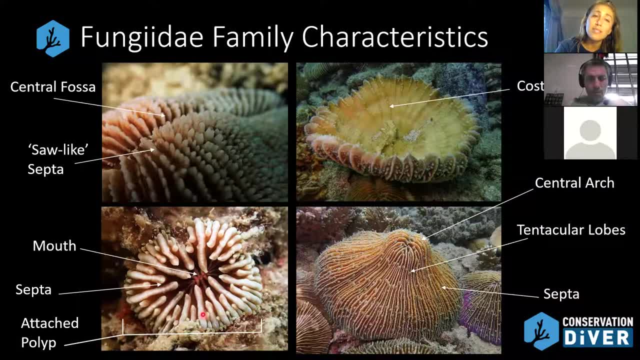 just like on all the other corals we've been looking at, these guys have got scepter. I used to be a little bit confused about the scepter. you know, the scepter are here, Sure, But where are the coste? 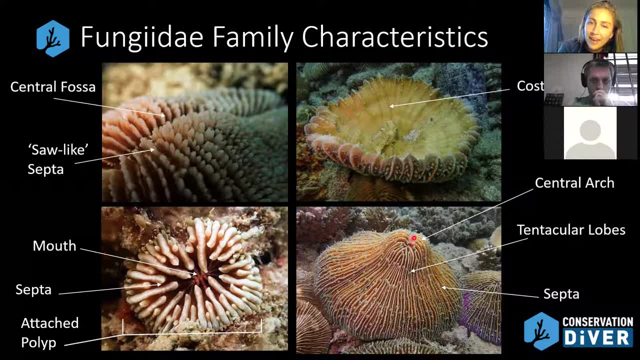 I nearly thought that it was like coming up from the mouth: You had a little bit of scepter. I thought it was like coming up from the mouth: You had a little bit of scepter. I thought it was like coming up from the mouth: You had a little bit of scepter. 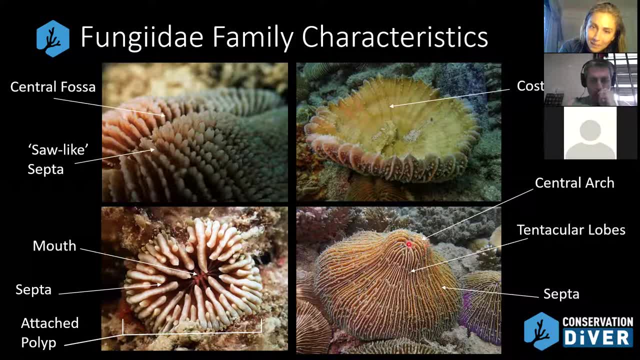 And then a lot of coste coming down the side. So coste, scepter. but that's actually not true. So what mushroom corals have is scepter. And then on the underside, if we go to this top photo, then it curves around and becomes the coste below. 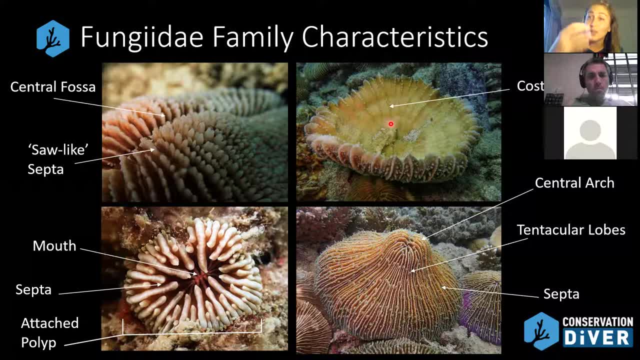 So you see these lines. this is very similar structures to those colonial corals that we were talking about before, but it's just. one side is the top with the scepter. The bottom side has the coste. Okay, We've got a lot of different types of scepter. 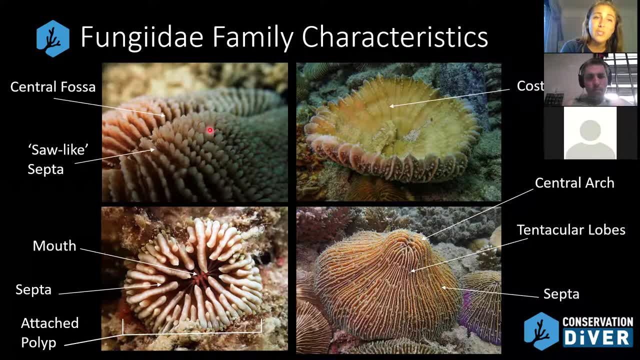 This is how we help identify some of the different mushroom corals. They can be quite sore, like they can be a bit smoother, but we'll get to it as we go. And they do have tentacles, only on the top half, which you can see in this photo just there. So let's jump into it. 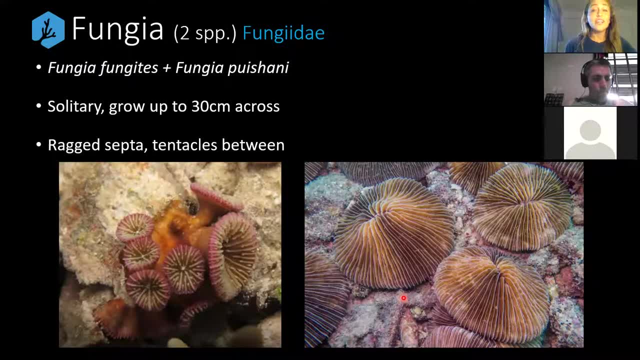 So first we've got the fungier genus. So fungier used to have over like a hundred species in it. Don't quote me on that, I don't know if it was a hundred, but it was a lot, A lot of species in it. And then they did all of this, you know. 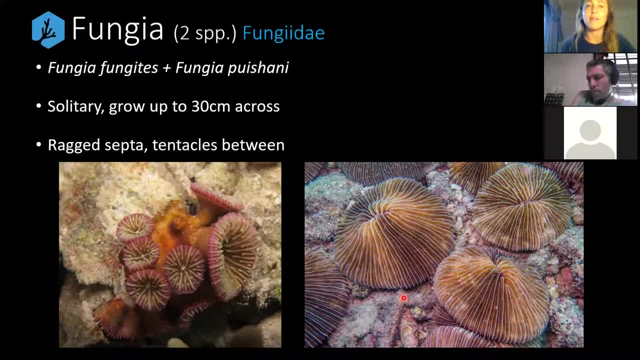 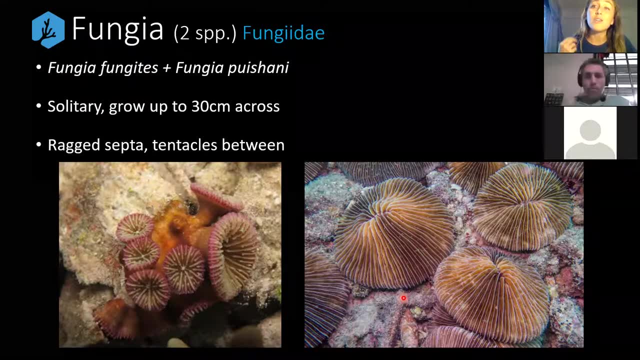 testing and they worked out that we were just quite wrong with that, that it wasn't all fungious. you know, genus with a few sub-genera. It's actually fungier is a genus that has got two species in it. I thought up until yesterday that I actually only had one species. 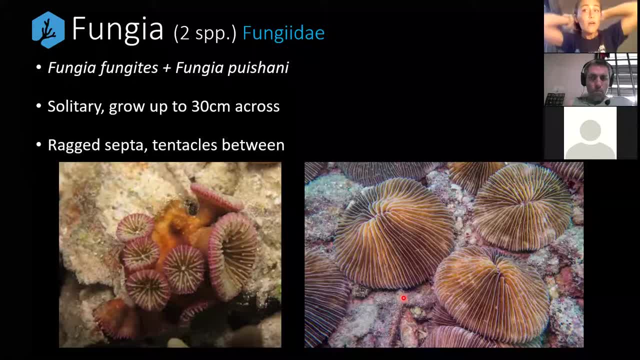 but I've now learned that there's two. Both of them only exist in the Indo-Pacific. Fungia fungidius exists pretty much all over the world, All over the Indo-Pacific, and fungier pushiani exists just on the west of the Indian ocean. 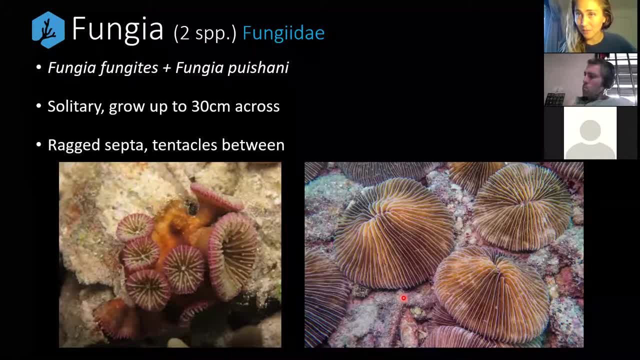 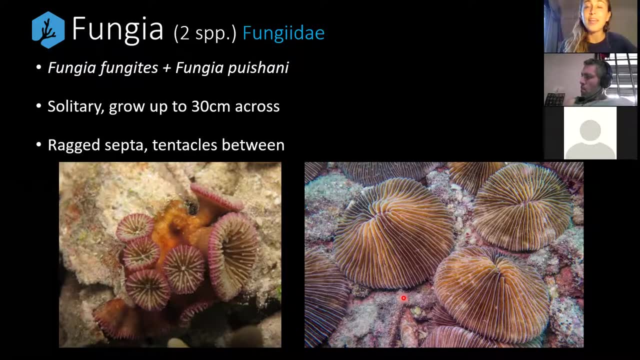 So, depending on where you are, you can forget that species name if you want to. Fungia fungidius is the much more frequenter of the Indo-Pacific in general. Just as a side note, I think this family is interesting when it comes to fungier fungidius. 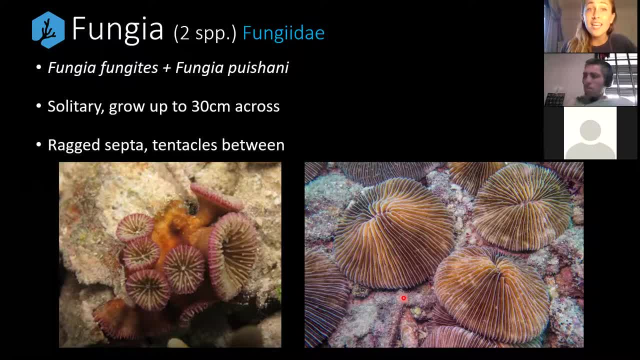 And when you say it, its family name is fungidae, genus name is fungier, Species name is fungidius and I just feel like that wasn't so creative And it's kind of a funny family name to species name combination. 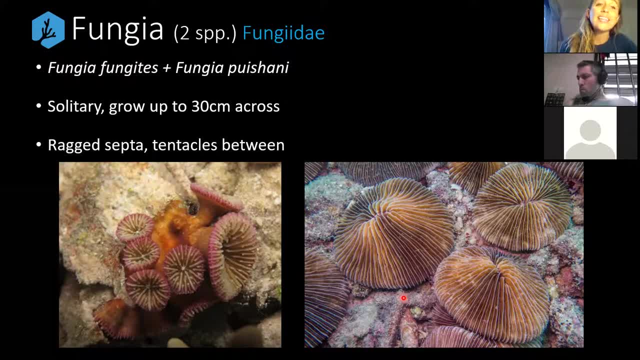 So anyways, so these guys are solitary and they grow up into these discs that end up being around 30 centimeters across at maximum. They have got rather ragged scepter. They don't have these sorts of saw like scepter that we just looked at before, but they are kind of kind of nearly quite sharp in nature. 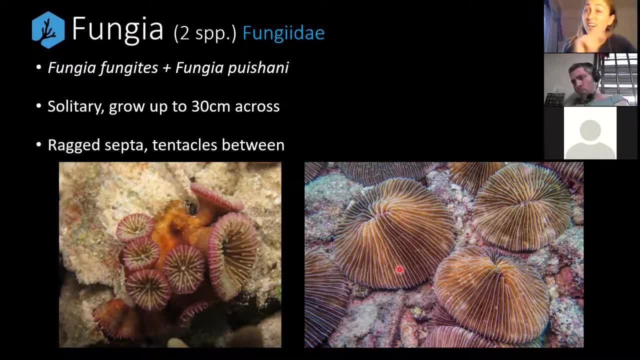 Like if you looked like if you're going to run your finger along, that you might, you know, cut it a little bit. This is how they look like when they're juveniles. You can see they've been crusted onto a rock here and there's quite a few juvenile individuals budding off there. 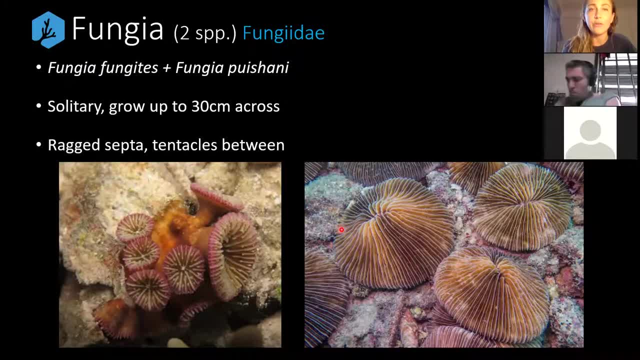 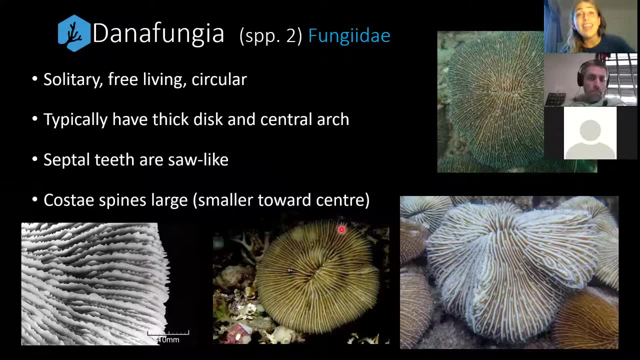 OK, and of course this is what they look like in their adult form. Then we've also got danafungia, So of all the mushroom corals, I think these two are probably the easiest to mix up. They've even got similar names. 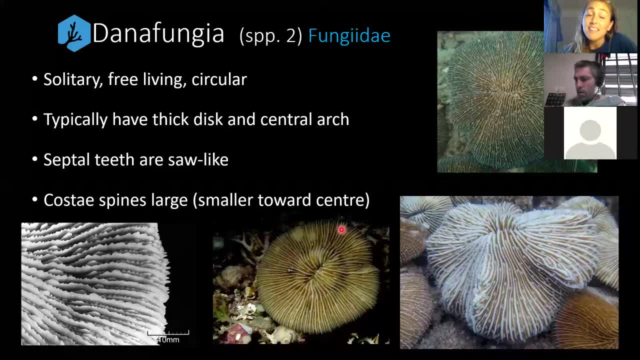 And some of the characteristics do overlap. OK, they both grow to be around that 30 centimeter mark. in terms of the diameter, They're both solitary and free living and circular Danafungia generally have a thick disc- I can find they can be a little bit thicker than the fungidae- and they can have a central arch. 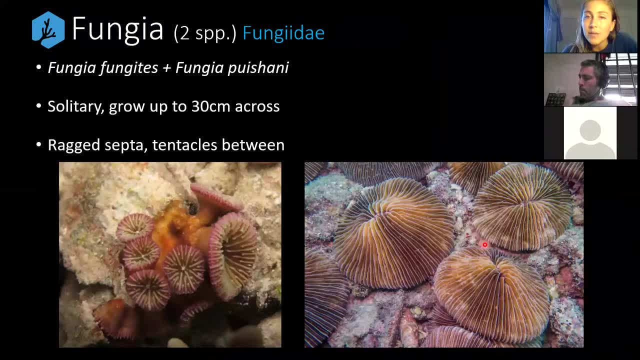 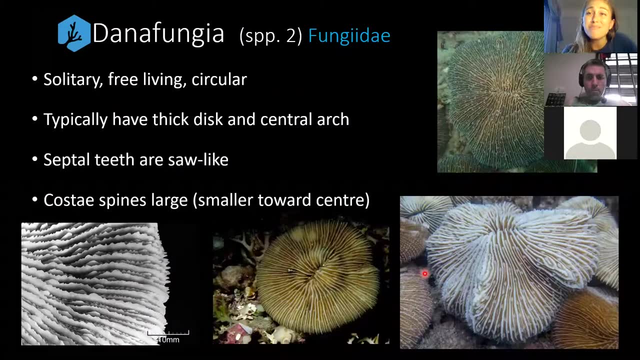 So it kind of goes up a little bit in the middle, just as we can actually see in here. This is the danafungia as well. This is actually a very nice example of that central arch, But all of them are not going to have it so distinctly either. 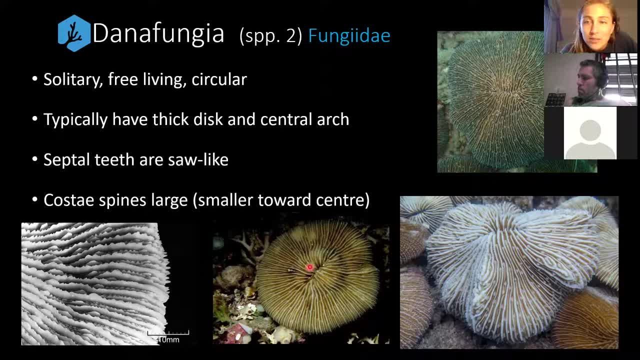 But the septal teeth are very saw-like, as you can sort of see across some of these photos, like in this part here. But we can see this black and white image that it's very. it kind of looks like an old, rusty saw that got thrown in the garage and you pull it out a few years later. 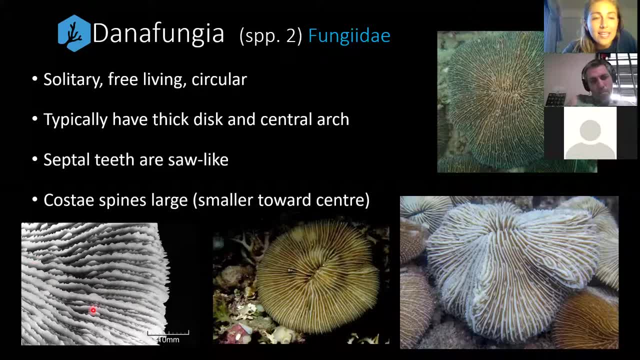 And it's a bit chipped and battered, but it's still, you know, an old saw blade. That's sort of what these guys look like. Additionally, the costae spines are large. especially on the edge, They're very, very tall and spiky, and they get smaller in the middle, much more distinctly so than the fungiae. 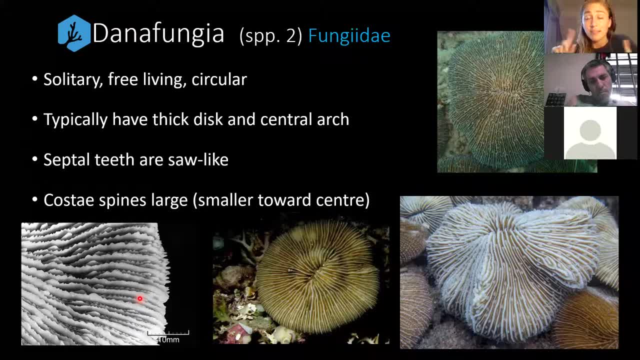 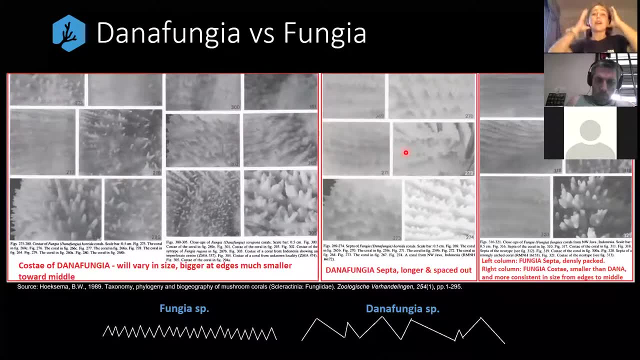 And me personally. that's how I tell them apart. I think the costae spines are the easiest place to spot it Cool. So this is obviously not our work right here. It's just from Hosama, an awesome guy when it comes to everything. mushroom corals. 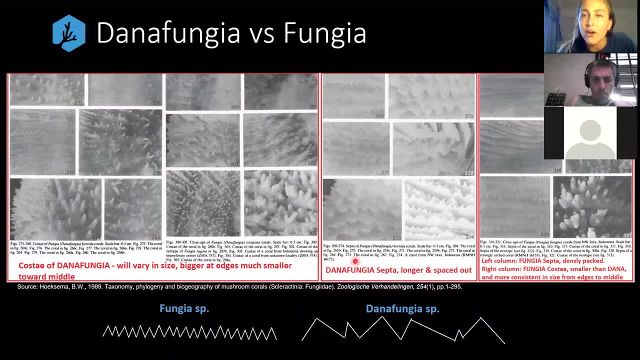 I'd like you guys to just you know. you can look at this if you want to, but take a focus to the right hand side. I'm going to show you how to do this To the right hand side and we're going to look at the fungiae scepter versus the danafungiae scepter. 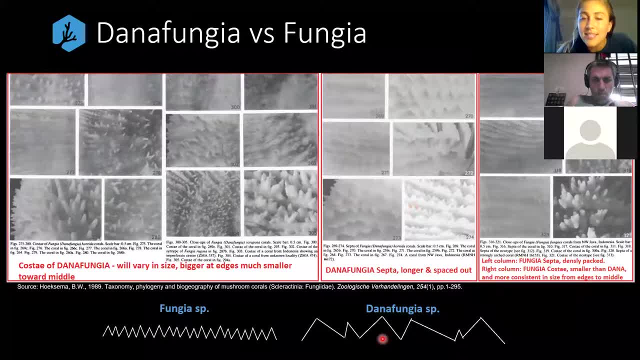 You can sort of see the difference there And you can look at my very artistic interpretation down the bottom here. Fungiae are quite uniform And they're quite, you know, uniformly ragged and even all the way along, as you guys can see here. 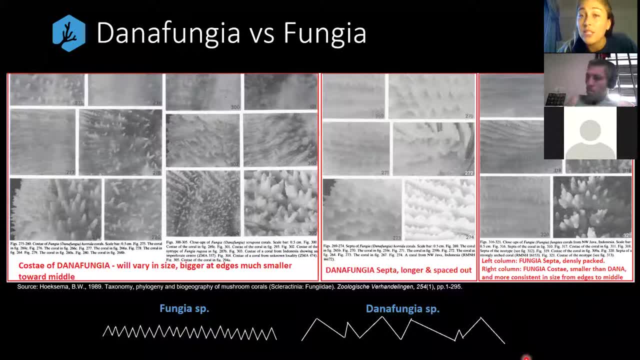 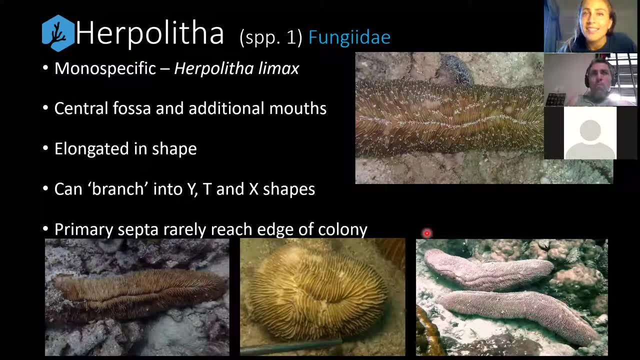 And the danafungiae are sort of all over the place, Again looking kind of like rusty old saw that might be a little bit broken as we can see along here. All right, so second monospecific genus of the lesson, Herpalitha. 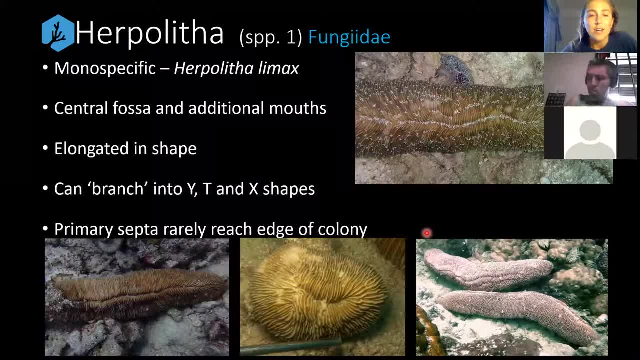 So Herpalitha sounds like herpy. You can use your imagination to work out a mnemonic device for that if you so wish. I did, and that's all I'll say Anyhow. so the species name is Limax, so Herpalitha, limax. here it's quite a cool, unique mushroom coral. 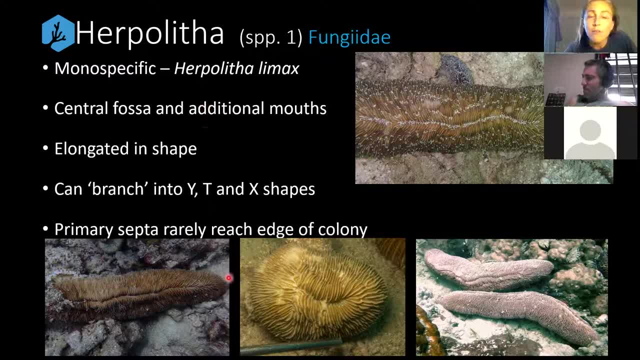 It's very long and extended And the edges have a bit more of a point to them. you know, compared to our danafungiae and fungiae that we just looked at, they are very nice and circular. Not all of them are circular. we'll look at some other ones in a moment, but this is probably. well, this is certainly the longest, skinniest and pointiest of this group of animals. 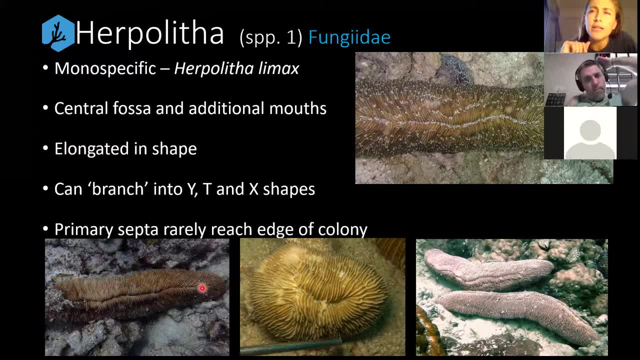 We have got a long central fossa which I just realized. I don't think I explained before. fossa on a mushroom coral is the same way it's describing a mouth, essentially. Interestingly enough, Herpalitha is colonial, so it's not a single polyp like our danafungiae and fungias. 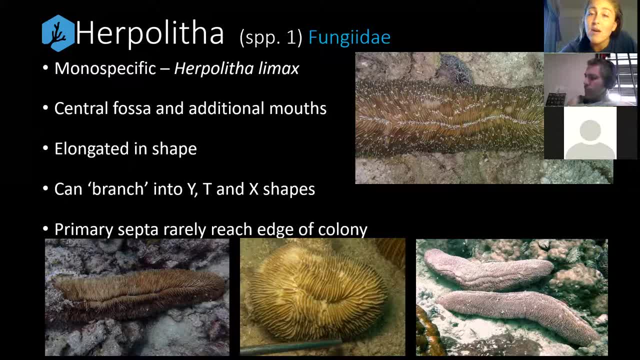 So we have a long central mouth fossa, as we can see on this photo at the top, and all these little white specks that we can see are actually tentacles. And if there's tentacles, that means there's a little mouth there that they're feeding. 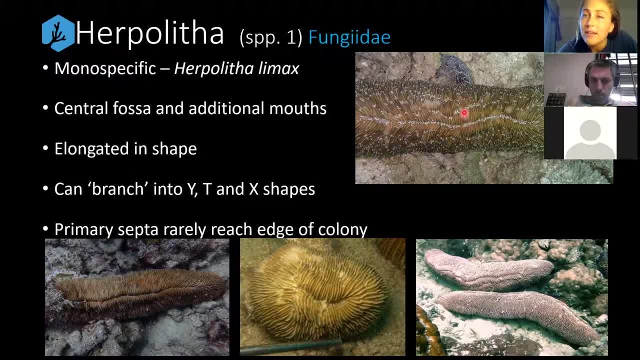 So they've got these nice septa that started the fossa, starting at the central fossa, And they don't usually make it all the way out, it all the way down the edge without meeting at least one or two other mouths. okay, they're also. 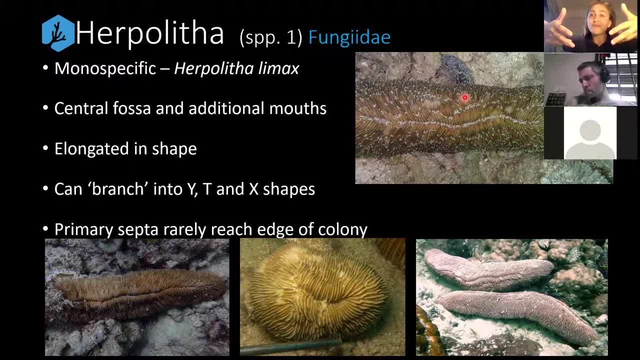 quite hollow below. so if you were to flip this over, you would see it's nearly like it would make a lovely long bowl you could like drink water from or store something in. um, i don't have any photos that right yet. um, by the way, if you guys want any more specific examples about any of these corals, 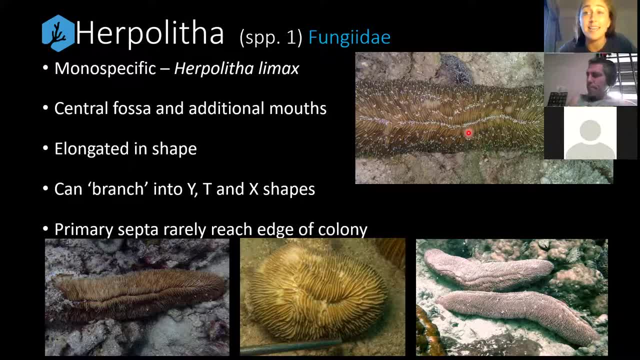 um, i've got a whole personal database on my computer. i can show you guys after. um, i know that i'm not working from home, so they might be in this direction as well- and what i do is i'm going to show you guys on the app, which is a really nice. 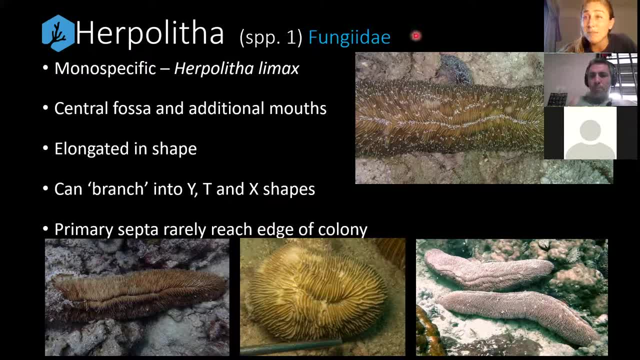 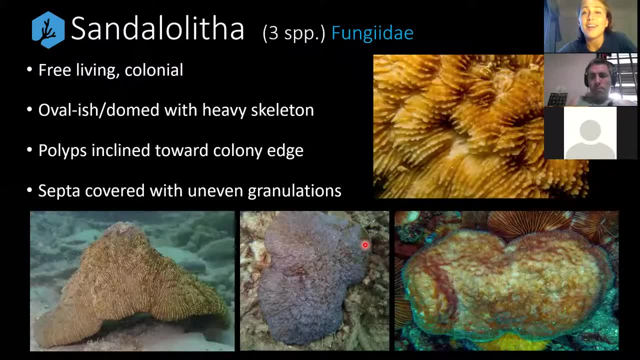 um, fun way to surf the netter. so if you guys want to see what i'm up to with the corals, um, it's a really fun way to surf the netter. so i'm going to show you something. i'm going to show you in this video on the netter, which is a really nice way for you guys to surf. 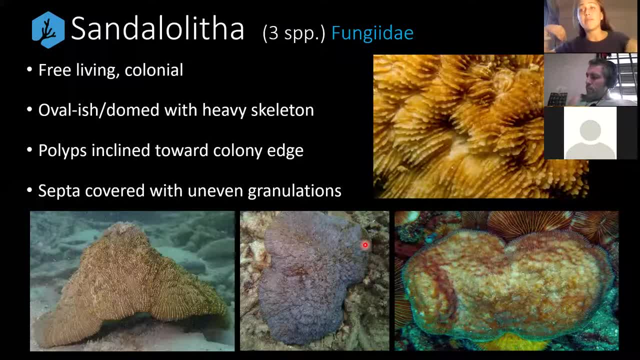 the netter um, and it's much more fun to see how it's done. so, yeah, so that's it for this video and i hope you guys liked that and i hope you guys found this video helpful and now you can let me know in the comments what you're going to want to see in the next video. okay, so you. 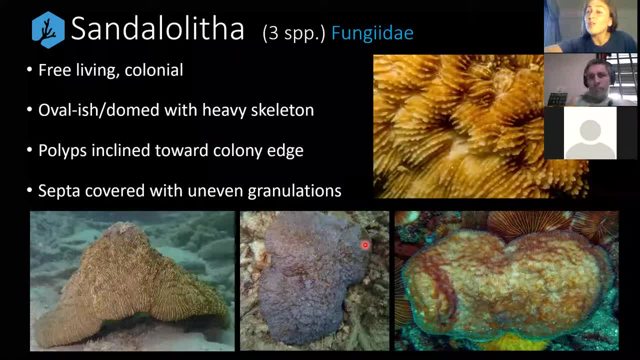 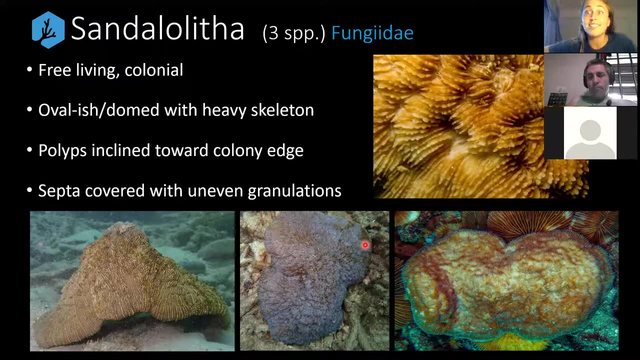 highland we'd just gone from referring to all of the mushroom corals as fungi to referring to them all as their now more correct names, and i remember one of the interns at the time- tia, she's so lovely. she rocked up to me and said: l i have the best mnemonic device for this coral. she said, and i 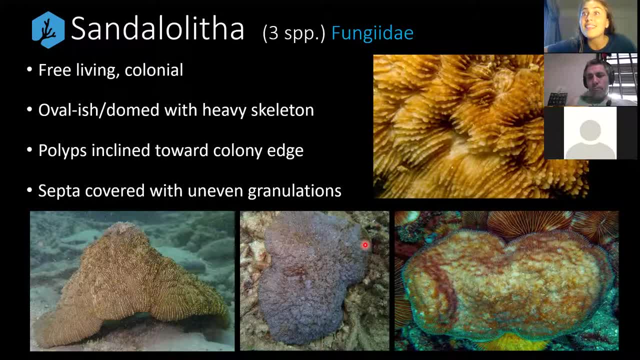 said: all right, amazing, give it to me. she said: sandal, aletha, sounds like sandal and wearing this coral on your foot as a sandal would be so uncomfortable. i was laughing so much. i was like dude, to be honest, like if you put any coral on your foot, that's not going to be that nice, i don't think. 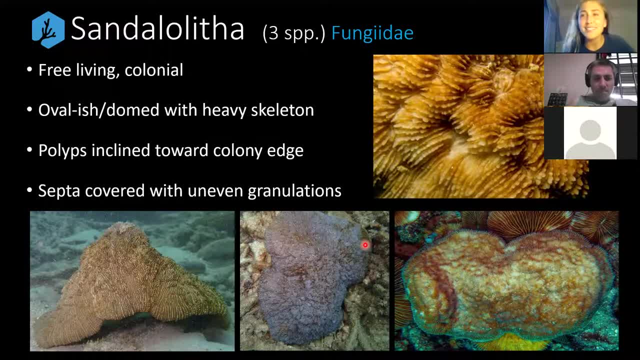 for the coral or for your foot. you know they've got ragged scepter and they're pointy and they've got stinging tentacles. but i thought that was kind of funny and i remembered it. so i think they kind of look somewhere between like a lumpy figure eight and a witch's hat. 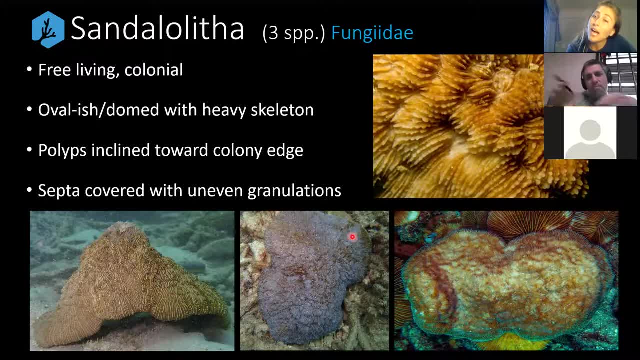 they are also colonial. they do not have a central fossa like the herpalitha okay. so they've got many, many different mouths and they actually take a thamnasteroid colony formation. so if you remember that bifacial color we were talking about earlier called pavona, which can grow in vertical or more, 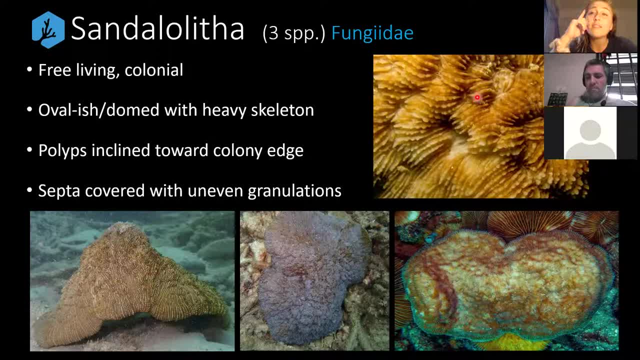 horizontal, depending on its exposure to sunlight. this has got the same colony formation as that one. sorry, the scepter just continuing. there are no distinctions or distinct walls there at all. um, the polyps are inclined towards colony edge pretty much. what i mean by that is that the scepter run towards the edge. they don't run parallel to the edge or anything. 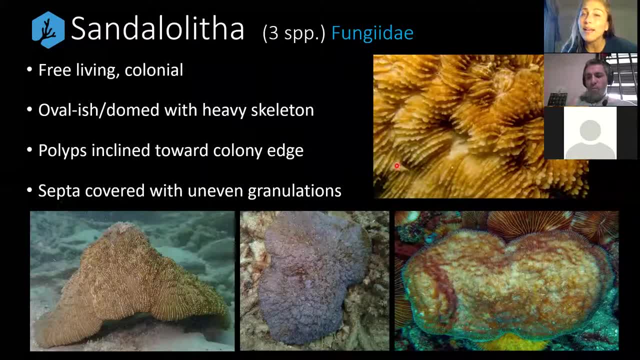 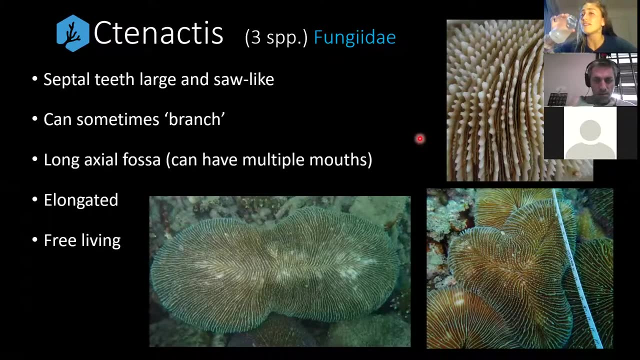 like that, and the scepter are also covered with uneven graduations, so it's nearly like they're a little bit, you know, bumpy or sore, like as we can see in this photo right there, and there's three species in this genus. is everyone doing good still? any questions or problems understanding? 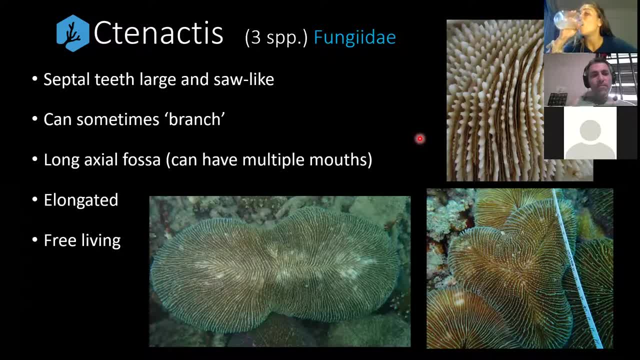 my accent or anything like that. cool thumbs up, awesome. i'll just continue for now. so then we've got tenactus, which i used to say synactus, which is wrong, but also it's latin, so there's not that many people who are going to go up and correct you. i suppose you've got three species within. 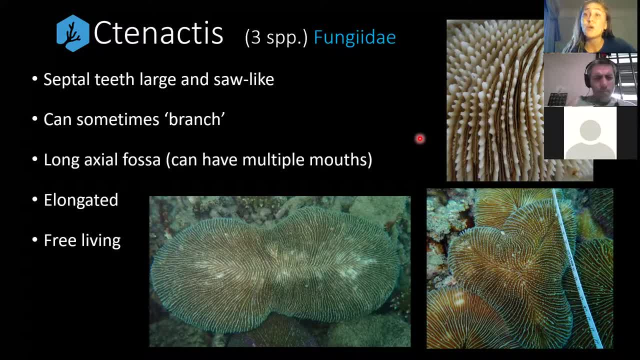 this genus it's got very nice large sore like septal teeth, as we can see right here, and we're quite a large mushroom coral. they easily breach, you know, the 30 or 40 centimeter mark. no worries, they are generally got a single mouth, but sometimes in this genus i have noticed you. 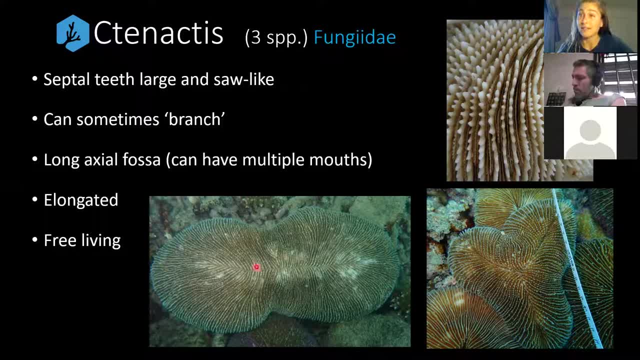 might get a break and you might have two, sometimes even three mounds there. and some of the other mushroom corals can do this too- that are more typically just got the one central long fossa okay. occasionally they branch, making that sort of x or y shape, as we can see in this example in the 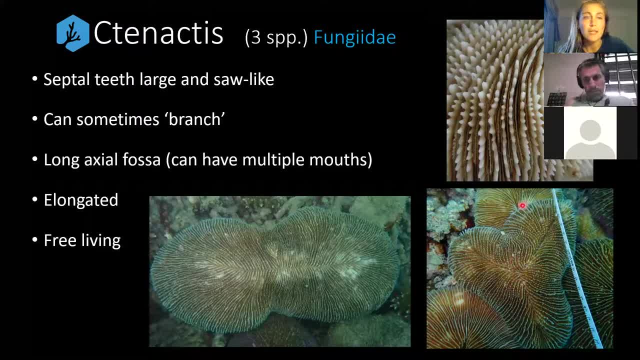 five bottom right corner sort of like, is a, is a y shape here. um, they're elongated and, of course, they're free living as well. yeah and um, i've got a bad mnemonic device to that, one that i just forced myself to think up. you can refer to the pdf if you want it, but i'd more highly recommend you. 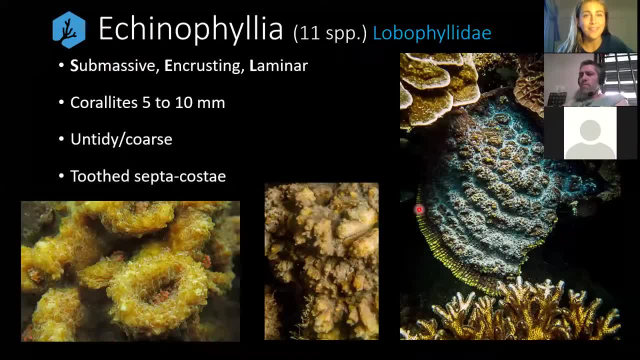 think of one yourself, which is better than mine. okay, so now we're moving on to the lobophila day. we're done with the fungidae family. if you guys hadn't noticed, we're going through all the families in alphabetical order. so echinophilia. 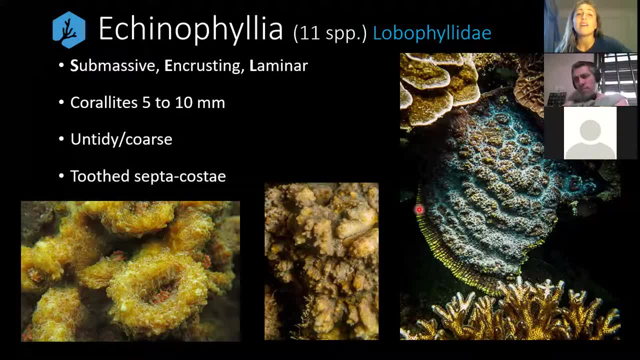 has got 11 species. okay, we wrote: well, they grow, we grow it. they grow in a submassive growth form, sometimes in crusting and also sometimes lamina. as we can see in this photo right here, the corallites are quite large, five to ten millimeters. it's not large when they get into that 10 millimeter size. 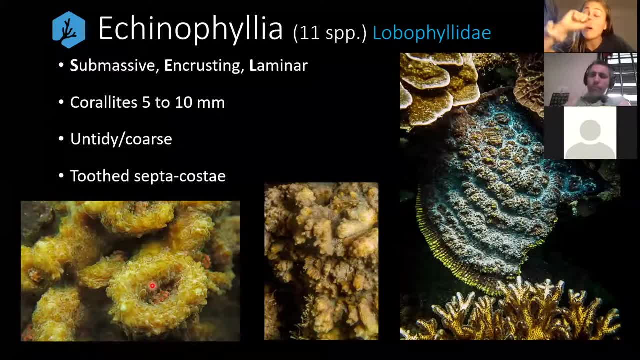 and they've got large, uneven scepter again going from the corallite mouth up into the wall. it's very bumpy and they're also very toothed, as we can sort of see across all of these photos. i think echinophilia- me coming from australia- we've got these animals called echidnas, which 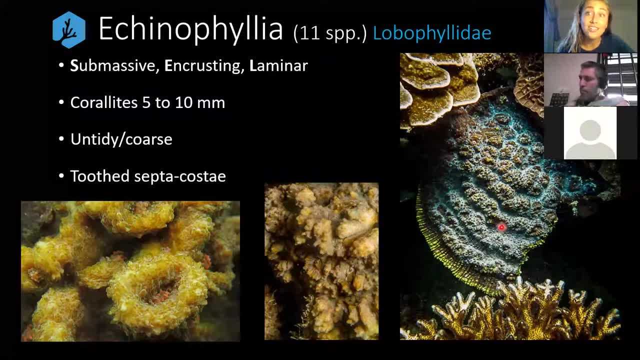 are kind of like the australian versions of what are? they hedgehogs, and because these are bumpy and spiky and small and round, i think that reminds me of an echidna slightly in my crazy stretch of the imagination. then i just made the little connection with echino and echidna. so 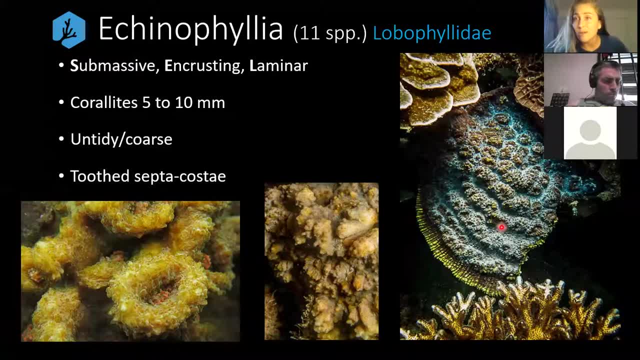 echinophilia, a little bit like an echidna, and that's what got me to remembering that one. in the end, after i wrote down the word echinophilia about 20 times or so, sort of glued it in there. all right, then we've also got lobophilia. 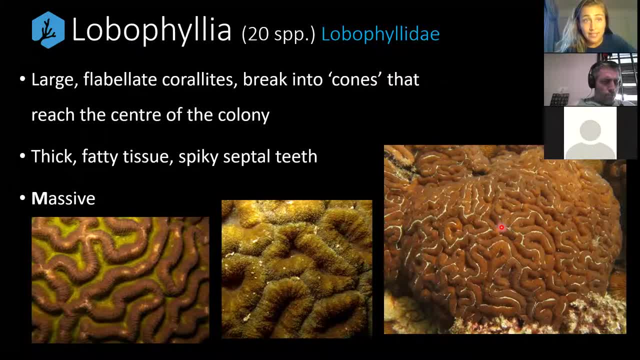 so this is from the lobophilia family. still, lobophilia is pretty common around the indo-pacific. often it's described as large brain corals. i'm sure you guys can understand why think of lobophilia as a brain. you know your lobes and your brain got you know loby in in shape, i suppose. 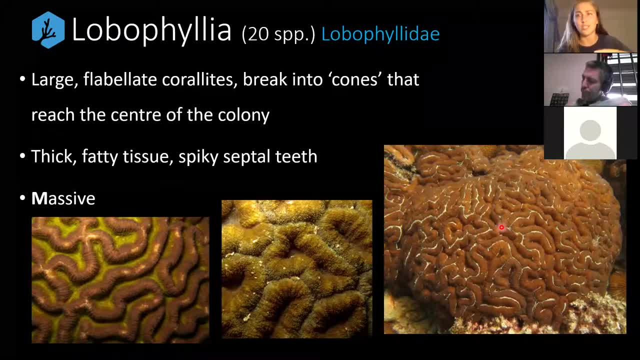 how we describe it. so it's kind of pretty easy to make that association to lobophilia: large flab like corallites. they break into cones that reach the center of the colony. so not that you would, but if you're to crack one of his colonies down the middle, you see like these sort of cone-like structures. you know the big. 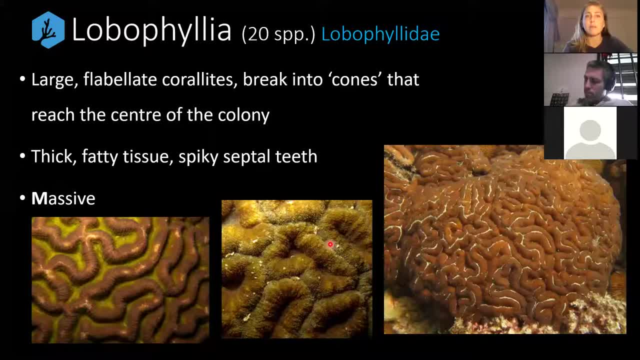 kind of lobes here will just get thinner and thinner, like an ice cream cone. um, they've got very thick, fatty tissue. if you ever did see a dead one, you would notice that the septal teeth are very spiky and sharp. but you're not going to notice that unless the tissue is gone and they do. 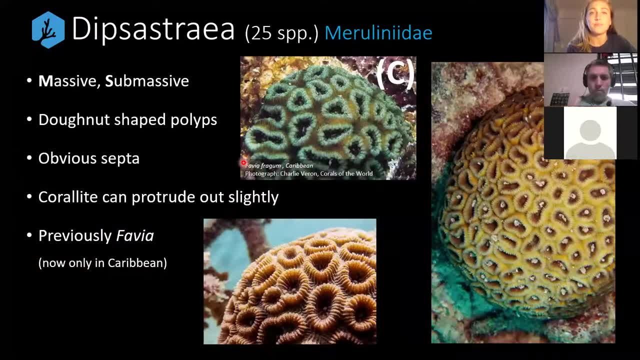 grow in these massive curved growth forms. so now we've got dip sastria, which is just it's new, it's relatively new. you guys might notice down here that i've got a c plugged on this photo. so dip sastria is within the last few years. 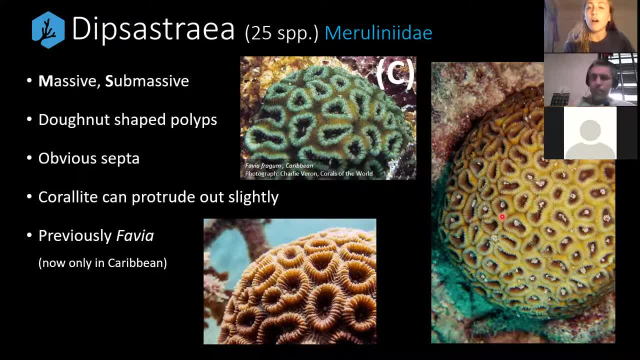 new to what we call these sort of donut, like corals in the indo-pacific. okay, we used to call them bavia and we also used to think that, like a lot of these sort of circular corallided, you know, looks like little donut, like corals with fabia in the indo-pacific. 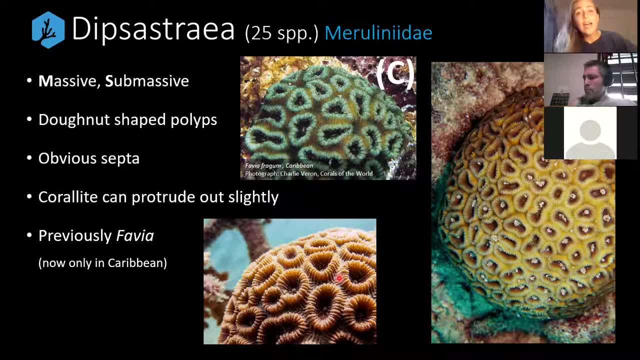 but we were wrong. okay, it's sort of been reclassified now. it only exists in the caribbean. this is a fabia phragm. this is not my photo, it's just um sourced down the bottom there. they are found in the caribbean and it's been also realized that they are not actually at all related to the. 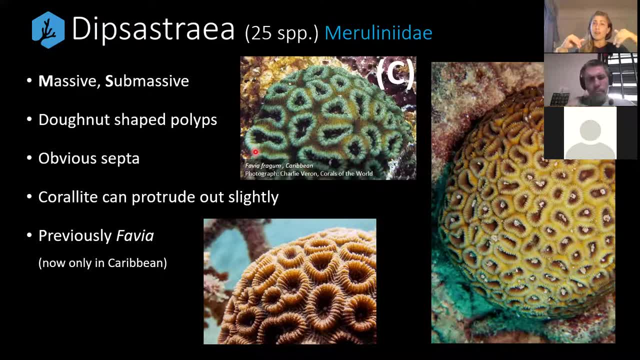 corals in the indo-pacific, even though their morphology is very similar. i mean, as you guys can see in these photos, they're not actually related to the corals in the indo-pacific. i mean, they do have some quite clear um characteristics that look um quite like each. 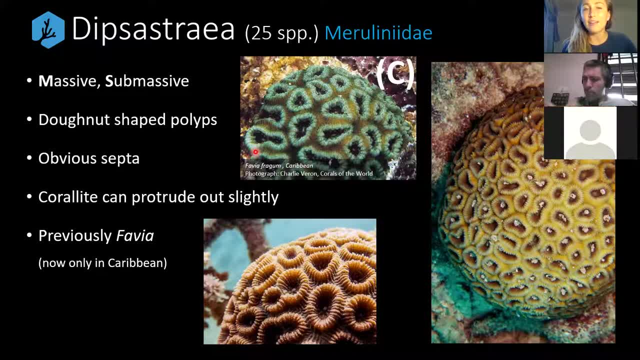 other. so i used to love saying fabia was my favorite donut, and that was how i remembered it, because it was a donut shaped coral. you can absolutely do that if you're in the caribbean, if you want to, but in the indo-pacific, please do remember that this is now called dip sastria. 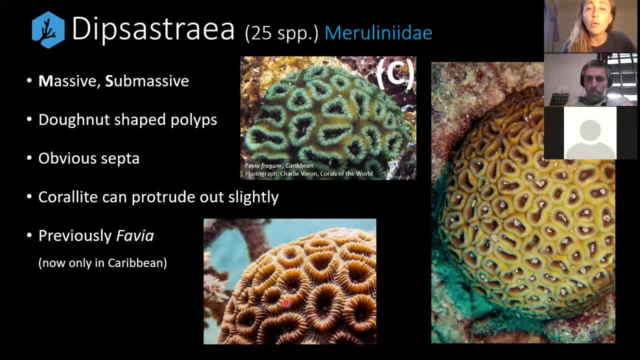 they grow as massive and submassive. they are usually quite nice circular donut shapes, but they have got this intra-tentacular budding, so occasionally you'll see these sort of figure eight shapes when they're pinching off to become more polyps or when they're growing more polyps. i should say okay. in this frame in particular, you can see 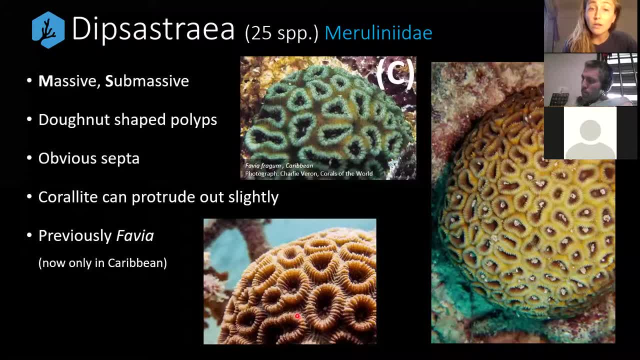 the obvious septa to costae area. it is not got a smooth synastrum. you can see that the costae run all the way down until they meet with those from the bordering um corallites. there, the corallites being the whole, you know, skeletal part of where the polyp sits, protrude out slightly. 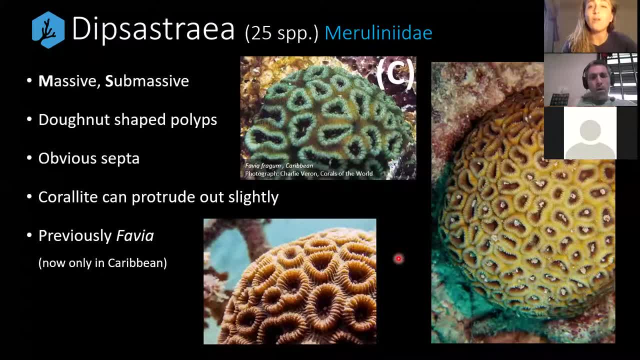 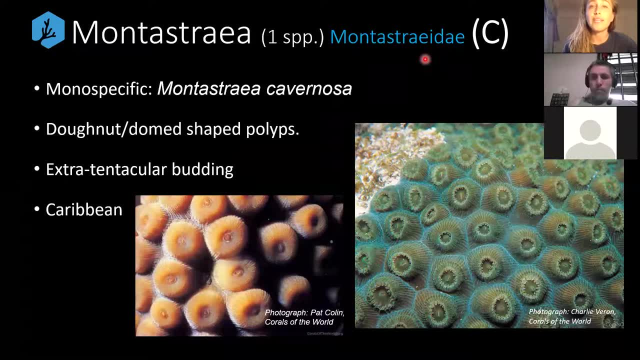 as you can see here. so also i forgot. we're in the marylander day now, which is another family name. great. so then we've got montastria. this is not in the indo-pacific. i just wanted to mention it because we used to again say that it was a coral in the pacific. it's not. it's actually. 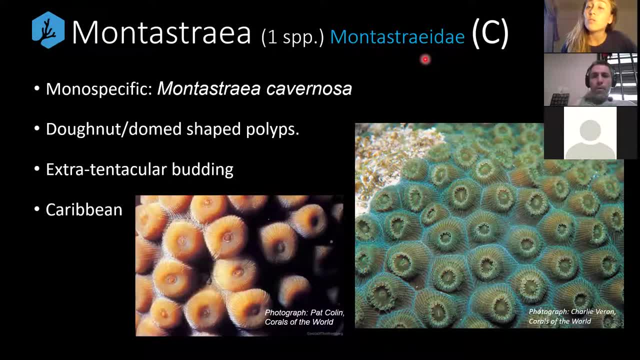 mono-specific. it is montastria cavernosa. it is one of the more commonly referred to corals of the caribbean waters. so, again, i wanted to include, even though this is a predominantly indo-pacific based lecture, that this is just one of those general species of note, uh, you know, of significance, um, if you guys did want to remember this, um, also. 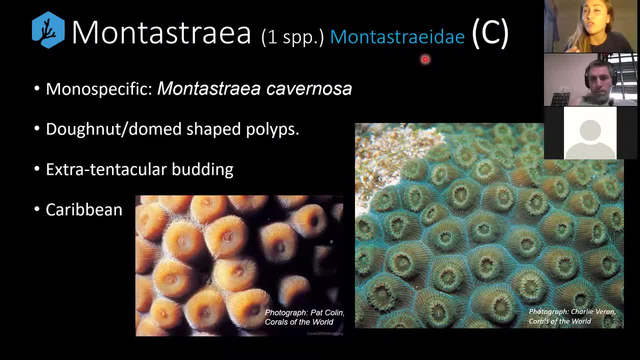 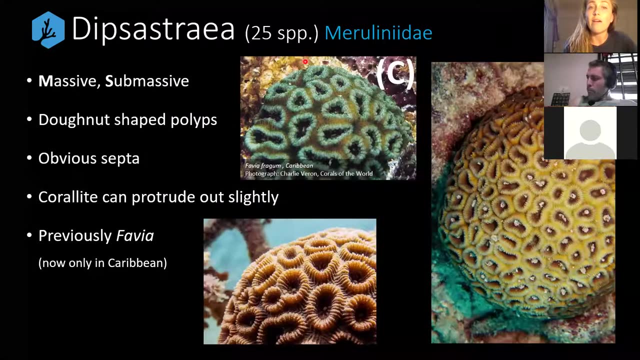 quite donut shaped. i think it looks somewhere between our dipsastria and our diploastria heliopora, which is the first mono-specific coral that we talked about in this lecture. this has also got extra tentacular budding, which makes it different to the fabia fragum. 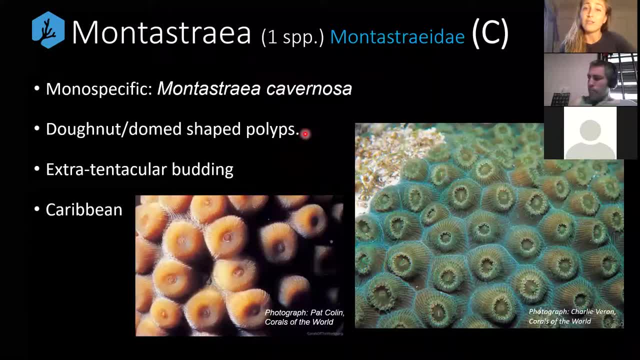 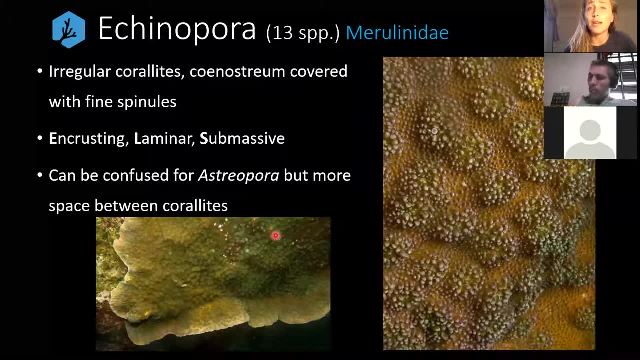 that is also found in the caribbean. that also has very circular sort of corallites there. all right, then we've got echinopora- also part of the marylander day- which has got irregular corallites. it's anastrium covered in fine spinules. so we've got spinules, we've got spicules. 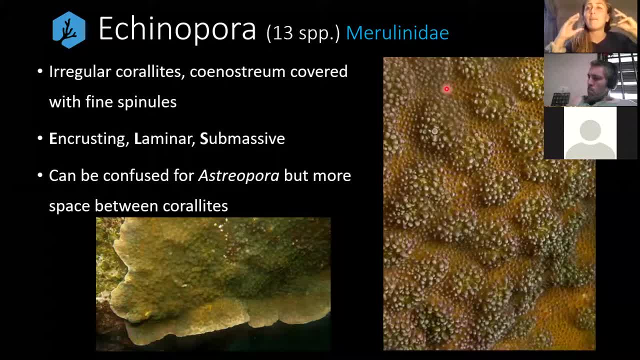 we've got monticules again. all just names. describe bumpy skeleton. if you want, you can just say: the skeleton is bumpy, that's totally fine. echinopora is the thing that we're aiming to remember today. they grow as encrusting, laminar and submassive. okay, these ones can be a little bit confused. 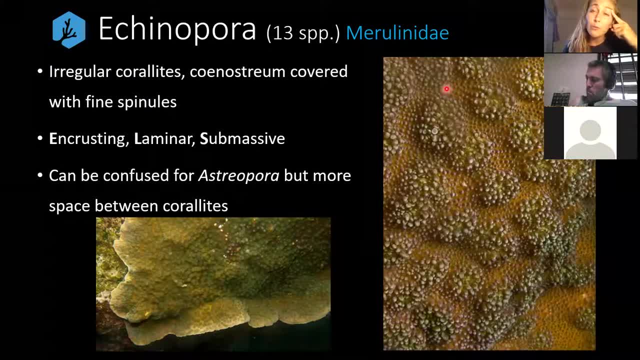 for astropora because if you remember, from the very beginning, from the acropora day family, acropora have also got that sort of scattered- you know, irregular corallides, good eyes scattered on the floor, kind of look to it. but astropora has a very dug out appearance in. 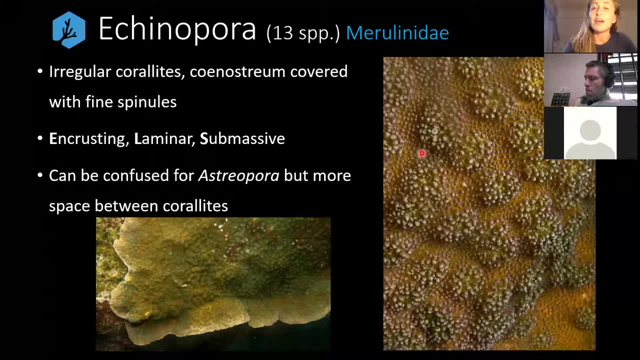 the center, whereas these guys do not. they've just got these nice bumps. i also think these are a little bit echidna-like- echinopora is the other echidna coral- these little mounds that just tuck themselves in and they put out their bumpy, spiky bark so that nothing is going to hurt them okay. 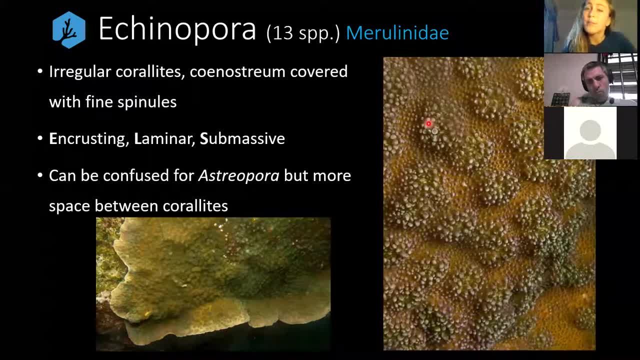 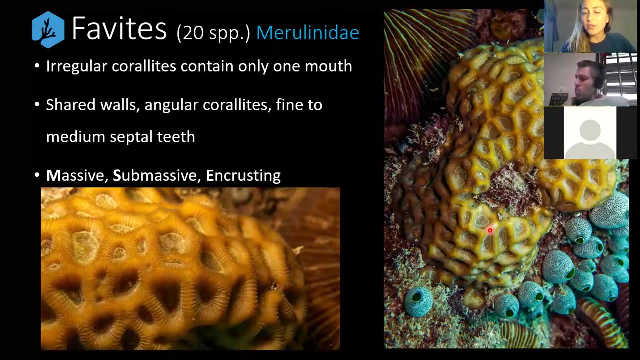 at least that's what echidnas do when they feel like they're being threatened. but again, irregular corallides, space in the middle and that space is bumpy sweet. so i just want to pre-warn you guys that the next few genera are a little bit tricky, but it's going to be okay, we're going to get. 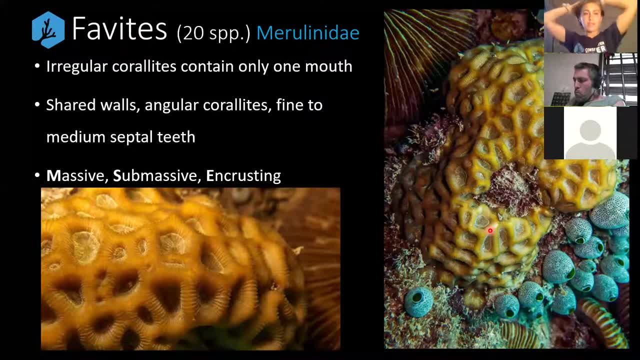 through it together. don't feel like you're going to have to remember all these on the first go, because no one ever does, except for some people, and let's be honest, i don't like those people, because this took me forever. um, we'll just dump, stride, drive striding, jump straight into it. so if i've got 20 species, it. 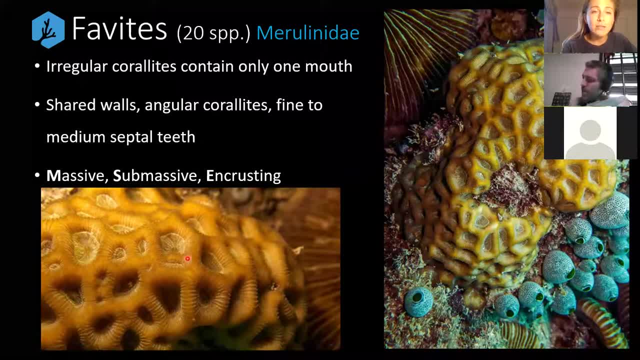 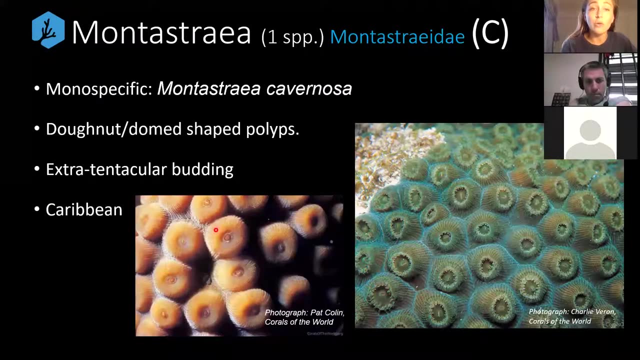 has irregularly shaped corallites. some of them look like little squares, some of them are triangles, some of them are ovals. so remember, favitis has got irregular corallites. we've got shared walls. they're not separate between corallite to corallite like in these guys here. that's its own wall. 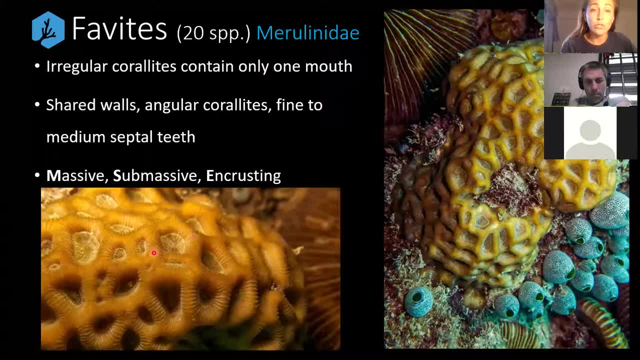 that's its own wall, whereas in this one it's just. the walls are shared between all of them. the correlates also very angular. from the top of the wall to where the mouth sits, it's on this nice, fine angle, okay, so that's another way to remember it. it's got medium sort of clean cut septal teeth. 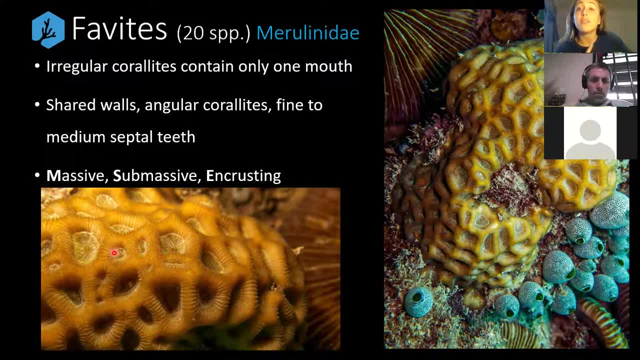 as well. they're quite neat and they grow as massive, sub-massive and encrusting. sometimes we get these cool color differences between the walls and so the base of the polyps. this is not that much, but you sometimes get like greens in the middle and yellow on the wall, and for me i always 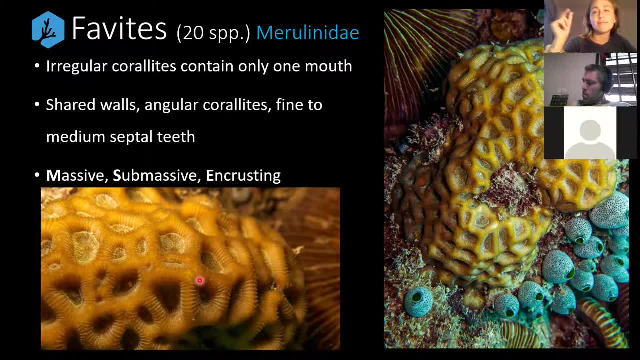 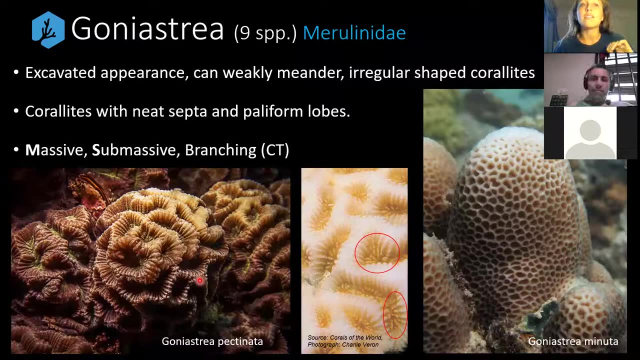 thought: wow, that's so pretty. for varieties is my favorite and again for body's favorite similar words, even though nowadays i've got about a hundred favorite corals anyhow. now we're going to talk about goniastria: nine species and it's got an excavated appearance. okay, quite dug out in. 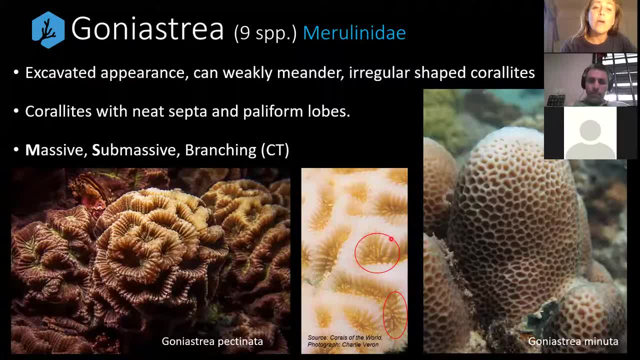 appearance. like you can see in this goniastria manata, it can weakly meander, so it nearly looks like it's trying to fully meander and become, you know, like the, you know not puzzle, like a maze, but it's sort of. 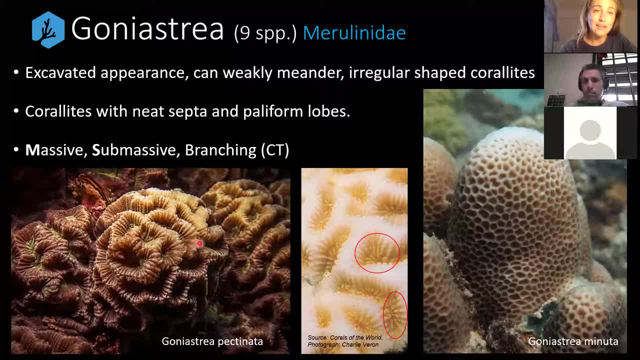 not quite getting there, as we can see in these photos down here. Okay, it's got irregular shaped corallites like Alphavitis, but they're much more dug out than Alphavitis. This is probably the nicer example. down here, The corallites got neat scepter And what I want you guys to remember, 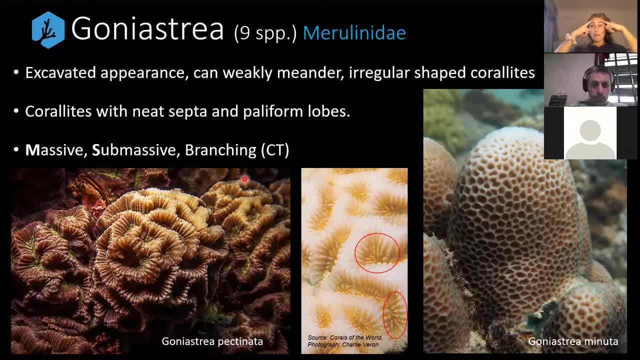 is that they've got paliform lobes. So if you remember from the beginning skeletal structure, I said paliform lobes. a lot of corals don't have them, but when they do, they're quite useful to remember that they do have, because they're often the distinguishing factor And this is 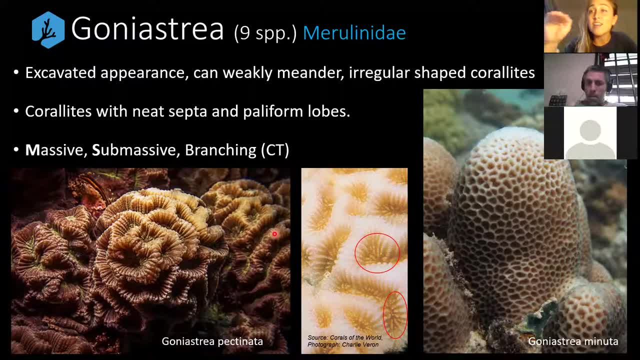 going to be a distinguishing factor for us. So it's kind of like the secondary wall or crown just before you get to the mouth of the corallite, As you guys can sort of see here. you've got the wall, it dips down and then there's like this is a secondary wall and then you've got the mouth. 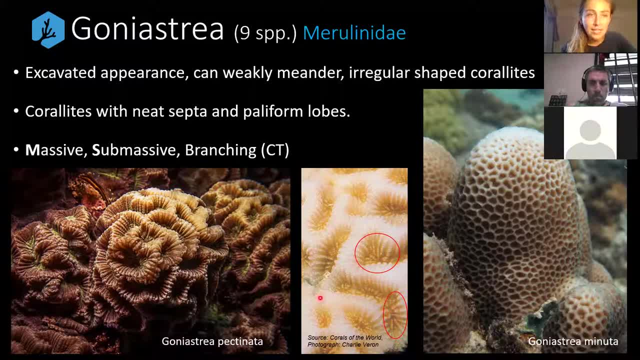 down there in the middle, in the bottom, okay, And you can sort of see them along here as well. So paliform lobes are going along with Goniastria. Goniastria sounds like gonads. When we do coral spawning work, we would often. 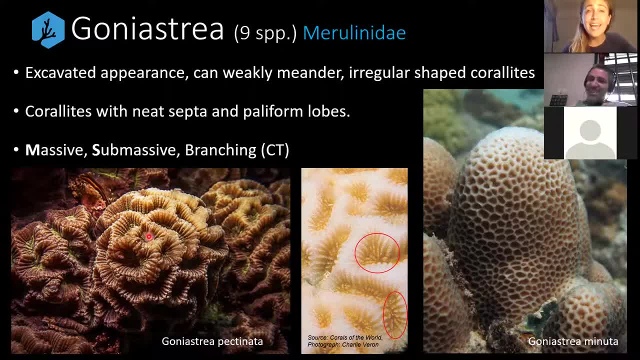 work with Goniastria a lot because they're quite a resilient species. So it'd be sort of on our priorities list and we'd play with their gonads. No, Well, sure Say that. if it's going to just think of it like that, sure These guys grow as massive, submassive and branching as well. 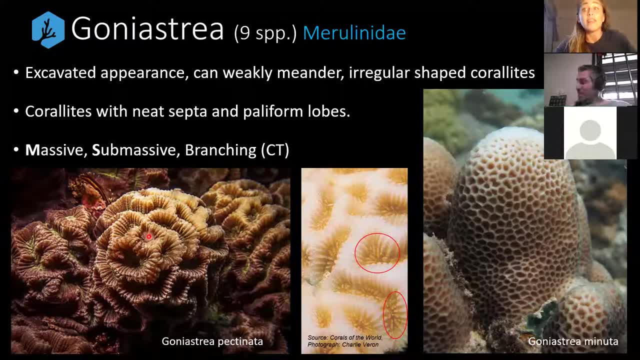 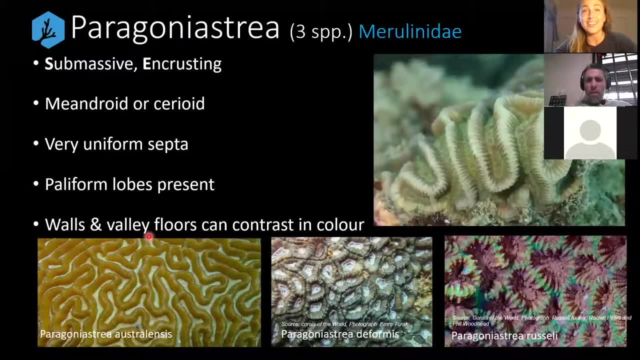 in very specific examples: Deep breath, And then we've got Paragoniastria. So I've got Garoniastria and then we've got Paragoniastria, And one that I really quite like is called Paragoniastria australensis. It used to be chucked in with the Goniastria genus. 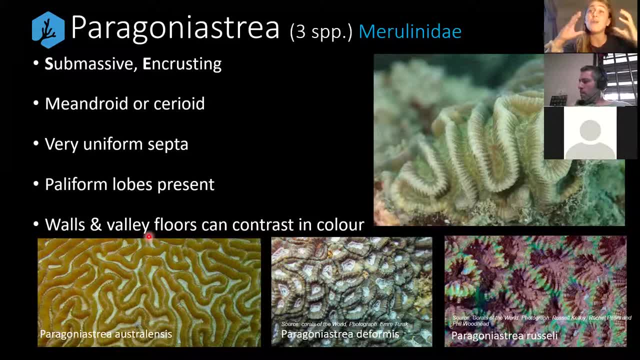 and then scientists were like, no, that's wrong, Actually it's got to go in their own genus called Paragoniastria, And so they did that. There are three species, and here's an example of all of them. One is full-on meandering baby, and look at that. It's like a crazy maze. that is just. 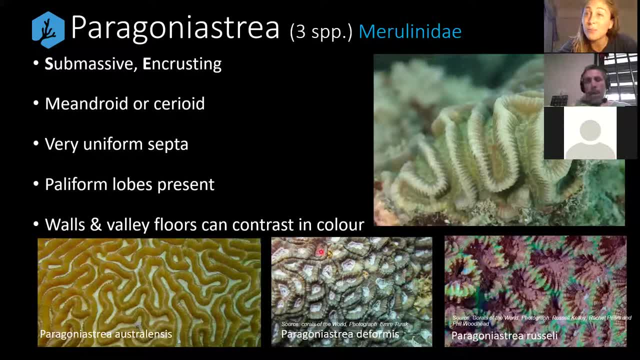 inescapable. And then we've got some that are just sort of your typical, more circular, round corallites, as you can see here: Roselli Deformis and Australensis- That's my favorite one, Submassive and encrusting. they are meanderoid or steroid. They've got quite uniform at scepter. 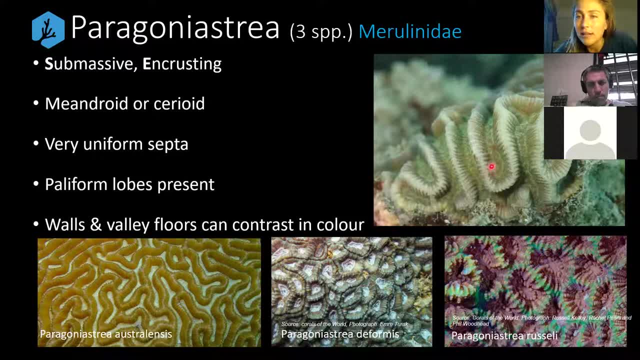 especially the Australensis. Look at those. Look how neat they are. I love it. They've also got polyform lobes present, but I think they're more present in the Deformis and the Roselli- just personally speaking from me looking for them, you know, amongst corals and so on and forth. 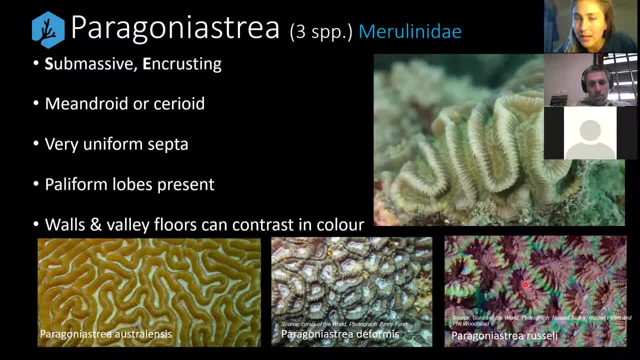 They're quite obvious, especially like where I'm putting my cursor right now. There it's like boom. here's my, Here's my mouth crown, Here's my polyform lobe, And then we go, Also the walls and valley floors. 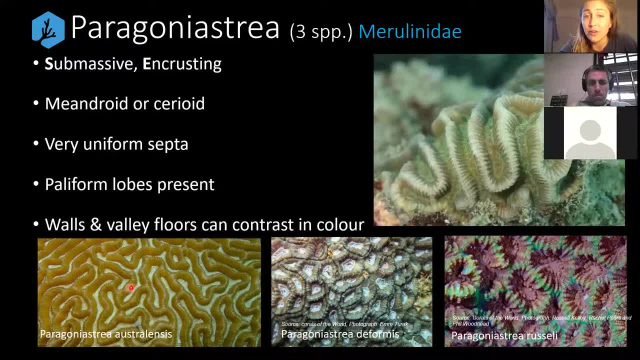 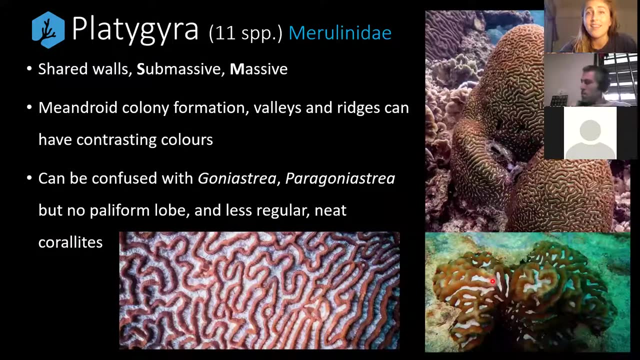 can contrast in color, just like in literally all these photos. You've got like brownish to the green, You've got the kind of blue to the Blue-green to the white, You've got the green to the pink. So they're aesthetic at least, even though they're a tricky genus. And then we've 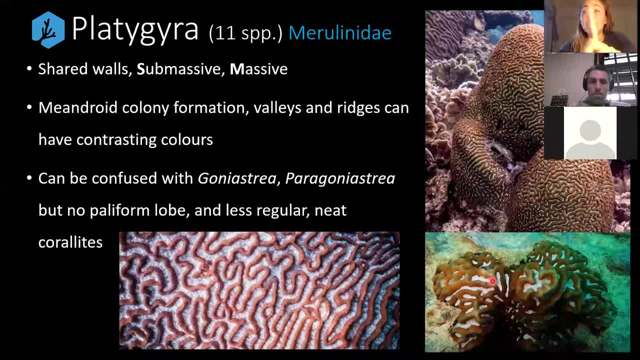 got Platygyra. I know this looks a bit different. I don't know if you've seen it. I don't know if you've seen it. Sorry, This looks a bit similar to Paragoniastria australensis, which is over here. 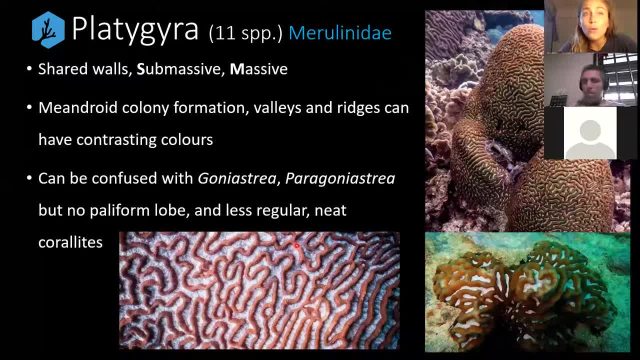 but it's okay On the tops of the walls. Platygyra are a bit more like this. So you've got your valleys and you've got walls and they're quite flat at the surface On the Paragoniastria they 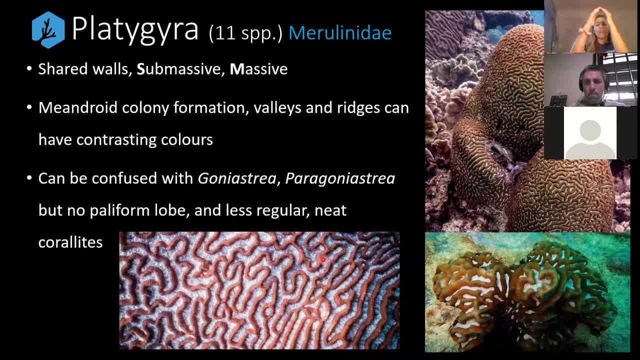 kind of like turn into this nice, like, sort of like rounded bit. I'm going to go back for a moment. As you can see here, it's kind of like a nice point Going. Platygyra is not quite. 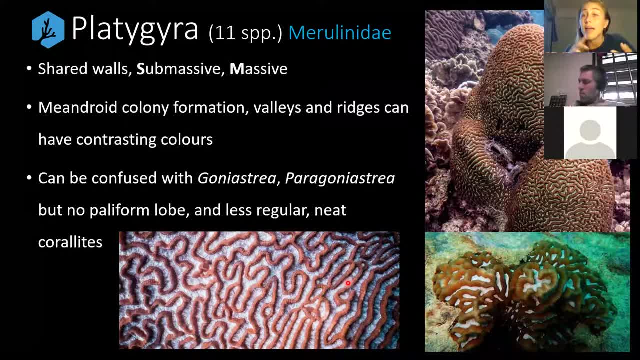 I like that. They've also got shared walls. of course They are fully meandroid, Valleys and ridges also can have the contrasting colors And sure they can be confused a little bit with the Goniastria and the Paragoniastria. but these guys definitely no polyformal, Like there isn't. 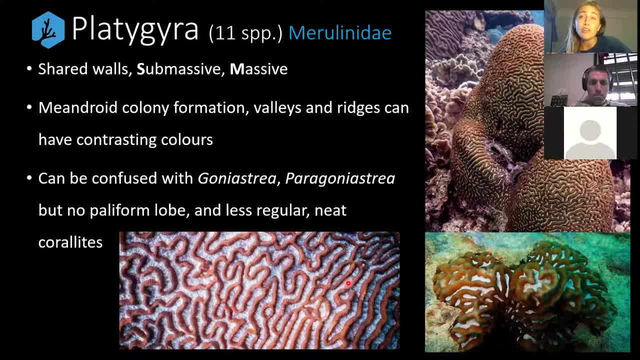 even a hint of them In some of the Paragoniastria australensis. you're looking down the valley and you're thinking, oh, it sort of is sort of, isn't? I'm sort of sort of not sure, Whereas these guys 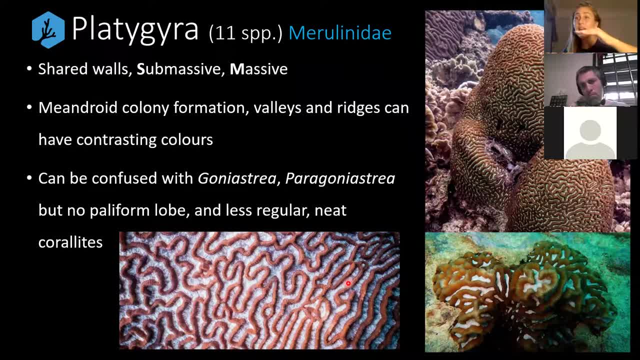 you look inside of it and it is incredibly flat, okay in those valleys. So, honestly, I know it's still a little bit tricky and time it gets better, but that's sort of like the characteristic that I go for every time. Okay, We can discuss later if you guys want to, but we'll move on to Hydenfora. 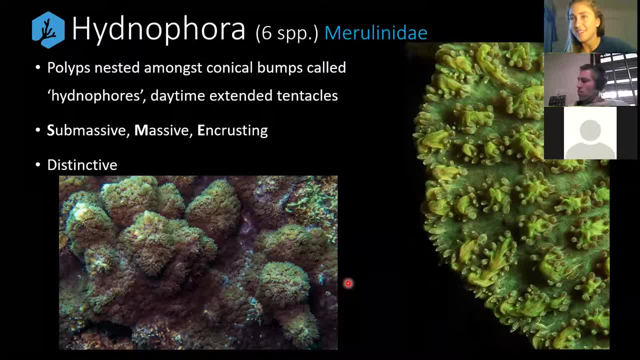 We are sort of leaning towards the later end of the corals that we're discussing today. So I hope none of you guys are, you know, hating me too much at this point in time, but I just wanted to tell you guys as much as we could and 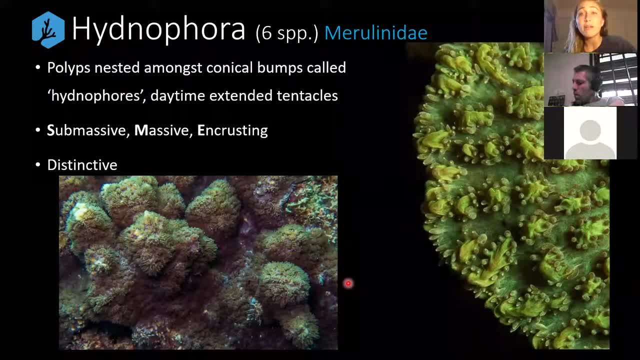 make the most of this. So Hydenfora is still part of the Marillynidae family. Hydenfora, if you guys remember, from the colony formation slide like at the very beginning there was this colony formation called Hydenphoroid. That's for this one. Other corals don't do it, This one does and they. 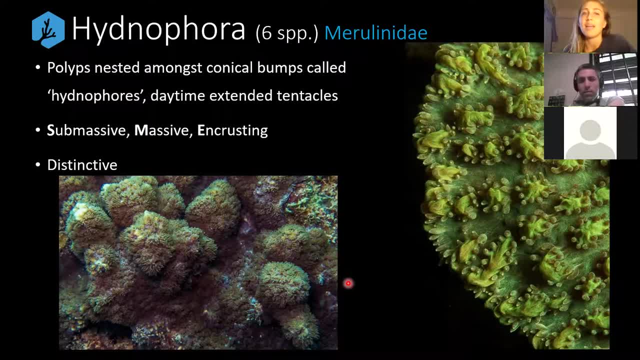 were like. we got to think of another way to describe this skeletal bump, So they came up with the word Hydenophores. okay, So polyps of this coral and nested in the middle of the corals are nested in between these Hydenphores and they've got these beautiful daytime extended tentacles. 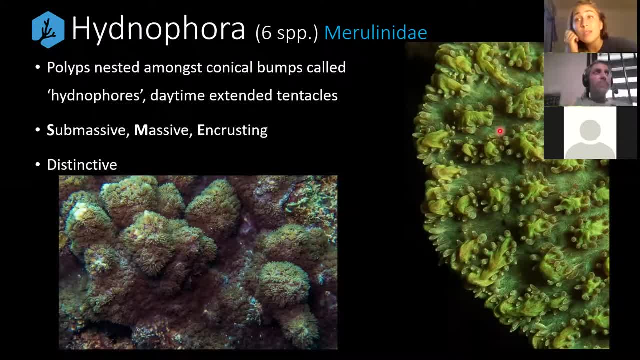 okay, I honestly guys to ID this wouldn't bother even looking for the polyps. All you've got to look for are these large bumps, these Hydenphores, and you're good to go. They can often look a little. 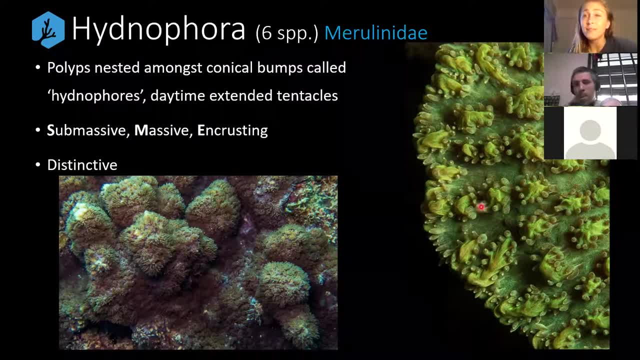 bit fuzzy, like in this colony on the bottom left-hand side, And I always, just, you know, remember the word association by saying Hydenphore, has got its polyps hidden amongst the Hydenphores. It's because, like, I usually can't see them, because they're kind of in the tentacles or the Hydenphores. 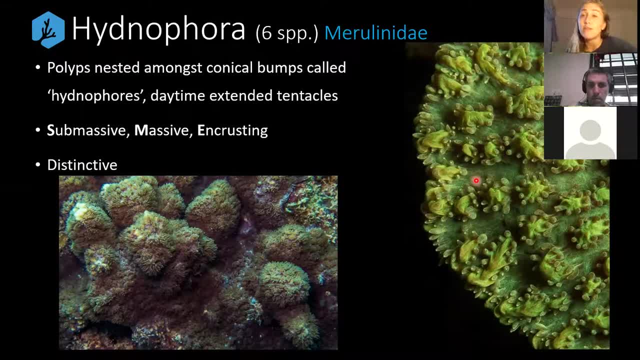 are in the way and they're dense anyways, But this is a very, very, very nice, beautiful colony, for sure. Actually probably not as common and frequent as the other ones we've been talking about today, but I feel like its beauty level was worth throwing it into the 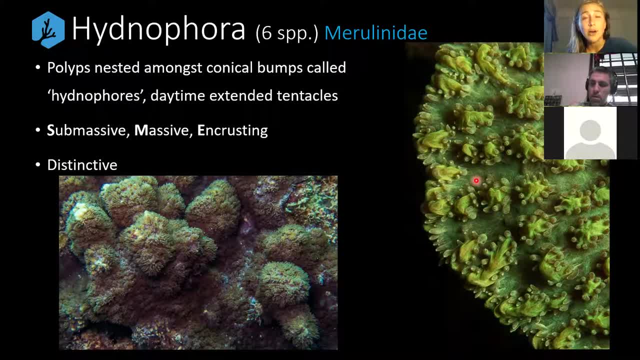 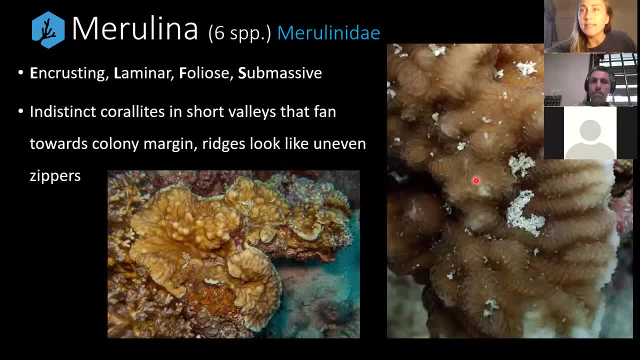 lecture. So if you guys have seen it in real life as well, I hope that you guys can appreciate that one there. So then we've got Maralina, which I think is the last the Maralinaidae for this family. It's a little bit, oh, it's not confusing. 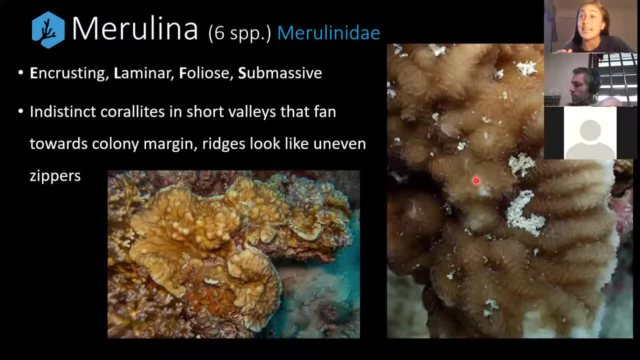 but it's not in one way or any other really distinctive. So what we can remember well, firstly, the growth forms are encrusting, laminar, foliose and submassive, but it has got rather indistinct correlates: There's one here, here's another one, there's a couple like that. 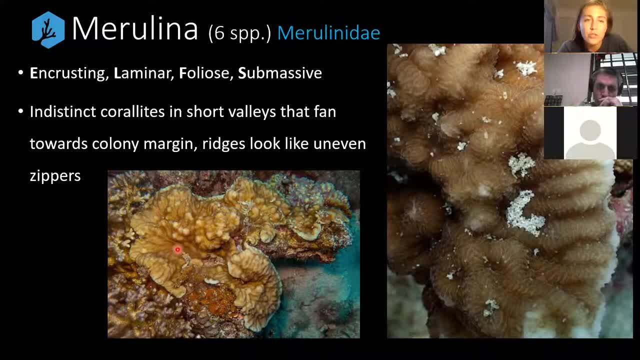 and they're in quite short valleys, which you can probably see, demonstrated a bit more in this photo down here, that fan towards the colony margin. So they're always heading outwards, as we can see here, as we can see along here and as we can see just all around the entire edge. It's never going. 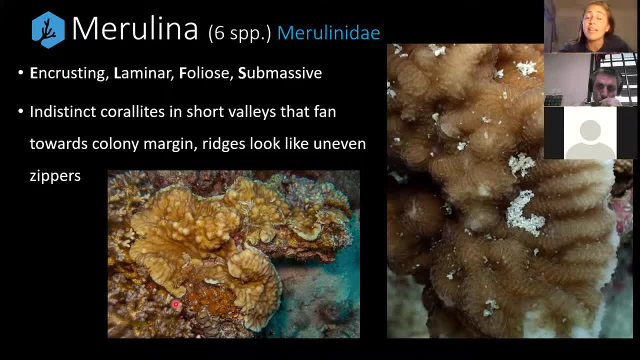 to be running. those valleys are never running parallel to the edge of the coral. They're always running towards it And for me, if you look at the tops at least, kind of looks like uneven zippers. Okay, You don't get a. 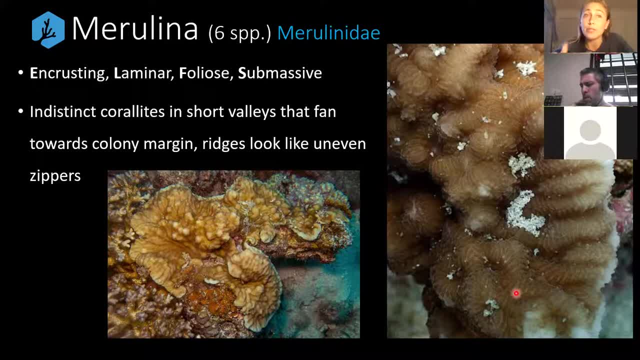 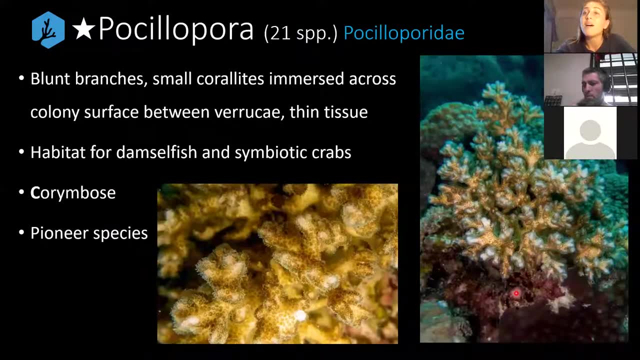 contrast in between the valleys and the valley floor, like we do in some of those other corals in the Marylander Day family that we were just looking at: Phew Postulopora. So anyone that's been to the New Haven Reef Conservation Program? 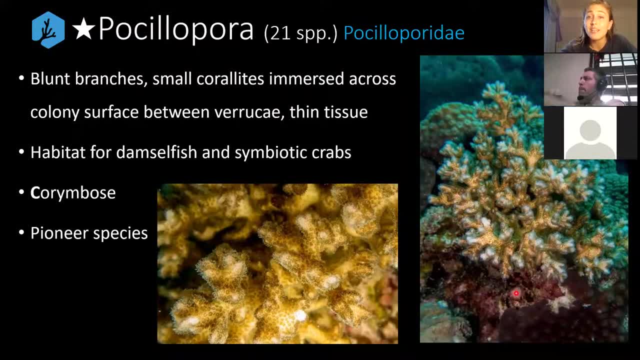 should know. Postulopora. I've put a star next to it. It is just so dandy at growing when there's space available and it's even believed and pretty much, yeah, it's got maybe an extra, I don't know, maybe a little bit of a. I don't know, maybe a little bit of a. 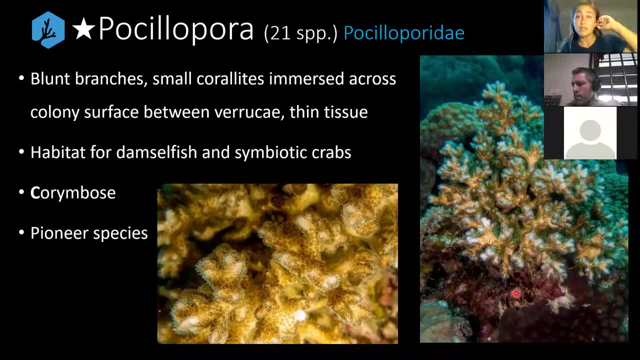 extra spawning season, even in many places around the world, So it'll spawn sort of mid-year, but also towards the end of the year as well. Very special: He's also a brooding coral, So pretty much in the evolutionary timeline of corals and coral sex. 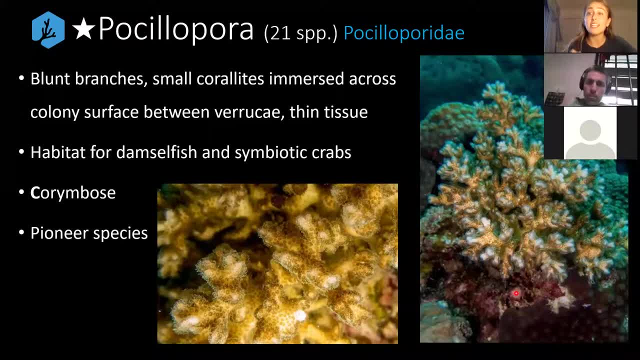 these guys are a little bit more advanced. What they will do instead of just synchronized, synchronously expelling their eggs and sperm together and then being like: good luck, kids, we hope you fertilize, these guys will expel their eggs and then other colonies will absorb the eggs. 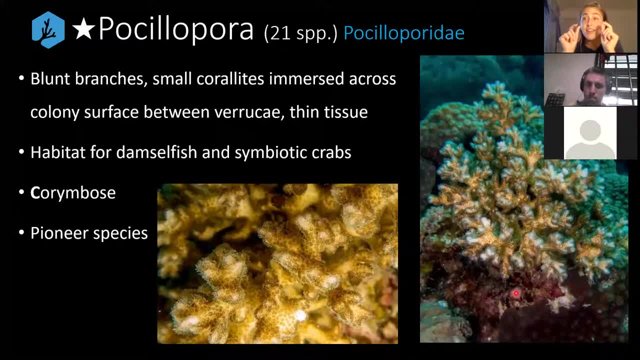 and fertilize them with their sperm. Then they will make a little larvae and put some zooxanthellae into it so that when they eventually shoot the larvae out, they've got a renewable energy source. They're like: hey, kid, we love you. Here's a solar panel. And that's actually how these guys 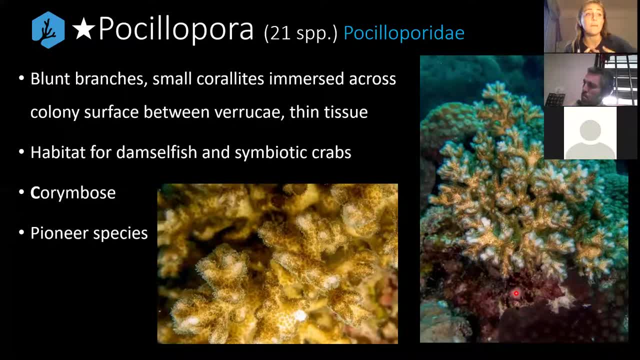 spawn, So they are a little bit more advanced, which gives them a lot more success in terms of having their offspring survive. But an implication of that is that it can lead to more genetic bottlenecking, especially depending on where the colonies are placed, where the spawning of the 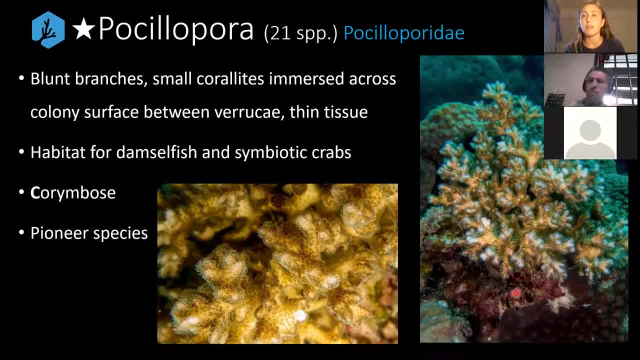 eggs is happening and absorption- You can get a lot of genetic similarities happening there as well, But very, very cool in terms of their approach to spawning compared to a lot of other species. Anyhow, Postulopora, a very successful genus, Postuloporidae in general are very good. 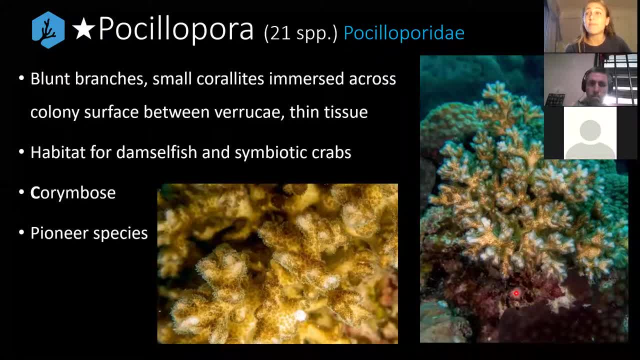 You've also got the Stylopora, the Cereatopora. Depending on your region, you might see those ones a lot. If you want more information on them, please let me know. But this one I think I see most diving I've done in the Indo-Pacific. We've got these very blunt looking blanches branches. 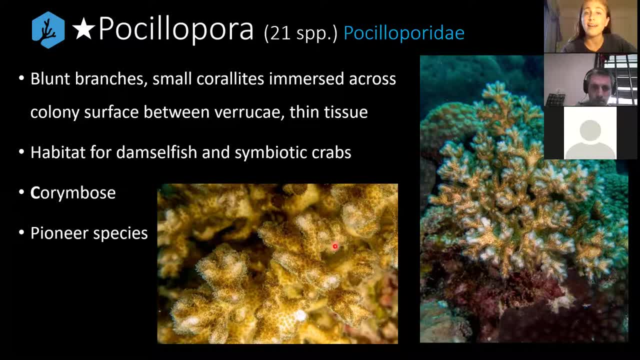 they are very, very, very muscular. they have this very fuzzy appearance pretty much all over And they've got these very, very short, skinny tentacles that are mostly always out, give them that sort of fuzzy all-around appearance. They are immersed. small coelates are immersed across. 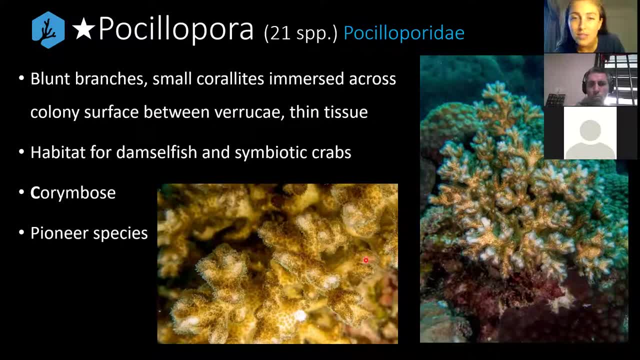 the colony surface between the variceae, which is also kind of like little bumps, which is not too obvious on these colonies here, But it can have a bit of a bumpy skeleton as well. structural complexity, like our acroporas did that we were talking about before, again providing cool. 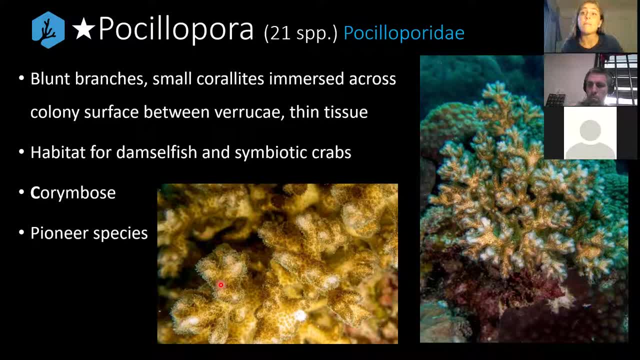 habitat for damselfish, symbiotic crabs and so on. they grow corumbos, which is the dense branching type of growth. okay, we don't get them in nice long skinny branches like acroporas. this one is very, very dense and it is what we call a pioneer species. does anyone know what i mean by pioneer? 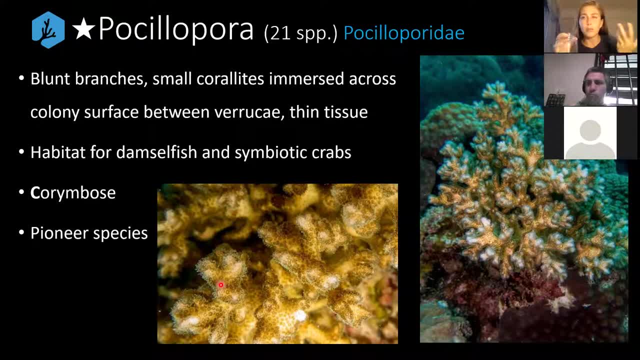 species at all, sort of a term that probably isn't thrown around that much. um, okay, i'll tell you so. you know, in the literature you sometimes do get corals being described as pioneers and think of it as literally like: what do we mean when we say a person is a? 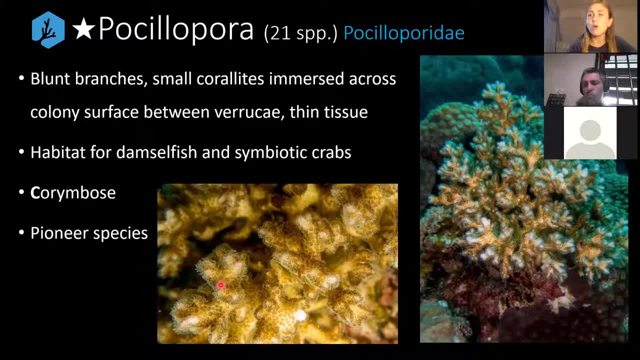 pioneer. maybe you know they'll go out and explore the ocean and find a new island. maybe you know that that person might be described as a pioneer, uh, for finding more land. we can you know, okay? so let's take a look at a lot of the questions that came in from the audience. 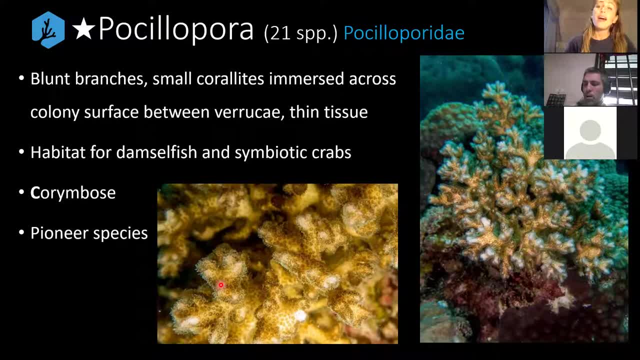 so I think it's 2 million people, right? so? so let's take a look at 2 million people, right? so this is also what we're describing for corals. So I said earlier on that corals require hard substrate in order to grow, and they pretty much do, But some can do a bit better when the 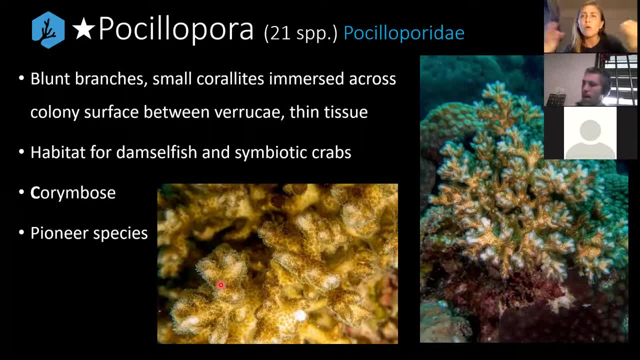 conditions aren't quite right. So say you've got a field of small rubbly patches or something like that. okay, For some corals that are very slow growing, if they happen to recruit onto a piece in unsecure rubble, they might get a pilot developed. they might, you know, asexually. 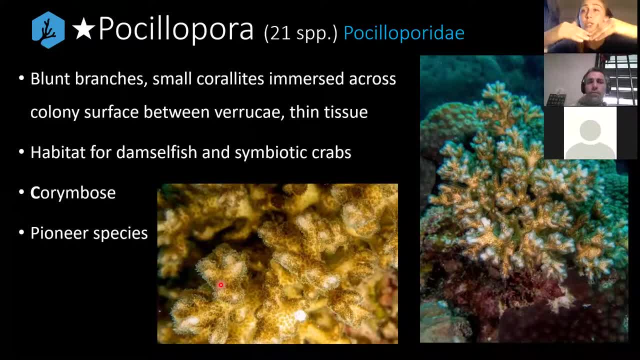 produce a few more. but if, like some surge, comes through and that piece of rubble turns over, it might be the end of its days and it might not do very well, Whereas a colony like Pocillopora can essentially like go and recruit and start asexually producing so quickly and invest a lot. 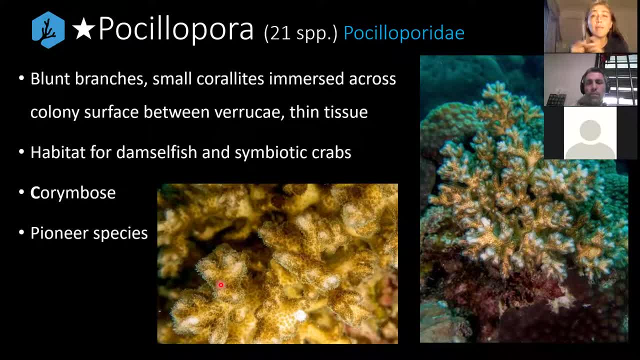 of energy into growth, that even if with time that fragment rolls over and dies, the colony might be big enough that enough of it survives, it's still facing the light. it'll grow back over and grow back over. So even if it is a little bit of movement, it can actually, it's shown to do. 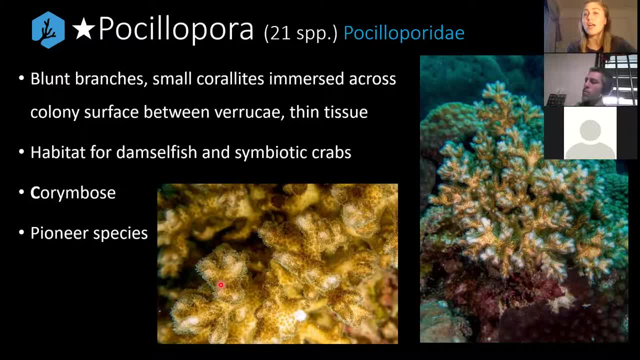 actually out-compete the movement of its substrate, Occasionally even breaching off into areas that were previously uncolonized by corals. they find a little bit of hard substrate. if it's not even 100% secure, it might just be enough for them, because they really do all their. 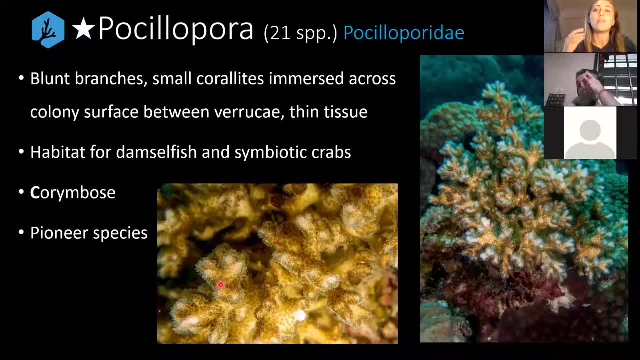 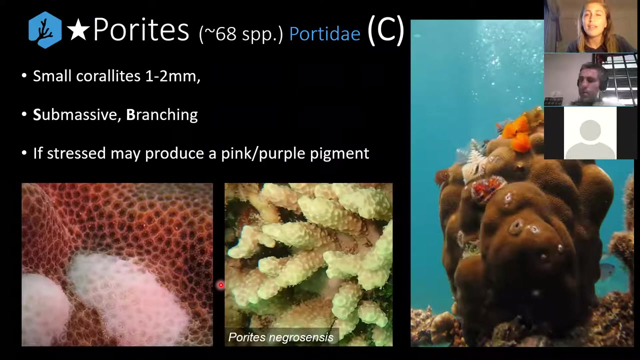 investment, A lot of energy into growth, they can kind of outgrow the disturbance nearly So a sick colony. in terms of resilience and, you know, hard work and, yeah, tolerance to moving substrates, I suppose we can say: All right guys. So parietes- we mentioned this one earlier- having lots of little small pores. 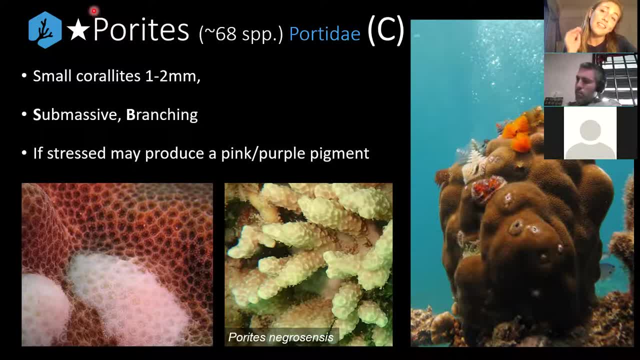 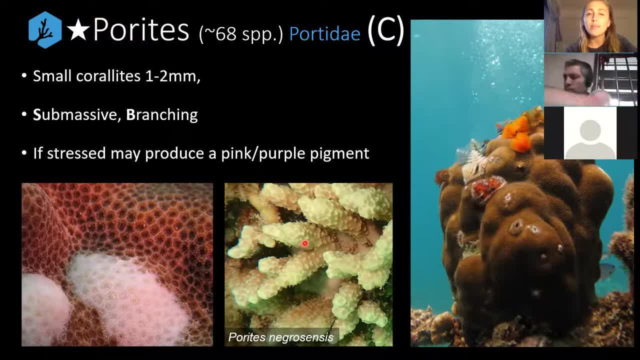 I think it's a pretty easy one to remember. Parietes, with the exception of parietes Negrosensis, is, generally speaking, a submassive, funnily shaped coral colony with a lot of small polyps that you could just say look like pores. 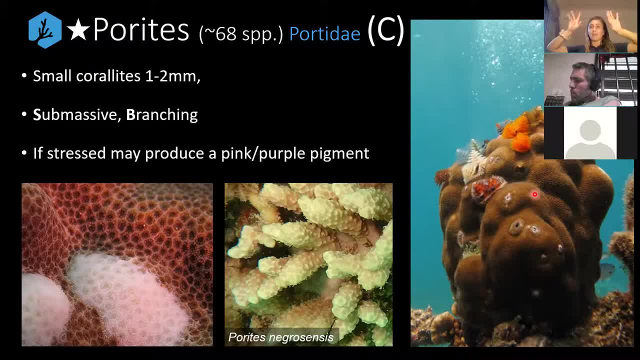 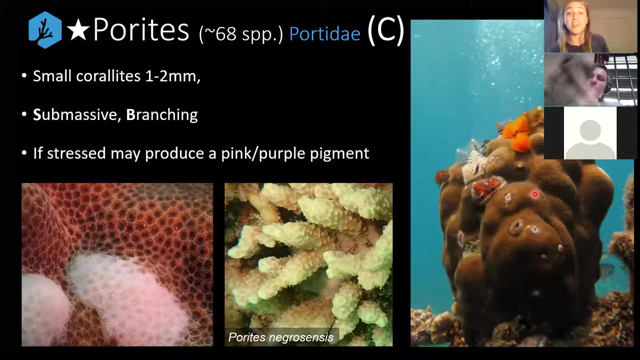 Think of us humans. We are funny-shaped animals with dangly bits on our extremes and funny-shaped faces And if you look up close, our skin is covered in pores. So parietes is a porous animal thing, if you want to remember it like that. 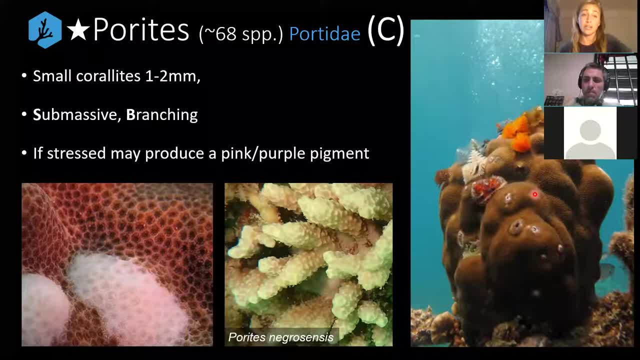 I think it's one of the easy ones to remember. So the correlates are very small, one to two millimetres. We get them submassive, as is on these outer two images, and then branching, as we can see in the centre here as well. Sometimes they produce a pink to purple pigment if they are feeling stressed. Some of you guys may have heard about fluorides- Fluorescent corals- when they're under stress. Fluorescent exists amongst all corals all the time, but usually we can't see them without UV light. 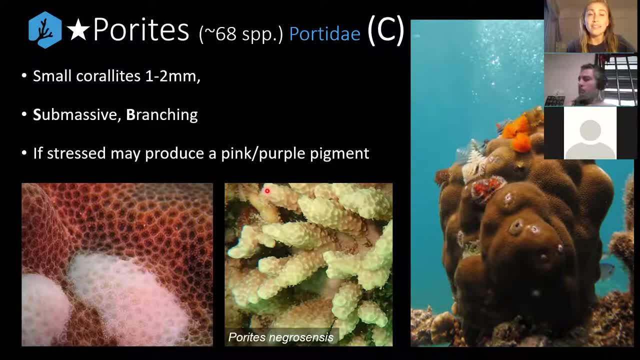 But sometimes under stressful conditions, even our weeny eyes can pick up on the fact that there is a stress response happening there And they can use it to either absorb more light if they are deep, and sometimes they use it to reflect light more if they are too shallow and suffering from, say, stress heat. 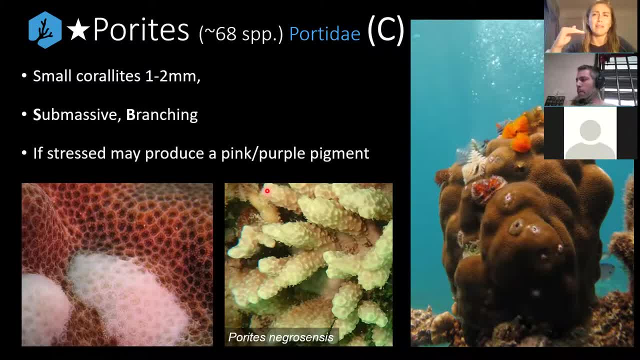 So really, really interesting there, And that's very, very, very shallow. There's a shallow explanation of it, but it is a stressed response. Also, note that there is a C plastered right here, which means parietes as a genus also exists in Caribbean waters, okay, and is a contributing reef builder there. Sometimes you'll find that a lot of Christmas tree worms will exist on parietes corals- not everywhere you go In the Gulf of Thailand. these Christmas tree worms love parietes. I don't know, But it's a nice little relationship they've got going there. 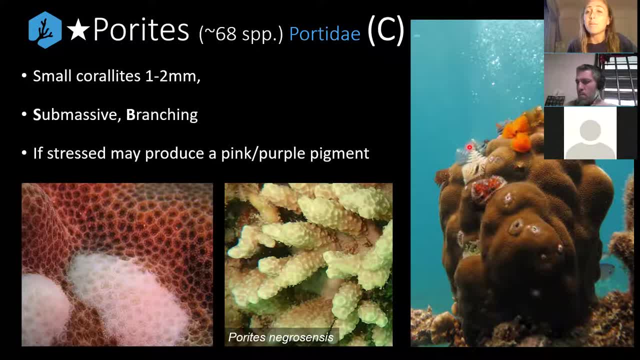 It's even suggested that these little Christmas tree worms actually protect corals like parietes from predation from crannothorn starfish. They like tickle the bottom of the starfish and the starfish are like. I don't want none of that. 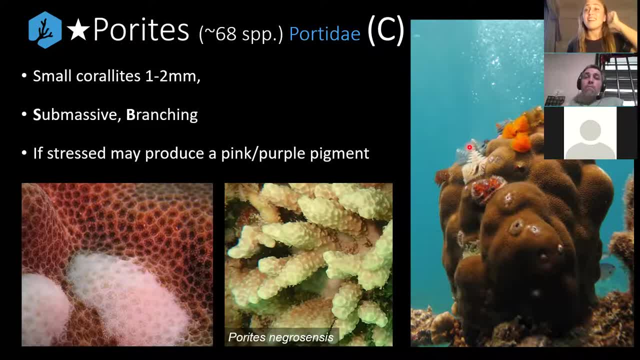 And then they'll go away. So they are showing that in instances where there are Christmas tree worms- versus there not being- they are less likely to be predated on by crannothorns than when there aren't Christmas tree worms. So How about that, guys? 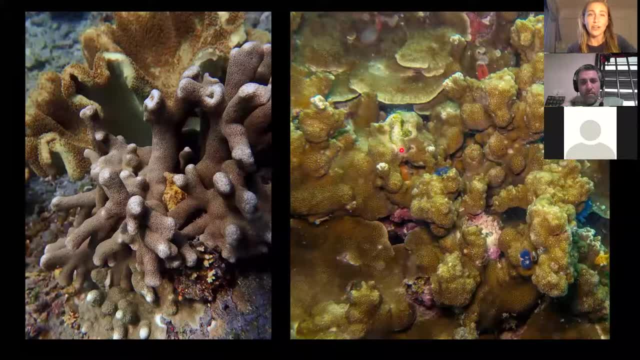 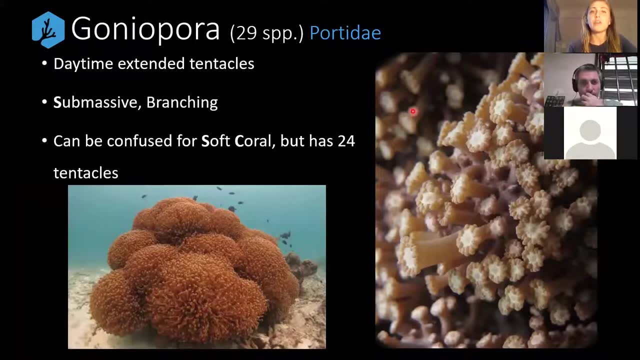 Beautiful. There's just a couple more examples of the different varieties: the branches, the plates, the kind of awkward submassive shapes here. All right, So then we've got Goniopora, which is a parietidae as well. 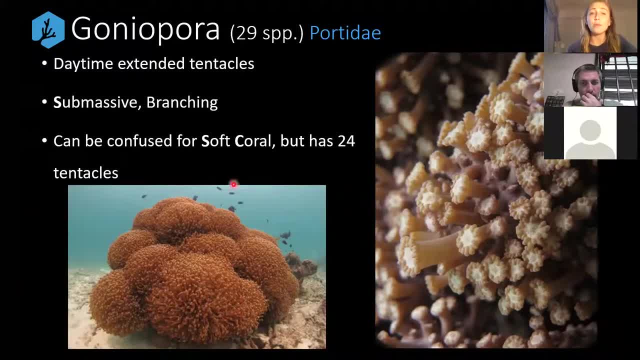 We have got these lovely long daytime extended tentacles. Some people look at this- and I know this is a 2D picture, but if you see it live it's sort of like all flowing about because it's got these lovely long tentacles. 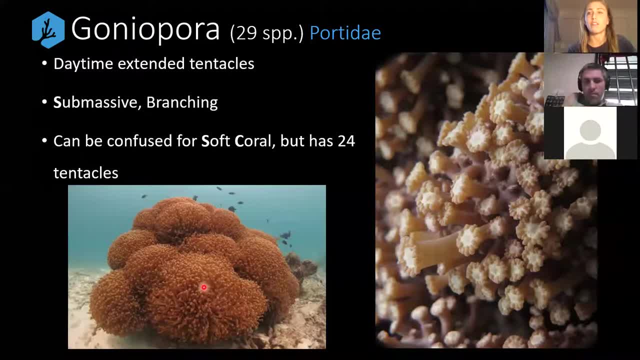 And a lot of people think that's a soft coral. It looks soft And I totally get it. It does look like a soft coral, But if you kind of try and imagine what its base structure is, that isn't moving. There is indeed skeleton below. 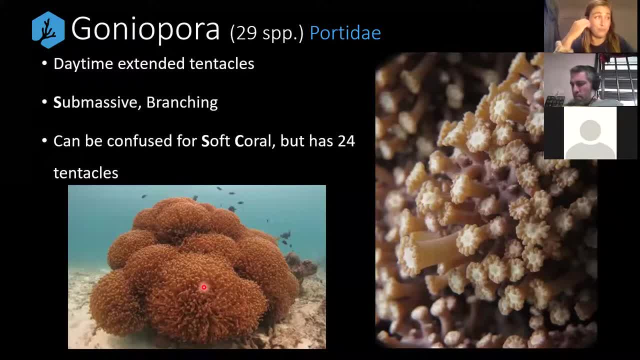 If you want to, you can give it a bit of a wave, and that well, don't do it just for the fun of it. But if you're really unsure and you're doing a survey, you can give it a little bit of a wave and that disturbance will often cause the tentacles to retract, as you can see they're doing in this photo here. 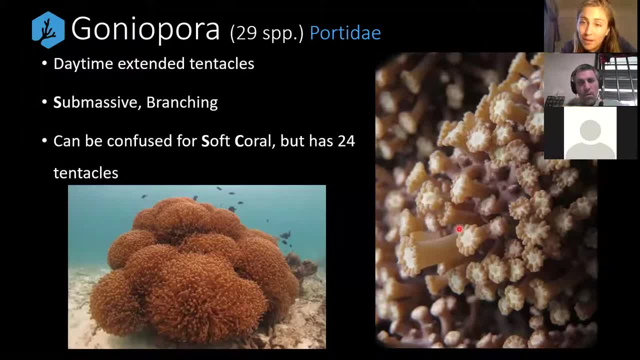 Also, these guys at the tips of their little flower-like tentacles here have got 24 tentacles. You guys hopefully remember me saying earlier: Sclerotinia have got tentacles in multiples of six. Octocorellia have got tentacles in. well, they have eight tentacles all the time. These guys' tentacles in, yeah, multiples of six, and this one has 24.. There's another genus called Aldeopora, which looks so similar to Goniopora. The difference is they have 12 tentacles. pretty much, okay. 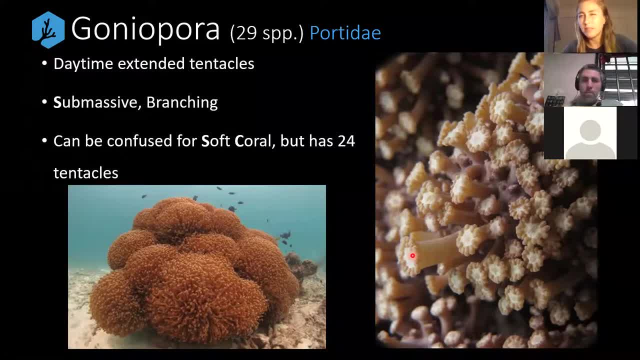 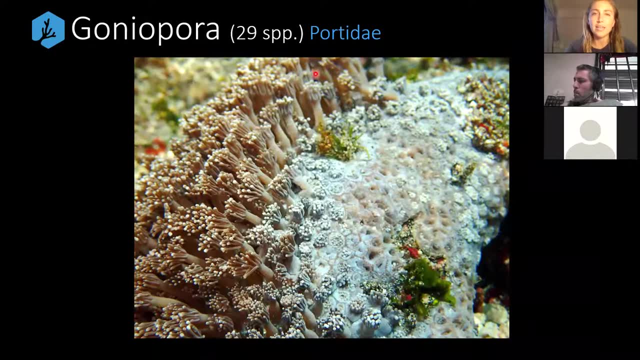 But Goniopora are probably a little bit more common depending on your location. Here we can see an example where you really have both happening. You can see the tentacles are long, they extend here and they are retracted here for some unknown reason. 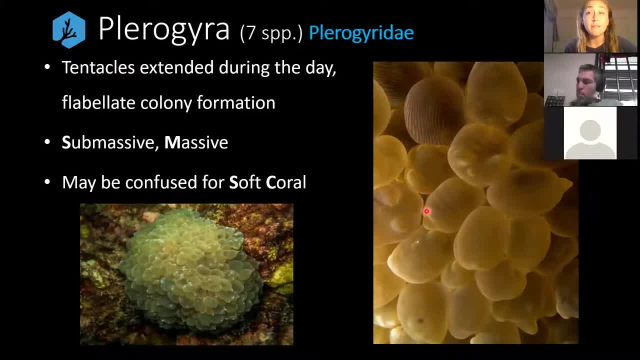 Cool. So let's look at one of the bubble corals, just because often people mention bubble corals, so I thought it's quite useful to include it here. We have Pleurogyne Pleurogyra from the Pleurogyraidae family. 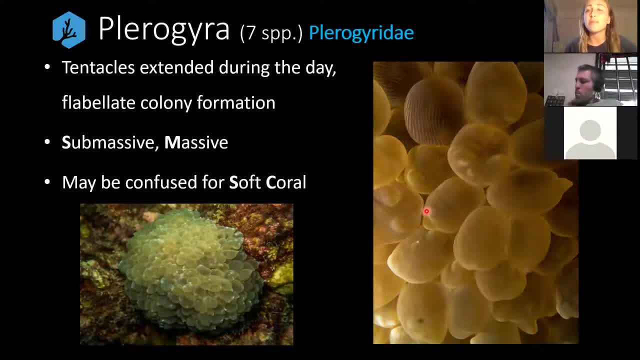 It's got seven species. Tentacles are extended during the day. To be frank, I've never seen one with the tentacles retracted. I've tried before giving it a little bit of a wave and it sort of seems like it tightens up a little bit in terms of these bubble tentacles, but otherwise not that much happens. 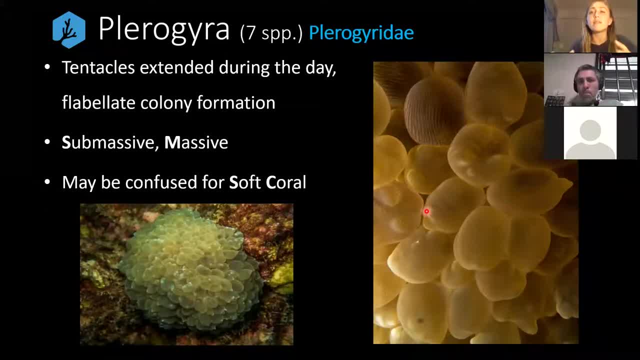 Understandably confused for soft coral, But you can see there is some solid structure below that. you know It's not wobbling like the whole structure of it. But if you remember Pleurogyra, yeah, The bubble coral, even though it's bubbly and looks soft and lovely, is a hard coral. 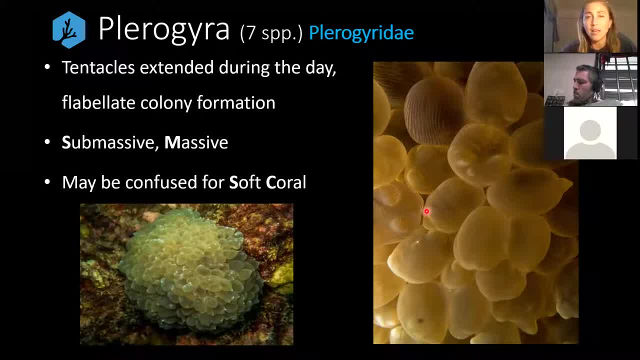 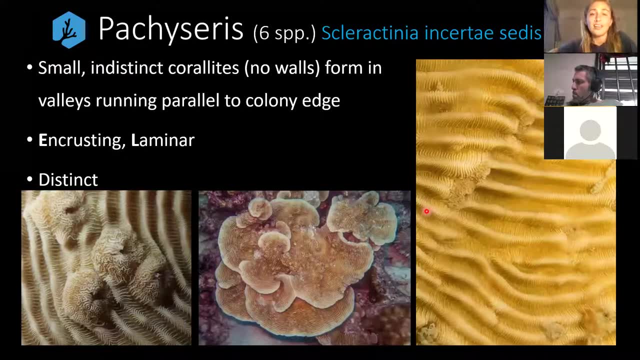 Just one that again people have asked, so I just threw it in there. But I won't go into too much detail about it. unless you guys want more photos or anything later, just let me know. All right, So then we've got Pachyceris. 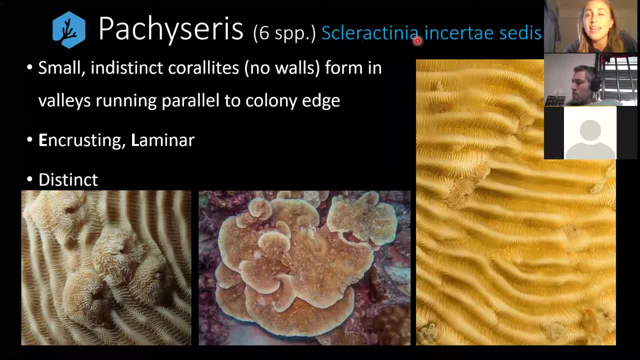 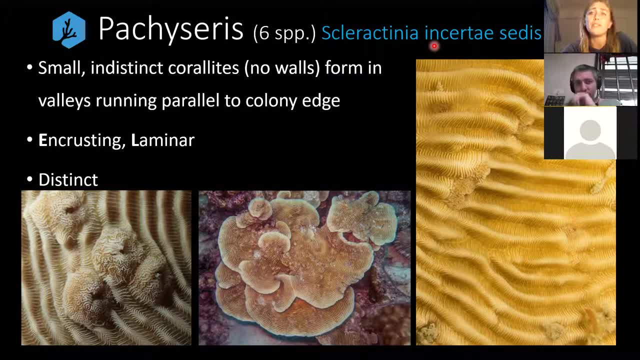 is that the family of the Pachyceris is still being confirmed in terms of genetics by the experts that deal with Pachyceris and other corals similar to that, So it hasn't got like an exact confirmed. where does this sit in terms of the taxonomic tree quite yet. 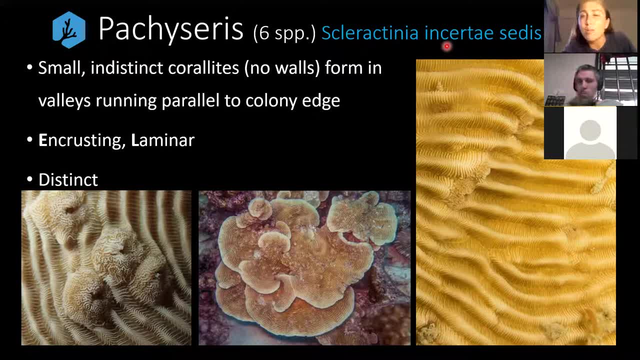 So Pachyceris has got an interesting form. It is sort of meandering. You guys might remember before. it's meandering Pachyceris type That's describing here. Yeah, I remember when I had my first coral taxonomy class. 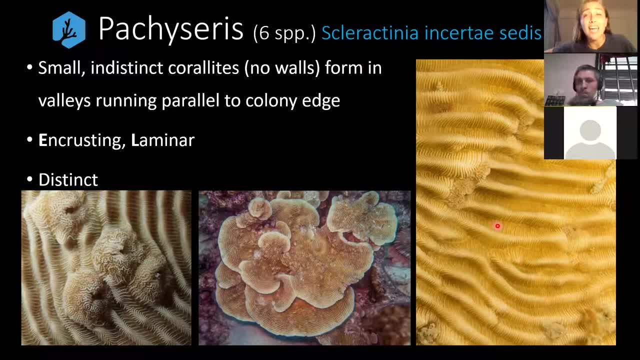 I was a conservation diver and at my coworker, Pau gave me this lecture and he or a variation of this lecture And I remember he got to this slide and he goes: Oh, Pachyceris elephants. I was like what man? 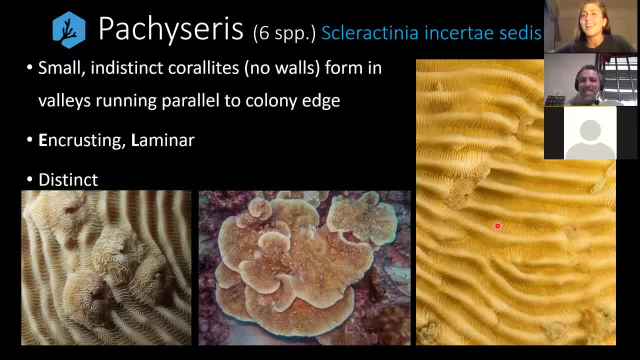 Yeah, I can see your face, Trev. you're saying that to me right now. Like what I was? like, hey, Pau. like what are you talking about? He's like elephants. their ears are wrinkly. I was like, yeah, cool. 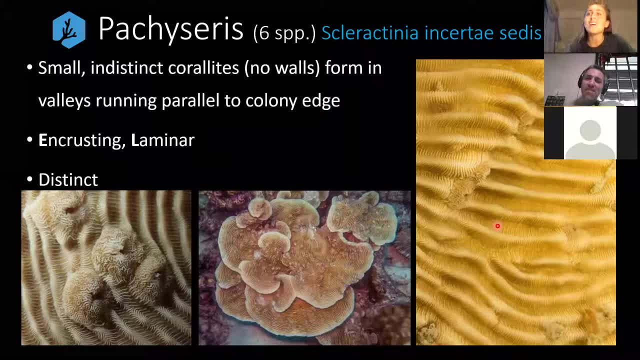 But like I'm still not sure what you're talking about, And he goes: taxonomy: elephants family name is Pachyderm. There you go. So the elephant family name is Pachyderm. Elephants have wrinkly skin to aid in heat loss. 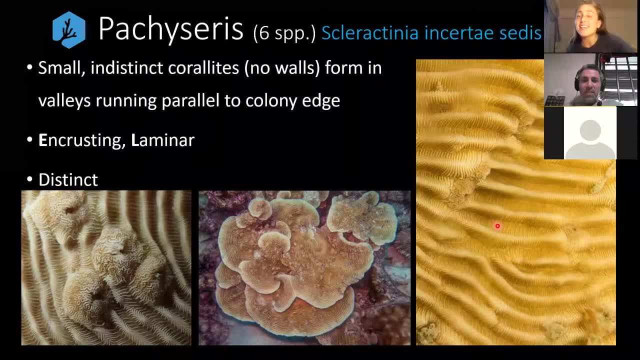 Pachyceris sounds like Pachyderm. Pachyceris is a genus of coral with folded. you know folded like growth form. So obviously this is where the connection is And I thought, oh wow. 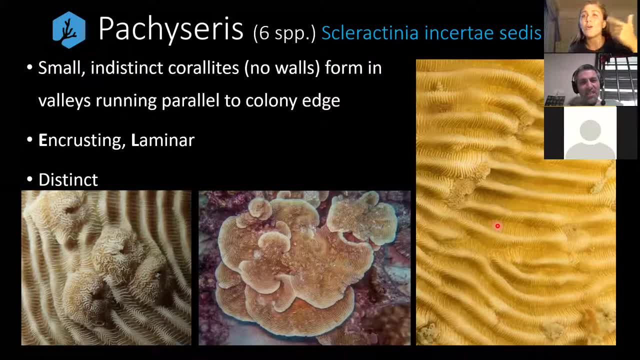 And now I've never forgotten the name of the elephant family or this genus of coral, So I hope you guys come out with the same, with the same outcome, as I did- And I didn't know either of them, though, when I went into this. 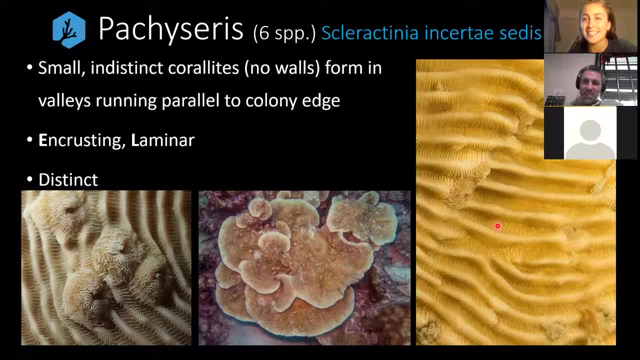 Anyway. so we've got small, indistinct coralites. You don't even need to bother IDing them precisely, Cause you just look for these wonderful valleys that run parallel to the colony's edge. There's nothing quite like it. It's a very, very distinct genus that has six species. 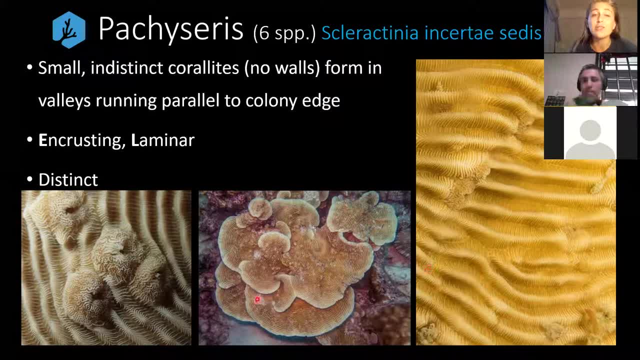 It grows in crusting laminar. It really does look like some big floppy elephant ears. Like he wasn't wrong, That's what it looks like. You know this photograph to your left here. it's not vital or anything, but just because of the, the sheer, like beautiful detail of the scepter which run along these valleys, when you have little invertebrates boring into the, the actual skeleton in the skeleton, 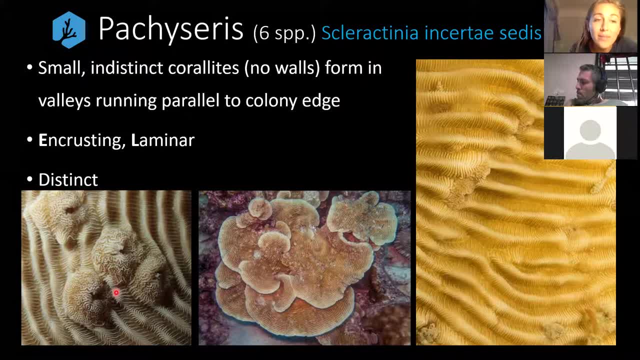 you can see it. You can see it, The skeleton reacts by, you know, trying to grow over them, and it just, you know, these phenomenal little patterns emerge And I just think it's so cool, So I just wanted to include that photo there for you guys. 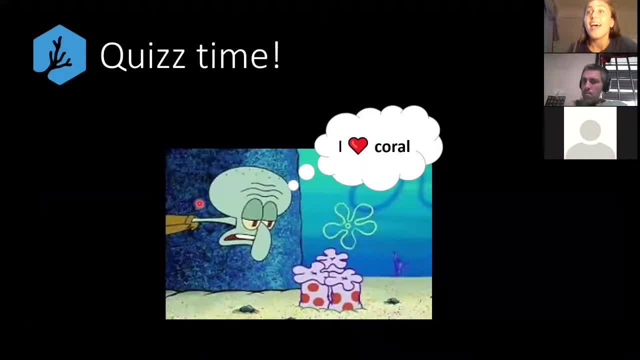 Anyhow, Pachyceres elephants. So, guys, we have a little bit of a quiz. Here's Squidworth from SpongeBob SquarePants, enthusiastically looking at some coral. And look at his back. He's not making his back. 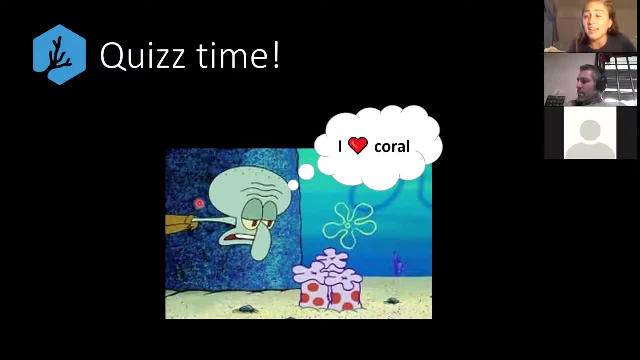 He's trying to do it again. Look at his back. So he's trying to do it again. I don't know He's trying to make his back again, But the, the Serpentess, is a very fast working pyramid And if you're going to test this, you can test the. 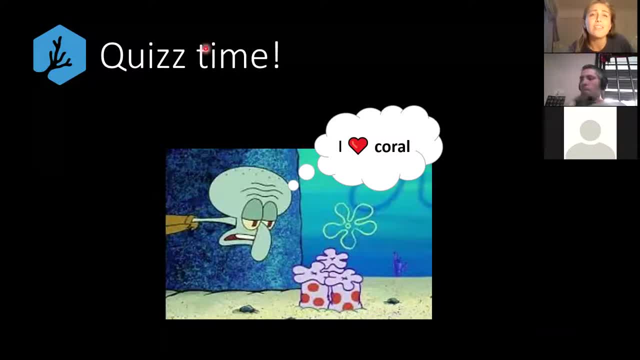 core and try to use thepture in the shape of a flower. If you want to test yourself, this is something that might be natural. if you want to, I think you could test yourself. I think this is going to be a really great example of a really cool work. to start with, 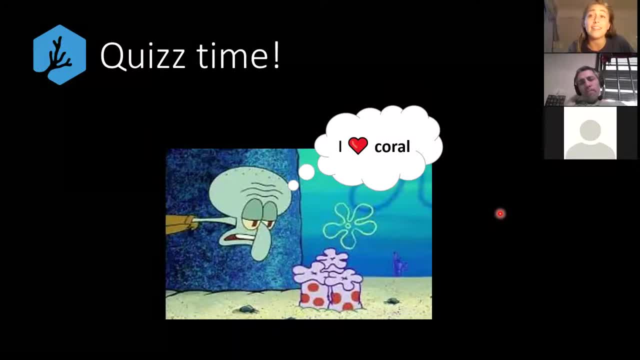 So, in terms of being creative with the Labrador Orchid, I'm actually not sure, But this is a really cool project that's been going on for us for a really long time, And I've told you that it's going to be a hell of a lot of fun. 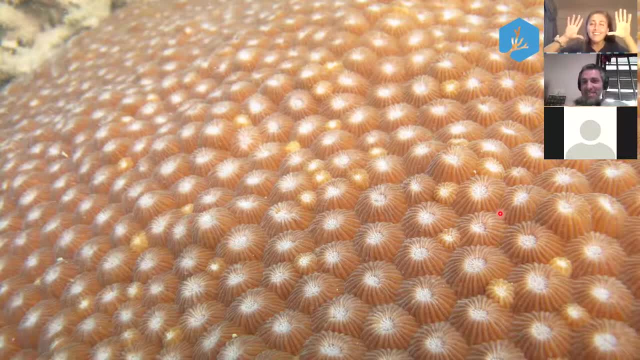 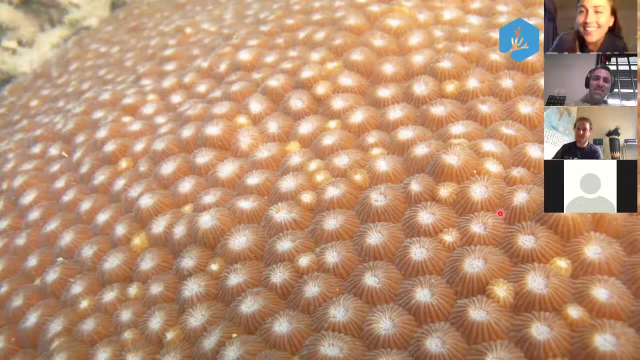 diploastria. ah, that's yes, wonderful diploastria. you nailed it on the first one, anthony. sorry, that's diploastria. heliopora legend- awesome, i don't, i should have written heliopora there, i just wrote species. anyways, what do we have here? 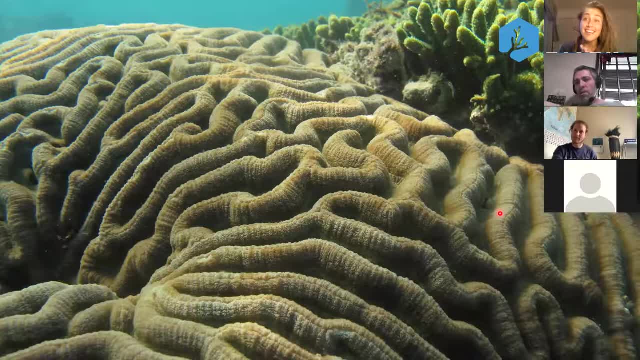 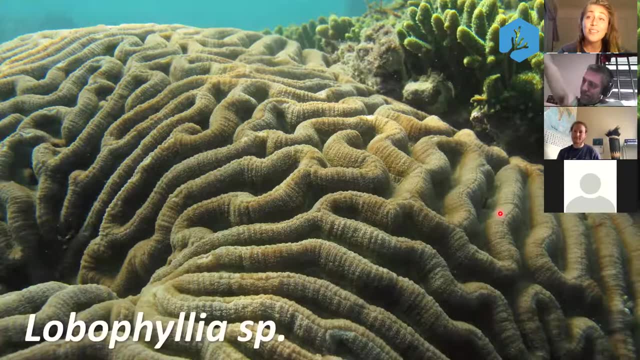 that's brain coral. it's a brain coral lobophilia, lobophilia- amazing. i love your work, guys. so this also has been recently, recently, in the last five years or so, changed. this one used to be called symphilia, um, but now it's lobophilia, which is an easier name to remember, so it's nicer. 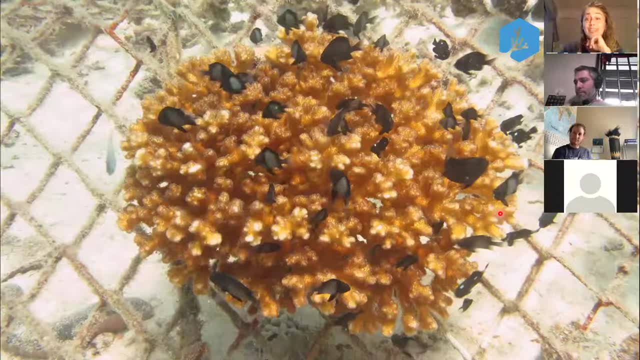 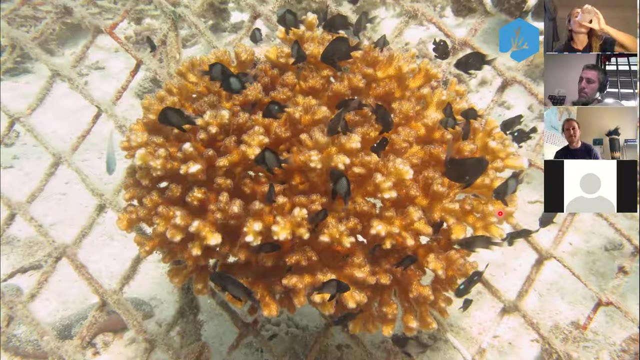 for everyone involved. what's this one here, acropora? oh sorry, we had an acropora, not quite right, but it branches and corimboses like acropora does poslopora. i think two, yeah two- of you guys just said it, then perfect this one's poslopora, which is: 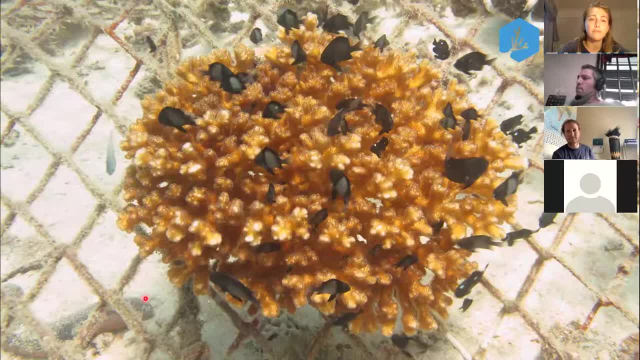 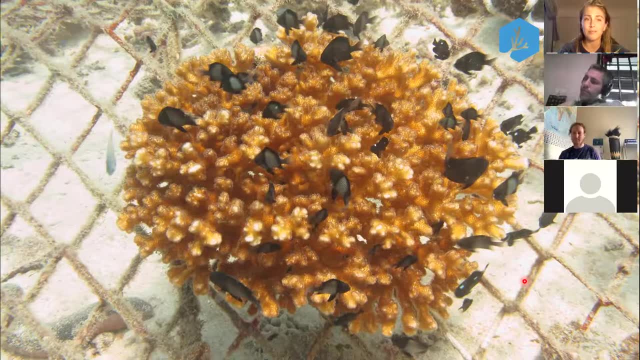 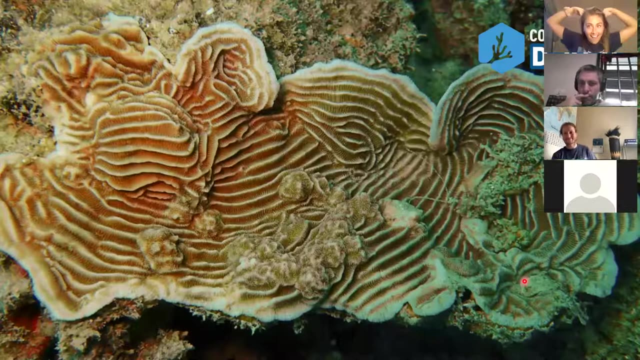 recruited or recruited, no, transferred onto this part of this structure here and they grow incredibly fast, um, unbelievably fast sometimes like yeah, it shocks me still to this day. so 없alby must definitely see them grow. i'm acting them all out, so you guys should be looking at my screen because i'm 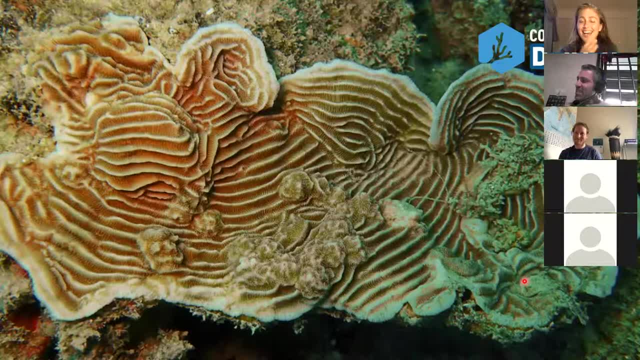 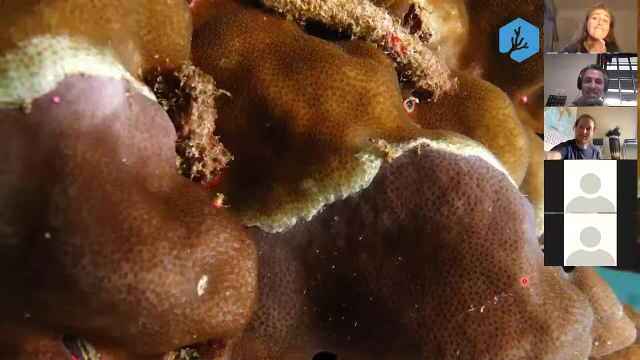 yes, yes, everyone's nailing it. love it. pachy series polytest. yes, tuobi sport couldn't tell who that was them, but two of you guys just yelled out parodies and that's bang on. can anyone tell me what's happening in this photo? warfare, so species warfare? yeah, warfare, we've got. 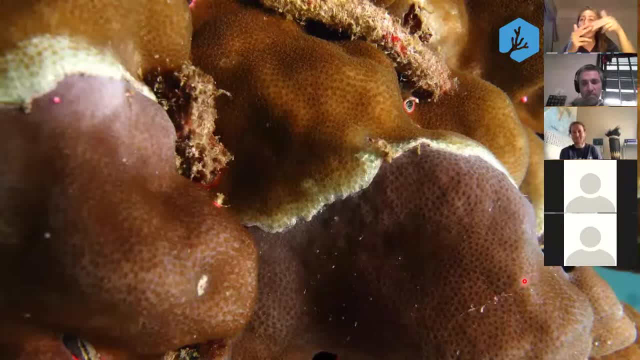 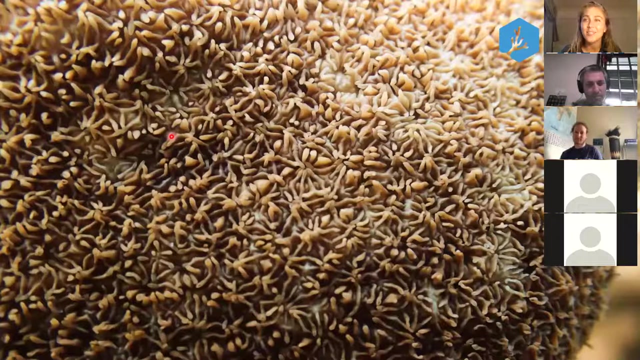 two, two of the same speed. oh, looks like two of the same species that are competing for space and they're trying to grow over each other, and it looks like the top variety is is winning awesome. well, this is a tricky one because the tentacles are out, so we'll see how you go. 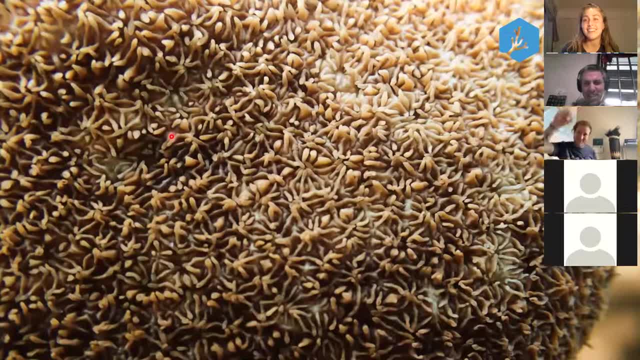 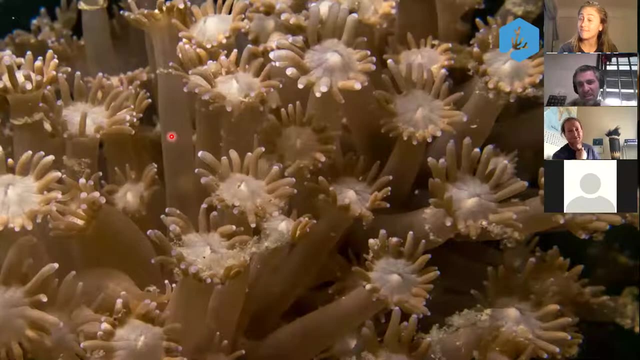 okay, yes, i like that, i like that a lot. that was awesome. um, i hope you all say that in your head now every time you ever go to three point awesome, what do we have? oh, yes, that was like three people. yes, you said, if you said goniopora, which is what i think you said- 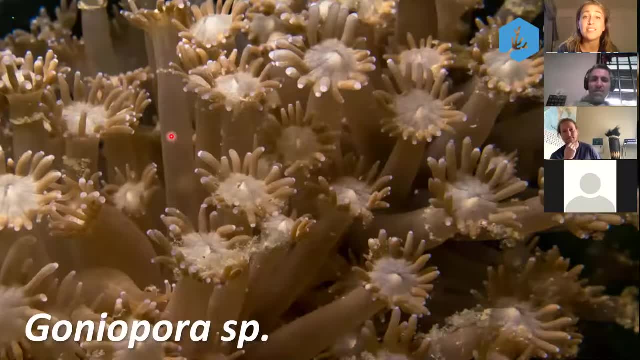 you'd be absolutely right, awesome. so there's the 24 tentacles there. there's the other one that looks the same, or at least very similar, long tentacles, but there's 12. that's alveopora, but that doesn't matter. you guys nailed this. i think this is the last photo, guys. 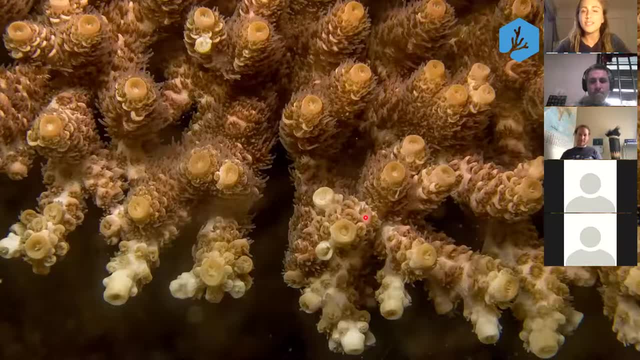 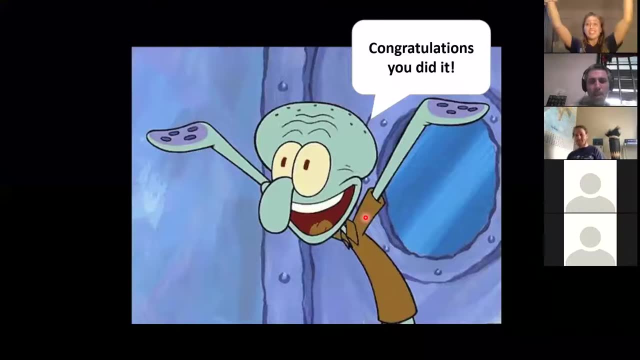 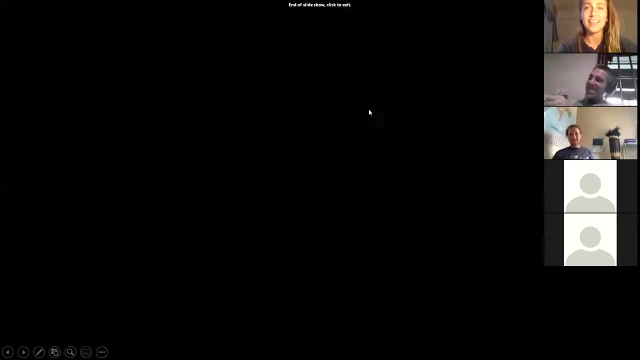 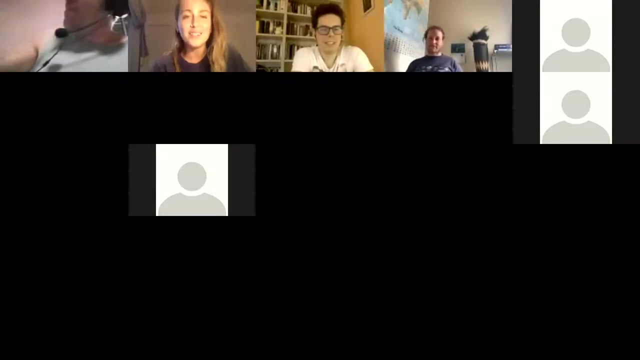 oh cool, yeah, i just heard it, a few of you once again. yeah, awesome, this is acropora, so good, congratulations. you actually made squidworth smile, which apparently is quite rare. yeah, i mean, i think we've all seen spongebob, so that was awesome, guys, um, not too many of you have. 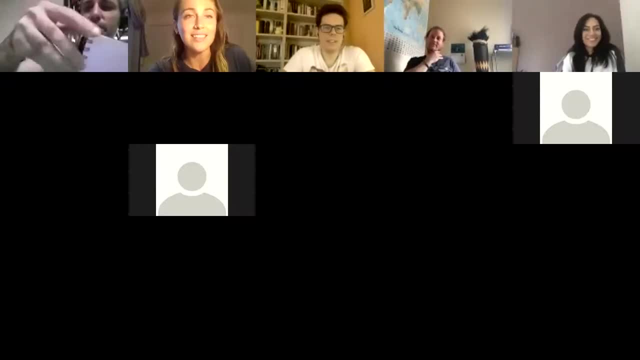 like logged out and you know, i hope you're not leaving this hating me and thinking, god, that was boring or anything like that. but i hope you're not leaving this hating me and thinking, god, that was boring or anything like that. um, have we got any questions? or sort of anything like that. 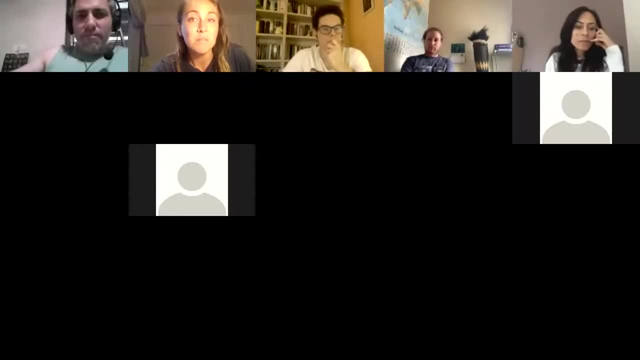 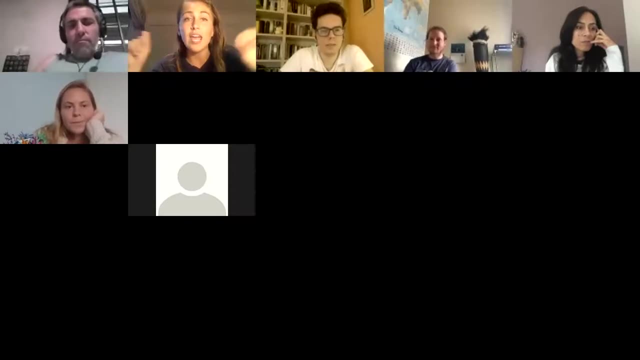 are we feeling like we want to do the exam? actually, maybe, in terms of the exam, some of you have already emailed me. if you did already, sweet. um. if you guys are seeing answers being written as well, all the right answers. um, if you guys haven't told me yet that you want to have 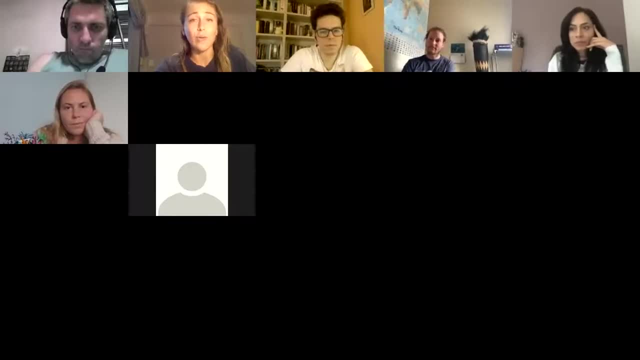 the exam. um, just send me an email and i'll see you in the next one. bye, bye, um. if you do, i'll send it to you. it's predominantly multiple choice. it's a lot of like photos being like. you know. here's this photo. is it this curl, this curl, this curl? you know i'm not gonna, i don't. 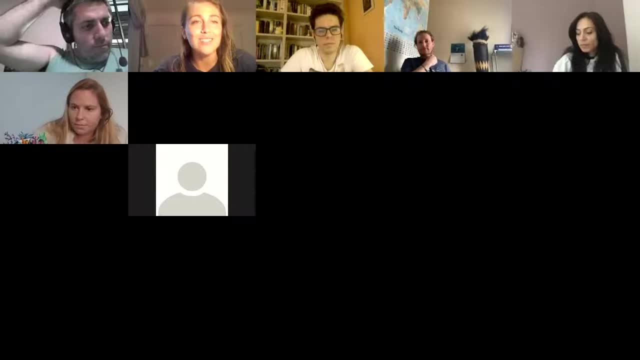 mind if it's open or closed. you guys can decide if you use other resources or not, but you know it's testing yourself, so send it to me when you're done. i'll send it to you as a pdf. um, you can use, you know, adobe or whatever you want to. 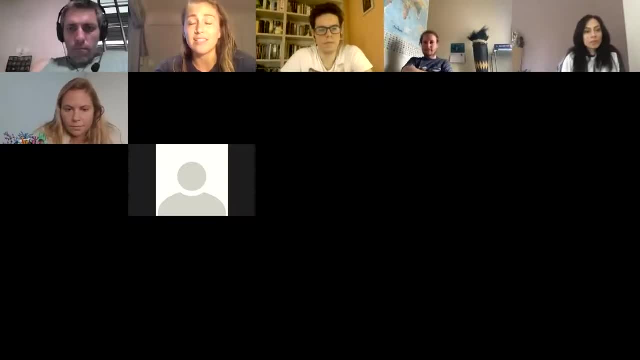 to write on top of it and i'll give you guys feedback. if i feel like there's anywhere that you need more, whatever i can i can let you know. also do let me know if you want, like, more resources. we've had some amazing students and interns and um teachers in the past have just made some really 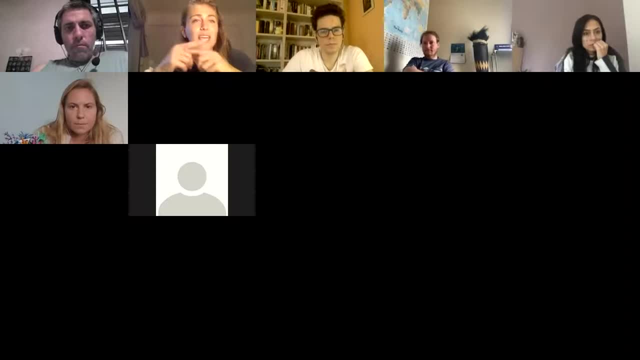 really cool resources like little puzzles and little keyword things and just cool lists with like symbols and how to remember different curl, um. but yeah, that's like mostly it's it from me. if you guys haven't heard already, my boss, chad uh, cd founder, is going to be doing. 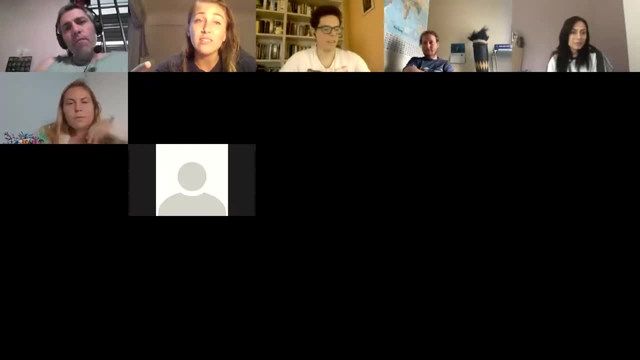 a series of talks on minimal creation, since you guys all did this one. if you want to do that, it's 20 off, no pressure, but he's awesome. so there we go, um and literally, if any of you guys have any questions right now, like just say it. um, you can unmute, you can type. oh, thank you guys so much. 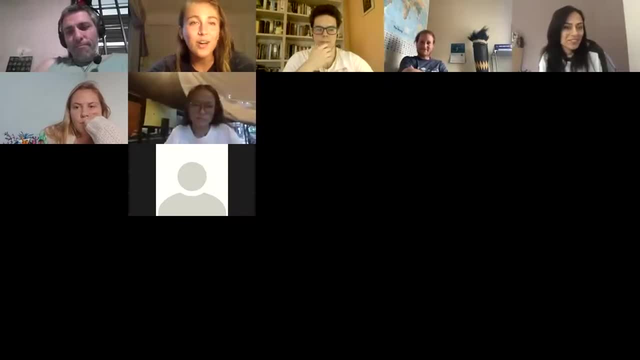 yay, i'm glad you guys liked it and i'll see you in the next one. bye, bye it. i hope you could tell that i was having a pretty good time. i love talking about corals, um. but yeah, really appreciate all of you guys being there. if you want to, you can start logging. 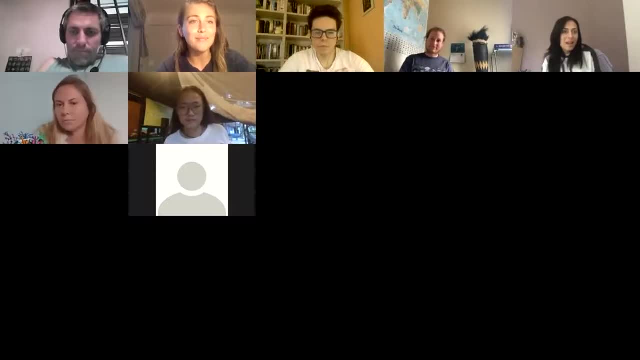 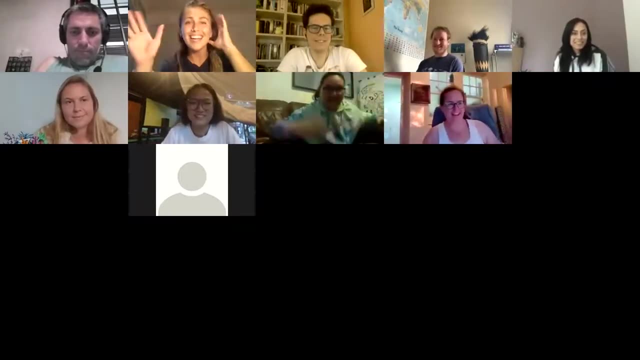 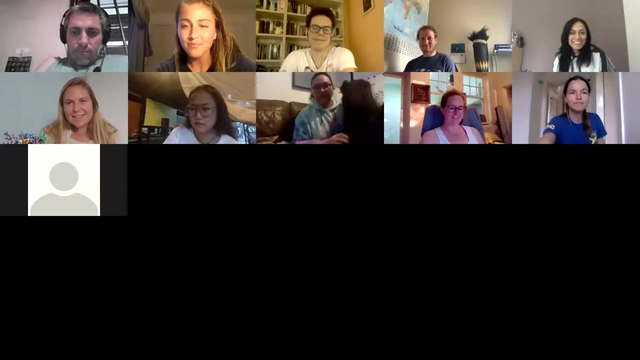 off. oh, actually, could we get a screenshot? could everyone smile, because i just love this stuff. yeah, you don't have to turn on your cameras if you don't want to. there's absolutely. oh, jade, hello, oh, alex, if you want to, though that would just be so fun, um, okay, five. 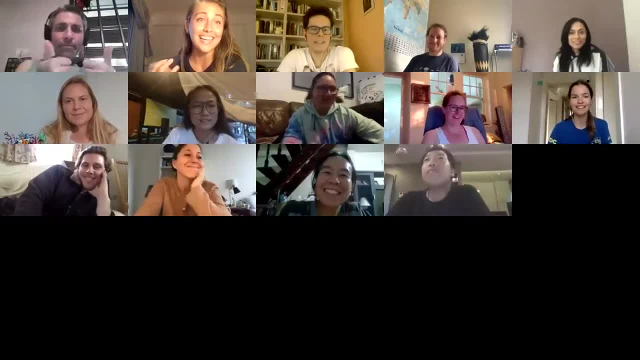 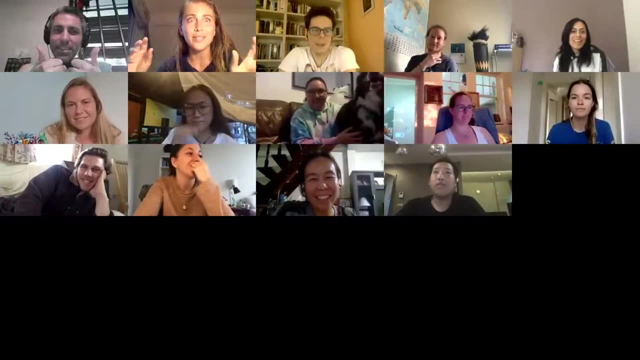 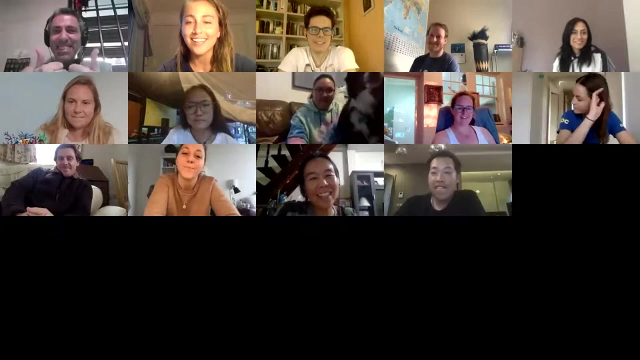 four. oh gosh, some more turning on. oh okay, i'll just wait for everybody in that case. ah, yay, was i understandable everyone? was i a little bit too loopy or was i sort of okay? awesome, i hope you felt the excitement from my end. okay, guys, three, two, one. 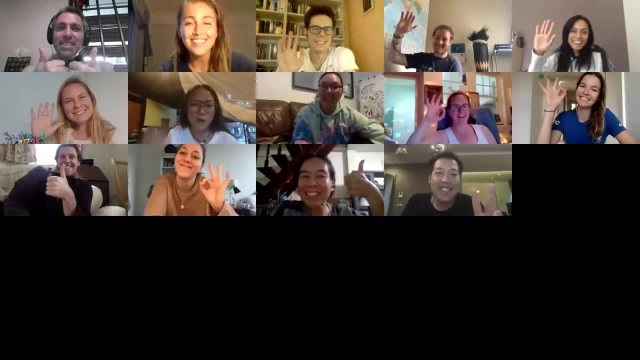 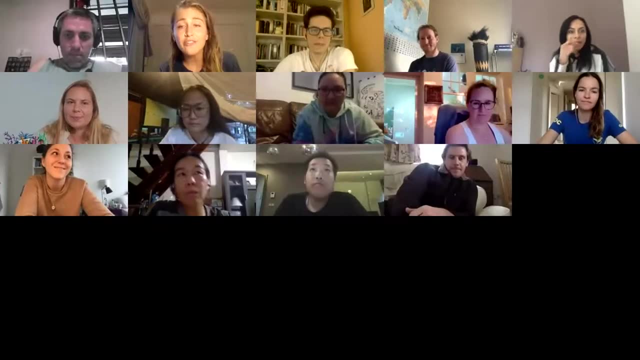 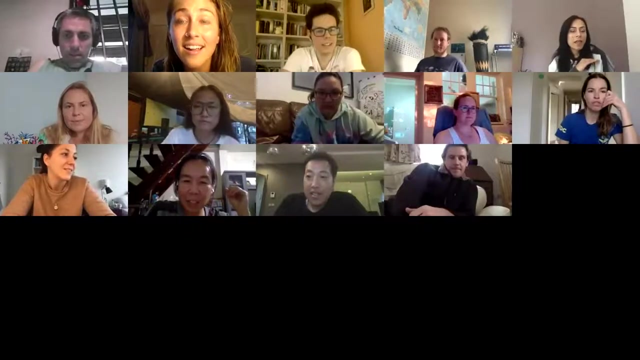 oh, thank you guys so much. i appreciate it. um, i'm gonna quickly paste that here before i lose it. um, yeah, feel free to log off. i loved having you. you guys were literally amazing. it was you guys. how are you guys doing under lockdown? you know everything that's happened in the world right now. 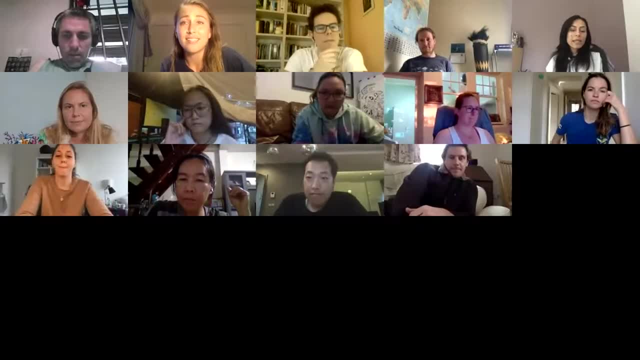 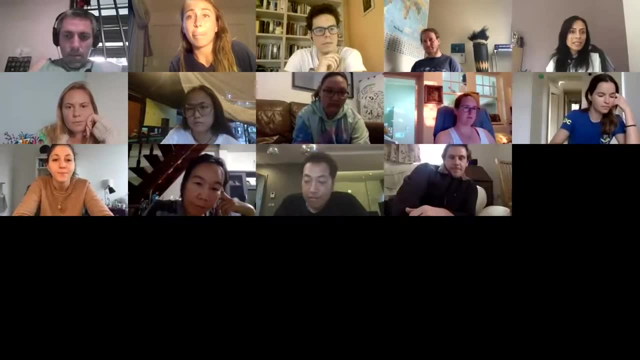 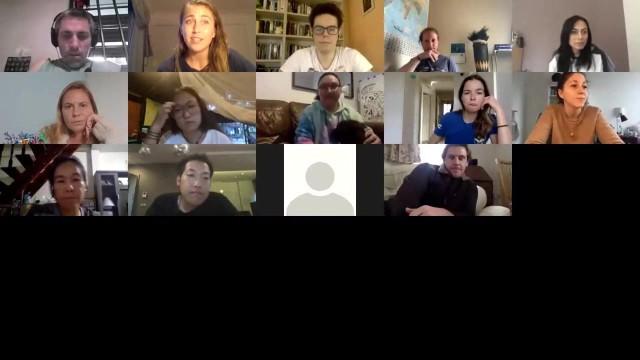 how are you guys doing in terms of getting out to the reefs and um doing your surveys? and also, how are the coral reacting to people being out of the water? well, corals, so there was a heat event last year. um, it wasn't like a global event, but some of our sites were recording like some bleaching, which 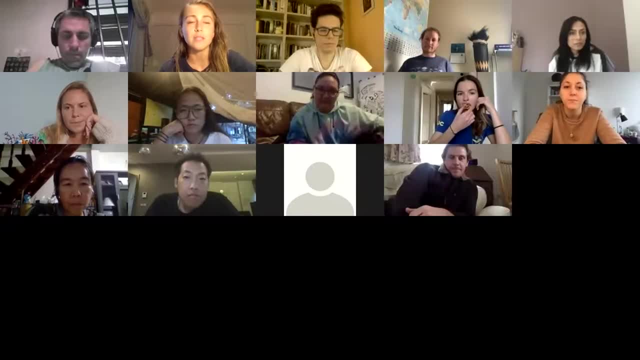 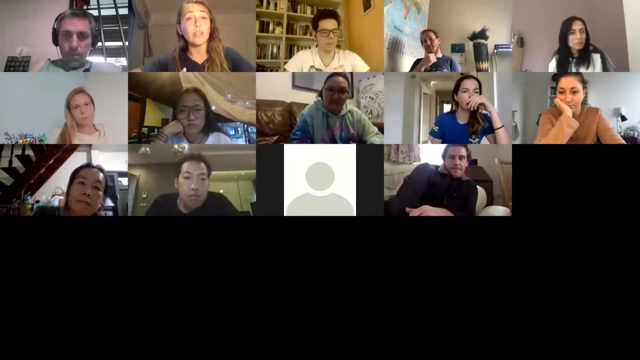 is an ideal, like i nearly you know, like it's not nice but the smallest part of me. i think a lot of people thought, oh well, if this is gonna take a little bit of pressure off of people being on the reefs all the time, maybe a little bit of good can come out of this. but of course there are other. 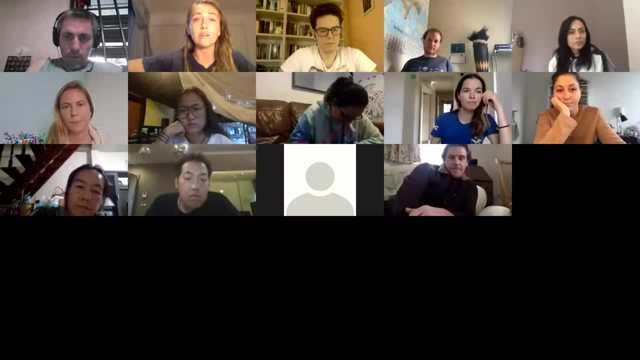 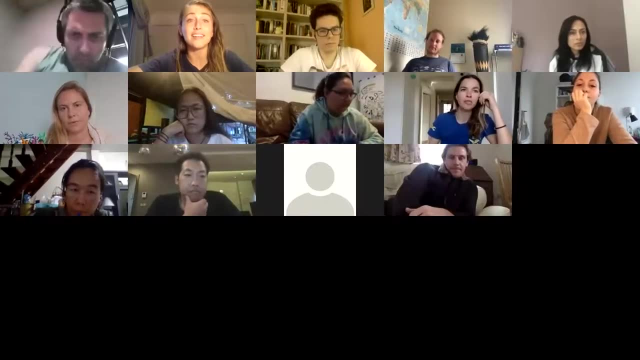 factors at play here: um, in terms of our centers, how are we getting out into the reefs? so we have got um instructors, so some of our instructors are going to be going to be going to the reefs. some of our sites are simply like the countries they're in: they are not accepting tourists. so in 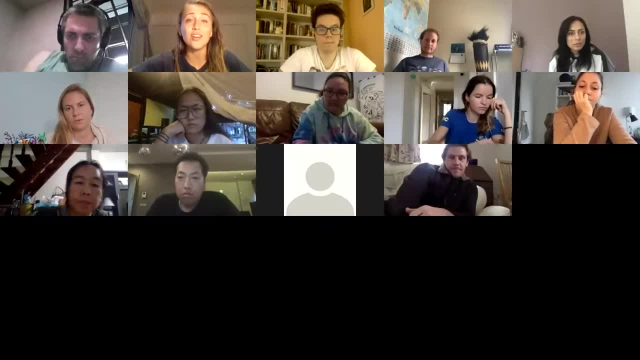 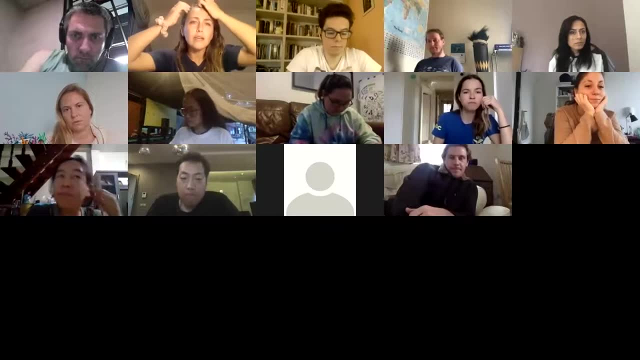 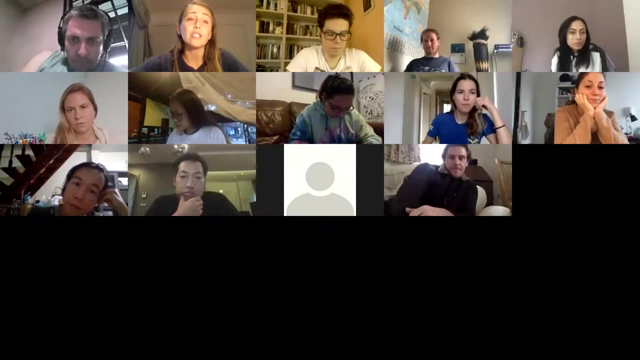 terms of like a program open for ecotourism and education and research. not much is happening, but we still have instructors at three, oh yeah, at three- of our centers, one, that's more, four if you include one that's about to be open. um, they are pretty much catering to local, uh, like customer. 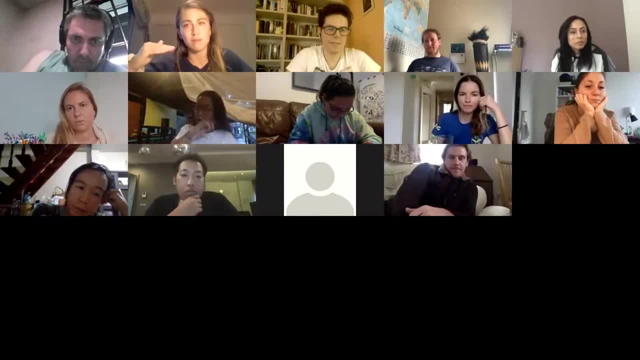 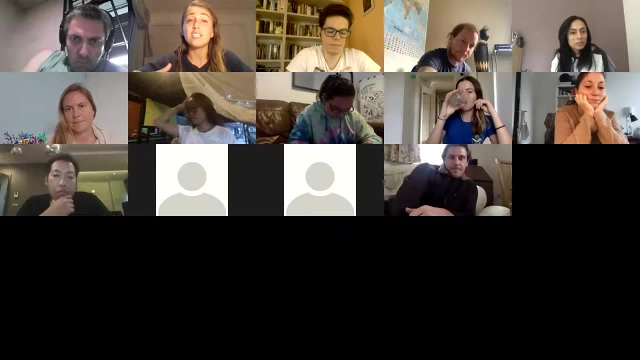 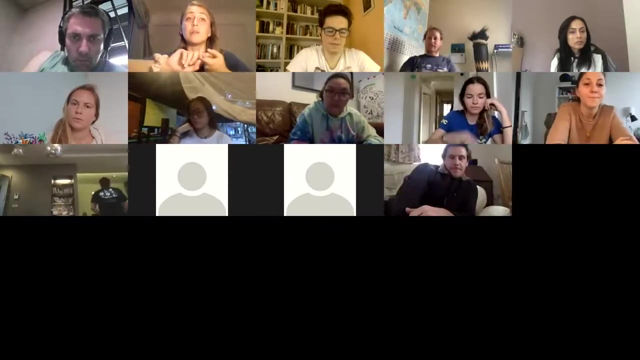 basis. they're still going, but it is a much smaller level to what it's going out before. one of our um locations isn't manned with one of our instructors just because of you know the circumstances. he stayed for as long as he could until he couldn't, and he's um struck up a deal. 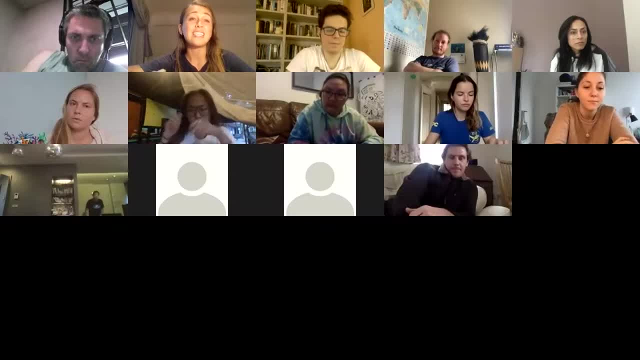 with some of the other conservationists on the island, essentially like taking them through the ropes, sort of said. you know, keep keep an eye on things as much as you can, and they were super wonderful about it. um, so things are definitely working at less of the capacity. we just want. 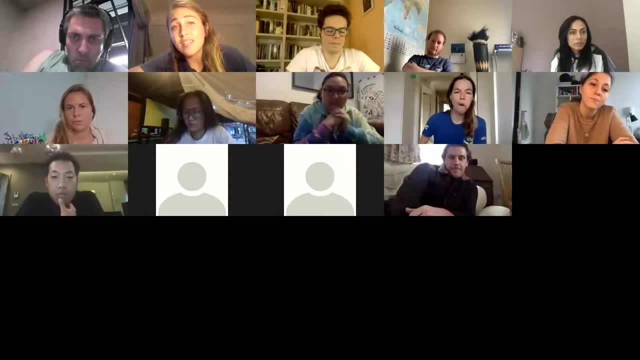 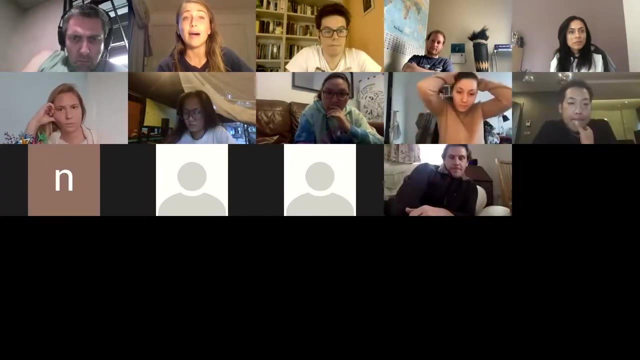 people to sort of remember: hey, we're still here, we're trying to have more of an online presence than we used to like. obviously, some people are saying: you know, like i wanted to do this marine conservation, now i can't get out of the field and like we feel that, like like a lot of us aren't either, i'm not at any. 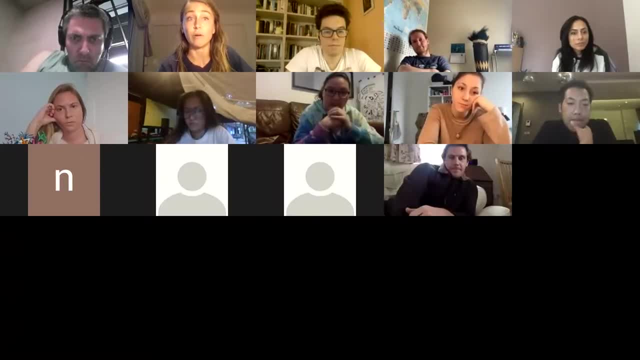 of our centers anymore. i was working full-time in our centers for two years before essentially was coming home to australia to say g'day before going back out and then got stuck here. so i decided to go back and do postgraduate because i was like, oh my god, i'm not going to be able to do that. 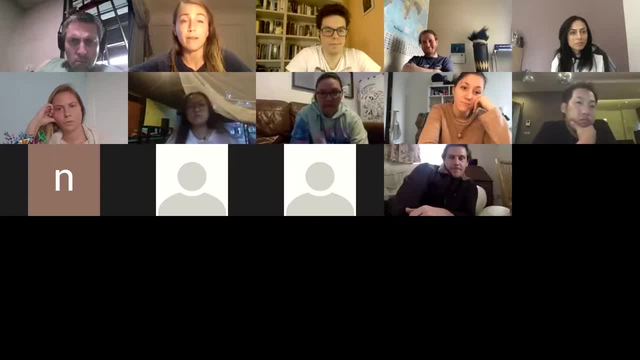 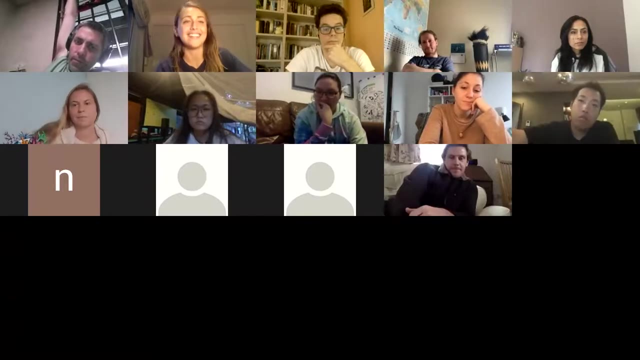 oh, i might be stuck here for a while, so i may as well. um, a lot of people don't realize, but australians are not allowed to leave australia, so we're locked in. um, it's working well, but i physically can't go anywhere right now. um, thanks for the nice messages, guys. um, but yeah, so we're. 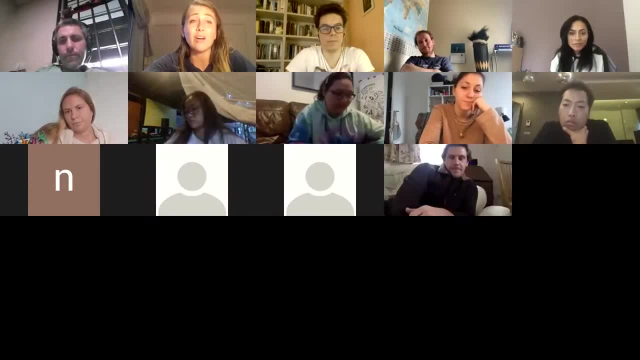 pretty much just trying. we heard, like we got questions from people saying: you know, i still want to do this course, we still want to do this course. and yeah, unfortunately, if you're not at like centers, we can't do the diving course. we can't do the diving course. we can't do the diving course. 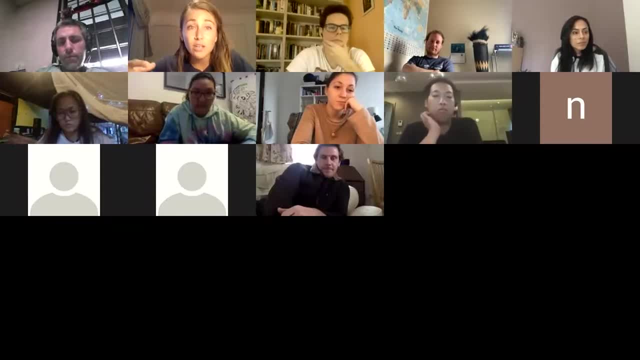 but, like we are so happy to provide the theoretical, to at least still keep people, you know, in the mode of: okay, i'm learning, i'm still. you know, there's not. it's not just conservation. you don't just go out and pick up corals and that's conservation. you have to know. 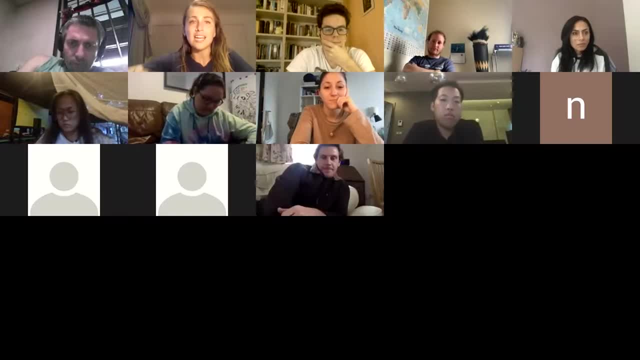 the theoretical. you know constraints and understanding before you go. do all that. i mean this lecture. for example, to collect in-depth data, you need to have an understanding of coral taxonomy. you know. so, even if maybe you guys aren't right now doing this course, you need to. 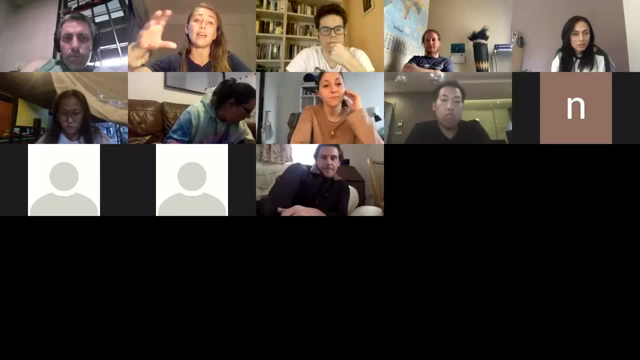 have an understanding of coral taxonomy. you know so. even if maybe you guys aren't right now doing work, if you were to go into the field later, or if i were to go into the field later, this knowledge is essential for doing that whenever that does happen. so we're still just trying to remain. 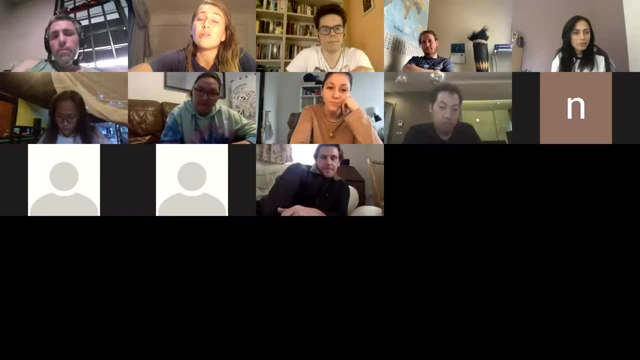 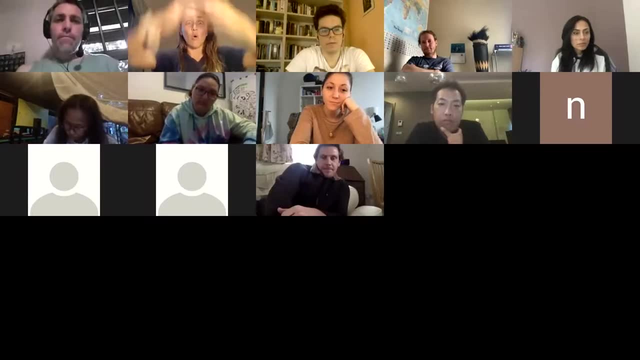 present, even if it is online. we're also just launched a patreon which we kind of want to make a more cost like, like a cost-effective way for people to access like all of our stuff. we're going to be giving advice on everything from, like some of the content like this, but also largely 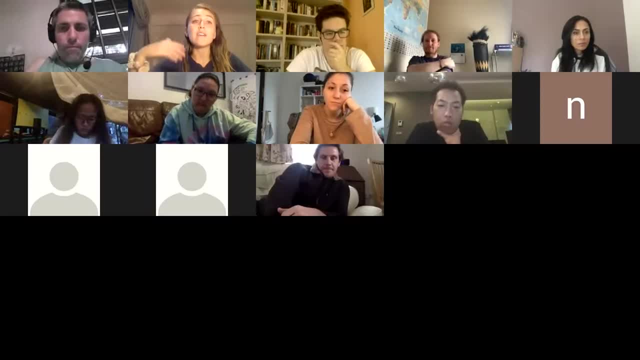 like advice, like: how do people like you and me, how do you get the information that you need to me? go out there and realistically start like a conservation or conservation diver program, you know? like what constraints might there be? like what permissions might you need? what business models can be useful? are you going to be a non-profit or a social enterprise, or you know? 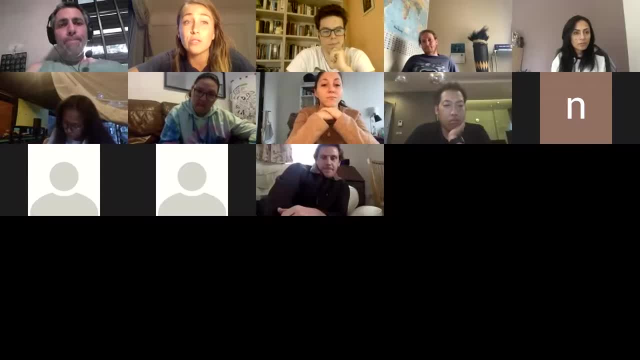 whatever it's going to be. so we're trying to provide support in those sorts of ways, you know, to at least sort of give people something else to work on when they can't necessarily be in the field doing stuff, doing work- um, that was a long-winded explanation, but yeah, so we do have some stuff doing. we're having 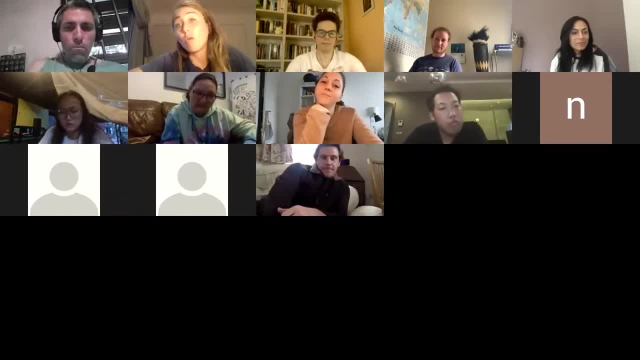 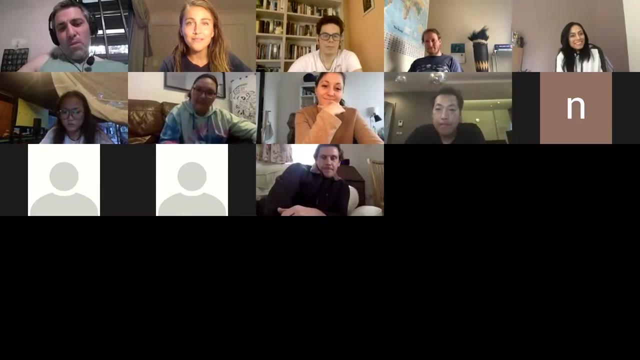 happening at our locations, but not as much and not all of them at the moment. it's just sort of what it is. yeah, anything else are we going into? corals conservation, diver, anything like that? i'm so thirsty after all that. yeah, cool, surprised you got any. 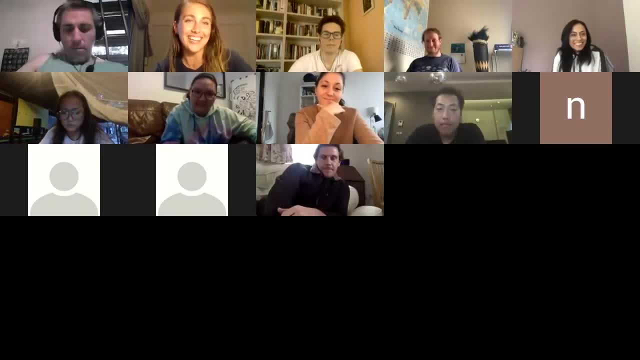 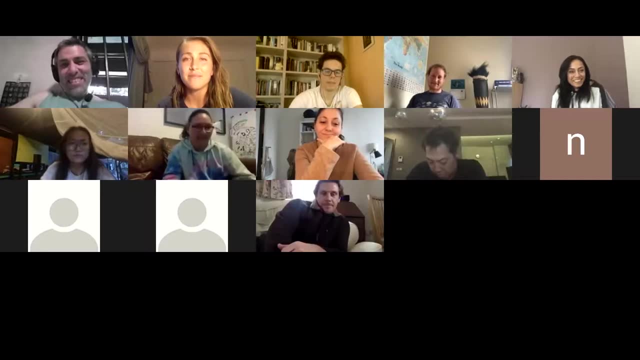 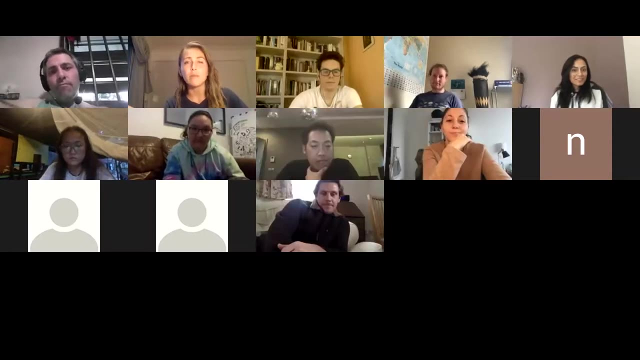 voice left. oh, trevor, i can talk, if you hadn't noticed already, yeah, um, but yeah, really appreciate having you guys all here. i'm just going to hang around, like in case some of you guys want to ask some questions, like when there are less people logged on, so feel free to log off. some of you guys probably have like. 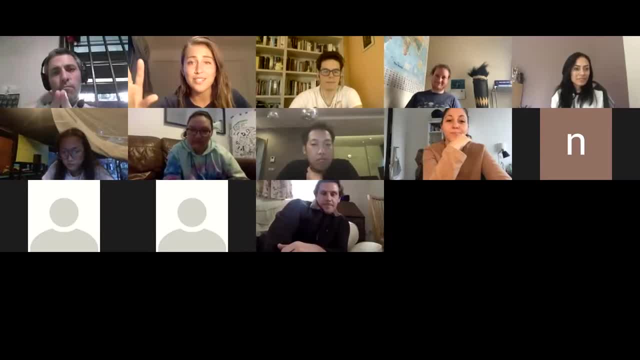 lunch to eat or dinner to eat. i know there was a jade is, i think, down the road from me, like in perth, which is amazing. um, we've got to be really close. perth is not a big place for everyone else out there. the most isolated, teeny, tiny city in the world, um, but yeah, so anything else, i'm gonna log off. 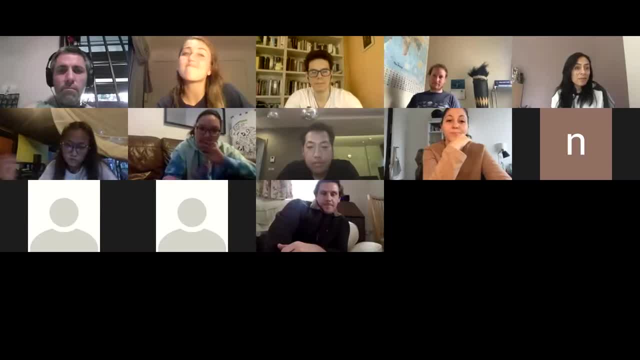 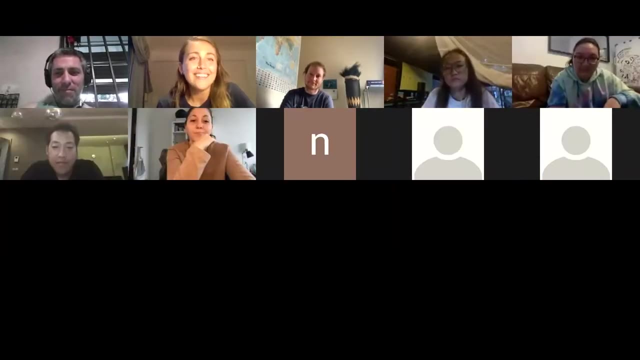 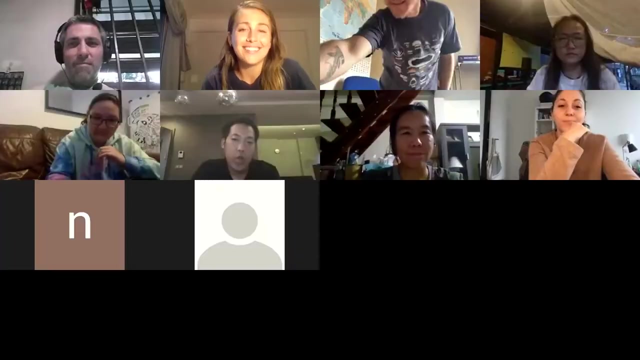 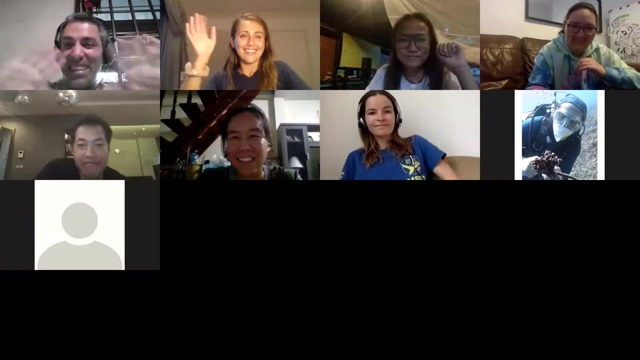 um, ellie, and i'll probably email you at some point. absolutely all right, it's been great. thank you so much for having me again. no worries, have a great love you bye cool. thanks for that. no worries, thank you so much for joining. yeah, that was awesome. be in touch soon. 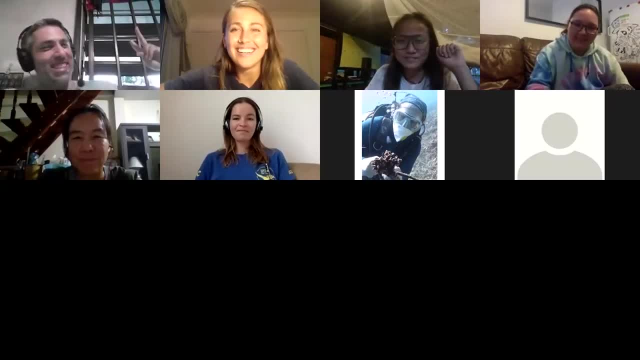 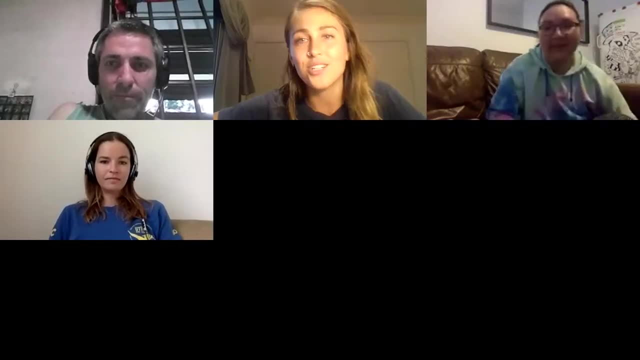 yeah, email whatever you need, absolutely good, yeah, lovely, thank you bye. thank you, bye-bye, bye. see ya, 바나 in braces. what's this, alex? do you want the exam? you're the one that initially inquired about the, about having another taxonomy presentation. only if you want to, i know you've done it before, so. 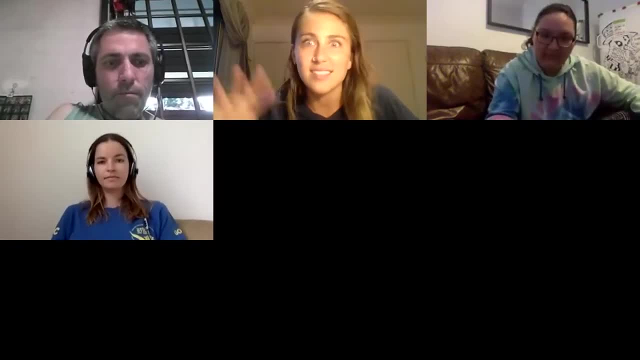 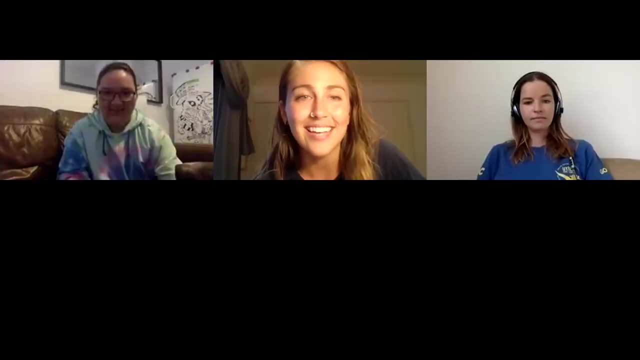 you don't have to um, but if you want to test yourself again, obviously i'll send it through. you can do it as as you, as you enjoy, as you want to. oh, yes, please, if that's all right. yeah, of course, too easy, awesome, great, cool. oh, just a couple of us now, wonderful. 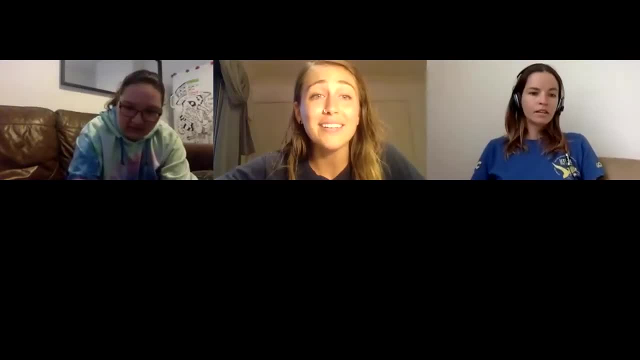 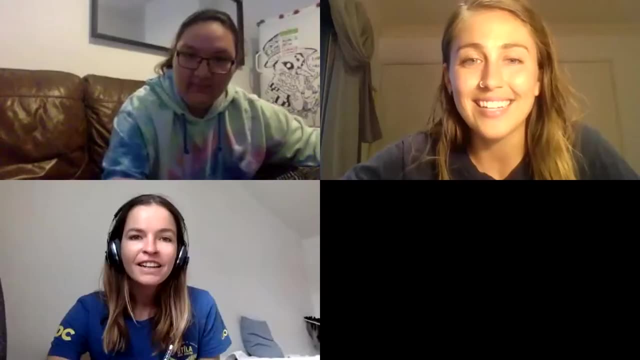 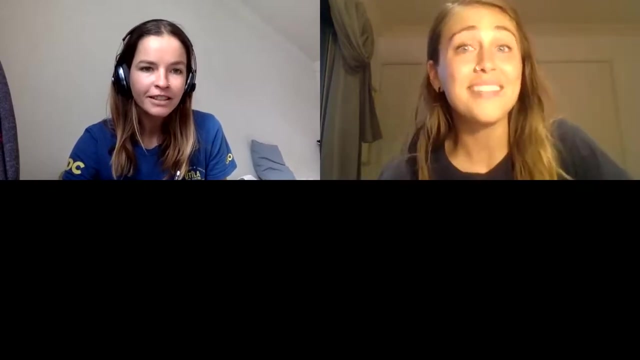 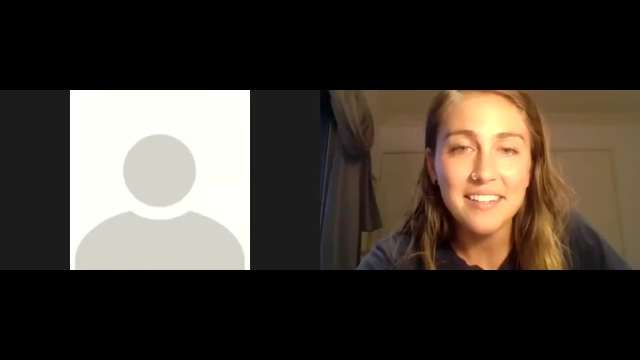 thanks for joining, natalie, by the way. yeah, no worries, thanks for the offer. yeah, it's absolutely amazing. yeah, glad you enjoyed very much. so all right, okay, well, hope you have a good evening. yeah, you too, talk to you soon, okay. all right, then, louise, i'm not sure if you're still there, but it's been really wonderful. 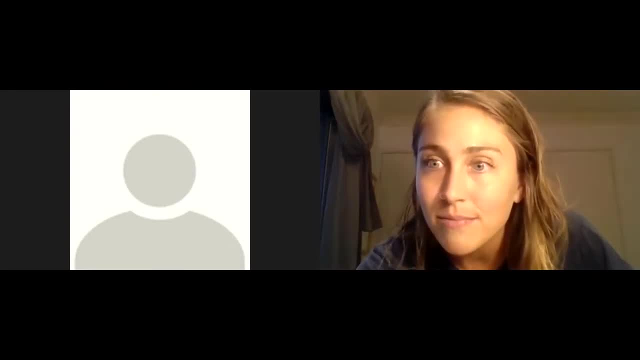 thank you so much for joining us. i'm just going to read through some of these messages and then i think i'll probably end the chat. um, but feel free to speak or to text if you want. uh, i'll write on the thing. yeah, all right, all right. 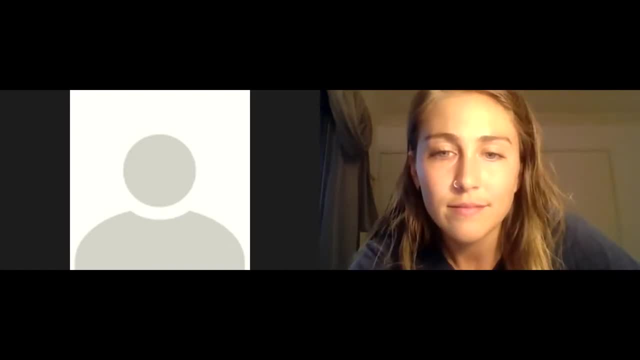 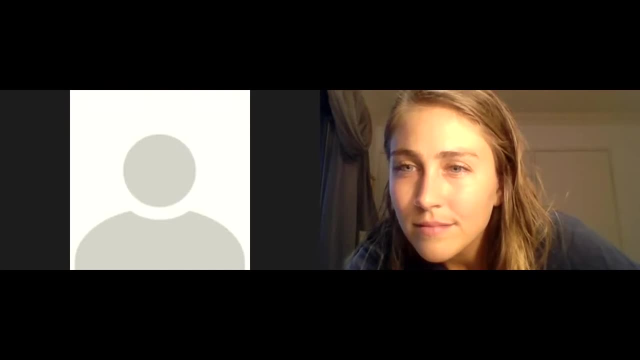 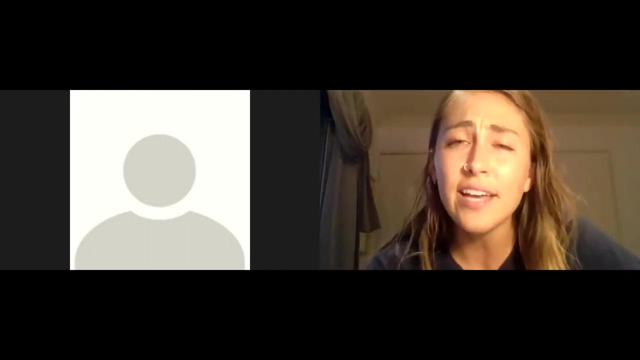 you some nice, nice people. oh message. hey, hey, louise, thanks, mash, okay, so we don't send out the whole slideshows. um, we used to and it's a little bit silly, but something like we did have a couple of people end up like sort of. 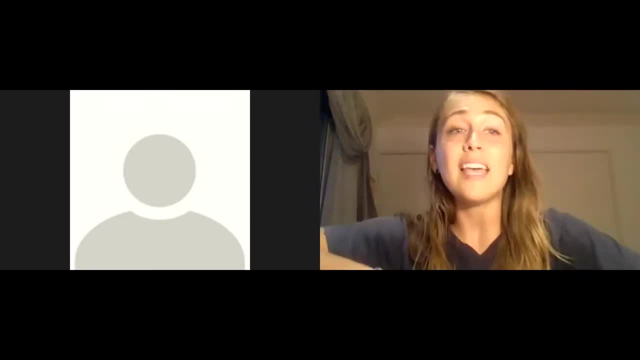 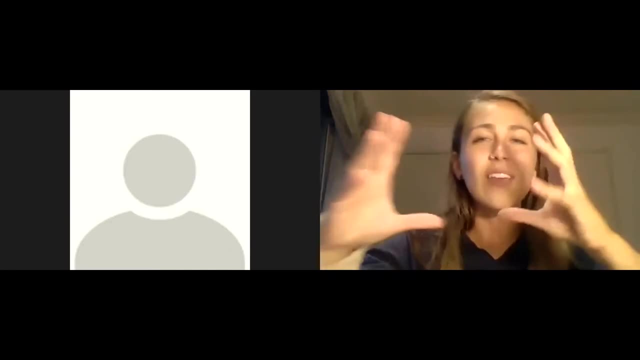 like. i know it sounds silly, but sort of selling it. um, but let me know, even if you want like a list of those corals and i'm happy to send you sort of like my own pictures, but just sort of like with the whole setup, with like our logos and stuff. i won't be sending you the whole thing. 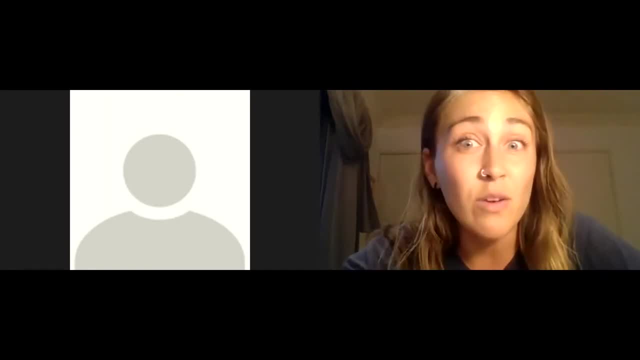 um, but yeah, if you want more photos, a list again, or even just like the family names, the genus names, so happy to send you whatever you want. um, if you want, just send me an email. i guess sort of exactly what you want in that regard, like, if those corals- i don't know if you're a diver or snorkel already- 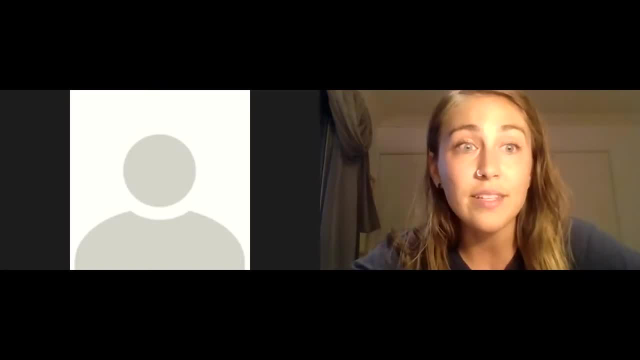 like she was pretty reflective of what i've seen. um, yeah, just just chuck me an email or send me another message right here and um, i'll send you through a list, happy to send you some of my own personal photos. nearly all the ones on these slides are compiled from our team, plus a couple. 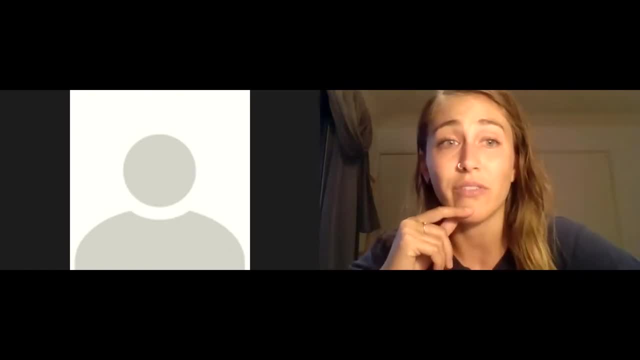 of other which are credited, but like we've got so much um that we can provide um, so yeah, um, and also let me know if you want the exam as well. um, there's no like rush to do it like you guys. you don't have to do it right now. you can do it in your own way. so i'll see you in the next one. 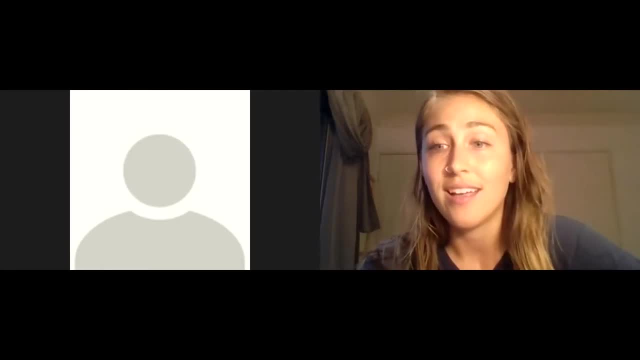 in time, but like so happy to provide some feedback on that too. um, so, yeah, um, and thank you. uh, yeah, so much for joining, louise. we've got pretty similar names. um, mine's eloise. so nice to meet you. um, yeah, oh no, yeah, i understand. 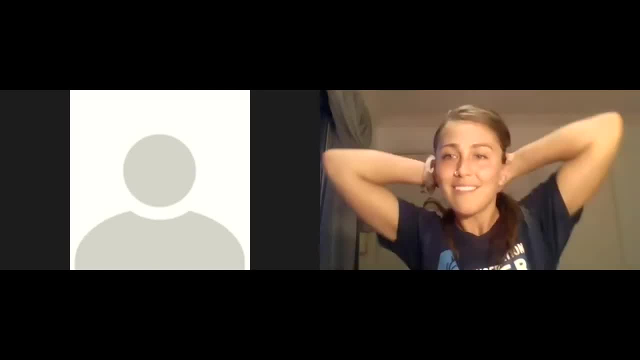 not a problem. um, at least fortunate. ah, awesome, beautiful. well, just if you do change your mind, you just like want some extra photos to work with everything's googleable, but just because there has been like a massive shift in. not a massive shift, but, like you know, taxonomy is. 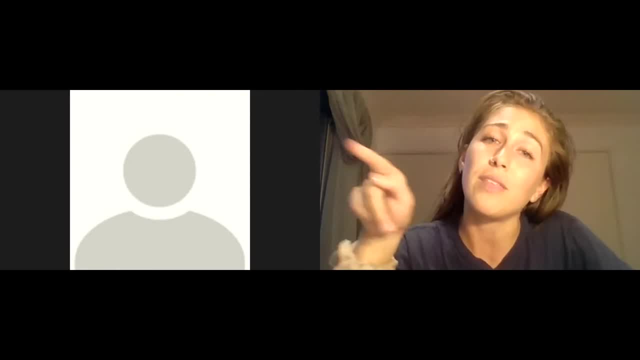 changing and being updated. if you're ever like unsure, if you're seeing multiple things come up for one search, feel free to message like whenever you like, because i really do love this stuff. if you can't tell, um, but yeah, i've had you for long enough, so yeah, i'll let you go and um, yeah, feel. 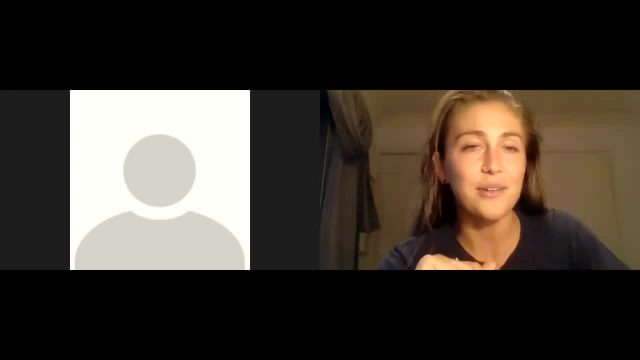 free to email and have a good morning, night, middle of the day, wherever you are, and, uh, yeah, have a good one, awesome bye.